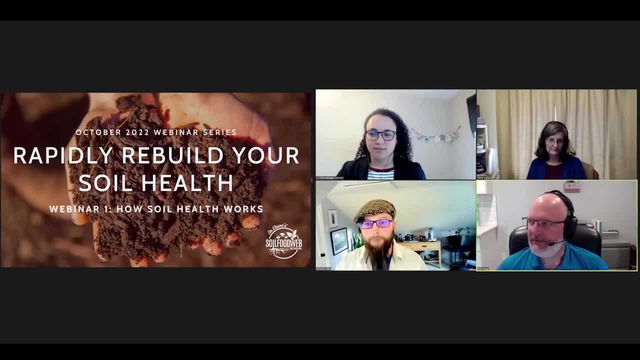 in the chat window, go ahead and type where you're coming from. We always like to see kind of where our audience is from around the world And usually it's a very international audience. I see people coming in from a lot of from the US- Oh, all over Europe. 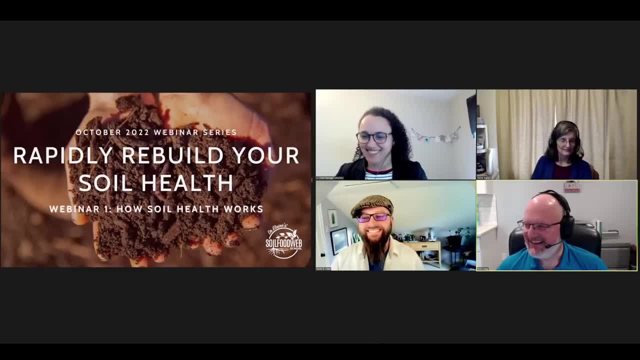 It's moving so fast I can't even read them. It's crazy. You name it. the country's in there Pretty much. Yeah, It is like it always. always amazes me how many people we have internationally joining our webinars, So this is fantastic. It's great to see that interest. 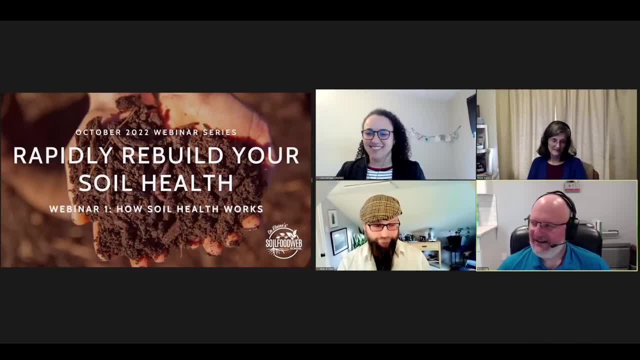 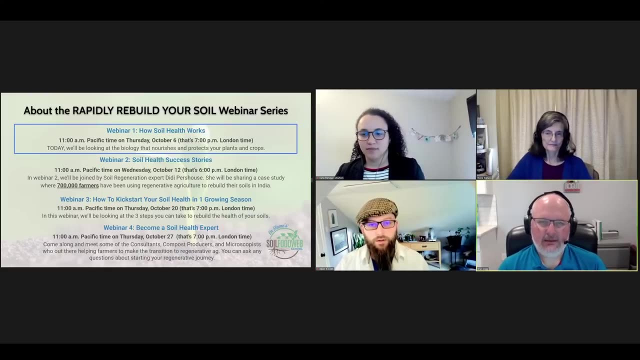 worldwide. It totally is Okay. Well, thank you folks for joining. Let's go ahead and get started. We actually have quite a bit of content to cover today. So before we actually really get into the meat and potatoes of our webinar, let's go ahead and talk about the upcoming webinars for 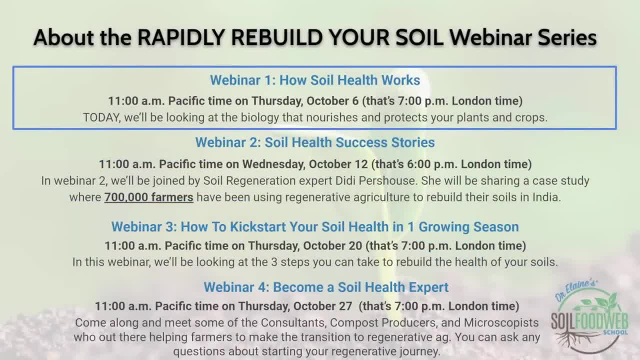 our October promotional series. So, as I mentioned, today's webinar one- how soil health works- And then we're on October 12th. We're going to have webinar two, which is soil health success stories, and Didi Purehouse will be there, So it'd be great to have her as a panelist. 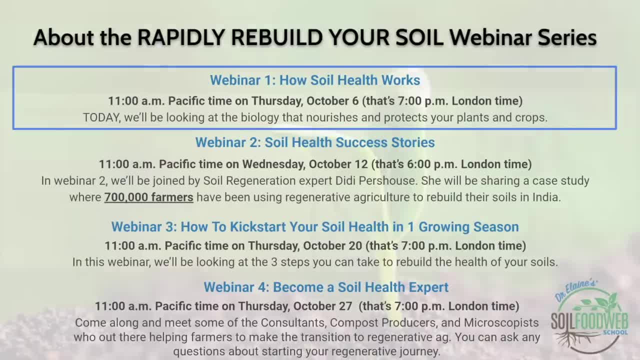 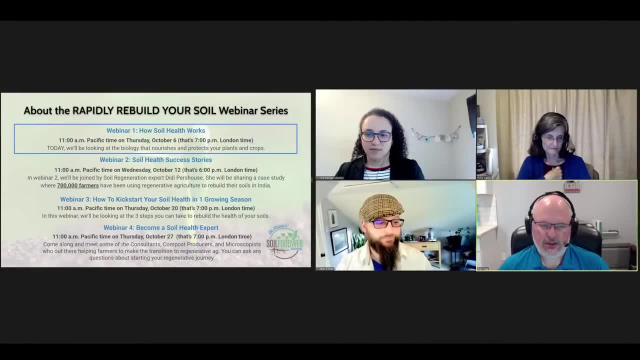 And webinar three is how to kickstart your soil health in one growing season, And that's going to be on Thursday, October 20th. And then we have webinar four: become a soil health expert. You'll be hearing from a number of the consultants and compost. 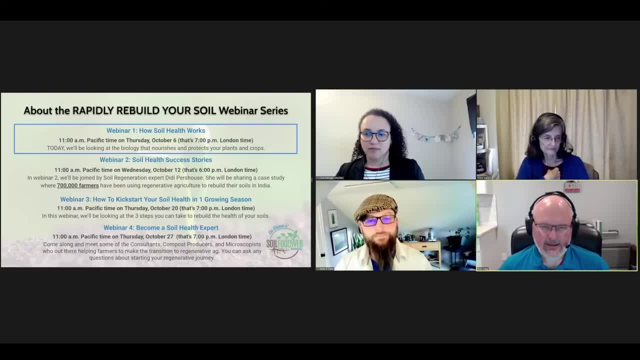 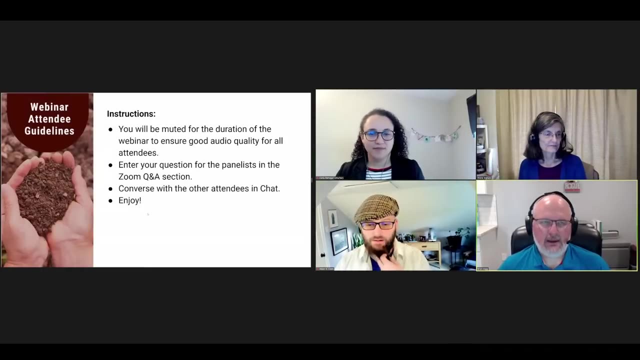 producers and lab techs, And that is on Thursday, October 27th. So hopefully you will be able to see you all on these other three webinars And, if not, they'll be recorded and you can definitely go back and watch them. Okay, Let's talk about some of the guidelines, Since we have so many. 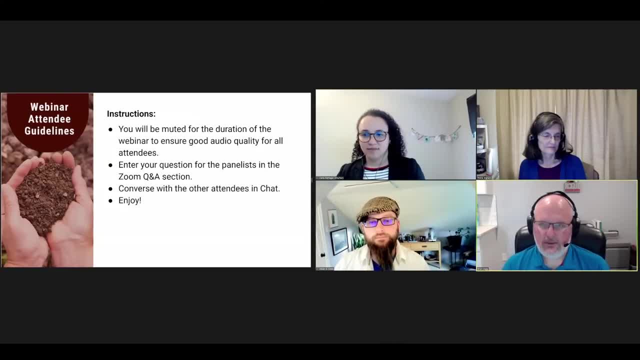 people joining. everybody will be in a muted mode for the duration of the webinar. Just make sure we cut down on background noise And besides the panelists, so we'll have the panelists on there And then also we'd like to 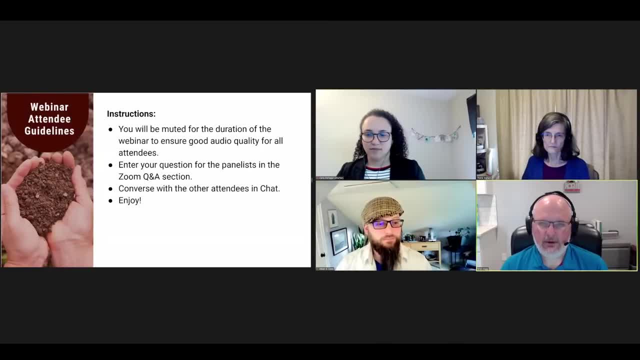 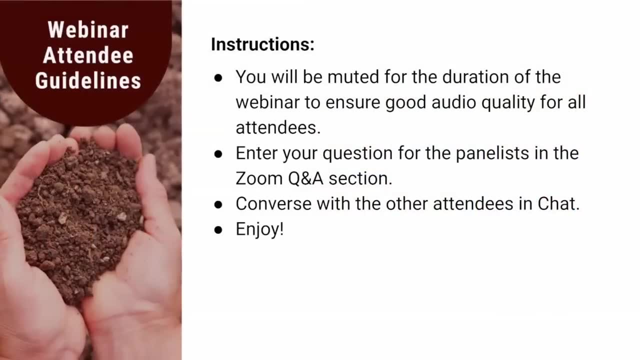 hear questions from you. We have really. almost half the webinar is for Q&A today. So at the bottom of your Zoom screen there should be a Q&A button, And if you go ahead and put your questions in there, that's fantastic. We'll put them and we'll choose the ones that we can have for our panelists. 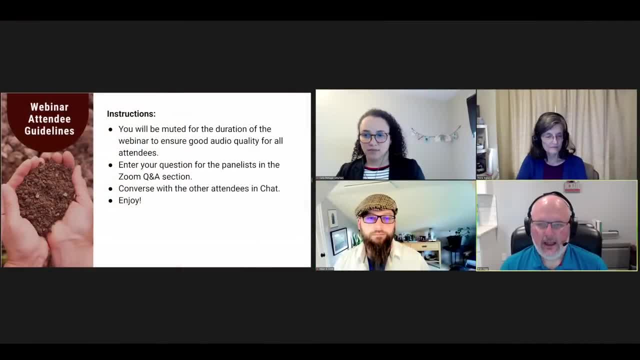 that would kind of make sense for the flow of today's webinar. And then also we encourage you to do that in the chat window. So just make sure that if you have questions you want the panelists to answer, you put them in the Q&A, And if you want to be able just to talk amongst 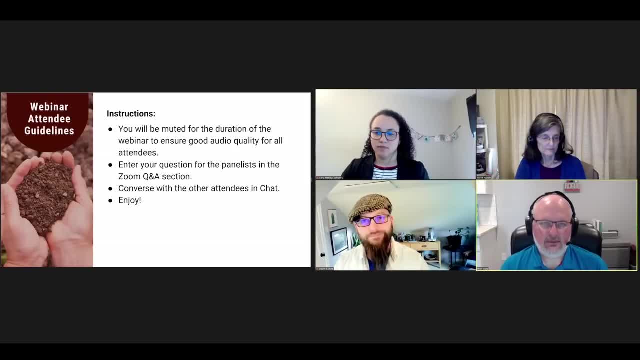 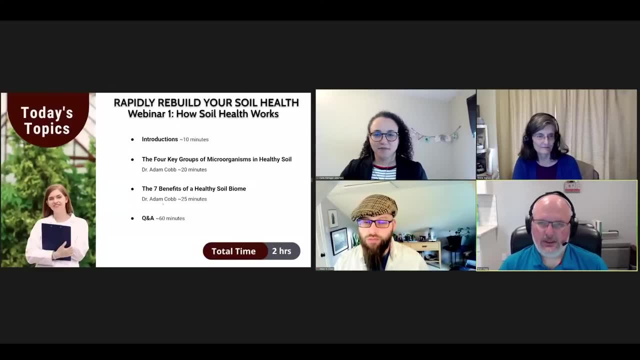 yourselves. that's where you would go ahead and do that in the chat. So please go ahead and enjoy today's webinar. So topics for today. we're just going to go through some introductions, introduce the panelists and kind of go through some of the housekeeping that I'm going through right now. 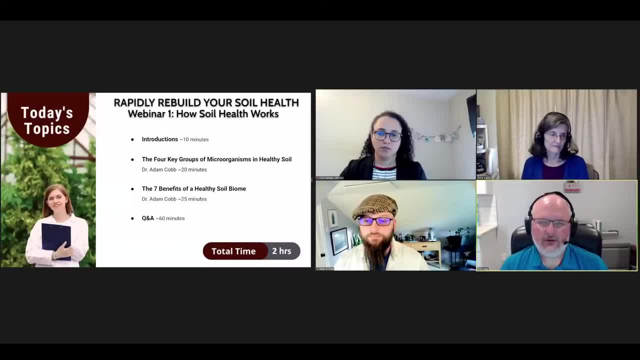 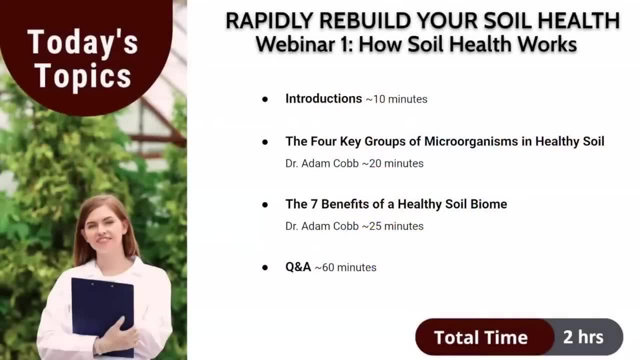 And then we're going to have two presentations by Dr Adam Cobb. The first one is the four key benefits in a healthy soil, And then the next section will be the seven benefits of a healthy soil- bio, And then, when Adam's done with his presentation, we'll have a short video and a 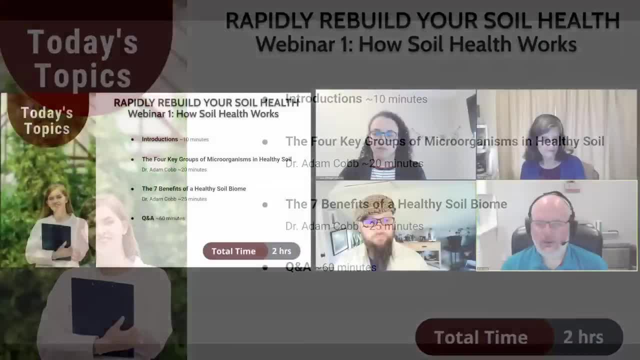 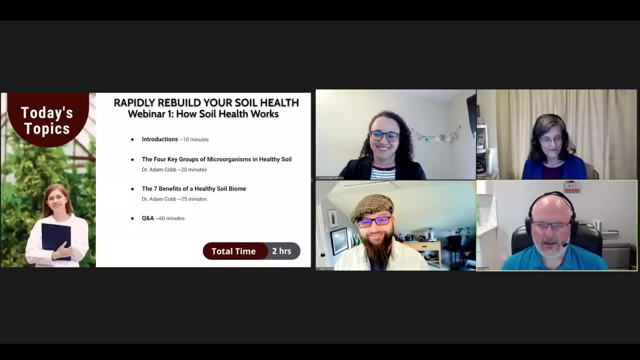 description of the promotion that we're doing for October. And then we'll jump right into Q&A And again, I always love the Q&A. You guys always have such great questions And it's fun to see what the greater group is thinking and wanting to know, And we expect that today's webinar is going to take. 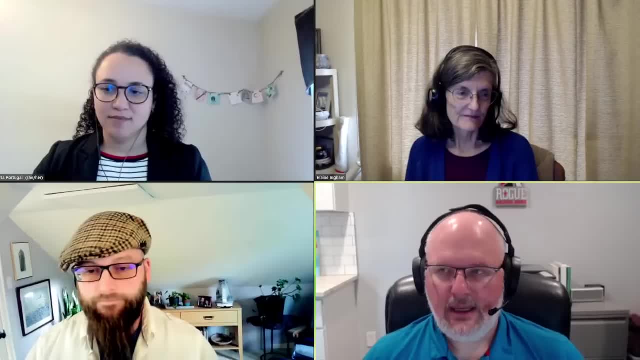 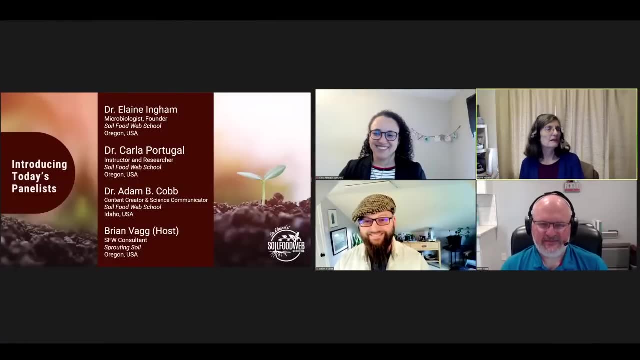 about two hours. Okay, so let's go ahead and introduce our panelists. So, Dr Lane Ingham, introduce yourself. Oh, I'm a soil microbiologist. I've worked in that area for something like the last 40 years. 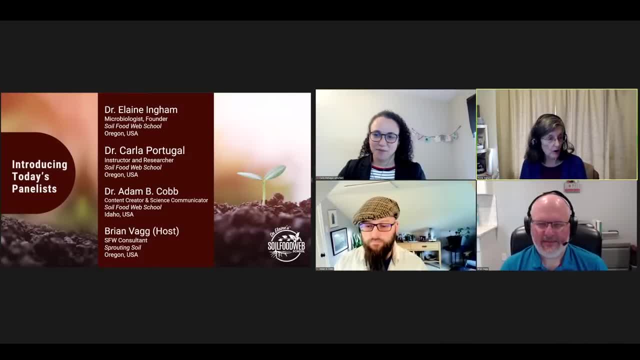 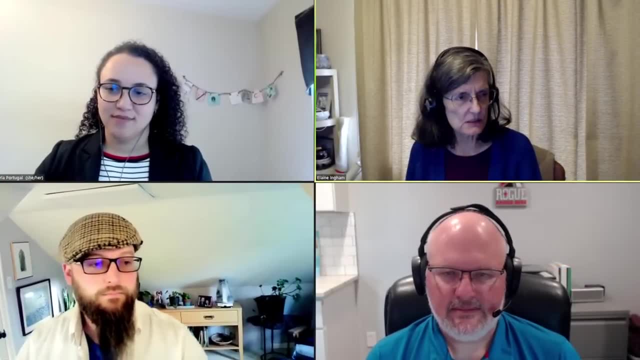 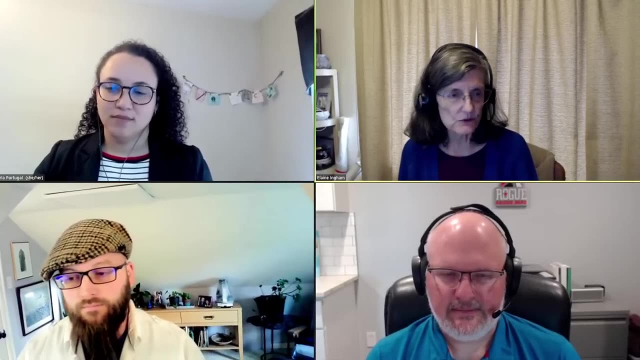 I've worked on the organisms that grow and find soil their home site. So, understanding the conditions that select for the beneficial organisms that you need to have in order to grow whatever crop it is you're interested in, we'll have to add subtract. 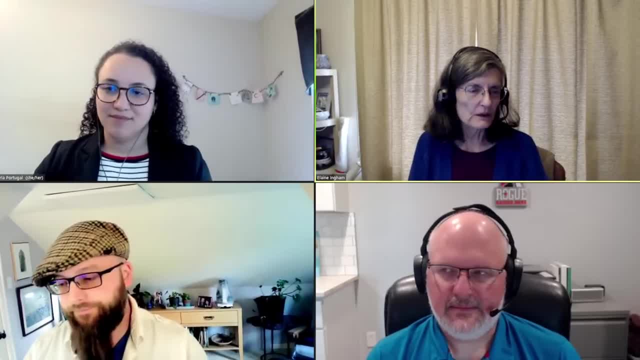 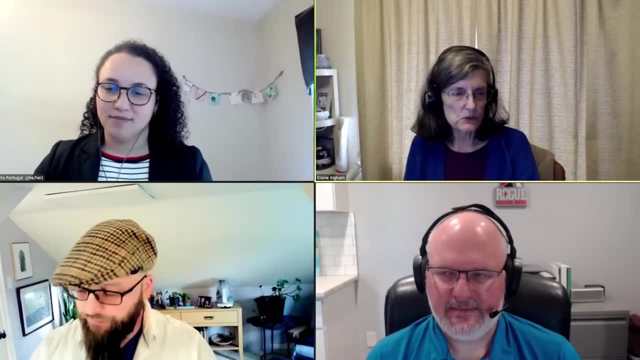 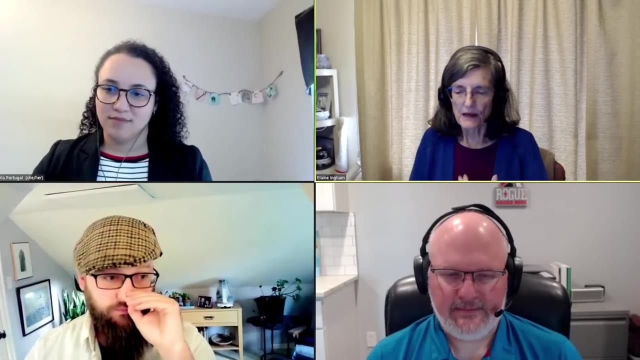 multiply and divide the different sets of organisms so that it matches what your plant requires. And so all of these interactions between organisms in the soil, so your plant can be the healthiest. no diseases, no pests, no problem organisms will attack. it's got all the nutrients it needs. So 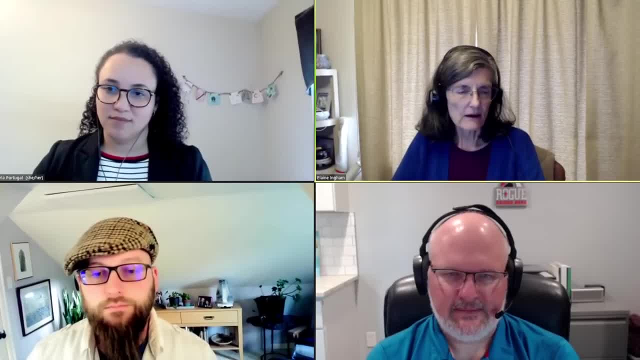 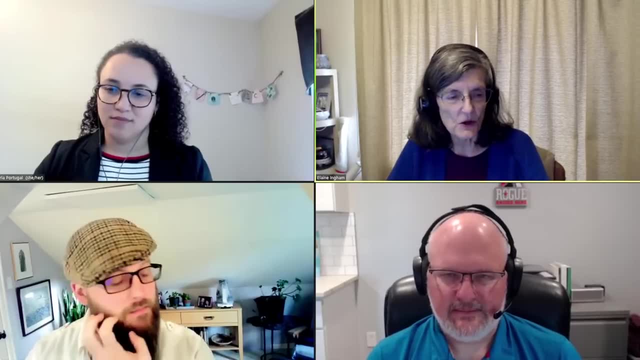 So it's never stressed for a lack of food sequesters the most carbon in the soil. there's the whole list of various things, So if you want to learn more about that, please come and take our foundation courses. Thank you, Elaine. 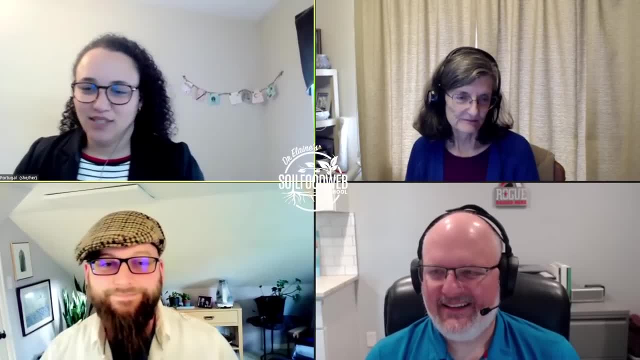 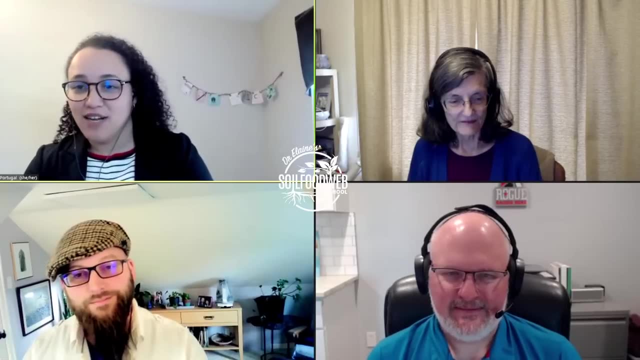 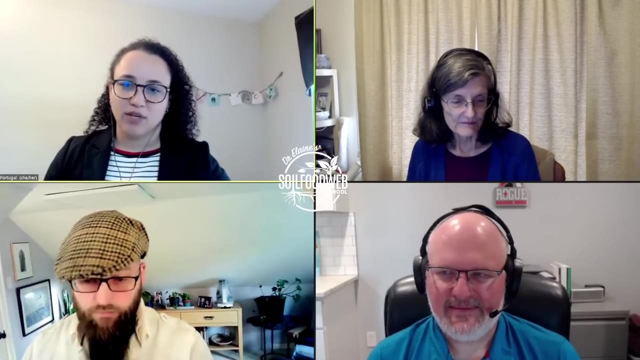 All right, Dr Carla Portugal. Hi everyone, It's a great energy being here, seeing people from everywhere around this globe. Thank you all for coming, And I'm a biologist by background. My PhD was in environmental sciences. look for green alternatives to reduce erosion in. 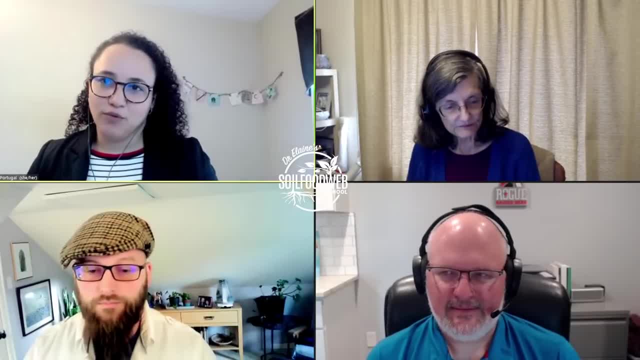 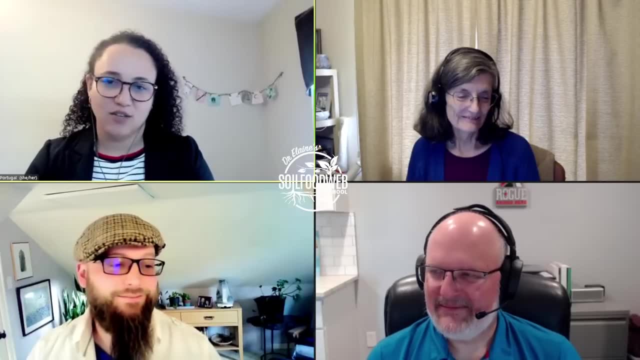 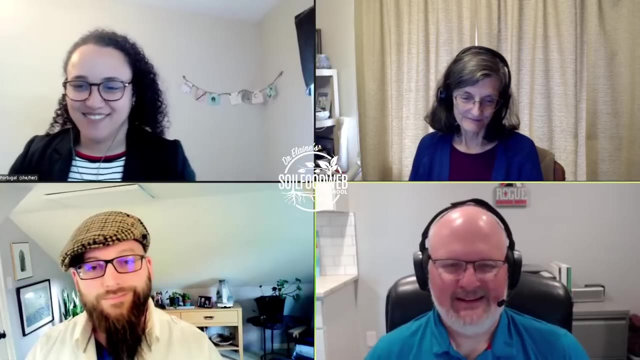 dirt roads, And working in school helps me to fulfill the gap between academia and all the hard work you guys are doing out there. So it's a very, very rewarding career and hope to see you guys in our classes. All right, Thank you, Carla. 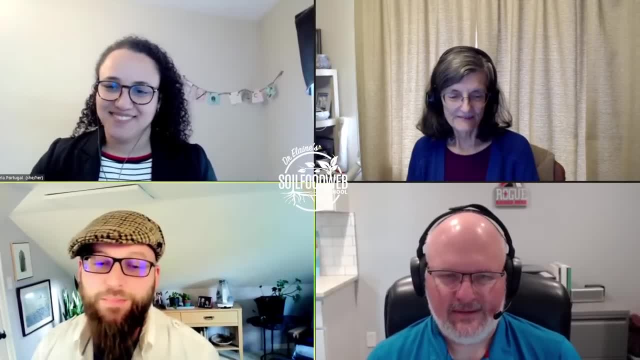 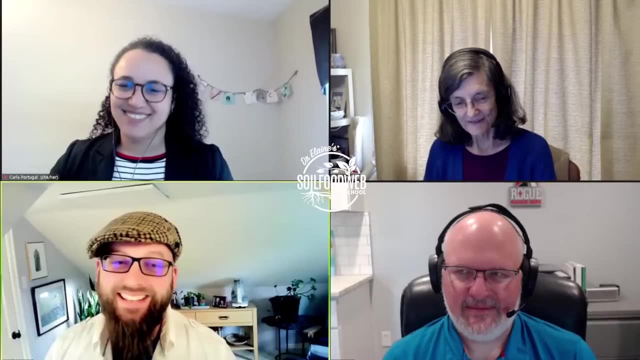 All right, Dr Adam Cobb. Hi, I'm happy to be here today and talking about soil health and soil biology with some of my favorite people in the world And my background- some of you may have seen in previous webinars that I have some I had. 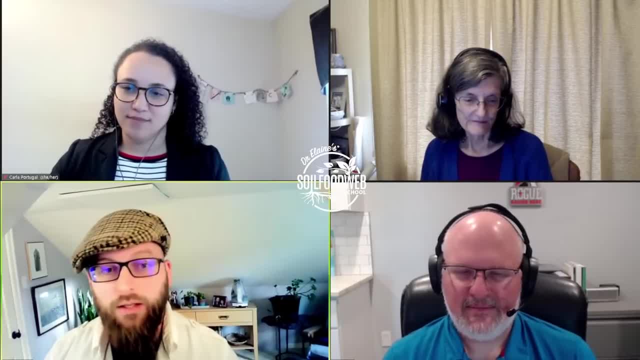 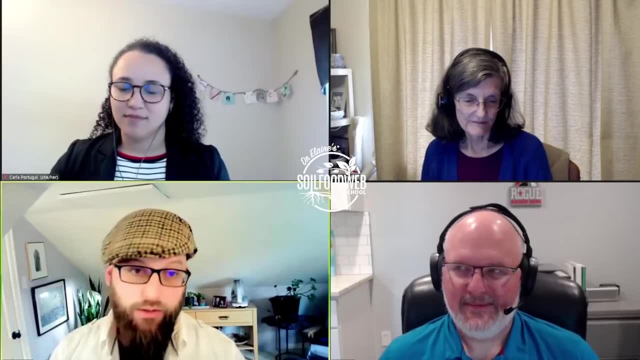 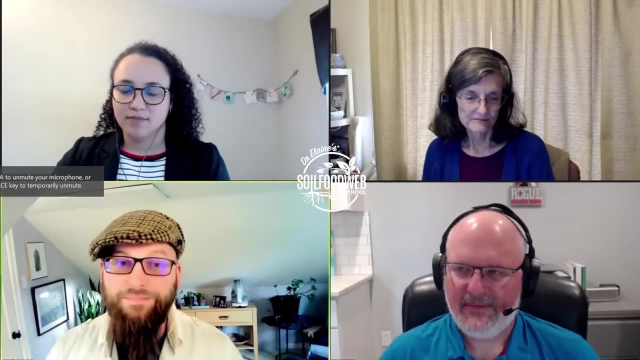 about 10 years in academia, primarily studying mycorrhizal ecology, especially the arbuscular mycorrhizal fungi in agroecosystems like grasslands, row crops and such, And so I've been At the school for about a year and had new horizons open to me about all of the many 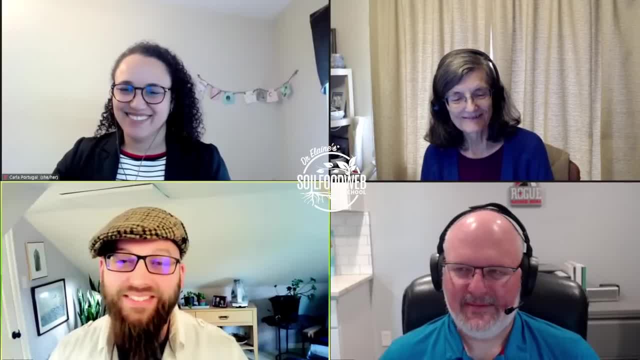 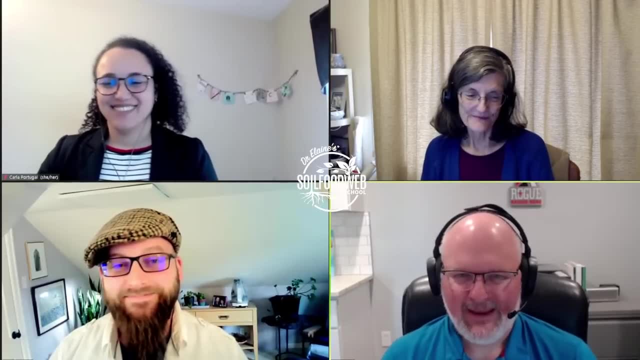 other wonderful critters in the soil. So I'm just happy to talk about about how it all comes together today. Thank you, Adam. And then I'm your host for today. My name is Brian Vag. I am a soil food web consultant. 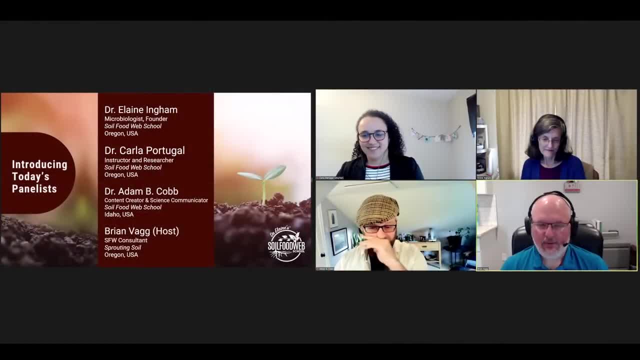 I own a company called Sprouting Soil And I really have a large variety of clients that go from Homeowners, homesteaders, landscape companies and a lot of industrial food nut crop vineyards and so forth. So it's great to be on with such an esteemed panel of guests today. 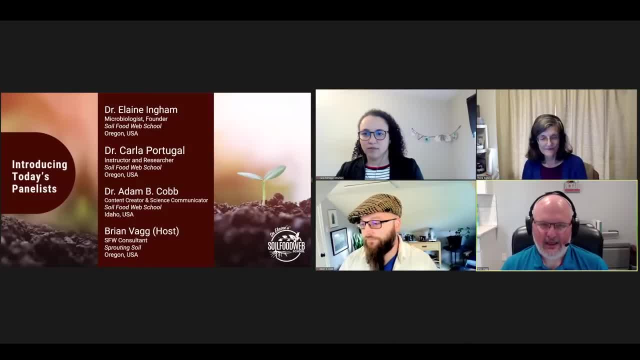 So, all right, Without further ado, let's go ahead, and I'm going to hand this over to Adam. Adam, I'm going to stop sharing and you can go ahead and share out, So let's go ahead and share. Okay, So let's go ahead and share. 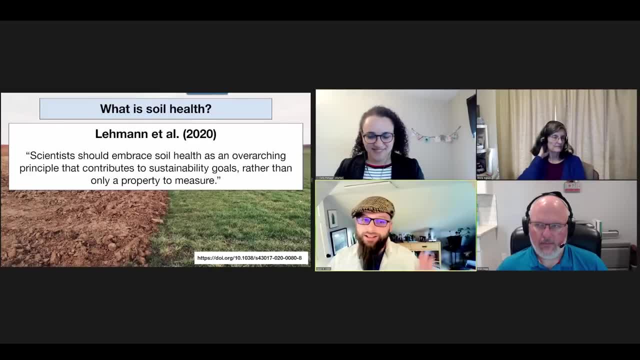 Okay, So let's go ahead to the next slide. There we go All right From the top. folks, What is soil health? Because that's one of the topics that I think people were brought in today to talk about rebuilding soil health. 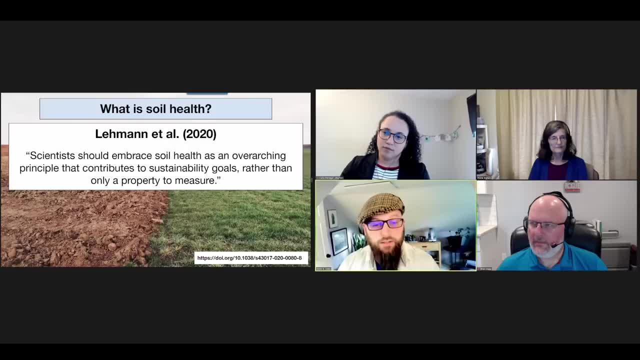 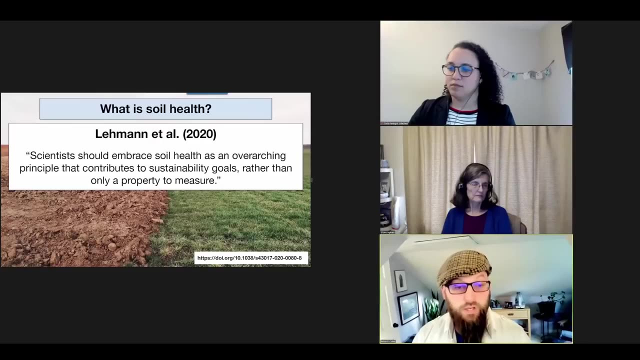 So when I was asked to present some of this information, I wanted to go to current scientific literature and see how are some of the experts talking about soil health together, And so this is one paper that was published in 2020.. You know that says: 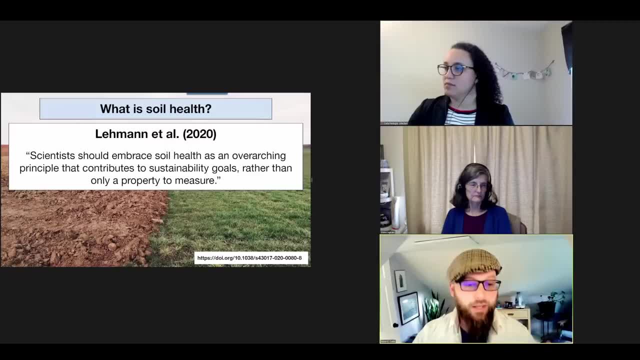 Scientists really should embrace soil health as this overarching principle that contributes to sustainability goals rather than a property to measure, And I think that's really important. and it would be easier if soil health could just be defined as a few numbers. Right, Then we would all be happy. 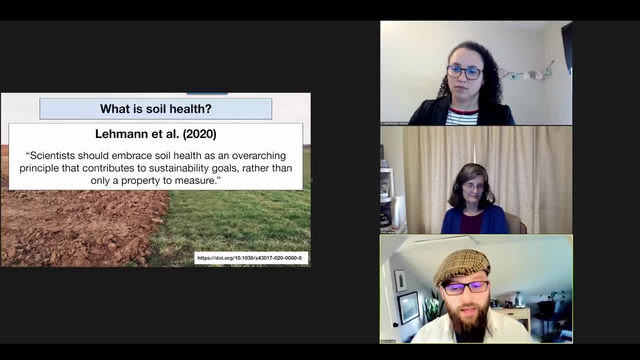 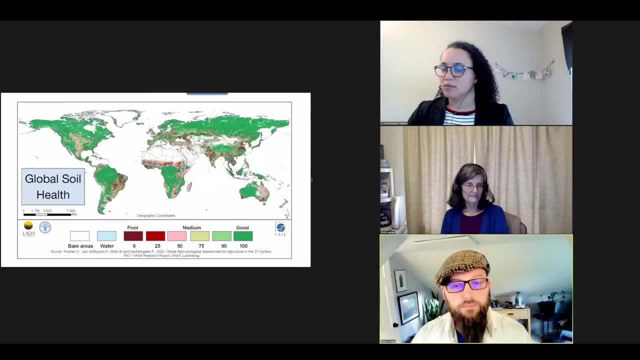 We would target those numbers, But it's really broader than that And I've included the link there if you'd like to go read that full paper. But could you go to the next slide for me please? Regardless of what we think about soil health- and it is something that you know is measured- 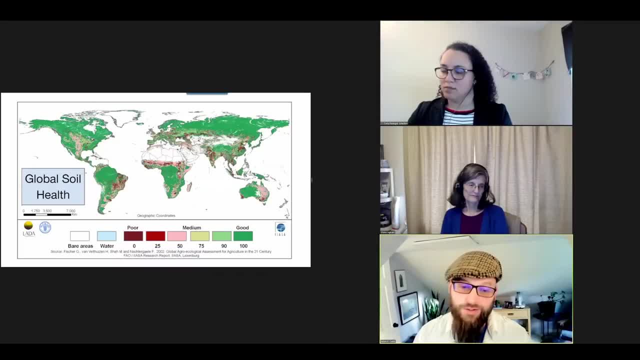 This is a paper. Actually, it's interesting because this is a 20-year-old paper now- But the Food and Agriculture Organization of the UN and some other researchers got together and they really tried to quantify where in the world we're seeing like a loss in soil. 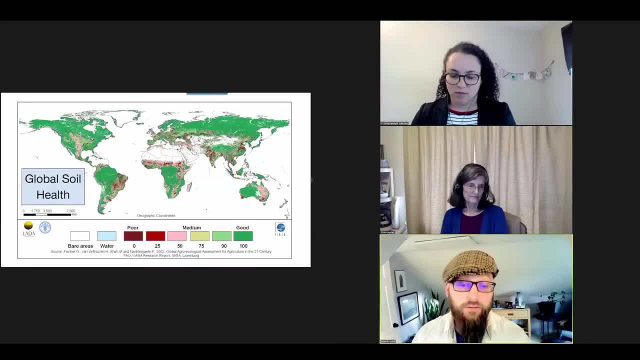 health, which is a lot of places. You'll notice sub-Saharan Africa, You'll notice parts of Brazil, The Central United States, South Asia, China, Australia And, honestly, you know, we could think of all of this as agricultural land. 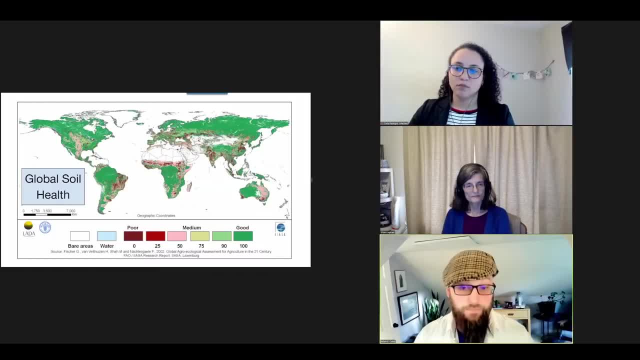 But deforestation is a huge part of this as well. I think a lot of us have heard about the deforestation that's happening in places like Borneo, for example, How that's threatening orangutan populations And how that's sometimes an expansion of something like palm oil production that's causing that. 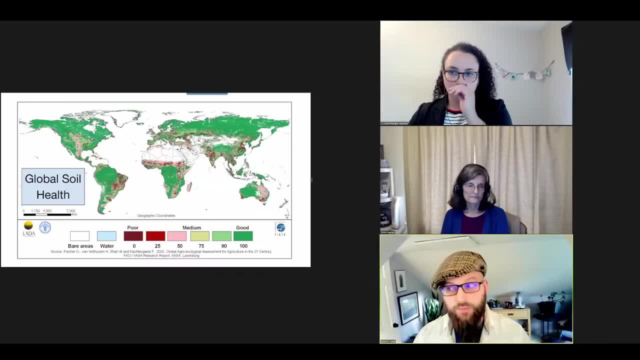 But typically when we go in and disturb those especially old-growth forest systems, there's a rapid loss of soil health. And so you know, like I said, this is 20 years old. I guarantee this map has gotten redder in the last 20 years. 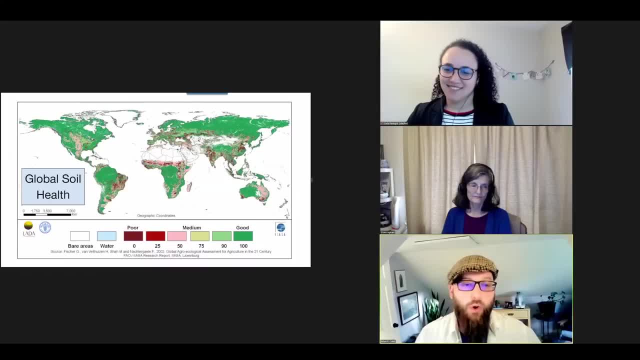 I mean, that's the sad truth of it is, while we're discussing all these different definitions, we know that globally there's a lot of degradation And in fact we put out a short sort of synopsis just the other day about a recent UN report. 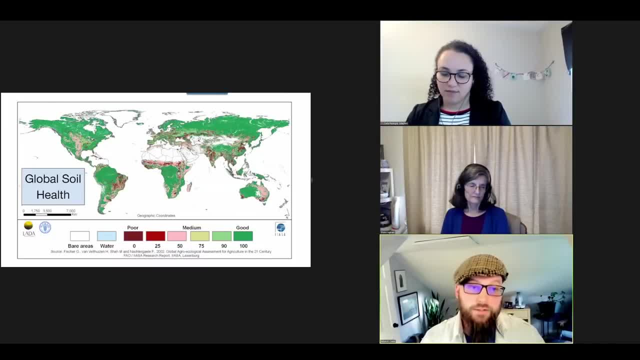 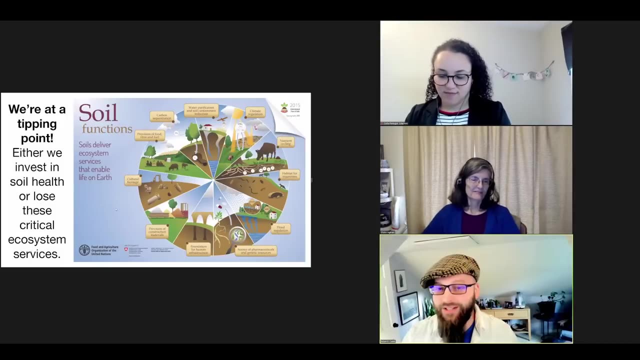 that indicates, you know how many tons of soil are eroding away every year on this planet, And so it's something that we all need to be aware of. Could we go on to the next slide, please? So, if you all can see the soil function slide, which is another FAO figure, I realize there's a lot going on. 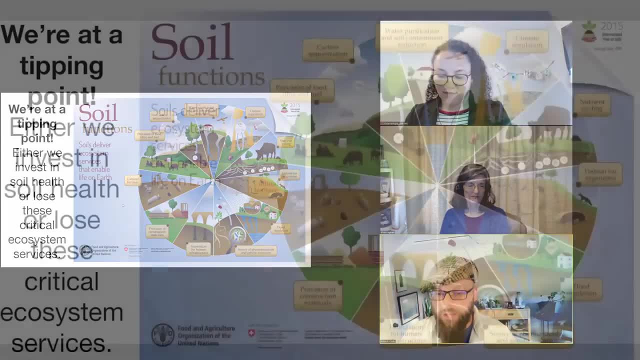 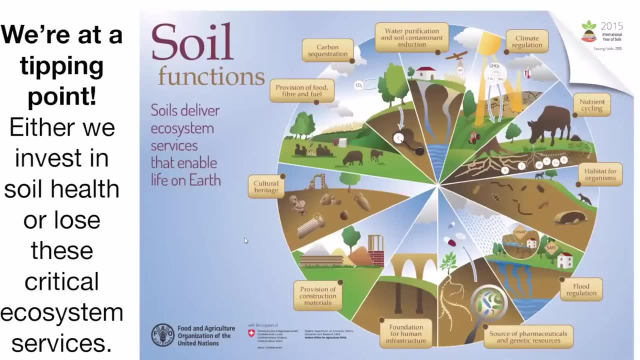 But here's what I want to focus on. Over time, instead of just looking at soil measurements, we're starting to really ask the question about like: what are the ecosystem services that are coming out of our landscape? And there's a lot of categories, not just food production or cotton production. 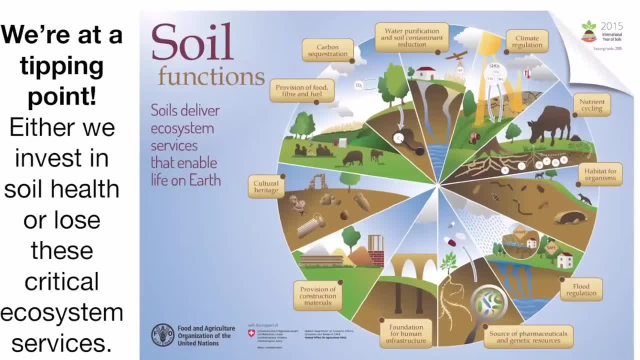 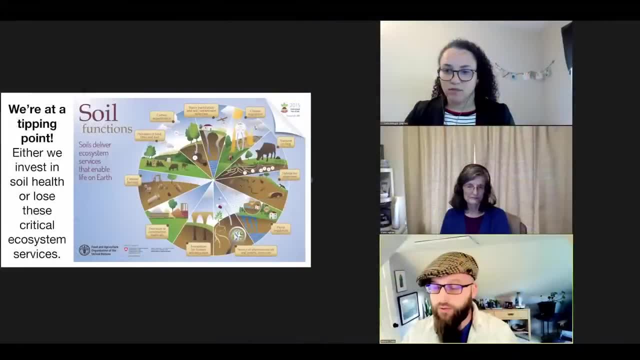 but things like water purification, climate regulation because of the way we can store carbon in soils, And so we're really starting to get focused on what are those ecosystem services and what are the soil functions that support those ecosystem services. But I got to say again, and I'm not just trying to be gloom and doom here- 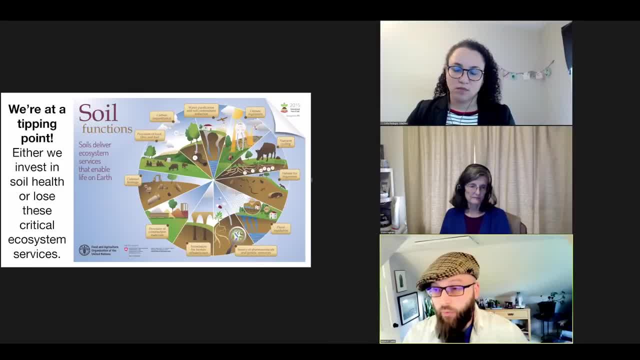 but we are really at a tipping point where now we need to invest in a lot of soil regeneration and bringing back these lost functions or we're going to continue to see a loss of these ecosystem services. It's happening all over the planet And, you know, I sometimes see a little bit of skepticism, maybe on our ads on Facebook. 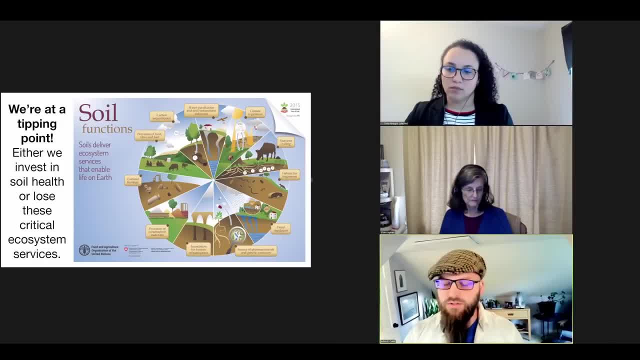 where we talk about some of these problems and people say: I don't think humans are really, you know, capable of affecting the climate. Well, I really would love to take some people to places around the world that I've been in- rural Africa. 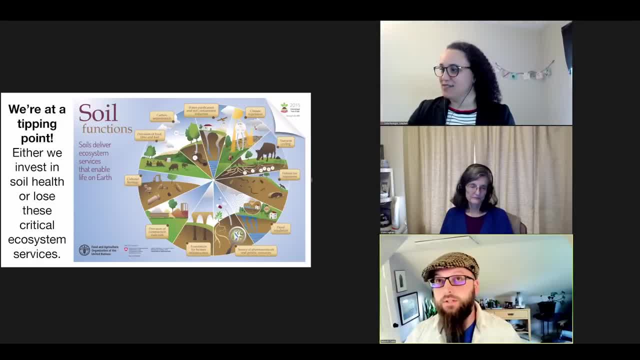 for example, where the poverty has caused an unsustainable use of the landscape. Not that I'm blaming anybody who's living in poverty, but you can really see that overgrazing by animals and other things, which is really. I mean, there's whole books written about how some of our ancient civilizations in this world 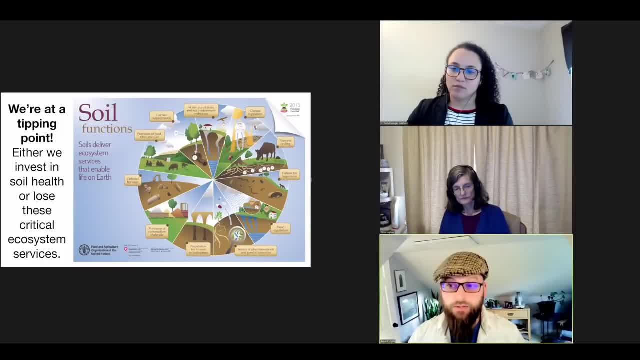 the Mesopotamian civilizations collapsed because of unsustainable soil degradation, right Overgrazing salinity issues, these things. there's a historical record and we're watching the ecosystem services of the world right now and seeing them diminish. 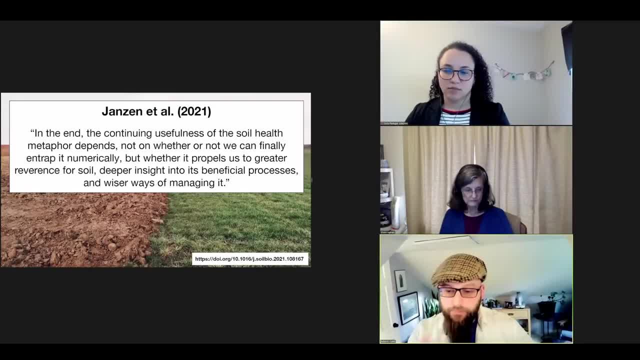 So it's just a starting point that we have to be aware of. So I love this quote and I've actually I've been emailing a little bit with Dr Jansen, the lead author of this. I saw a presentation by him. 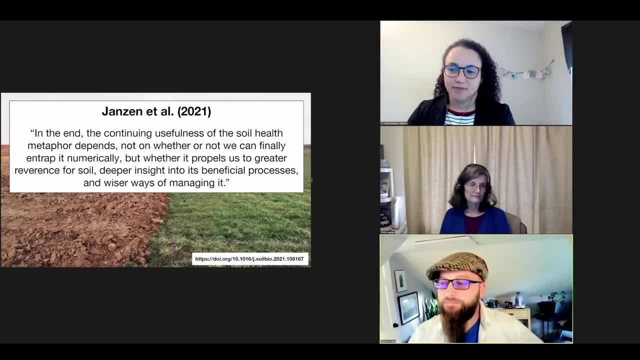 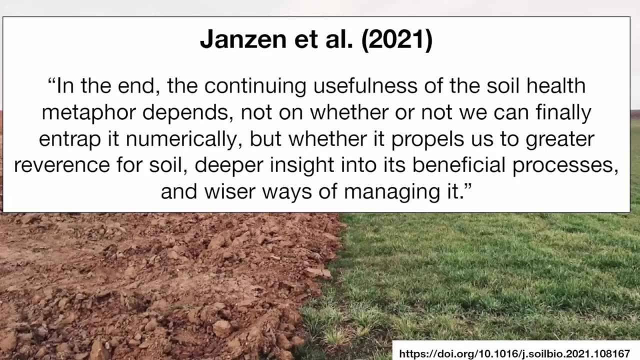 and it is just pure poetry to me because it says: in the end, the continuing usefulness of the soil health metaphor depends not on whether or not we finally entrap it numerically, but whether it propels us to greater reverence for the soil. 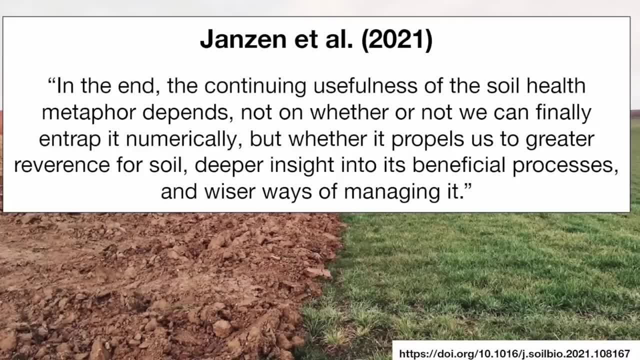 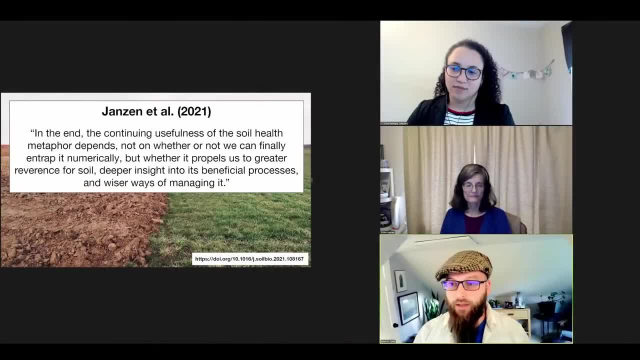 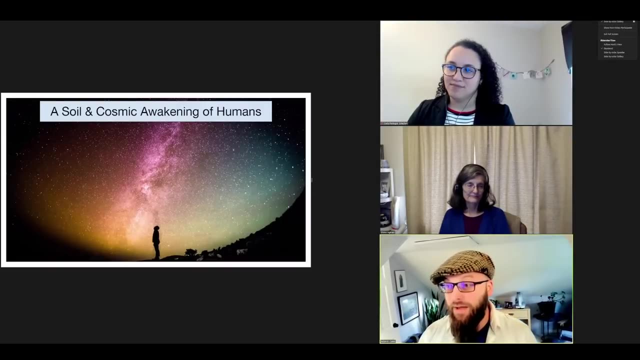 deeper insight into its beneficial processes and wiser ways of managing it. This is why I like talking about soil health, because living things have health. That metaphor is valuable. It gets us thinking this is a living system And so really, this is part of something I would like to invite all of our participants to think about. 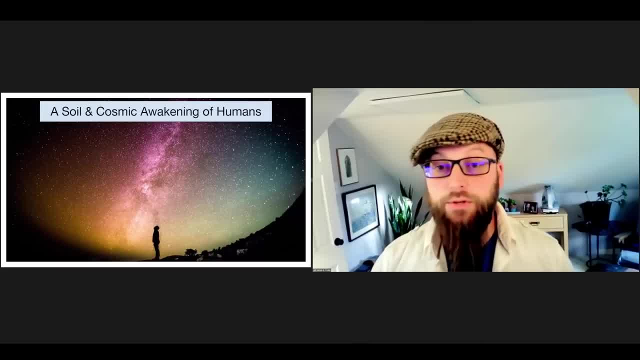 because all of us can be part of this, with our neighbors, with our friends, with our families. I think we need to have a soil and cosmic awakening of our society. What I mean by that is the word cosmos really means a harmonious system. 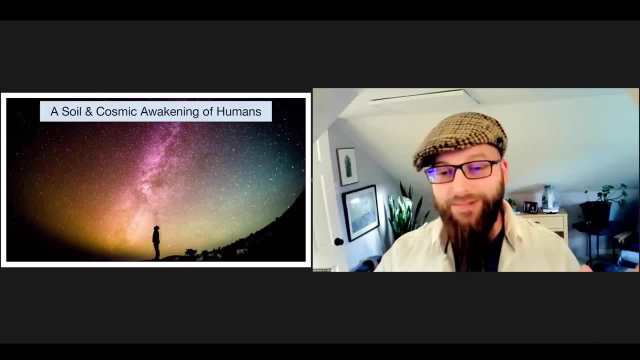 So when we look out at the stars in the sky or, like, look at space images from the new Webb telescope, I see this beautiful, beautiful reality. And there's this. they used to call it the music of the spheres, right. 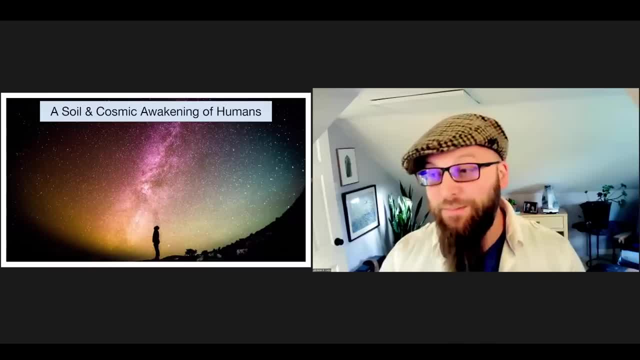 This thing that's happening out there in space. The same thing is happening in soil. If we look, we have to look with different tools, We have to understand it in different ways, But soil is like another cosmos And it's been one of the funnest parts of my job here at Soil Food Webb School. 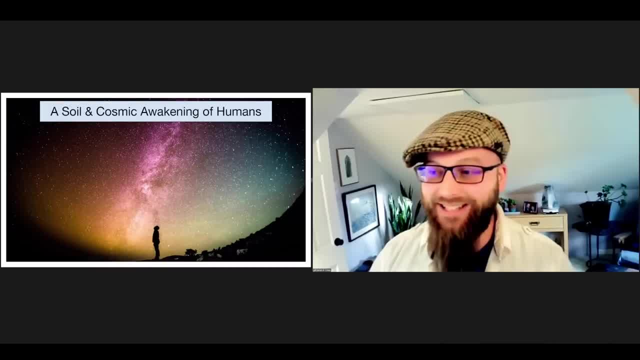 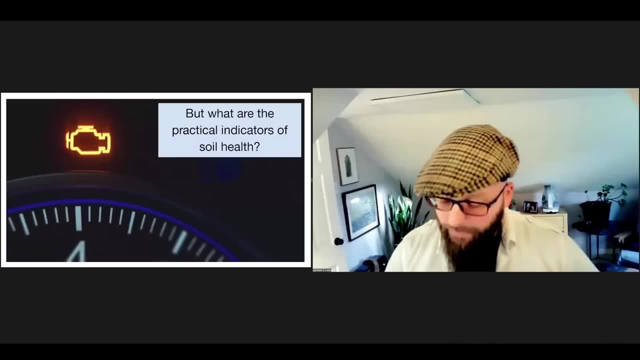 that I get to actually peer into that in a new way And I get to see through the microscope the living parts of the soil. But probably, if you came here today, you're also looking for some practical information And there are some things that we can say. the check engine light of your soil has come on. 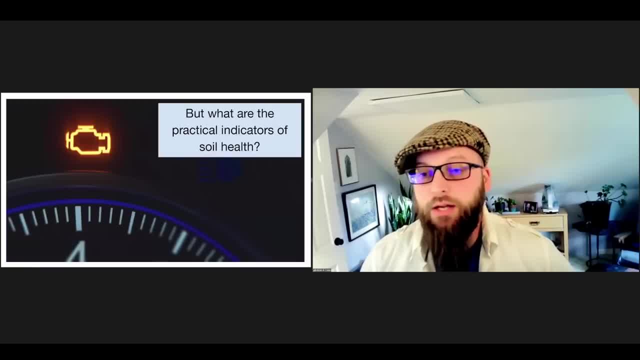 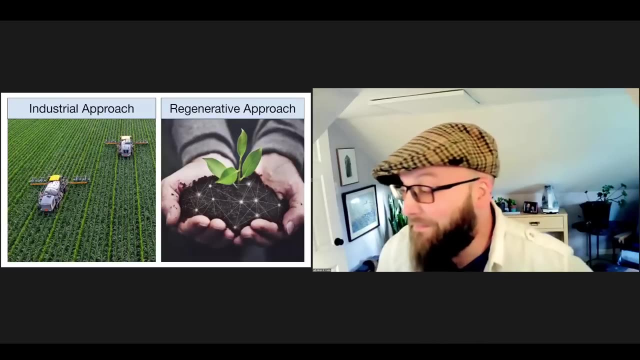 There are some practical indicators that we can use to get at this idea of you. know what direction are we moving? Is the system collapsing, Or is it moving towards a more resilient soil, Or is it moving towards a more healthy state? And part of the reason why there's so many definitions is the industrial approach to agriculture is so different from the regenerative approach. 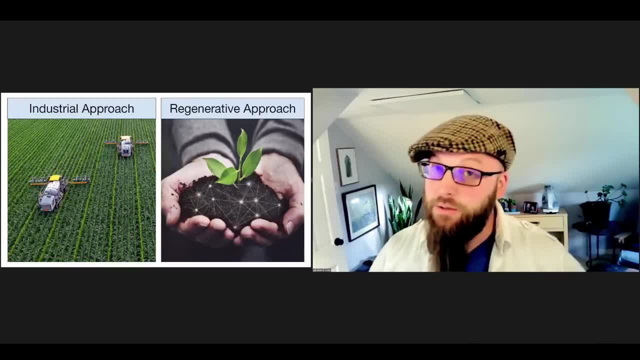 And I wrote about this a little bit in that recent blog as well, because I used to be more in the industrial mindset in terms of I taught classes on global food security. I had a hard time imagining that we could sustainably feed a growing human population. 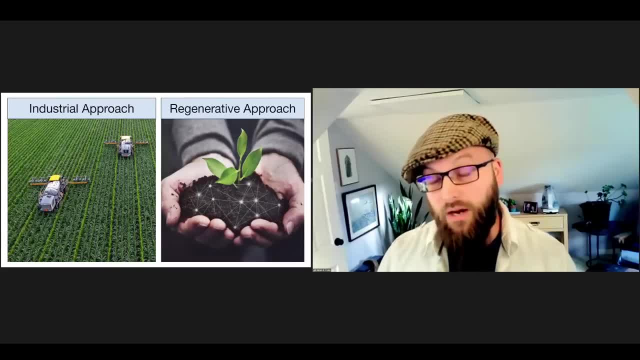 Without green revolution type technologies. And then I really started to understand more about how this entire web of life comes together And the ways that it can be so much more efficient right In industrial approaches. for example, you might pour on 200 pounds per acre synthetic nitrogen fertilizer. 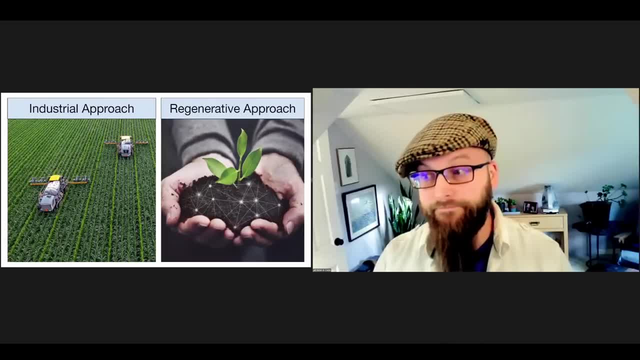 That's about 225 kg per hectare Every year And we know that like 50 or 60% of that is not used by those plants that year. And what happens to it? It goes into rivers and streams, It turns into nitrous oxide and goes into the atmosphere and contributes to climate change. 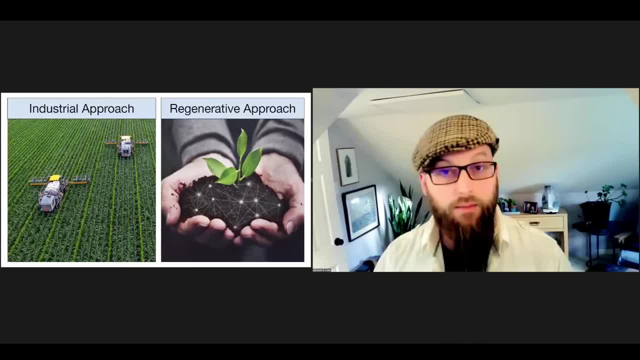 So there's a system where we kind of say: I'm not blaming. I have many friends that practice industrial agriculture. I'm not blaming them. They feel trapped. They feel trapped by that, They feel trapped by that chemical system And they think that they can't make profit any other way. 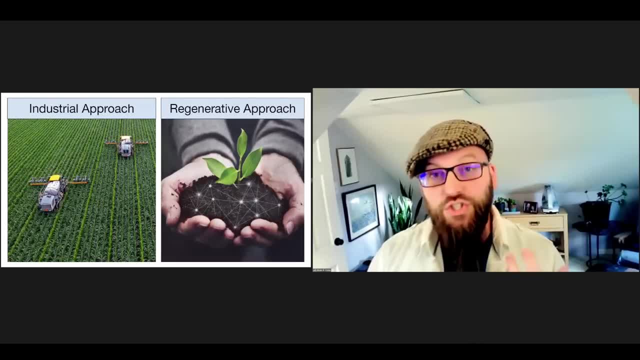 But there is this emerging thing, This regenerative approach, These different ways of managing systems, These different ways of managing nutrients. That understands each part of the soil food web has a role and function And supporting the soil food web supports the plant health. 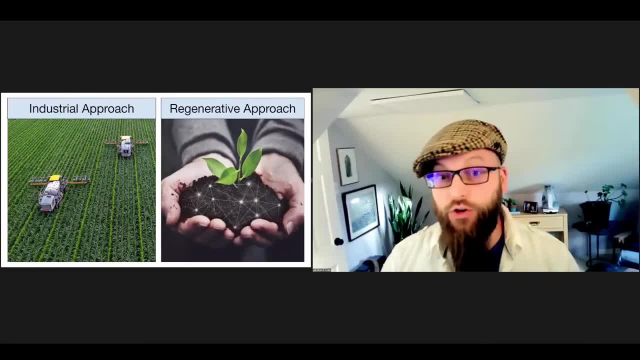 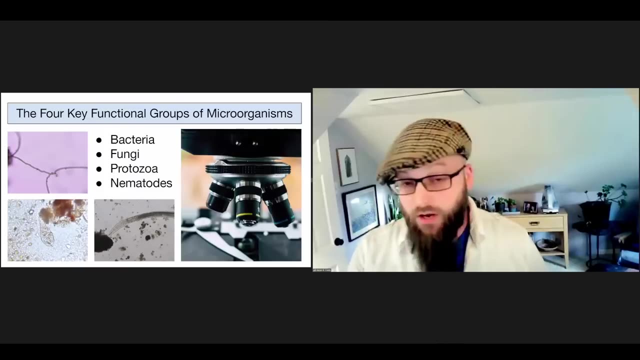 And the productivity And the nutrition of the food that comes out of that system And all these other ecosystem services that the UN talks about. So what are those key groups? Well, we talk about bacteria, fungi, protozoa and nematodes. 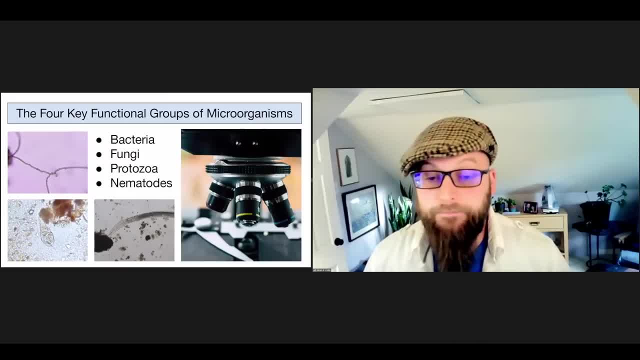 Primarily. That's what we focus on. Dr Lane and other researchers in the world have found That if we can understand not just how much of each of these organism groups are there, Like their abundance, But also their diversity, How they're interacting with each other, 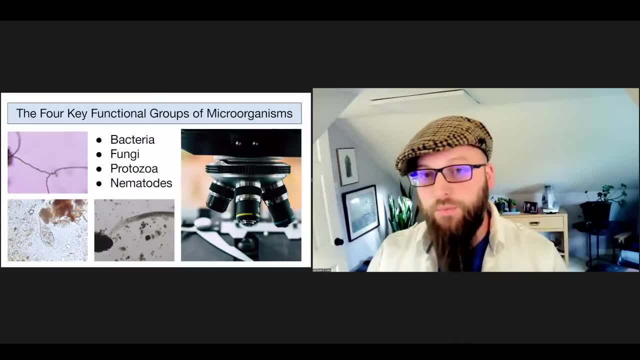 How the organisms that are sort of like the lions and tigers and bears- Right The predators of the system- Are interacting with the organisms that are like the deer or the other grazers in the system. It's like It's like a jungle. 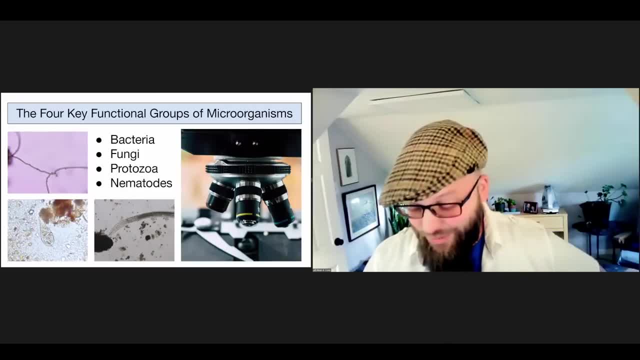 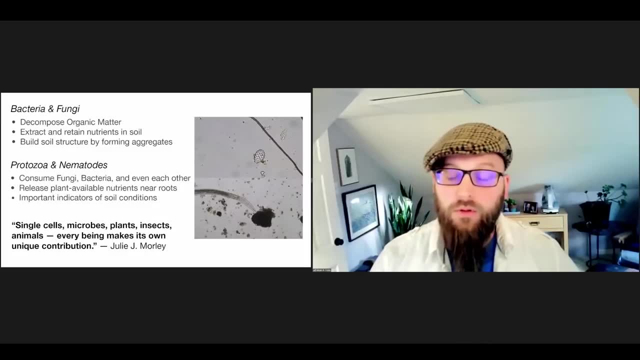 But just really tiny. So What do some of these groups do? Well, bacteria and fungi. A huge part of their role Is to pull nutrients out of organic matter, Or parent The parent material Right, The pebbles. 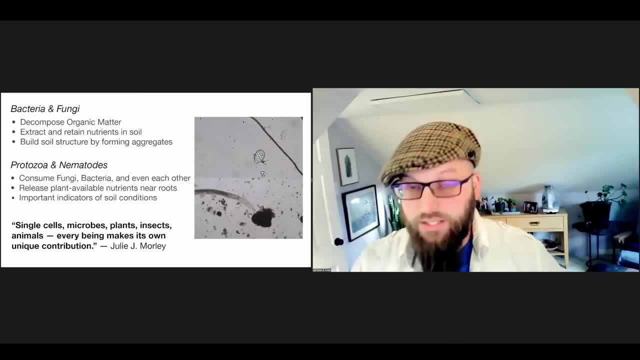 The sand, The silt, The clay. They have the right digestive enzymes To chew on those inorganic substances, As well as the organic matter that's in the system, And to keep extracting those nutrients. And they retain them by putting them in their bodies. 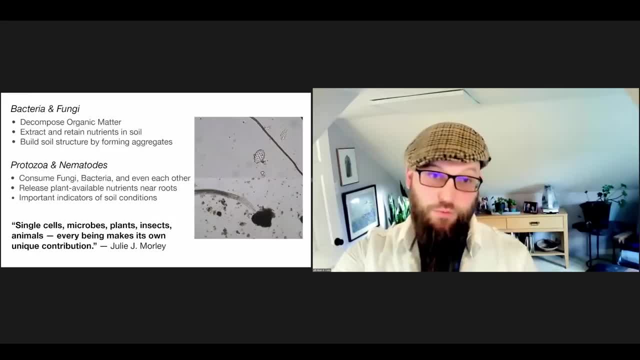 So, instead of dumping on lots of chemical fertilizers That disappear, The nutrients that they pull out of the soil environment Are stored in their bodies. They're not lost to the atmosphere or to the water. They're stored in their bodies And so. 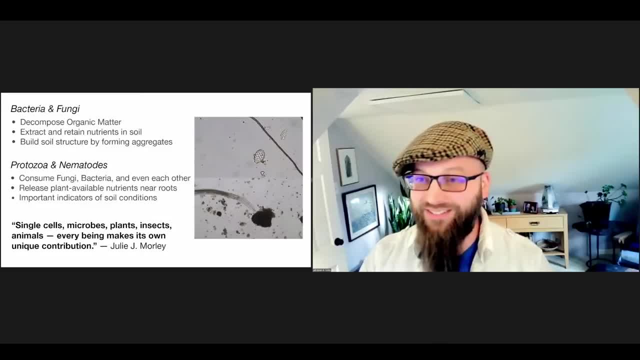 They have this amazing capacity To entangle everything And to create Complexity In terms of how the soil aggregates, That's, the crumbs of the soil That allow passageways for water and air to cycle. And so They have this really. 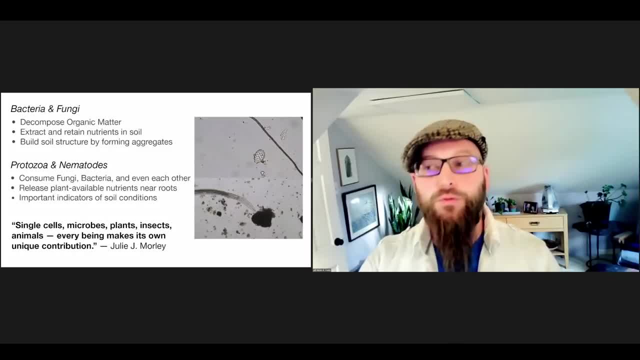 This key role in In making things Move around the system Right, And so I don't know if you're familiar with this. Fungi and bacteria are really three-dimensional organisms And they can be of all kinds In terms of what we eat and what we eat. 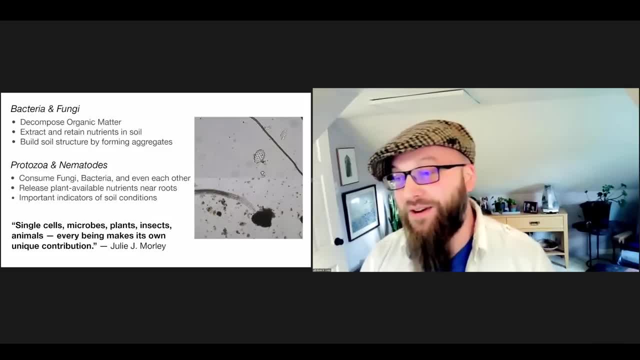 So we see a lot of, Let's say, a lot of Artificial plants. What we eat, We see a lot of �mels, Or plants, Or plants And so And we see How they can have that Transformation. 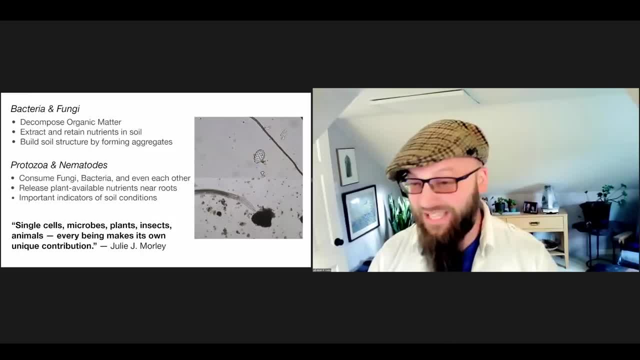 And so We see, And then the protozoa, like a meadie that will hunt other nematodes. it really is a jungle in the soil. But when they consume primarily fungi and bacteria, these predator organisms get more nutrients than they. 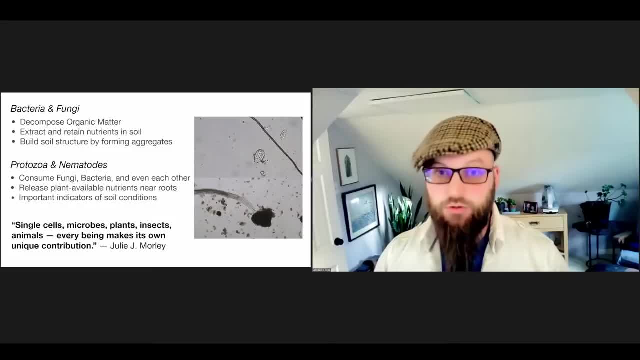 need right. The bacteria have more, say, nitrogen than the actual needs of the protozoa or the nematode for nitrogen, and so they excrete the excess, And that releases the nutrients in a plant-available form really close to the roots of plants. So instead of dumping on a bunch of 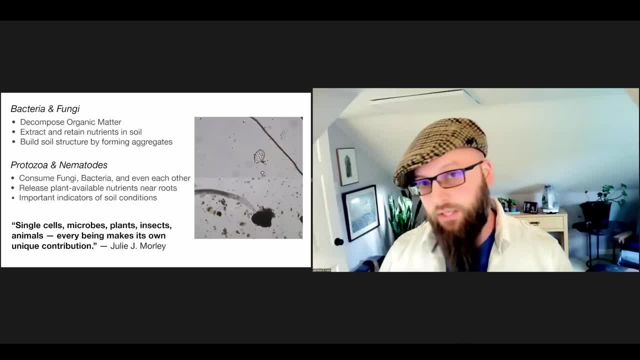 fertilizer early in a season and having it inefficiently be utilized by plants, the soil food web cycles these nutrients, retains these nutrients and releases them in this trickle that perfectly feeds the plant. That's right, as it needs it constantly And, honestly, it's like a symphony in the soil when 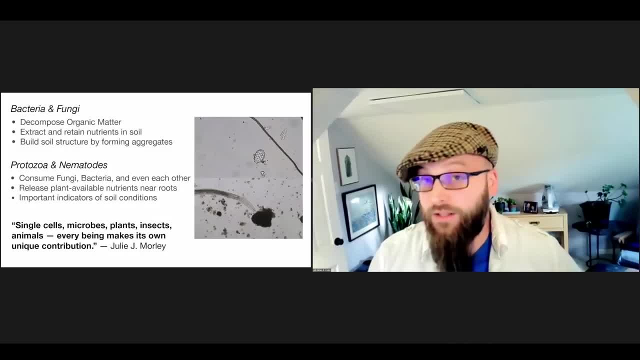 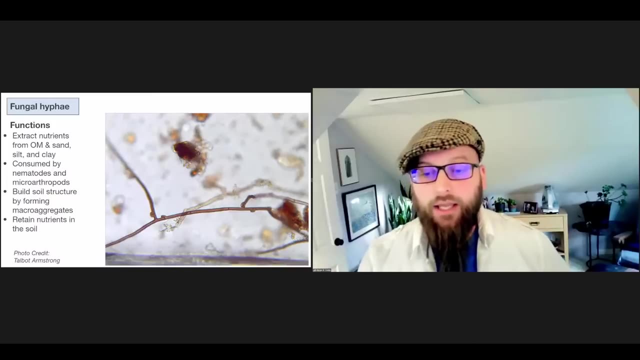 you look at what these organisms do. The neat thing is for us that a lot of what we see under the microscope or through the microscope can also help indicate what the soil conditions are. So when we see a lot of fungi and diverse kinds of fungi in the soil, often that 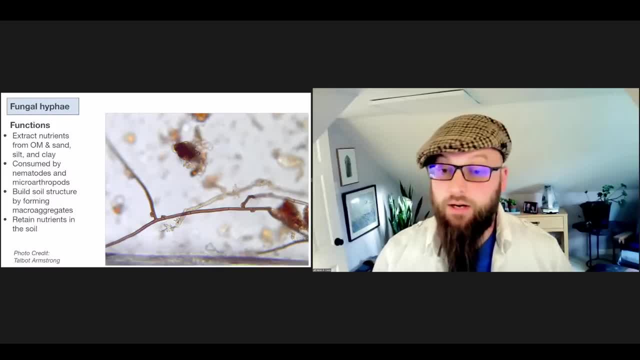 indicates that the soil is in a so warped condition. So when we see a lot of fungi in the soil, that indicates that the soil is in a so warped condition. So when we see a lot of fungi and indicates to us that it's pretty high oxygen environment, The fungi are not necessarily. thriving in a low oxygen environment, And high oxygen environments, or at least moderate oxygen environments in the soil, tend to be the right environment to encourage beneficial microbial activity or microorganism activity and constrain the growth of the things that could harm our plants or keep them from switching on genes to become pathogens. So it's amazing. It's amazing. 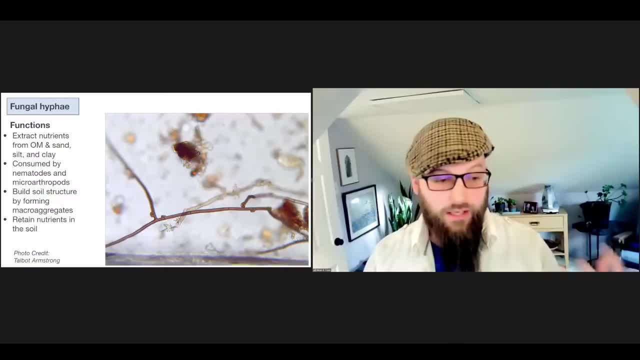 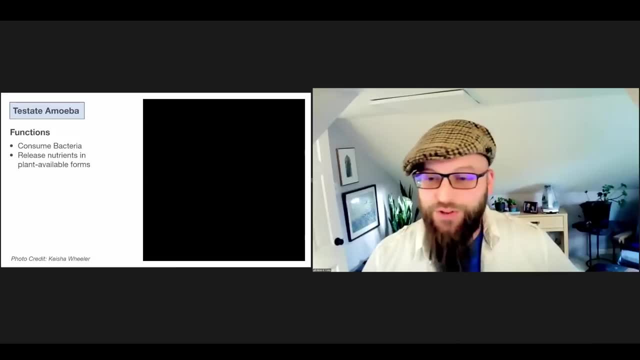 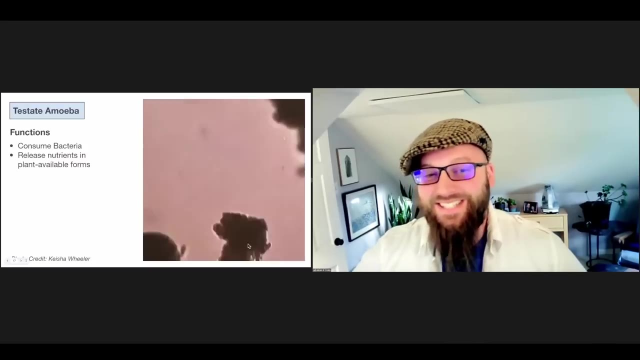 how the whole thing works together. The fungal hyphae: like I said, they entangle and help create that structure. And then we have a little video here, because things like this testate amoeba, which is just cool when you think about how alien these are. 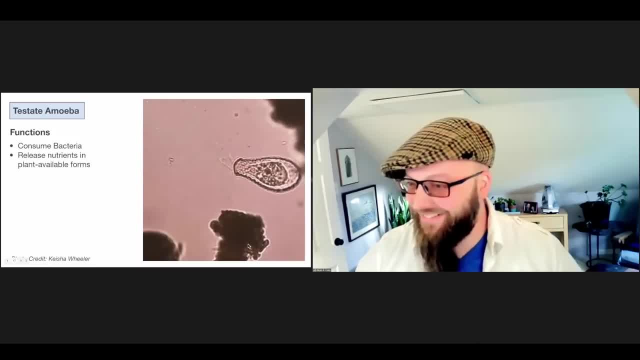 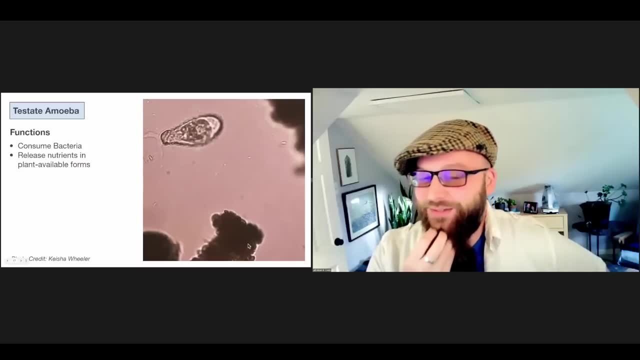 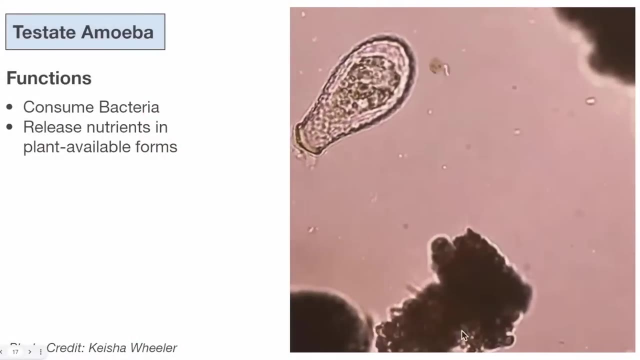 right. They're sticking out pseudopodia, pseudopods- it's tentacles- and crawling across the surface of the microscope slide And it's looking for bacteria to eat so that when it consumes a bunch of them- hundreds thousands of them in a day, even again- it's excreting all. 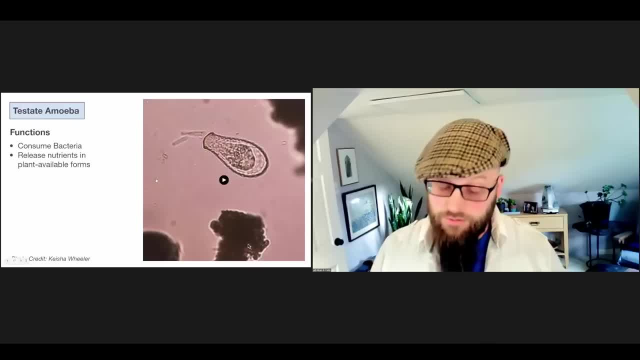 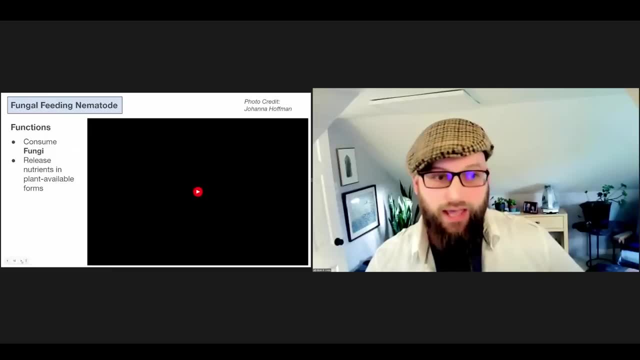 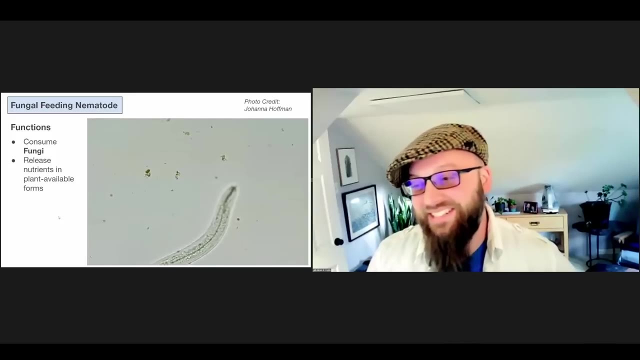 those excess nutrients, And it lives near the roots of plants, so those nutrients become available. Let's see if I can get to the next slide here. Okay, This is another fun one. I mean, these little nematodes are like my new favorite thing to watch. They are just so cool, In fact. 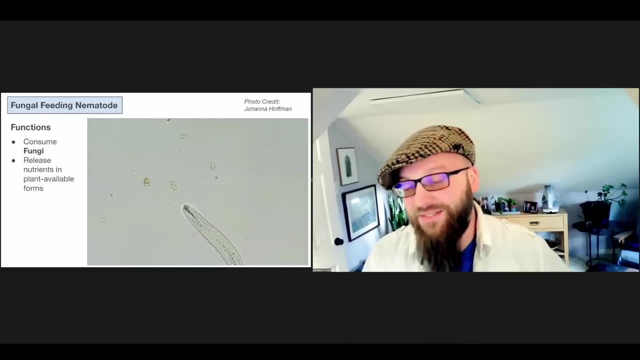 I don't want to creep anybody out, but there's thousands of these millions even inside and on our bodies, right, They're just interesting. This is a fungal feeding A nematode. a big way that we can get a clue for that is that it has a stylet or kind of a spear. 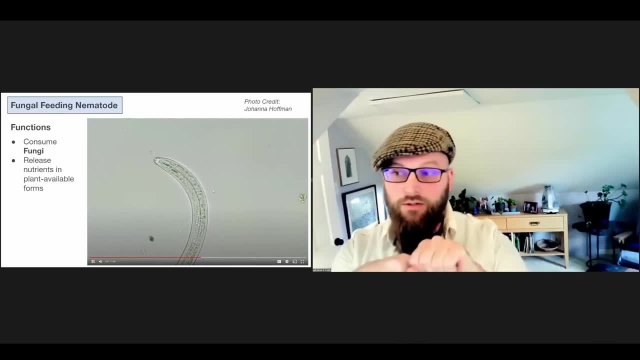 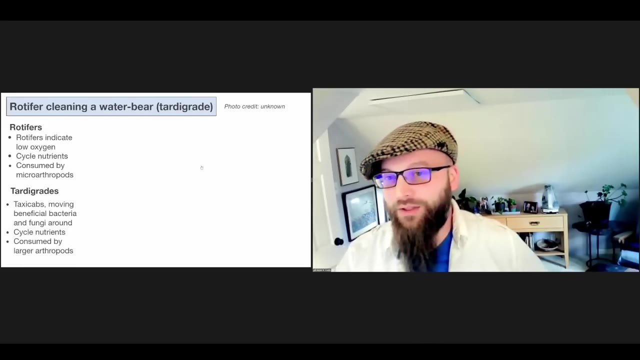 in its mouth so it can puncture those cell walls of fungi and suck things out through that straw. suck out the good stuff, the food that it's looking for. Okay, Continuing with our show of interesting biology. This you can actually see here. 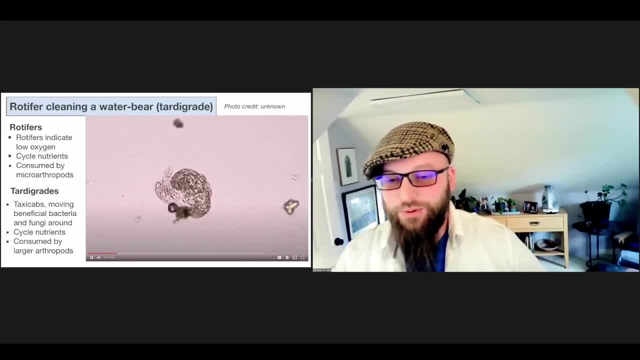 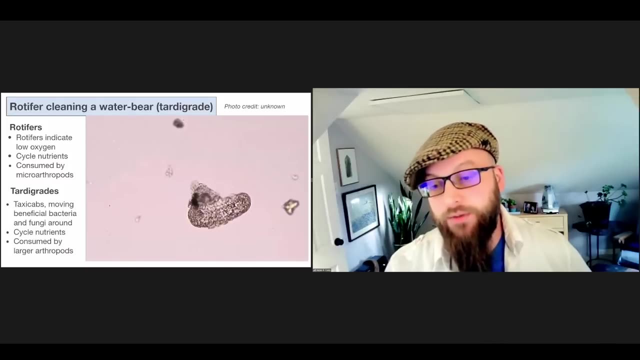 a rotifer and it's attached or near. it seems like it's even cleaning the surface of a tardigrade, also called a water bear. Now what's interesting about these is the rotifers can actually be an indicator to us if there's a lot of them in one of our samples. 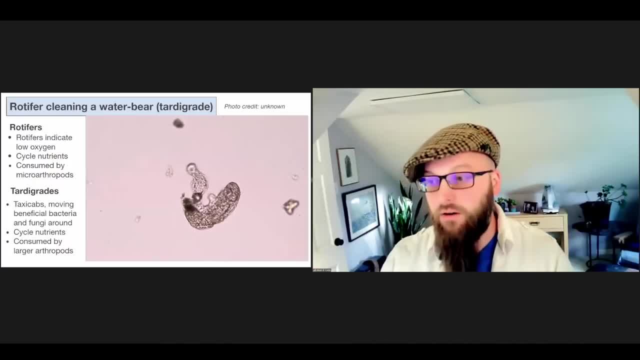 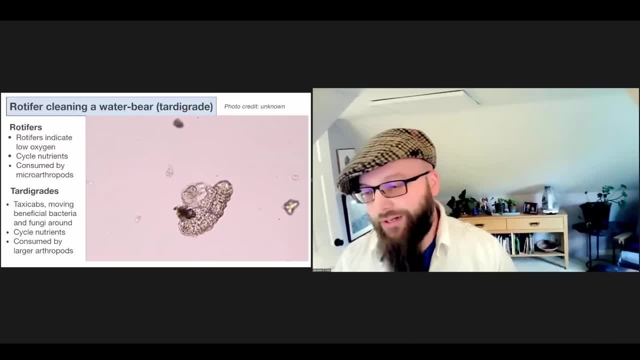 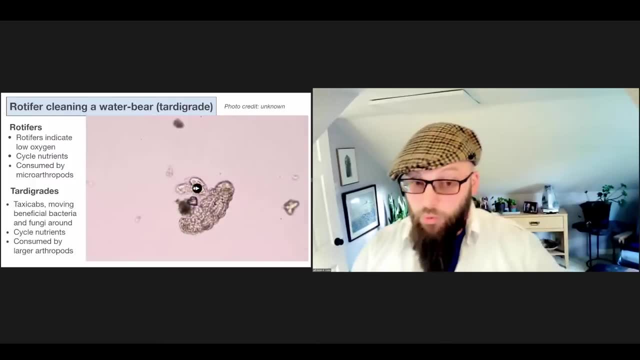 you know, if I saw a rotifer in my soil, I wouldn't worry. If I saw hundreds of them, I might start going: okay, there's something, there's something a little bit off here, But they have a role to play and they're food for microarthropods. 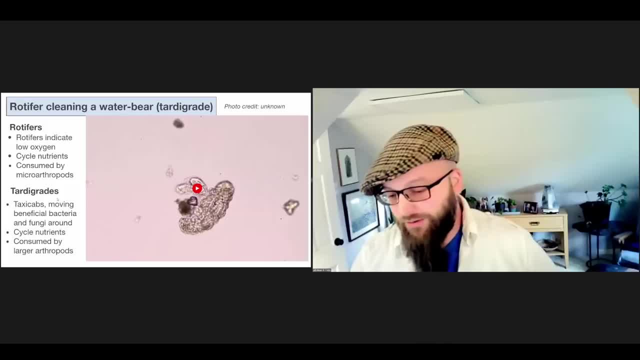 And tardigrades are fun, not just because they are among the most adorable things that we find in the microscopic world, but because we consider them taxicabs. They can move around. Other organisms can kind of latch on to them and move around- beneficial bacteria and fungi. 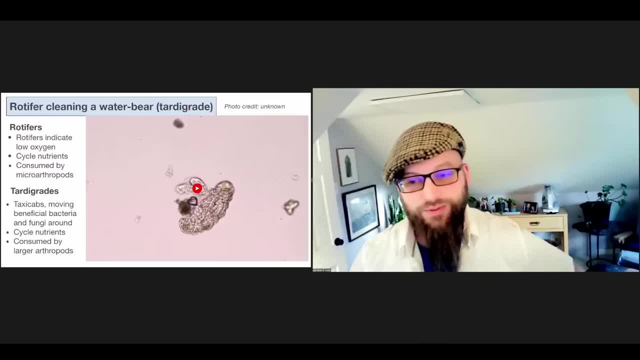 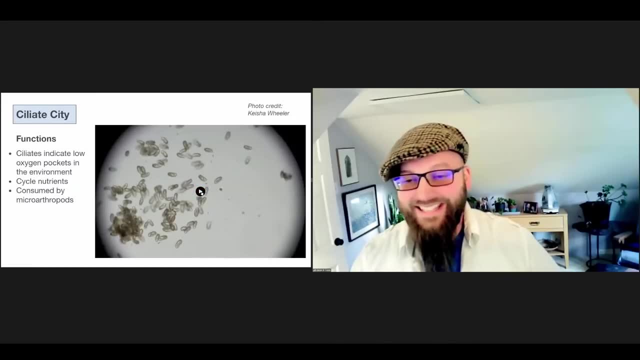 so that they can colonize new parts of the soil. So yeah, rotifers, Tardigrades Love them, And then ciliates are another indicator to us that we may have some low oxygen conditions. And so actually, if I start collecting these, if I cover them in glass, then I'm in trouble. I'm just going to be a moron, And so if I start collecting these, I'm in trouble. And so if I start gathering these, I'm in trouble. And so if I start collecting these, I'm in trouble. And so if I start collecting- 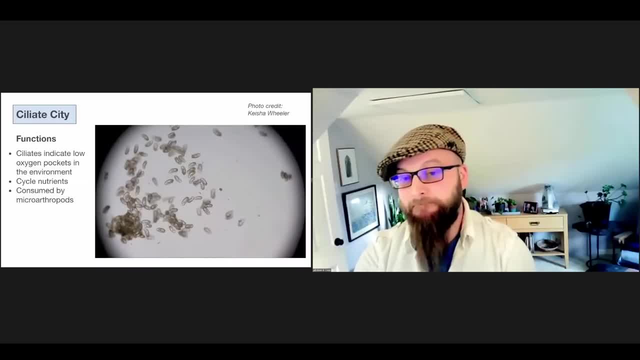 saw this ciliate city going on in a compost sample. I'd be pretty concerned that that compost wouldn't necessarily be good to apply to my system, that there's a lot of opportunities for some pretty nasty, low-oxygen-loving pathogens to be in there as well. right, See a few ciliates. 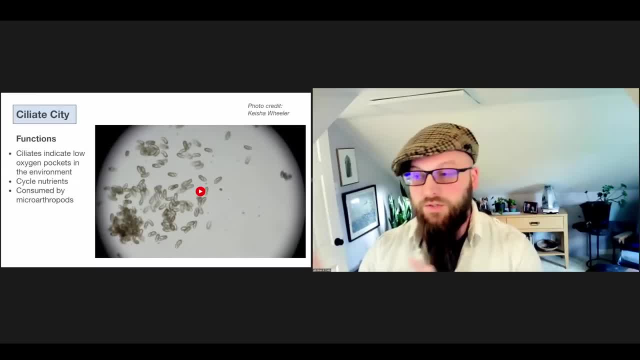 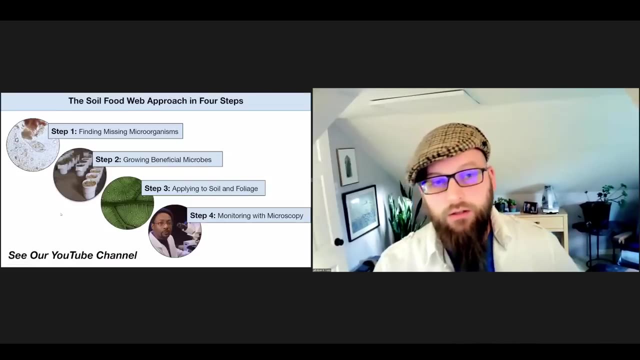 they might just be living in a little aggregate or pocket, which is fine. See dozens, hundreds of them. you got potential issues going on. So the life in the soil. you know, and I would just like to mention here that on our YouTube channel, especially in our January videos, we have a lot. 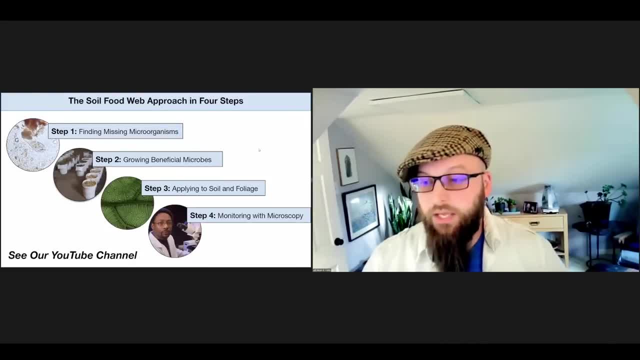 about the steps that Dr Elaine has developed and taught here The school, about how we can assess the microorganisms that are in our soil, figure out what's missing. that's a huge part of the equation. Maybe diversity is missing, Maybe there's not enough of a population there. Maybe a key functional group is completely gone. 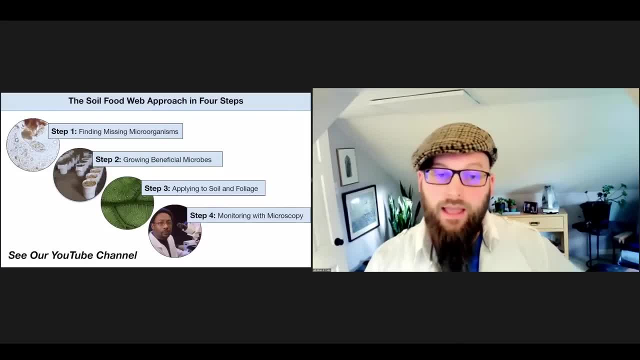 because of something historically that disturbed them. And then how do we grow out beneficial microbes and apply them to the soil and foliage effectively So that we can get them back into that ecosystem? And it's like a pretty standard idea in restoration ecology that you need to put back the things that are missing. 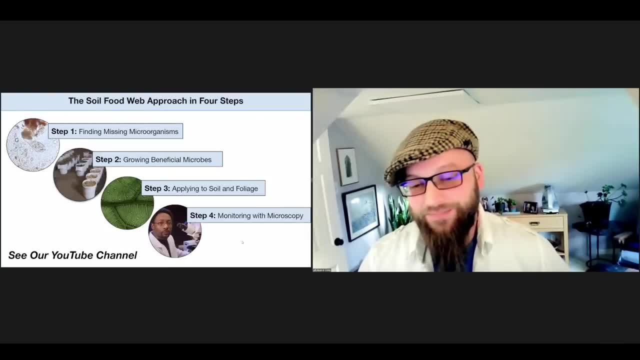 to really get the system sorted. And then we monitor with microscopy the changes in the soil food web over time And we consider, like any practices that we're using in our garden, on the farm or ranch. we want to understand how do those impact, how do those influence the soil. 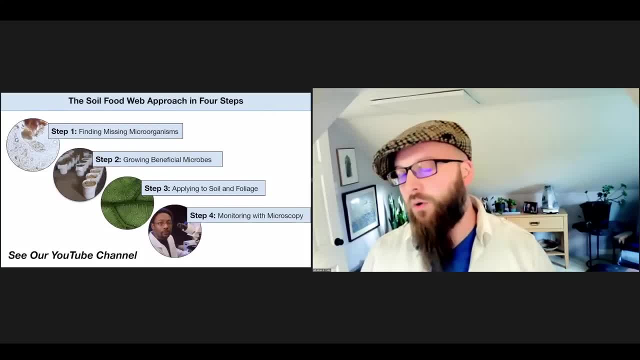 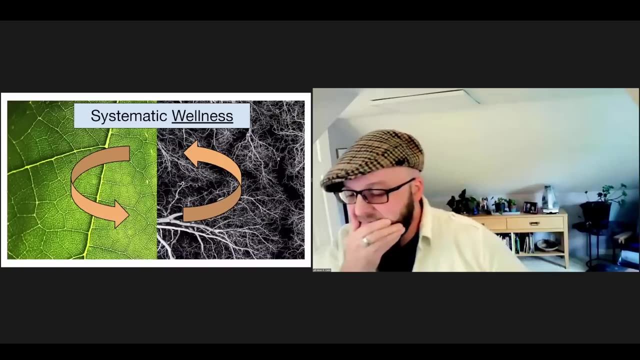 food web so that we can start to remove or alter practices that are harmful and put more practices in that are more management tools in that are going to help it thrive, that are going to create that healthy microbial system. So I hope that you're getting the idea. 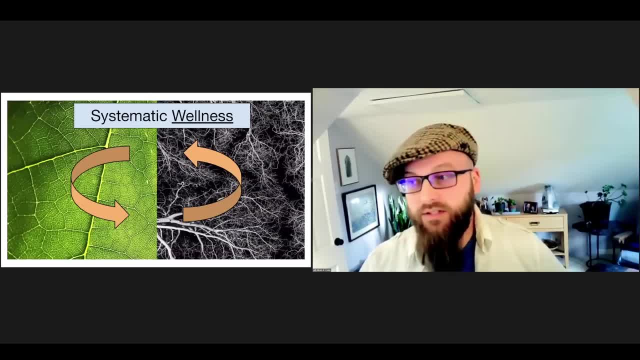 I heard a whole group say that, And I'm надing, I'm in awe. if you're hearing it, Hurry up and collect those questions. let's do it. You should reflect on that as well, Like I do. So I'm here to talk once again. 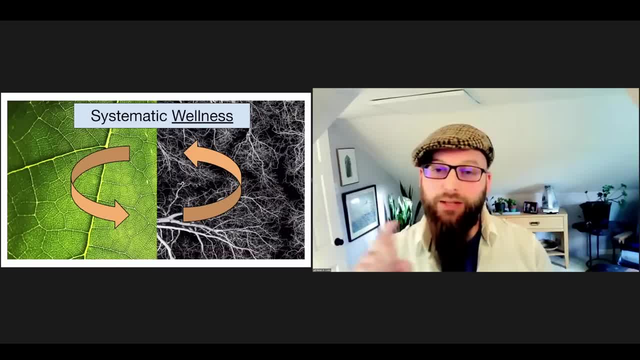 Because I think that this process is so important that that this is holistic, systematic thing that really even soil health is not nutrients up and it increases their ability to photosynthesize, which means more sugars are coming into the plant, which means the plant is sharing more sugars through its exudates. 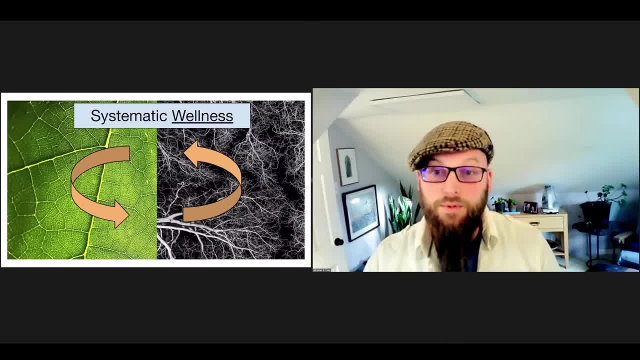 with the, with its microbiome, with its associated microorganisms, And so there's this beautiful- I mean it makes me think of like yin and yang- There's this beautiful coming together of forces, symbiosis, And- and we believe that, one of the most important points of leverage. 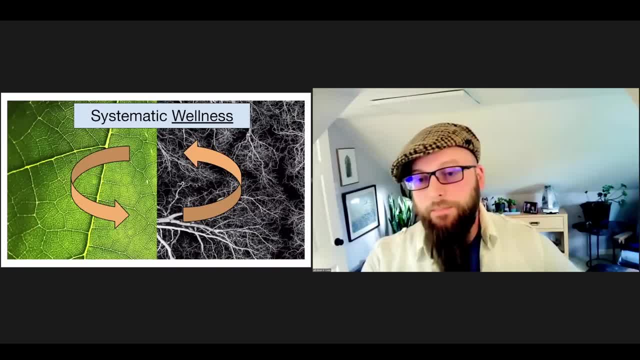 is to get in there and make sure that your soil food web is complete, right? If there's something missing, then the plant is not going to be healthy, And then the plant is not going to be feeding what is there as much as it could, And so we steer the ship. 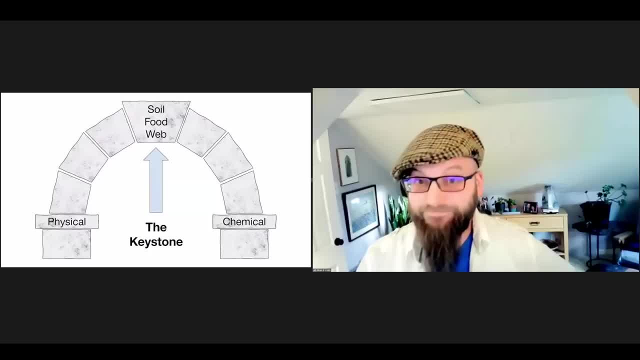 Through the um, through the soil food web- And that's really because you know, this is the metaphor I like to use- is there's there's chemical ways of of um. I don't just mean modern agrochemicals. There's there's mineral balancing and things that we can think about. 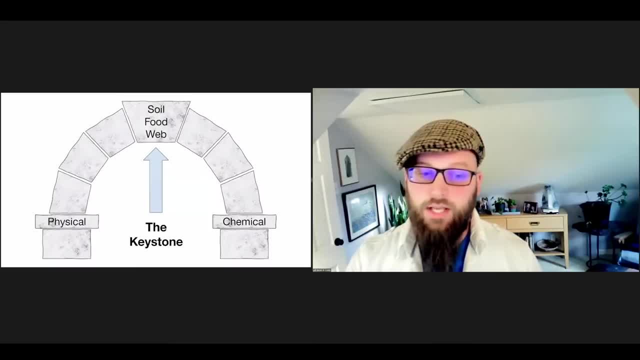 doing in soil. And there's physical interventions, Like if we have compacted soil, we may have to deal with that in a physical way at least one time, And there's all these other management tools that we can utilize. But if we are not constantly going, 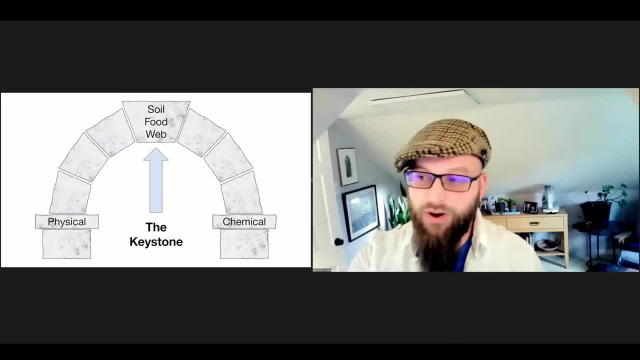 back and thinking: what about the soil food web? What about the soil food web? How does this influence the soil food web? How can the soil food web um be part of fixing this chemical issue or this physical issue? Then we're missing the keystone, the thing that holds the arch. 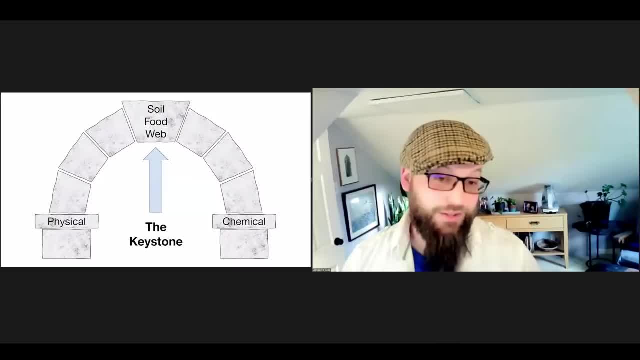 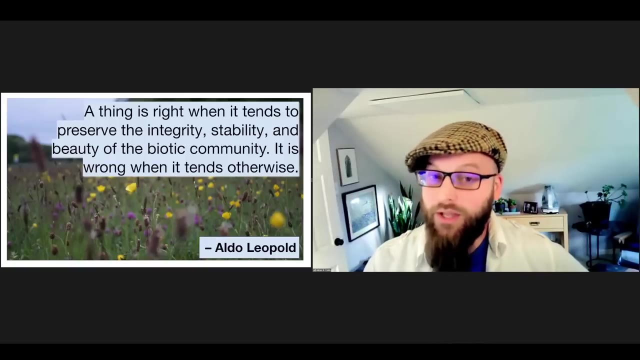 together And so, um, you know, that's sort of going back to my thesis with the soil food, the leadership statement, and then having to wrap up all of that thinking about the soil food web. um, the foundation of healthy soil is the foundation of our lives and the soul food. 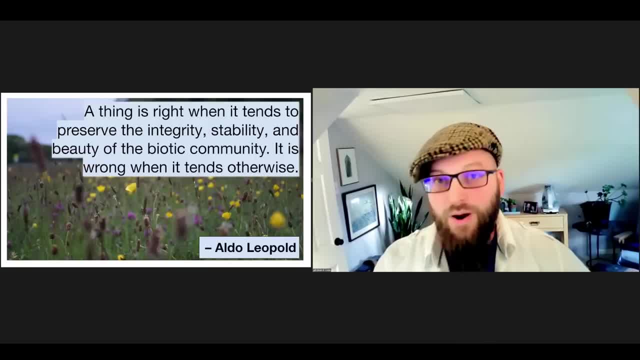 web is the foundation of healthy soil. Um, so I want to end this section, uh, with a, with a little quote here by Aldo Leopold: I, I will, I, uh, we've promised to tell you some more of the. 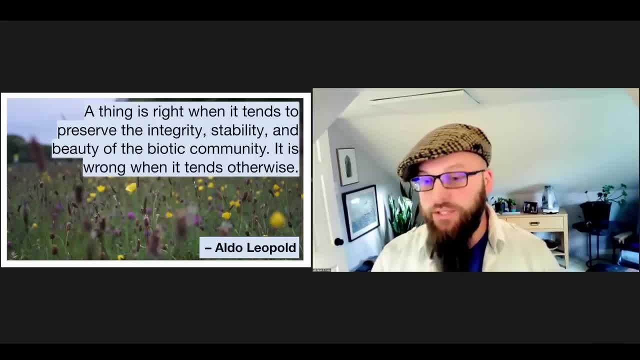 direct benefits of a thriving soul food web. but, um, I absolutely love this. This is a uh, a farmer and a researcher in the thirties, recognizing tends to preserve the integrity, stability and beauty of the biotic community. It is wrong when 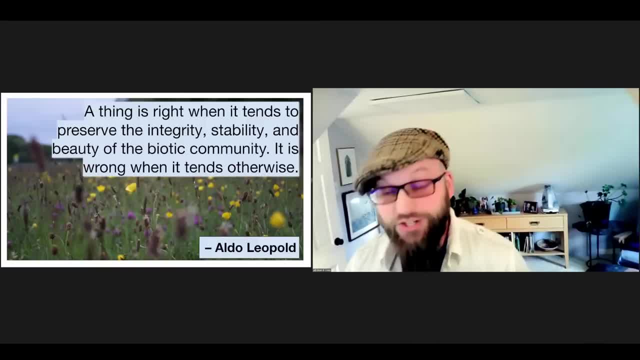 it tends otherwise. So the industrial agricultural practices that cause a loss of fungal biomass and diversity: they're not the right pathway for us. The use of herbicides that maybe disrupt the protozoa in the soil: they're not the right pathway for us. They interrupt the integrity. 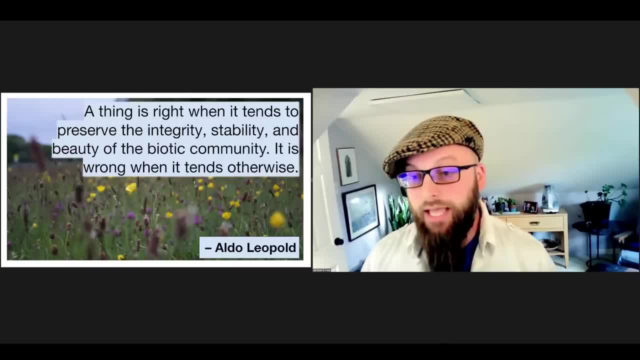 and stability of that biological community and we need to find alternatives. right? If somebody says, well, regenerative ag needs to prove itself, I also say, well, industrial agriculture needs to stop causing all this disruption. right, And there's probably transitions and compromises. 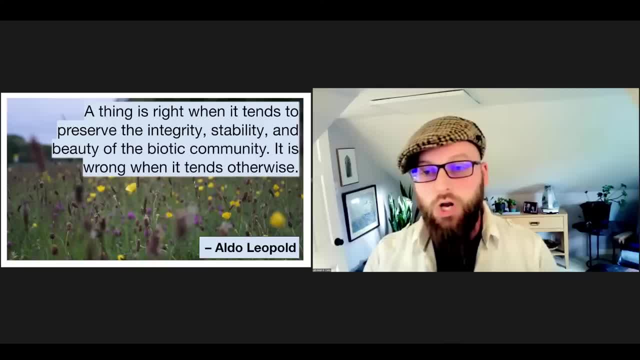 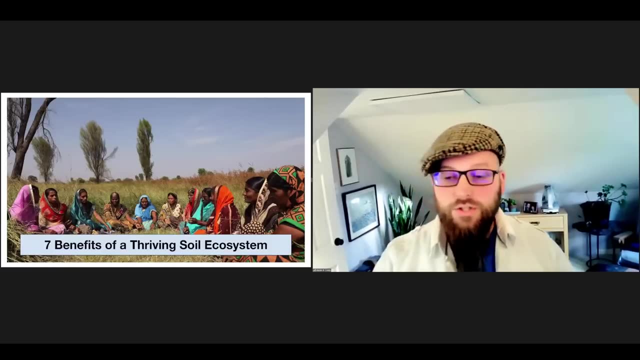 and a mosaic of different management that we need to work on, but we need to move towards biological farming. It's the future. It's the only future that works in my opinion. Let me take a breath here. We're going to transition. just a few more slides. 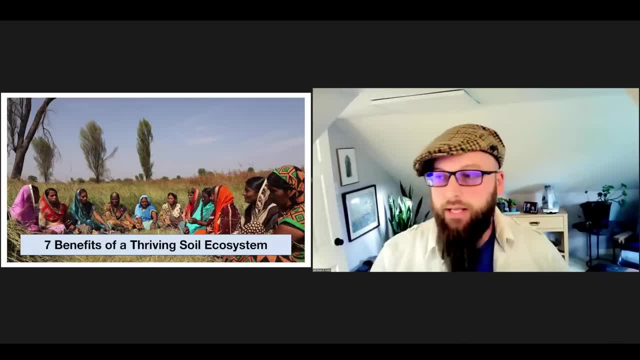 like seven, eight more slides and then we'll get to Q&A. Maybe people are sick of hearing my voice, so I promise we're almost done. But I did want to say you know, it's natural for us to say: but what are the benefits? right? 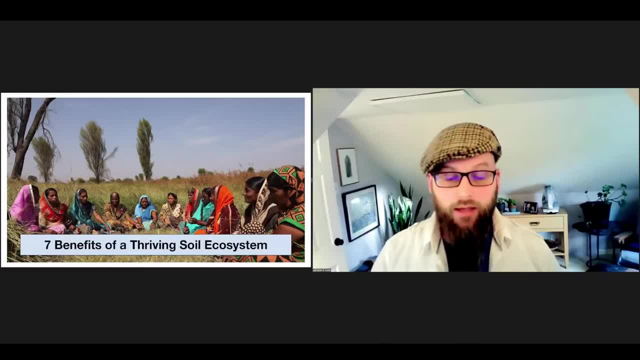 People need to make profit. if they're involved in agriculture, for agribusiness or in your garden, you want to say, well, okay, this is going to take time and energy and money to make these investments. What do I get out of it? So here's seven benefits of a thriving soil ecosystem. 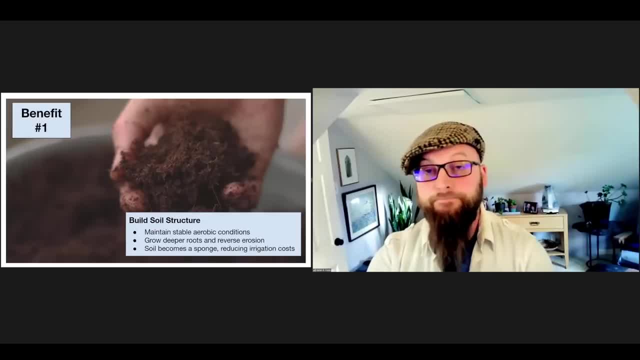 I already mentioned a little bit about the benefits of a thriving soil ecosystem. I already mentioned a little bit about structure. I have actually assessed fungi in several different places around the world and I found that most of our agricultural practices, like tillage, 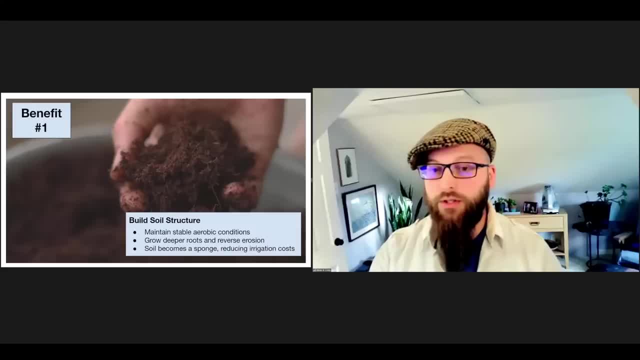 leaving fields fallow and planting monocultures, they've really reduced the biomass and the diversity of the fungi in those systems, And so we've lost some of this ability to have the fungi help us grow, And so I think it's important to think about that, And I think it's important to 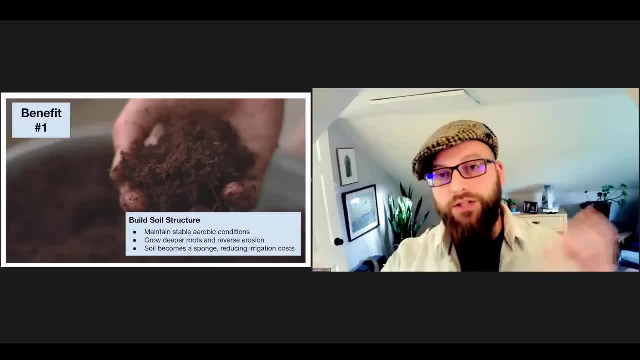 think about that, And I think it's important to think about that, And I think it's important to think about build soil structure, a sponge that will take in water, a structure that will allow air to flow around and keep pockets of the soil from becoming so anaerobic that they only breed pathogens in. 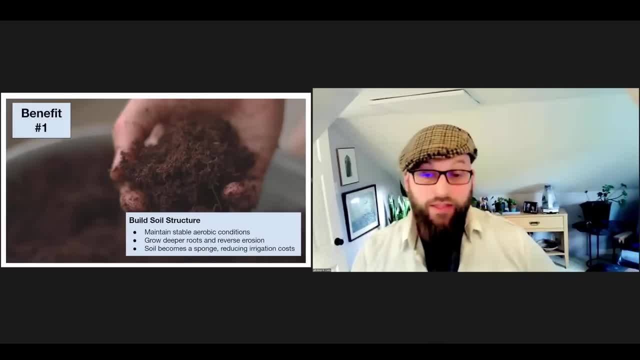 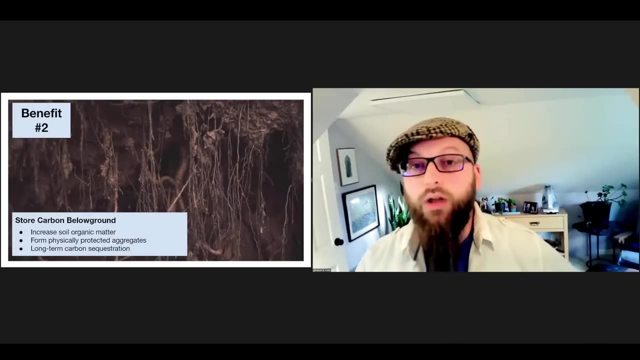 there. So it's one of the key benefits. Get your soil food web right and you'll see an improvement in soil structure. Along with that- I mean very closely paired to that- is we'll store more carbon below ground. We'll get that organic matter up. It needs to really be above three percent before that system. 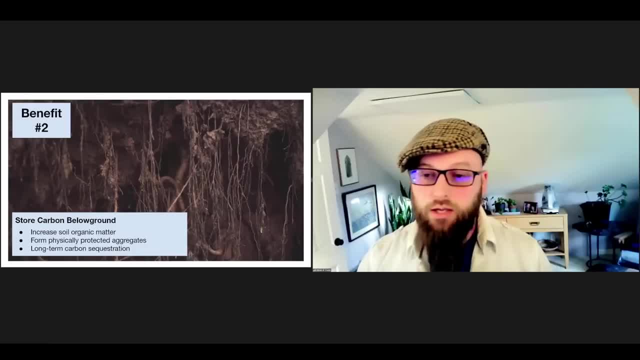 can take off And we're not just talking about- I say store carbon. sometimes people use the word sequestration. There are forms of carbon that we can. they can be locked up for like hundreds, if not thousands, of years, And fungi are. 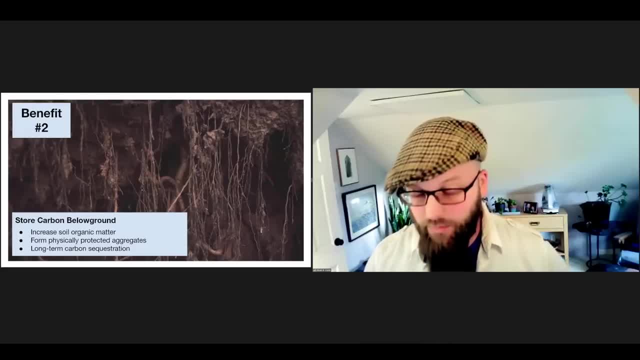 they're a huge part of that. There's this structure with which they store carbon, So get that system thriving and it can be part of addressing climate change in the world. A big chunk Agriculture contributes to the emissions of greenhouse gases. Agriculture can be a huge part of the solution. 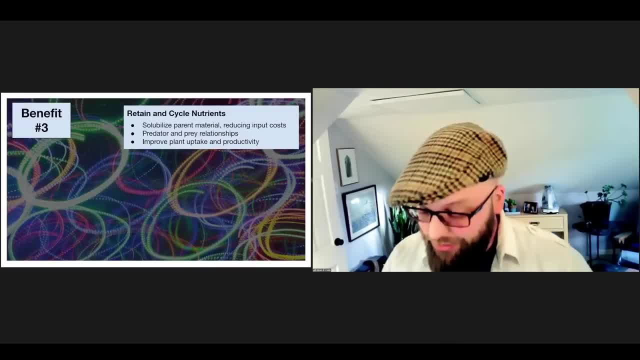 And then there's that retaining and cycling nutrients. I already talked about that in a great deal because of those predator and prey relationships, And I think it's important to think about how we can. we can still save the environment And I think it's important to think about how we can. 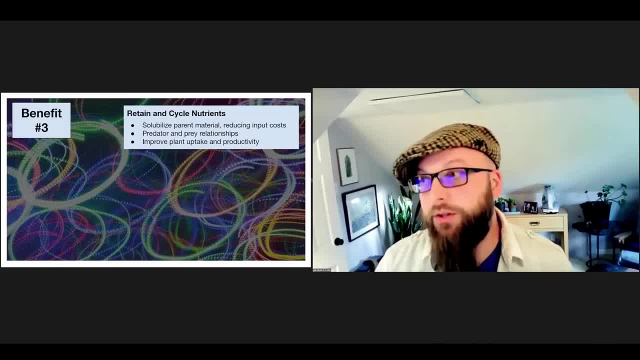 save the environment, And I think it's important to think about how we can save the environment. We need to. there's there, even the industrial agriculture. folks realize that the future is about producing more with less, with fewer inputs, with less irrigation. You know that those water 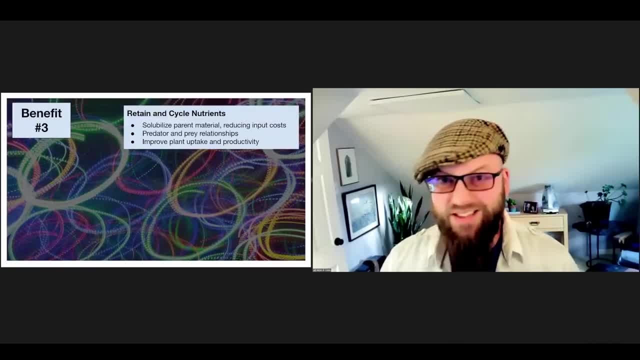 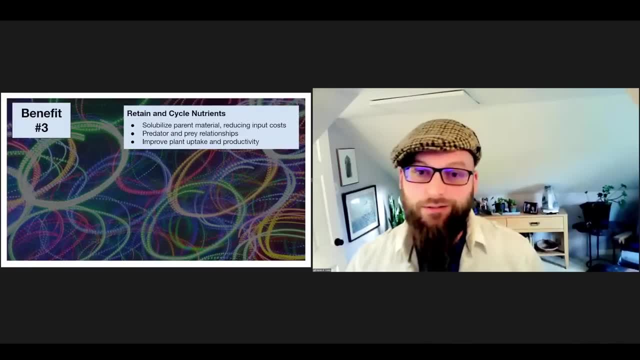 dynamics are huge because agriculture uses currently like 70 or 80 percent of our fresh water supplies in the world, And so you know, efficiency is the name of the game here: Optimizing. For so long, we just focused on maximizing the yields. 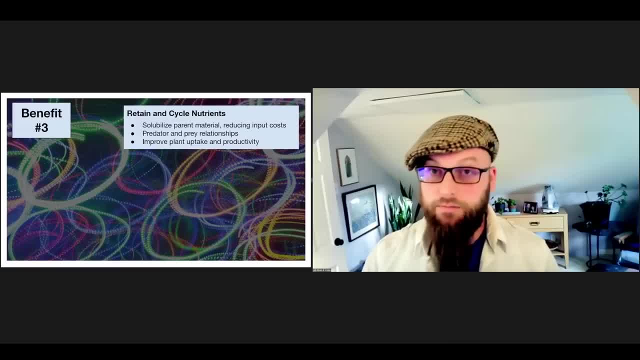 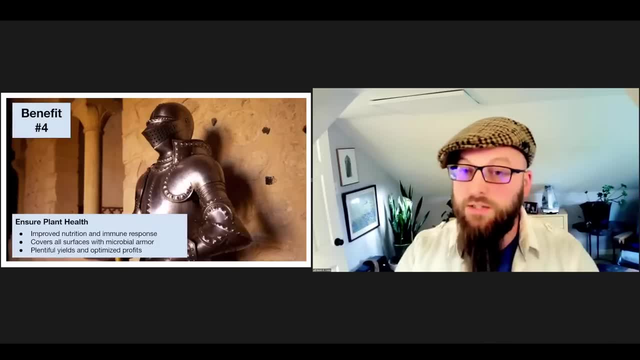 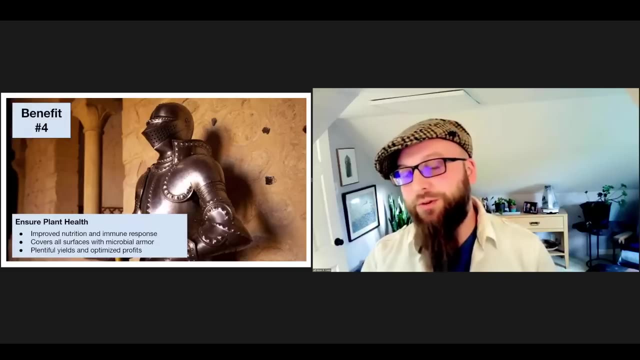 without thinking of these other negative outcomes, but optimizing all the outcomes, And the Soul Food Web can do that. It also protects plant health, not just by improving the nutrition of the plant, but as young plants emerge from soil that is full of all of these. 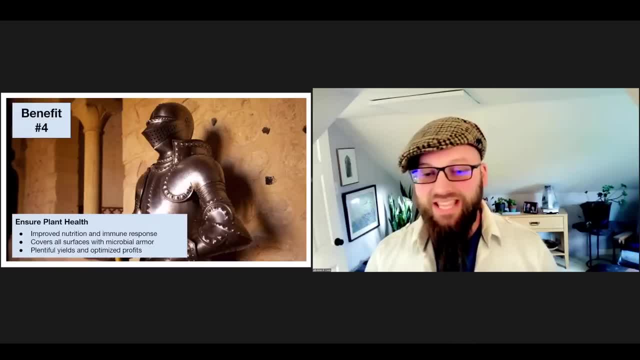 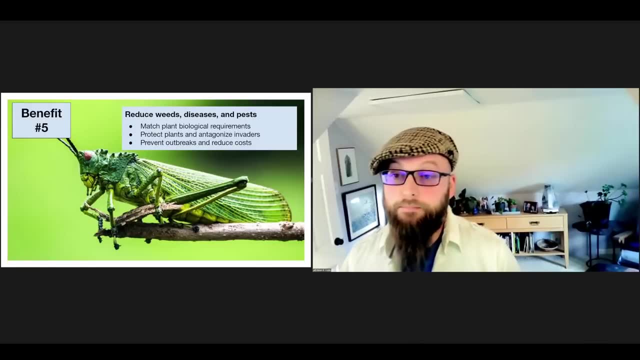 bacteria and fungi and nematodes and protozoa. they get coded in communities. This can reduce disease outbreaks. This can reduce pests dramatically because a lot of times the insect pests that would chew on our plants, they'll just go. I don't want this plant. It's hard to deal with. It's got all these. 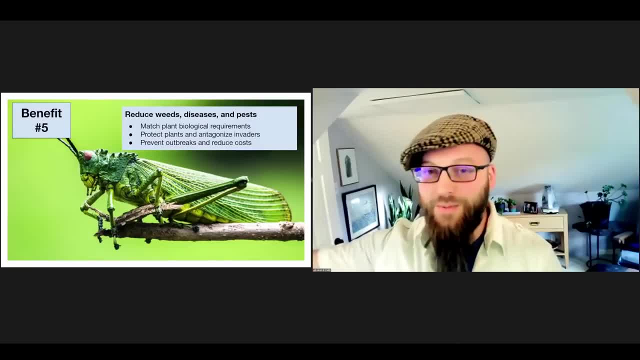 it's got all this arctic And they'll move to your neighbor and eat their plants, And so, yeah, we have just this amazing capacity. There's also antagonistic organisms, So one of my new favorites is there's a bacterial feeding nematode, So it can just happily live in soil eating bacteria. but 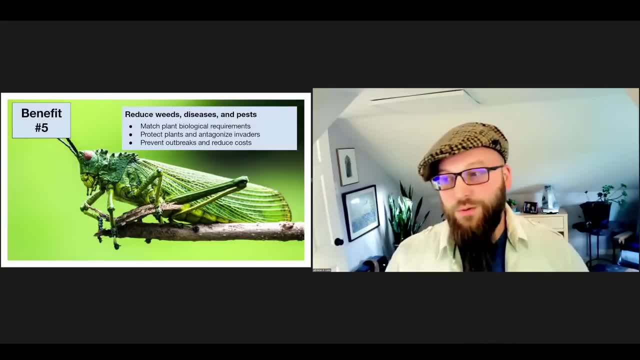 it will. when snails or slugs come into an area, it can infect them. It can infect them, And so, instead of putting out slug bait which has all kinds of nasty stuff in it, or spraying plants to protect them, or constantly, you could have nematodes in your soil system that, 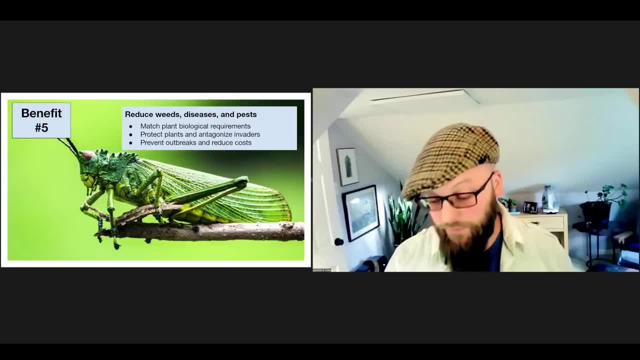 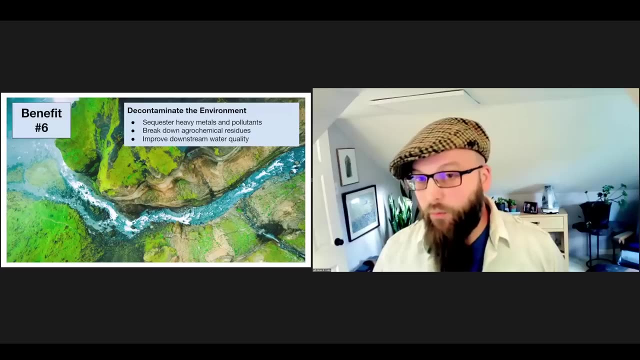 just antagonize and keep the slugs and the snails from getting out of control and eating your plants. This can also reduce your costs significantly. And then we start getting into the bigger benefits, right. The wider environment. Yeah Yeah, We already have soils around the world that are full of heavy metals and other pollutants. 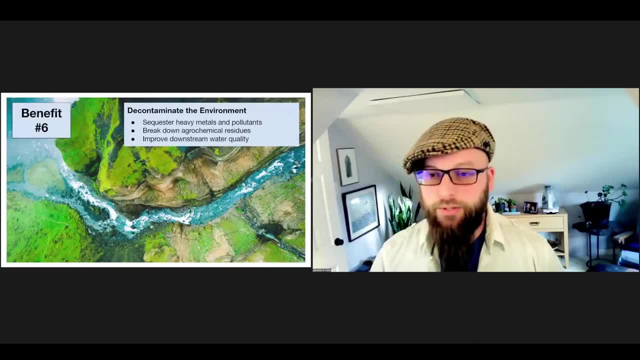 industrial waste and those kinds of you know, even oil and natural gas drilling causes these issues. There can be this remediation of those chemicals. They can be locked away or transformed into something inert by many of the microorganisms That um, that are thriving in a in a healthy soil ecosystem. This can have those effects on. 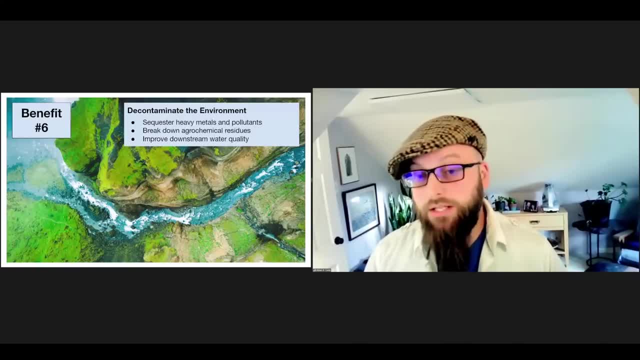 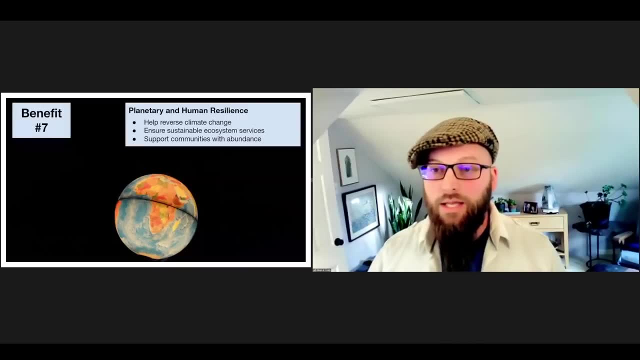 downstream water quality. Uh, yeah, it's, it's amazing, We're it's all connected right. These, these larger systems, even to the point where I can say, globally they can that this full food web, a thriving soil food web, can help us reverse climate change. Um, it can help stabilize those. 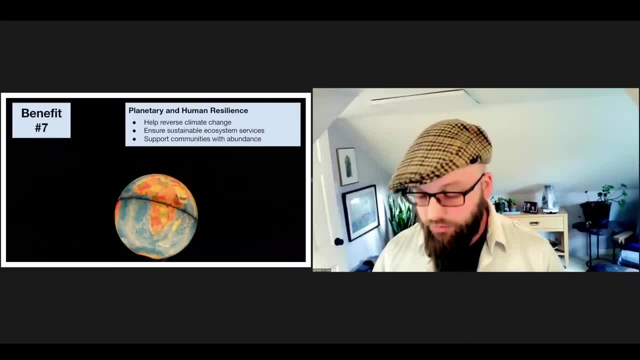 ecosystem services that I brought up earlier and really have this overall supply chain and, and, and, and, and, and, and, to grow, and to grow even more. Yeah, Yeah, They're good, And they're good. It's very useful. 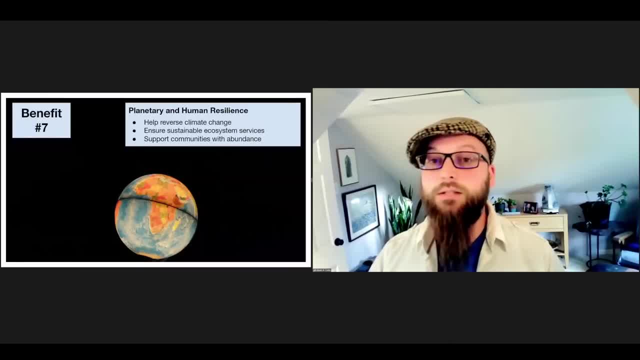 That's good support on human communities right That we can see more abundance and less poverty in the world if we have these. what Dede Pursehouse calls these, this essential workforce going in these systems, as opposed to buying expensive inputs from outside year after year. So here's my last. 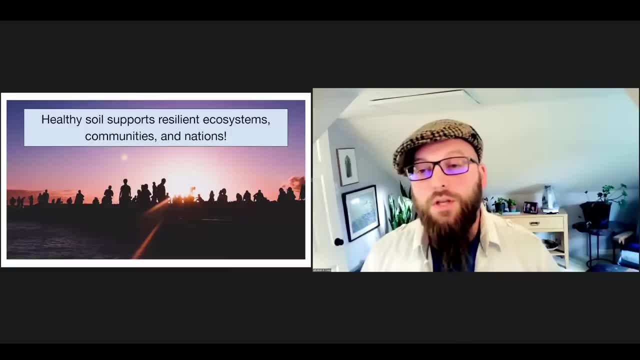 slide. Healthy soil supports resilient ecosystems, communities and nations. And you know US President Franklin Roosevelt, who was in office during the Dust Bowl in the central United States. he famously said: a nation which destroys its soils destroys itself. And so I want us to. 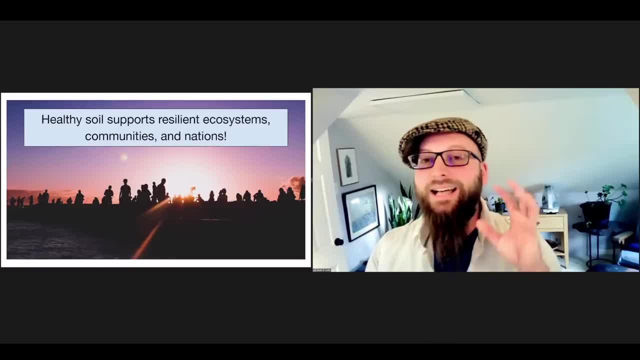 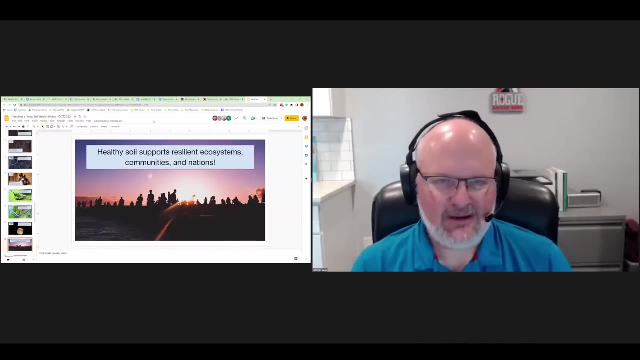 recognize that that also means we can turn that around and say: a nation which invests in its soils invests in its future. All right, Awesome, Adam. What a great presentation. You did it in such a good, succinct way. Great, great job. I think people in the chat are agreeing. 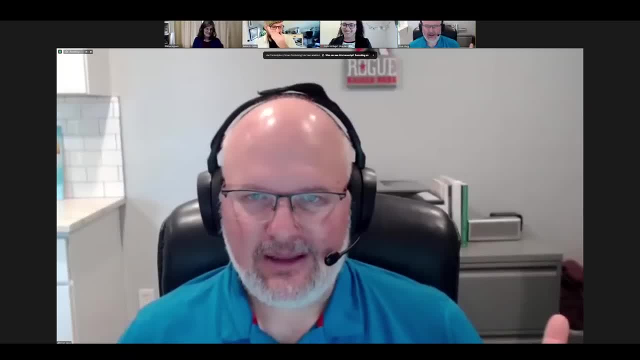 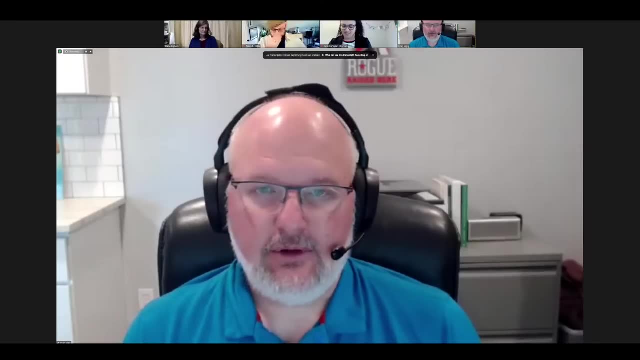 with that sentiment as well. So, okay, let's move on. We're going to have a quick discussion about our October promotion and then we're going to jump right into Q&A And thank you, folks, for putting questions in there. There's some fantastic ones. I think we're going to be able. 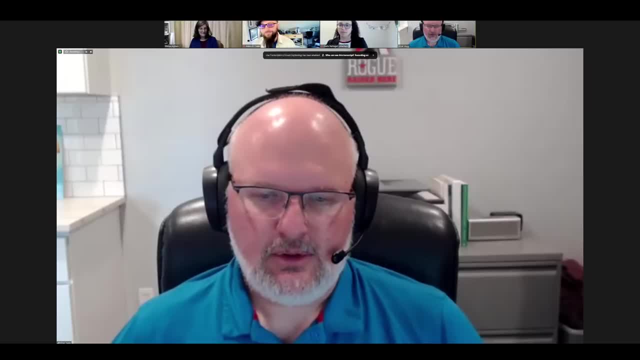 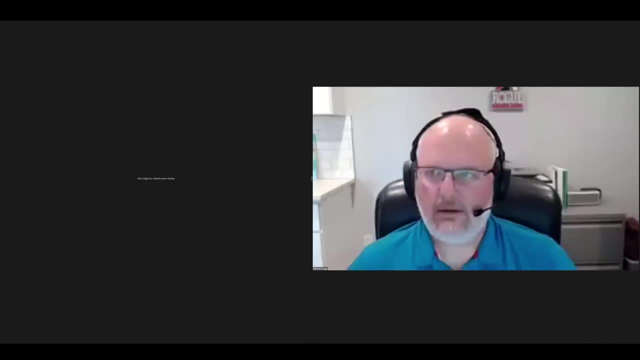 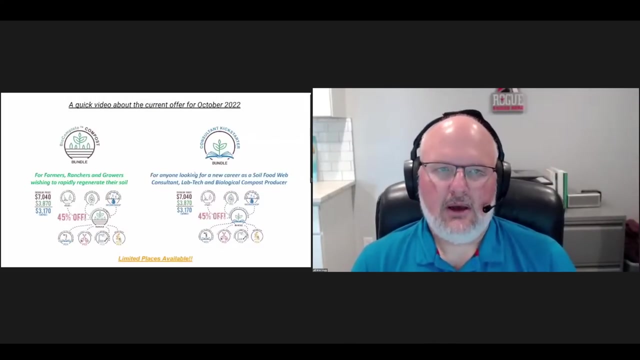 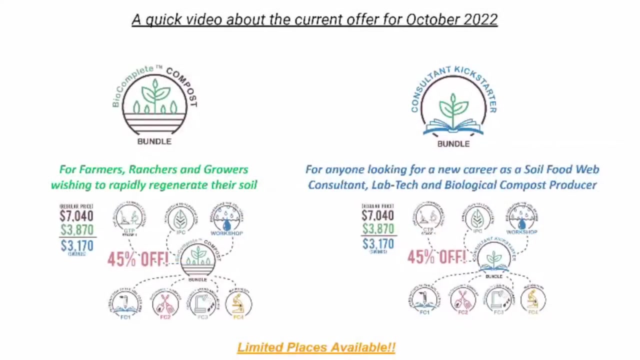 to cover with our panelists today. So, without further ado, let me go ahead and share my screen, All right, And let me go into slideshow mode, Okay. So for October 2022, we definitely have a great promotion where we'll be offering discounts on our BioComplete compost bundle, which is going 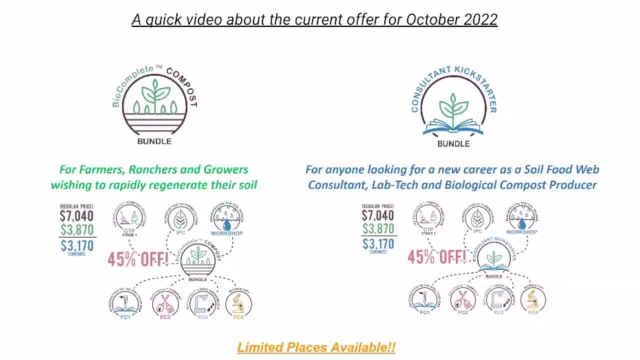 to be really geared towards farmers, ranchers and growers wishing to, you know, really regenerate their soil. And then there's the consultant Kickstarter, which is going to be more geared to folks that actually want to do kind of the work that I do, which is being a consultant, and 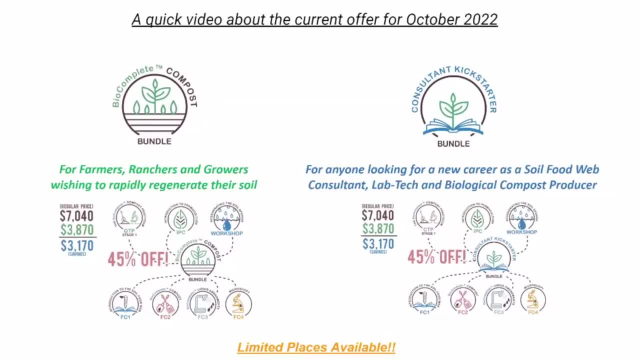 helping people transform their soil. And then there's the consultant Kickstarter, which is going to be more geared towards farmers, ranchers and growers wishing to transform their growing operations from agrochemical, traditional, organic to farming with biology, And so you can see, 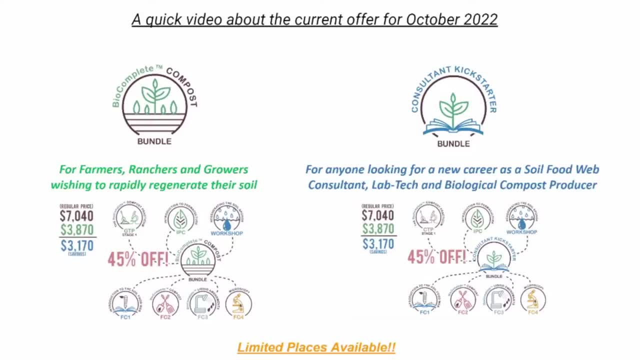 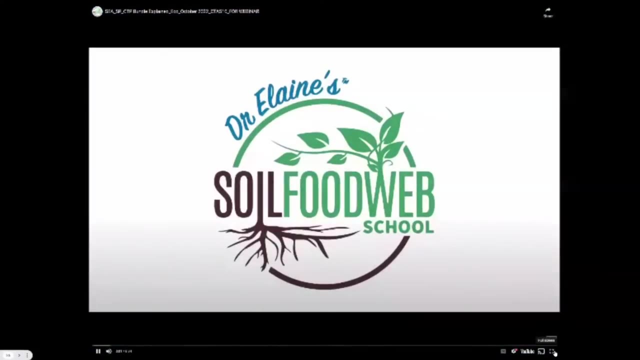 there's some pretty significant discounts with this particular promotion, And what I'm going to do is go ahead and run a video here that's going to talk about the promotions and what we do here at the Soil for Web School. All right, If you're interested in joining the Soil Revolution. 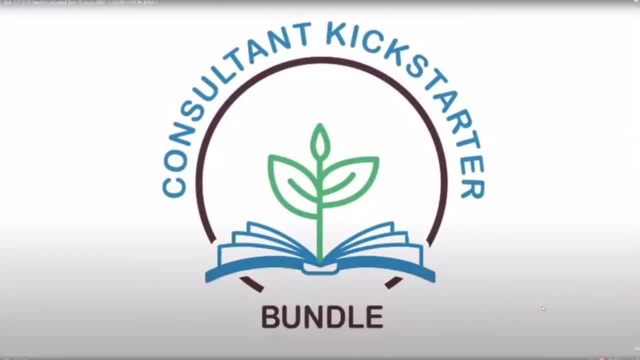 this is a great time to do so. So if you're interested in joining the Soil Revolution, you're welcome to join. With a consultant Kickstarter bundle, you can register for the soil Food Web Foundation courses with Dr Elaine Ingham for just $3,870, saving. 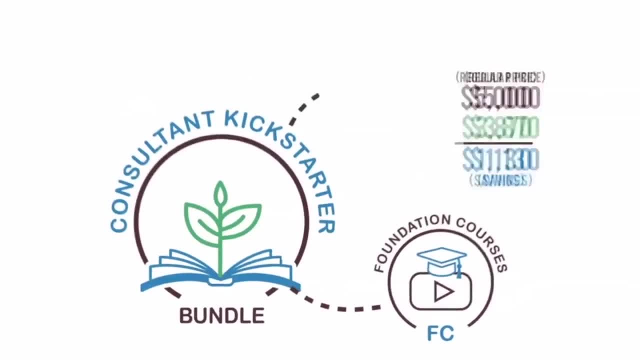 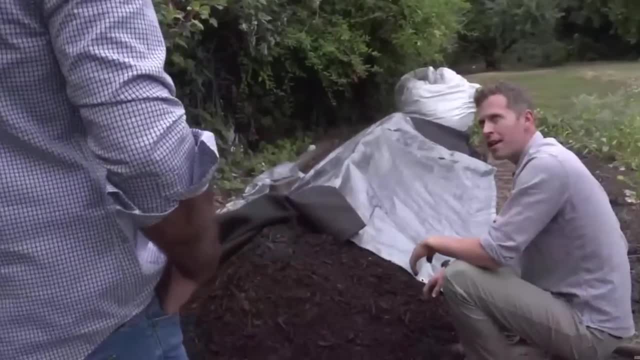 over $1,100. through October 20th, You'll also get Stage one of the consultant training program totally free, saving a further $1,540.. That's 26 hours of mentor time dedicated to helping you make your own biological compost and develop your 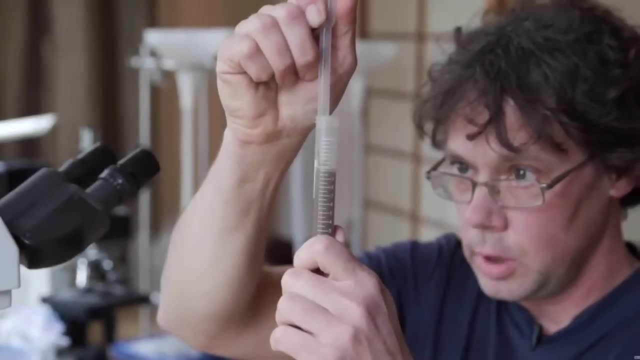 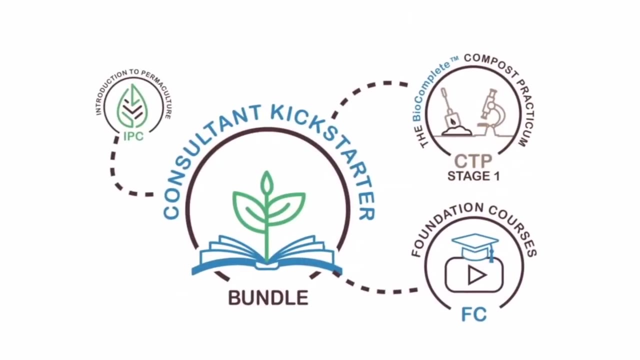 microscopy skills to the standard required to qualify as a certified Soil Food Web technician. you'll also get two free bonuses with this offer: the introduction to permaculture course with Graham Bell and the soil sponge regeneration workshop with DD purse house, saving a further $500 the total value of this. 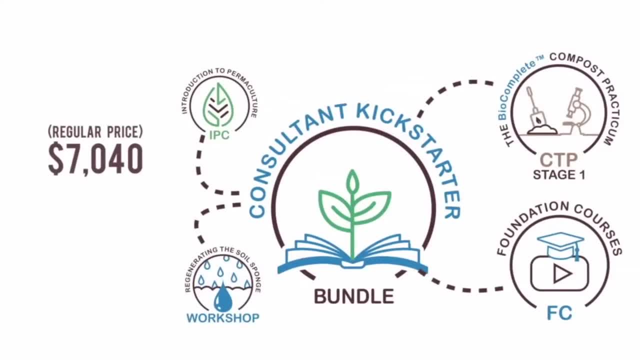 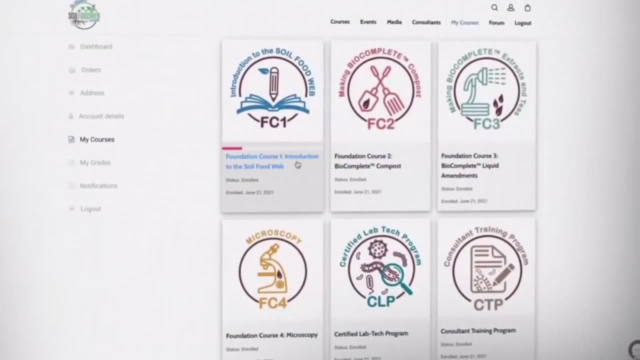 bundle is over $7,000, for which you'll pay just 3870, saving over $3,100. that's 45% off. there are limited places available with the consultant Kickstarter bundle, so please don't delay. in foundation course one, you'll take a deep 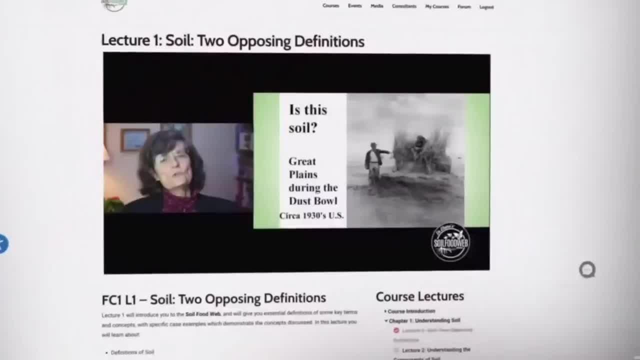 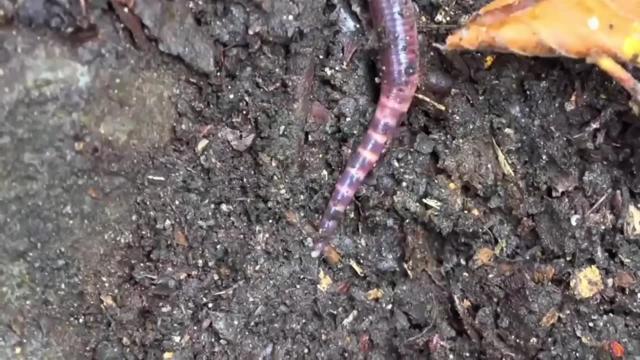 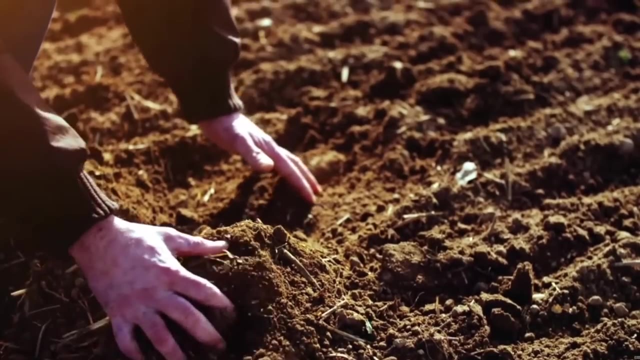 dive into the science and methodology that underpins the soil food web approach, which was developed by dr Elaine Ingham. over the last four decades, you'll study the history of soil on planet Earth and how the agricultural practices we've been using in the last hundred years have degraded our soils to 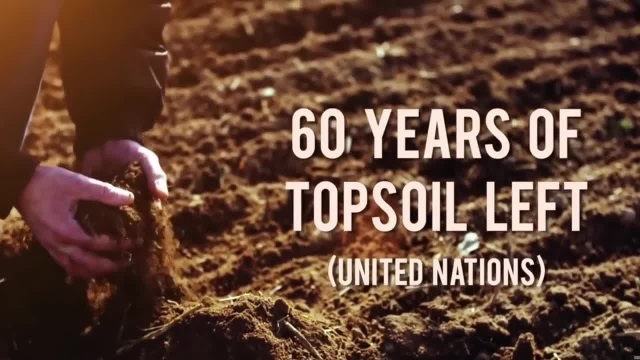 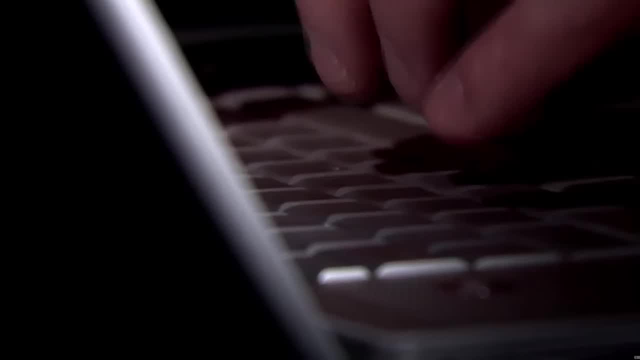 the point where we now only have around 60 harvests left, according to the United Nations. you'll learn about the solution to many of the problems that we've been dealing with in the last hundred years and how the problems that are familiar to farmers all over the world today problems. 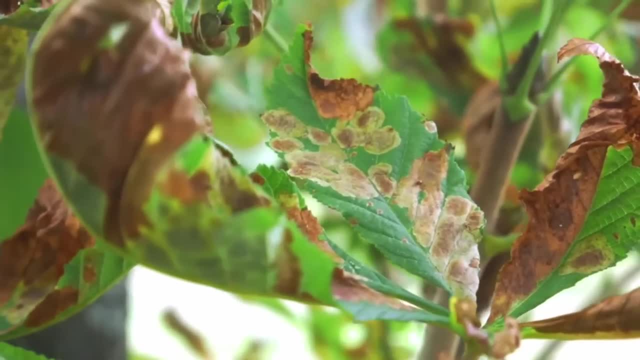 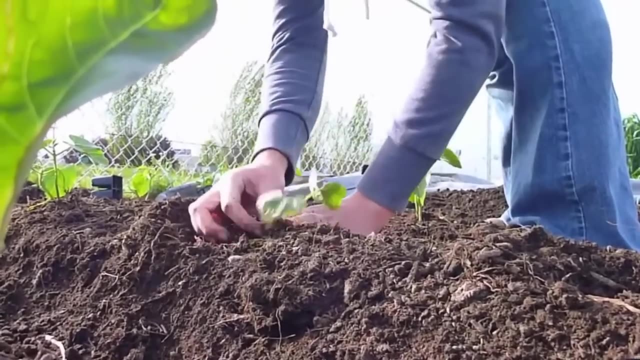 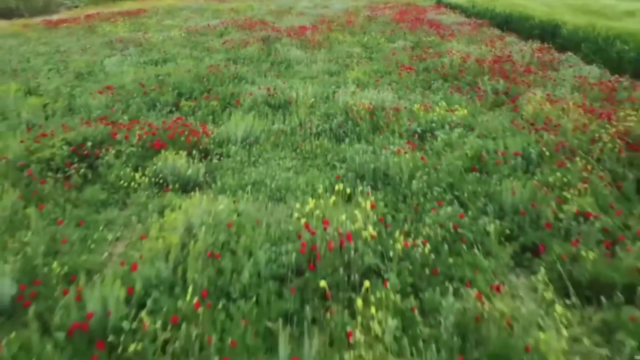 like diminishing soil fertility, pest and disease pressure, low crop yields, drought, flooding, compaction and soil erosion. regenerative agriculture can address all of these problems. you'll be introduced to regenerative practices like no-till and the use of cover plants. you'll also learn about the four major groups of 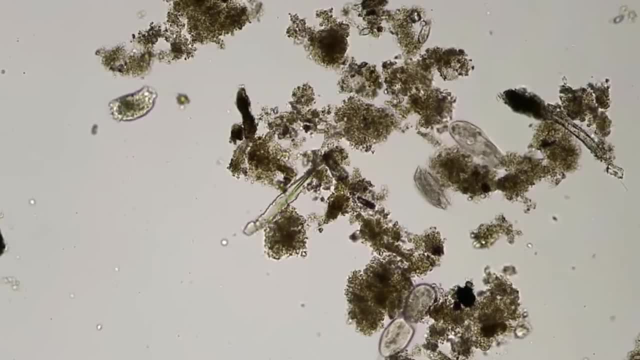 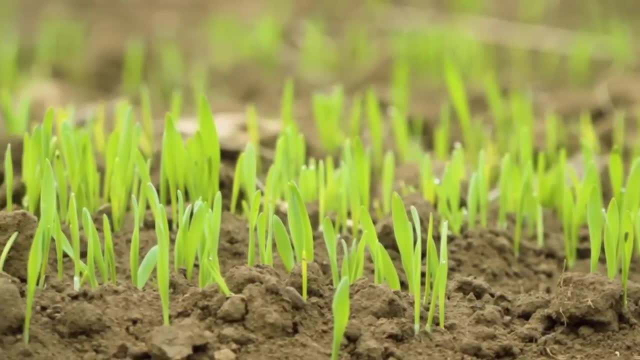 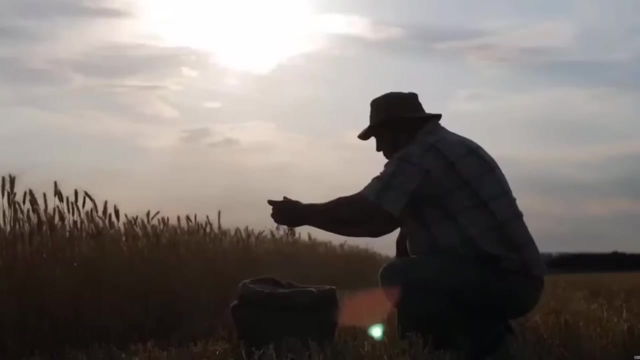 microorganisms that drive soil regeneration and how the process can be accelerated by restoring the soil to its original state, by restoring the microbial community, or soil food web, to your client soils. dr Elaine will present a number of case studies from around the world that she has worked on personally. here you'll see some of the amazing results that have. 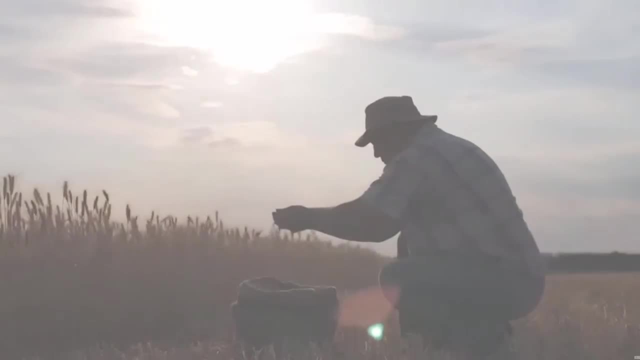 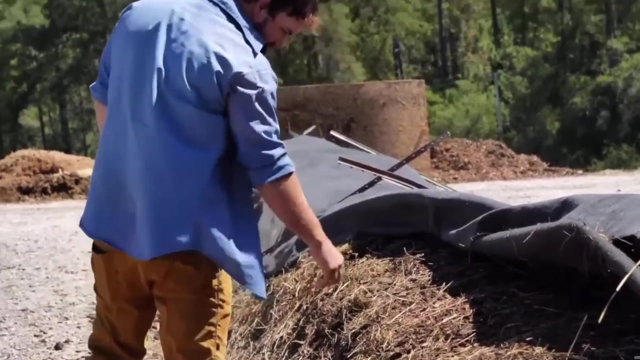 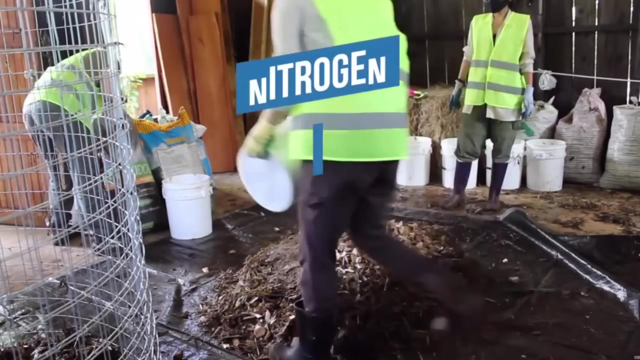 been achieved using the soil food web approach. in foundation course 2, you will learn all about the importance of biological compost and how it's very different to regular compost. when most people look at compost, they only see a means of delivering nutrients to their plants, so they think about how much nitrogen, potassium, phosphorus and other elements. 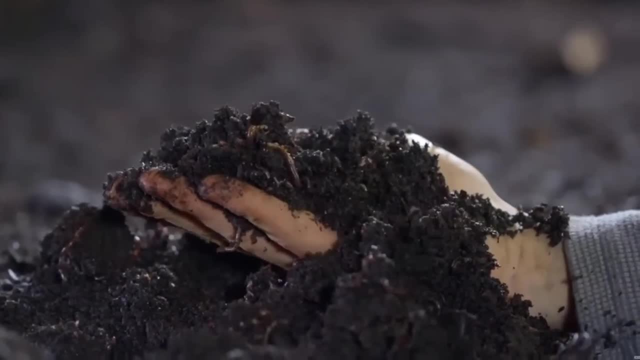 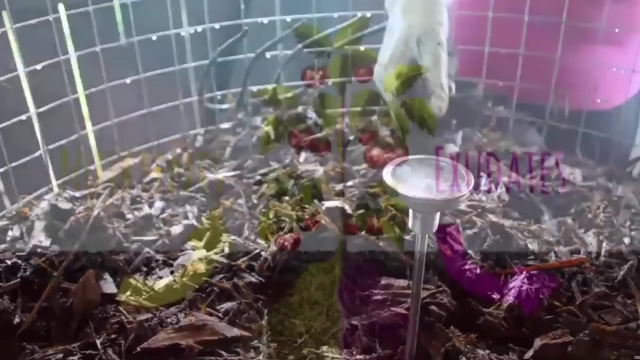 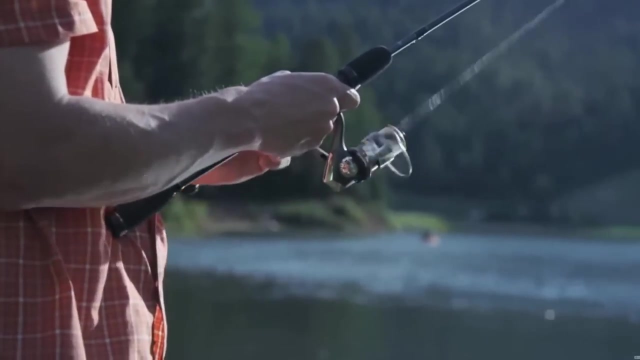 are in the compost. when we look at biological compost, we see a means of inoculating the soil with beneficial microorganisms so the soil ecosystem can start to function again, providing plants with a continual supply of nutrients. this is kind of like teaching someone to fish so they can feed themselves for. 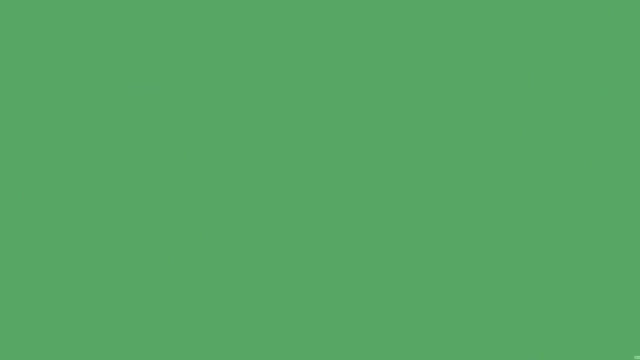 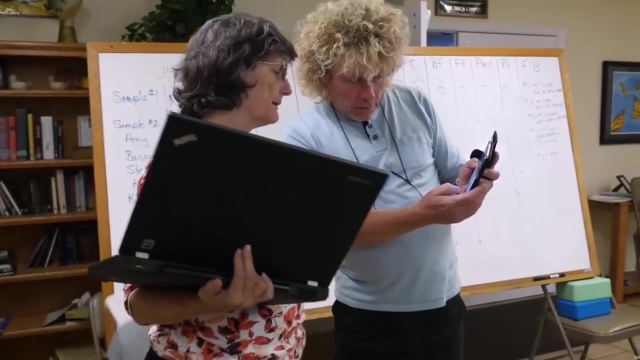 life, as opposed to just giving them a single meal. in this part of the training, you will learn how to make biological compost and how to make organic compost for your plants, using various starting materials to create a recipe that will produce results. you'll learn how to monitor and control moisture levels, aeration and temperature. 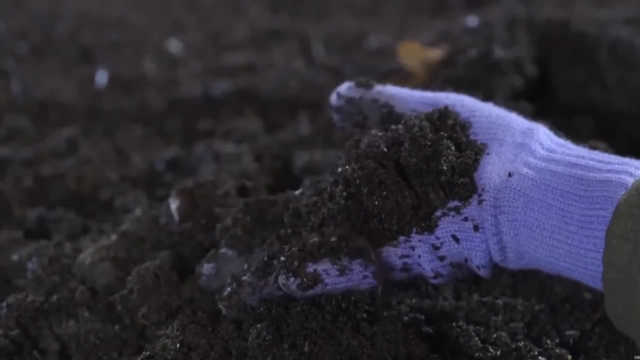 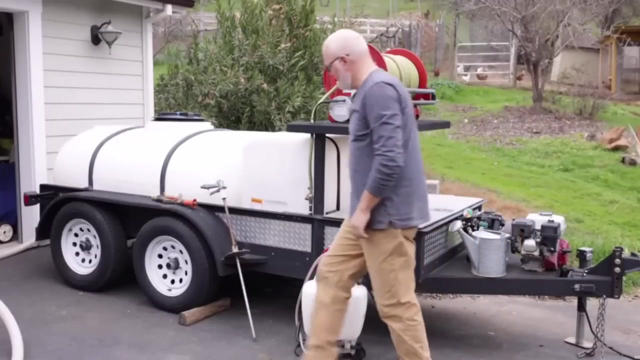 in order to ensure that beneficial microorganisms are multiplied while disease-causing organisms are destroyed or become dormant. you'll also learn about the various types of equipment that can be used at different scales, and you'll learn about the different ways in which biological compost can be applied. 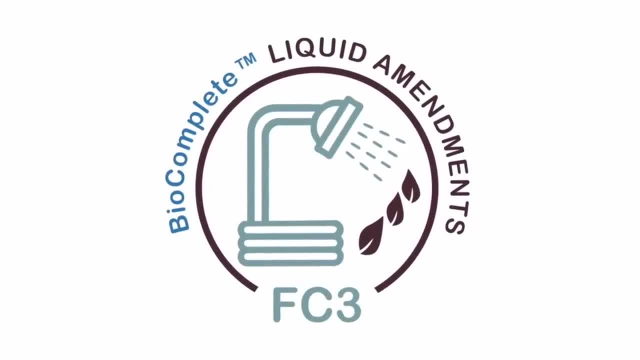 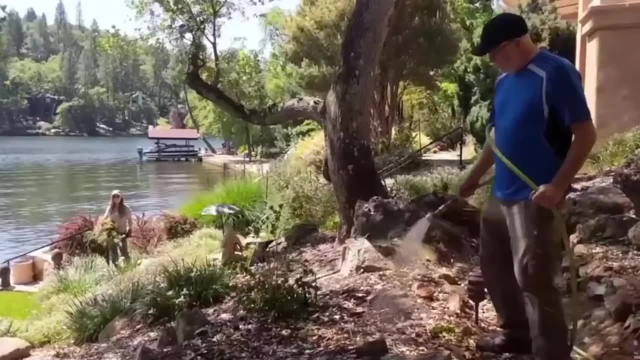 to the soil. in foundation course 3 you'll study dr Elaine's methods for making liquid biological soil food web and how to make organic compost for your plants. soil amendments- compost extracts are used as a soil drench, delivering microbes deep into the soil profile where they can interact with the plant's. 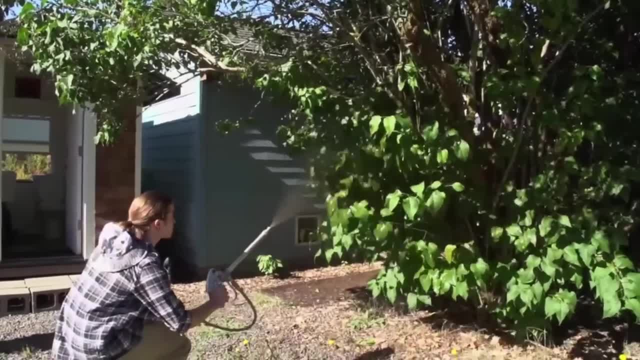 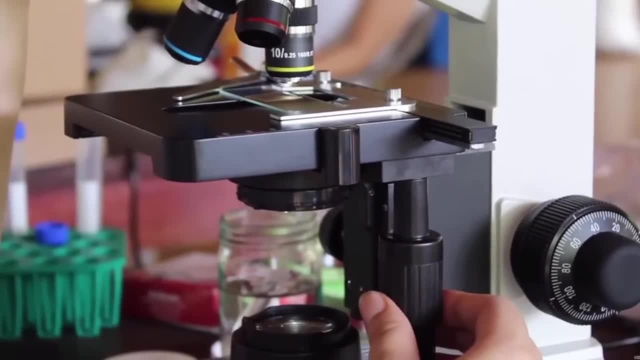 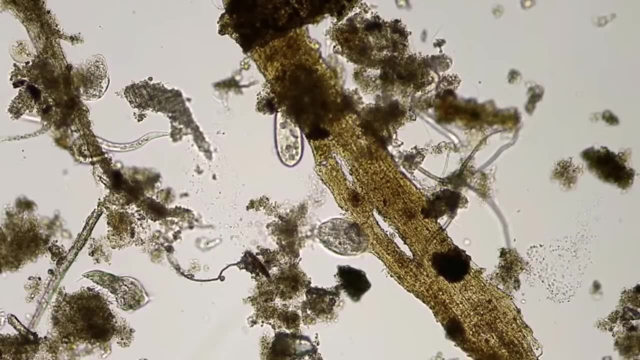 root system, compost teas are applied to the plant's foliage, where they form a protective barrier against foliar diseases. in time, as your soil biome becomes more diverse and vigorous, your plants and trees may be entirely covered with beneficial microbes without having to continually apply them in foundation. 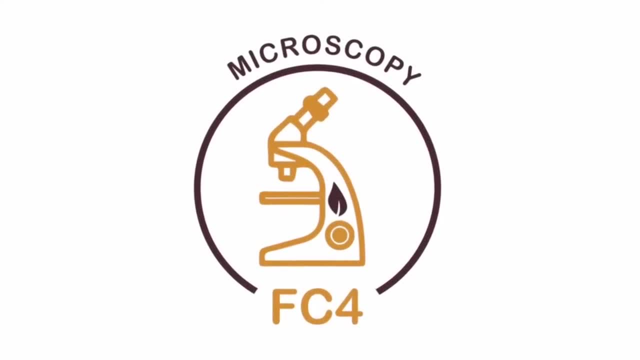 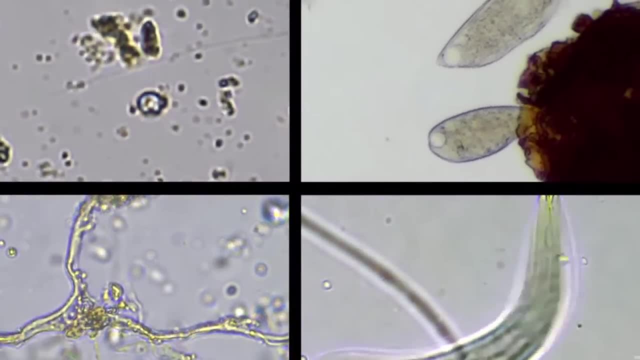 course 4 you'll focus on four different methods to make organic compost for your plants: major groups of microorganisms in the soil, food web, bacteria, fungi, protozoa and nematodes. you'll learn how to use a compound microscope to identify and quantify these microbes so that you can really see what's going on in your 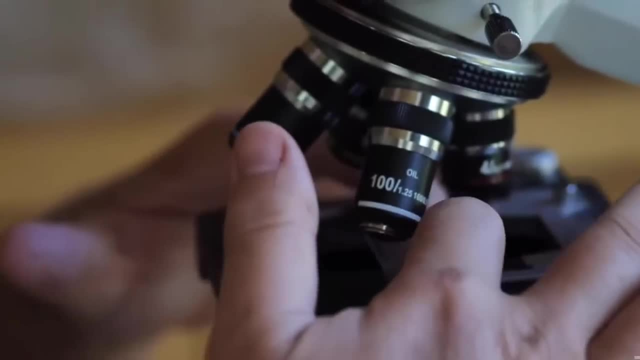 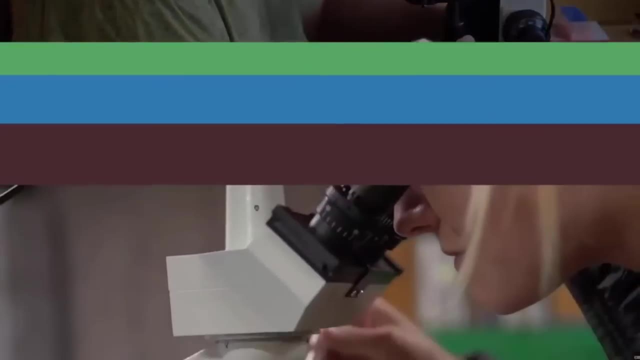 compost and in the soil. this will give you the ability to assess the quality of your compost and liquid amendments before you invest all the time and effort that is required to apply them to the soil. you will also be able to monitor the progress of the microbial community in your soil over time. so if 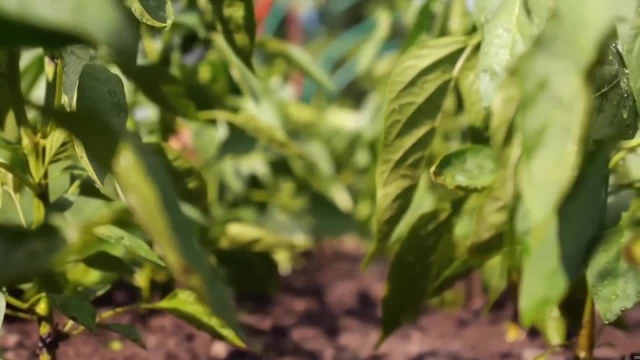 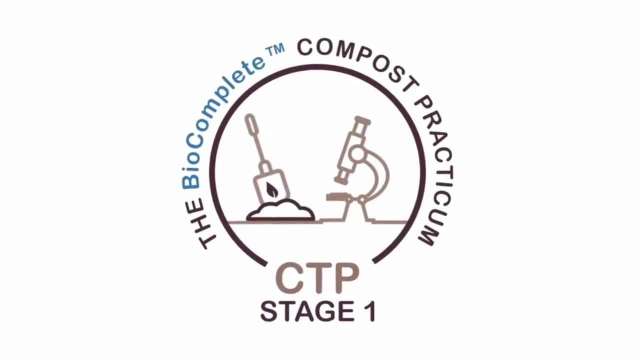 something is going wrong, you will know about it before the plants start to suffer. this gives you the opportunity to take remedial action early on in the growing season. in stage one of the consultant training program, you'll be assigned to one of our highly skilled mentors, some of whom are soil food web. 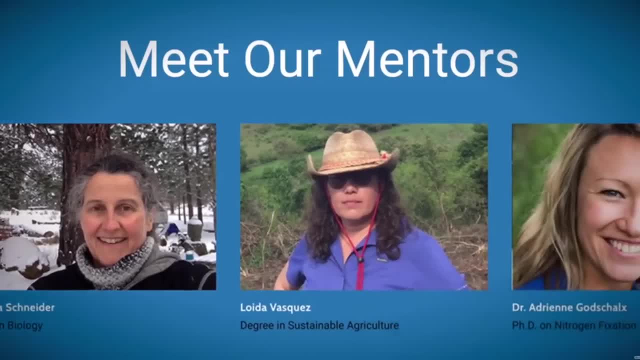 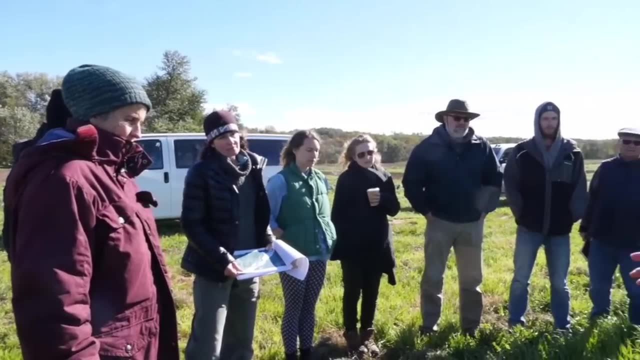 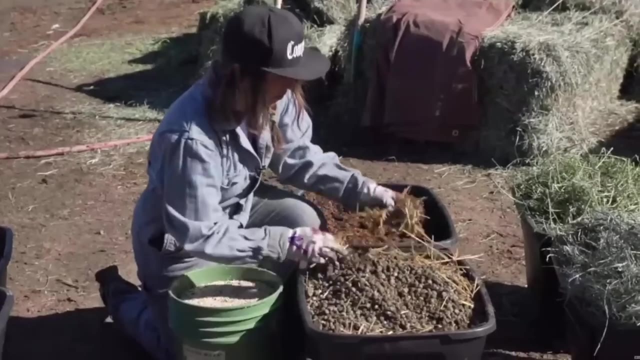 consultants who run their own businesses supporting farmers to make the transition to the soil food web approach, and others are PhD biologists who have been working closely with dr Ingham for several years. you'll work one-on-one with your mentor to develop your compost making and microscopy skills. when it 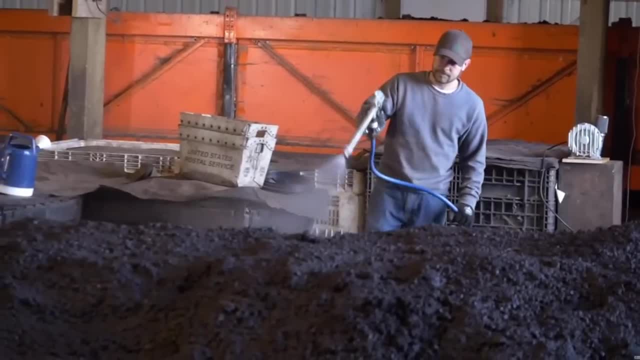 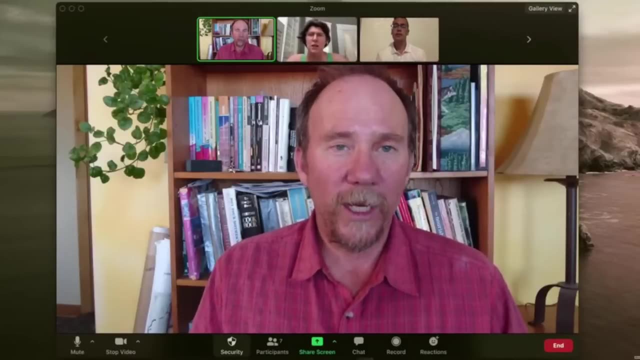 comes to making great biological compost, there are many variables and every situation is different. our mentors have worked with dozens of students making compost in many different conditions, so they'll be able to help you address some of these challenges that are unique to your location. they'll also guide you to 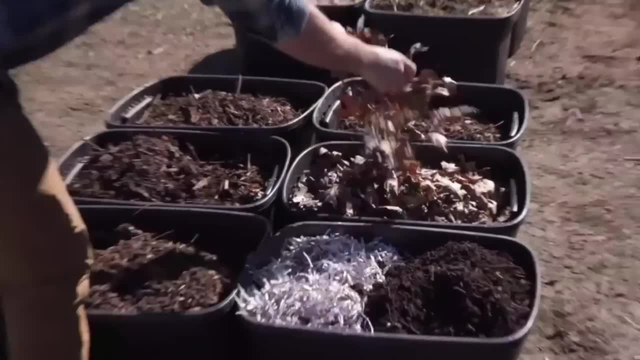 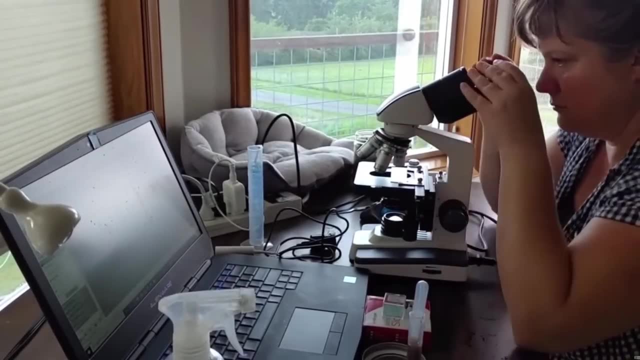 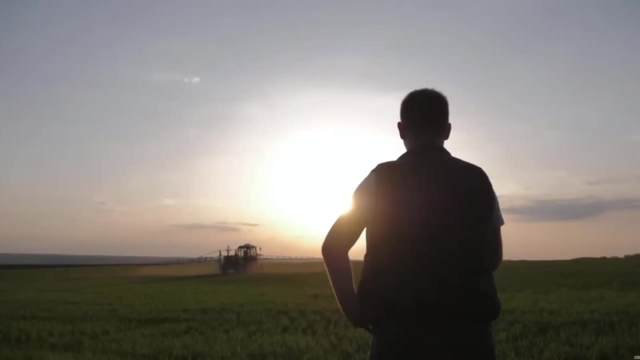 avoid making common mistakes that can cost you lots of time, money and effort. your mentor will support you as you develop your skills to the required standard to pass the microscopy proficiency assessment. achieving this standard will give you the confidence to really know what's happening in the microbial community in your compost and soil. you'll be able to identify and 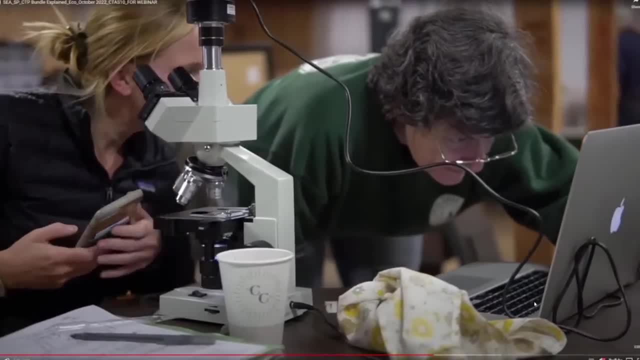 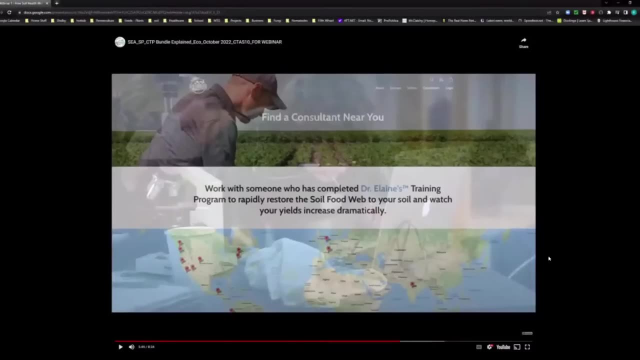 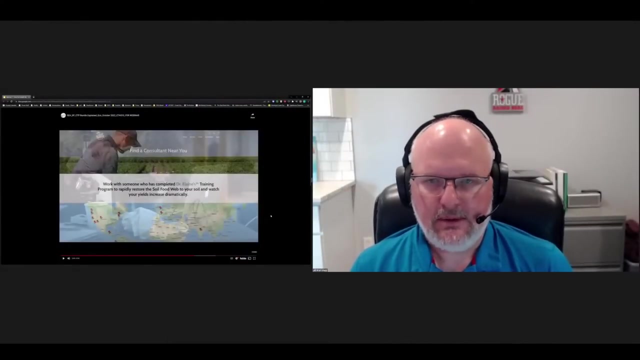 quantify the four major groups of microbes in the soil in about an hour or less. once you. thank you everybody for watching our video about our October promotion and if you want to find out more information, please visit our website. and I know that there are some limited space for questions, but I will be happy to answer any questions you may have. 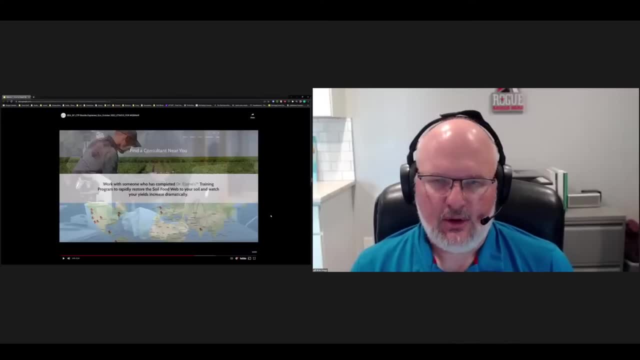 Thank you everybody for watching our video about our October promotion, and if you want to find out more about让您 楼上port事件有问题就请找我们的不是按照上方的评测区是我们的楼上注册区有空间不然我们会在哪里知您的所以请先在下方加入我们的评测区. 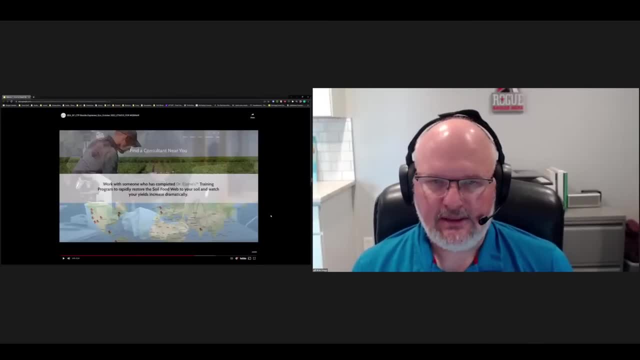 go ahead and definitely take a look at the information that we have and hopefully something fits for you and we'll be able to see you guys coming in as students or as potential growers or consultants. All right, let's move on to doing some Q and A. 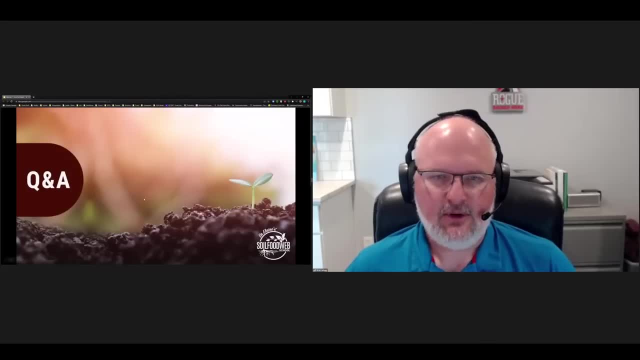 So there we go. So our first Q and A question, and this is going to be for, so I wanna make sure our panelists go off mute. This first question is coming in from Vince, which is: I would like to know if there are some tools. 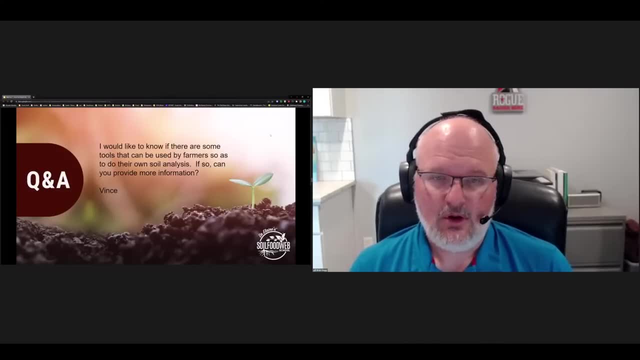 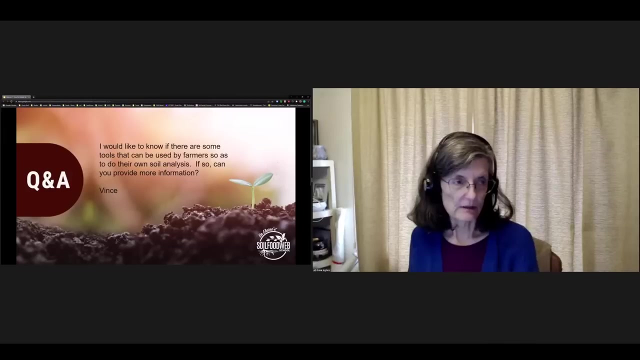 that can be used by farmers so as they can do their own soil analysis? If so, can you provide more information? So what say you panelists about farmers being able to use different tools to analyze their soil? So are you hearing me? 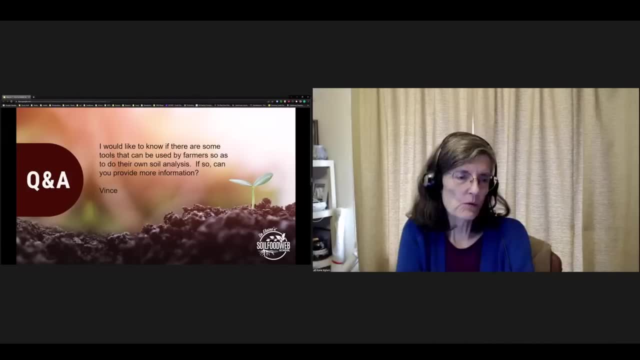 Yep, you're there, Elaine, Yep, all righty. So the tools kind of depend on how precise the soil is, how precise you feel you need to be, to get the changes in the soil that will do all these wonderful things for your plants. So you can go fairly simple by getting a metal rod and pushing that metal rod into the soil to find out where the compaction layer is, where your water is puddling and not moving down through, And then how do you get those organisms back into the soil? 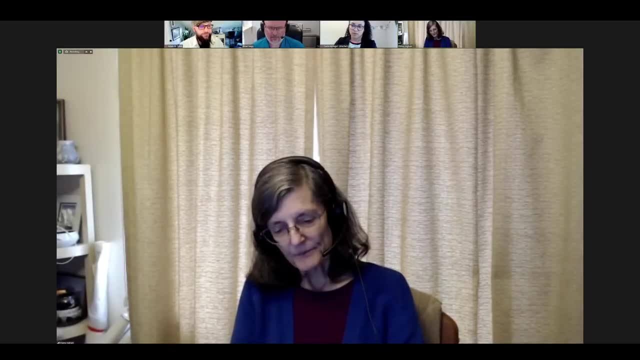 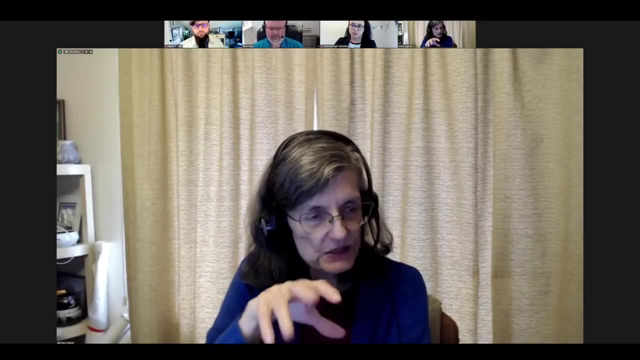 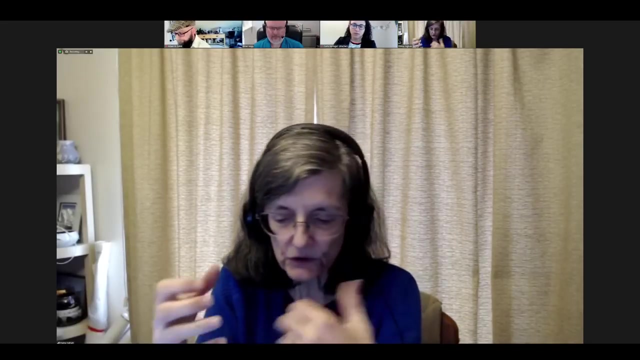 If it's missing? do you want to kind of do guesstimation by picking up a handful of soil, shaking it and looking at the airways, the hallways, the panels, the passageways for the oxygen water routes and the organisms to move through? 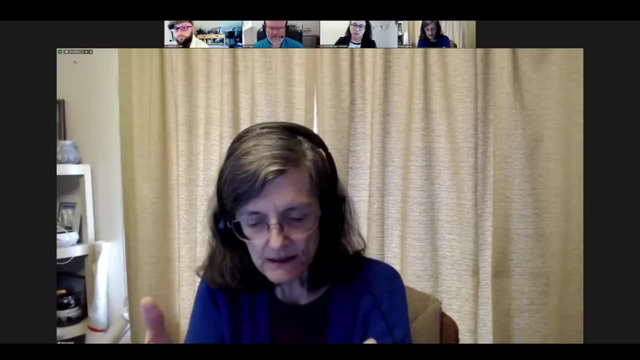 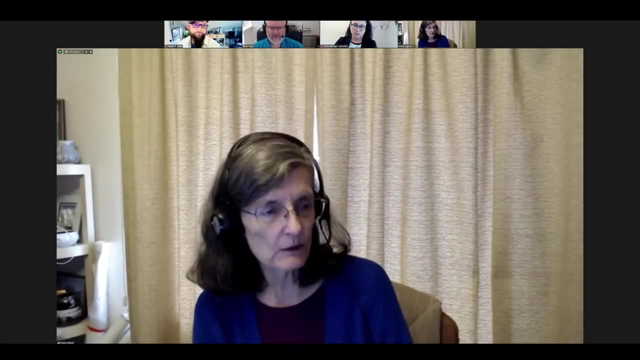 It's hard to be real, concise or precise if you don't have something where you can quantify, And so we always encourage that you buy a microscope, simple microscopes or nothing fancy. We always encourage that you buy a microscope, simple microscopes or nothing fancy. We don't need electron microscopes. It'd be nice, but we don't need the electron microscopes for the kind of work that we're doing out in the field. So a good microscope, light microscope- that costs somewhere between 350 to maybe $500,. 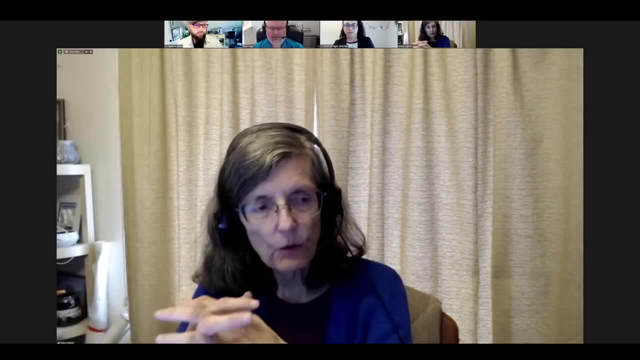 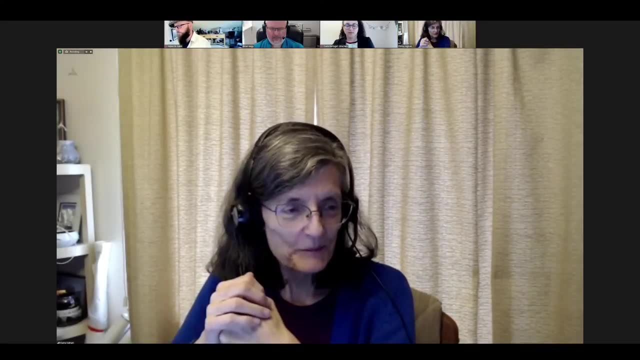 a camera to be able to record the organisms that you're seeing, especially if you have questions about what you're seeing. You see your very first, your very first, your very first protozoan in your soil samples and you're not sure. 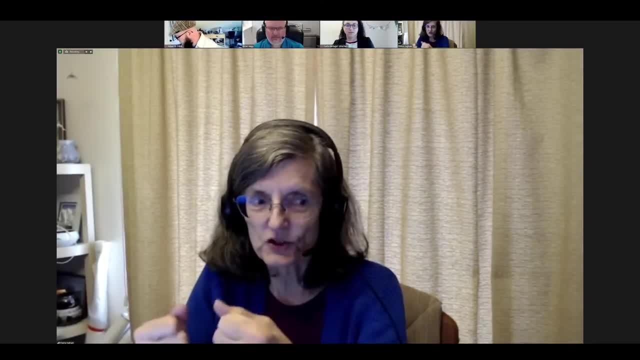 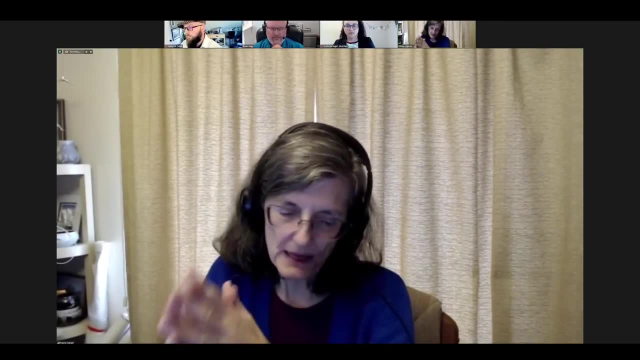 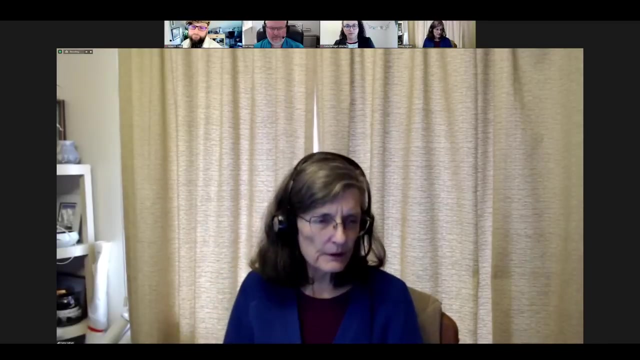 protozoan in your soil samples and you're not sure. you really want to have the help of somebody here at the school to be able to assure you that here are the characteristics. this is what you need to be looking for, So there are quite a number of ways. 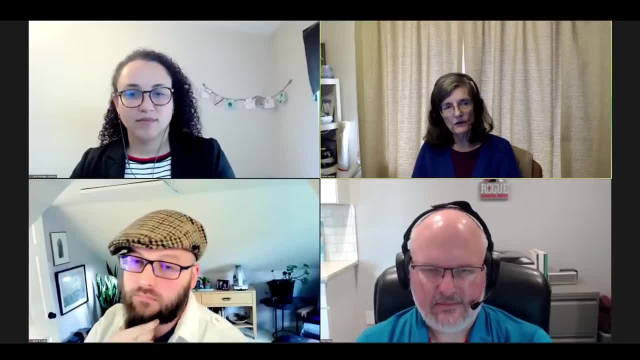 to get the biology back out into the soil. How are you going to make your compost? You know somebody in the chat said you know you can make your compost. How are you going to make your compost? You know somebody in the chat said you know you can make your compost. 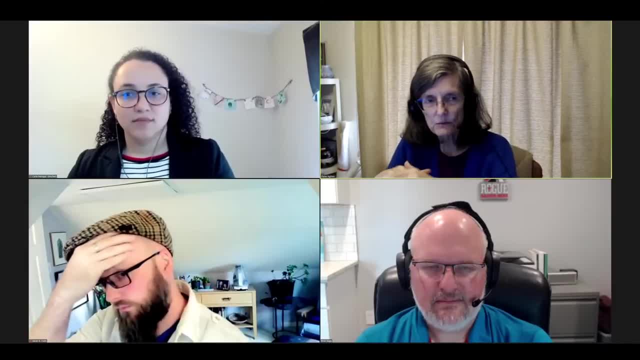 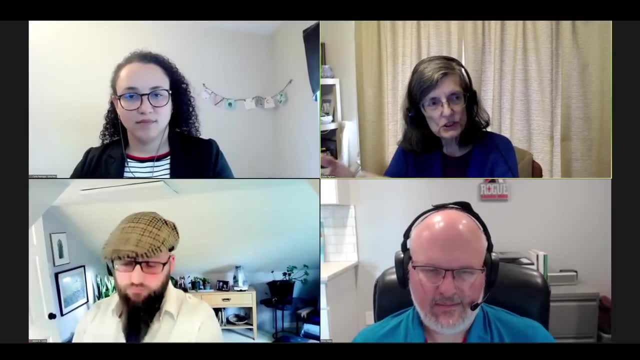 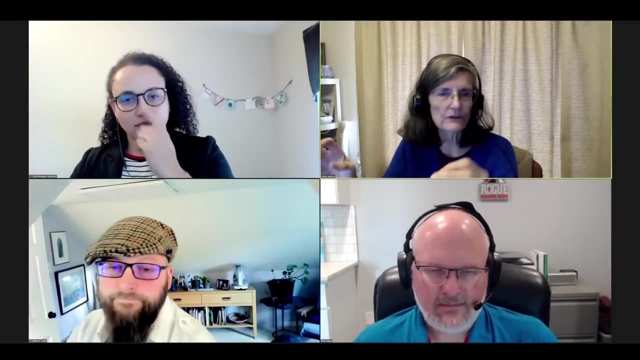 How are you going to make your compost? You know you can make your compost, Make worm compost. Somebody else said: well, thermal compost is better. It really depends on your lifestyle: which way of making the biology in that soil get the whole diversity. 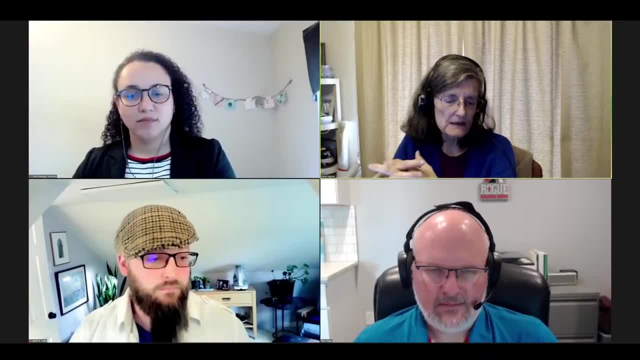 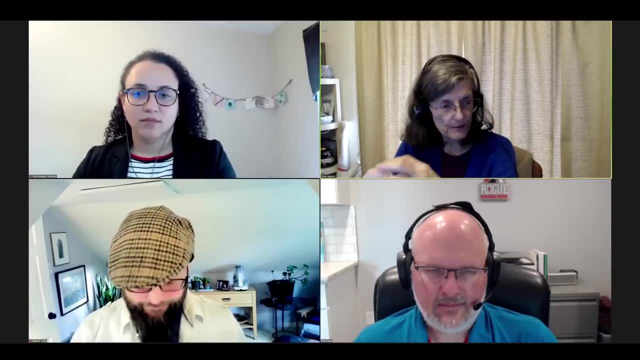 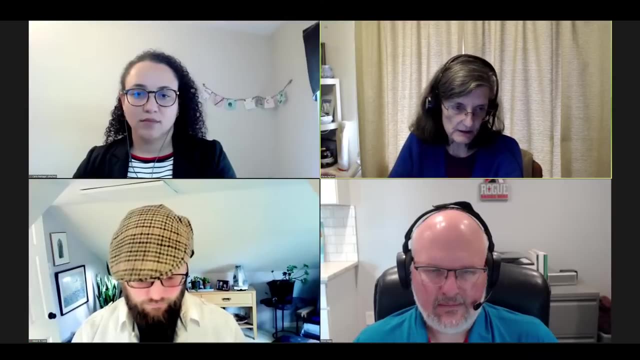 get all of the organisms moving properly, interacting properly. We want to make certain that we have the conditions that select for the beneficial organisms, that select for the beneficial organisms because something that's going into your pile is going to have human pathogens on it. 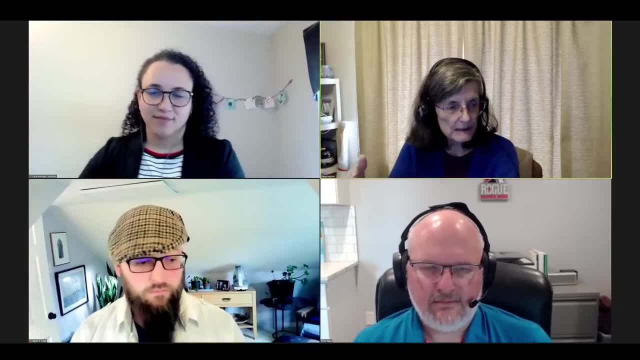 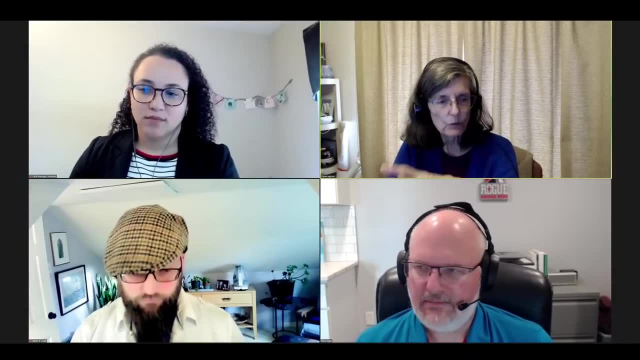 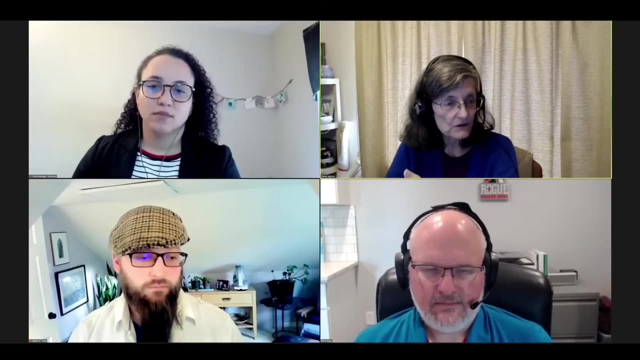 There might be some animal pathogens, there might be plant pathogens in there, And so we want to make certain that we are taking care of, we're wiping out, we're preventing any of those bad guys from being able to reproduce or out-compete our beneficials. So it's really important that you pick a composting process that you that fits in with your lifestyle. When you're doing a worm bin, you have to really be looking after that worm bin. at least once every three days you have to be looking at your worm bin. 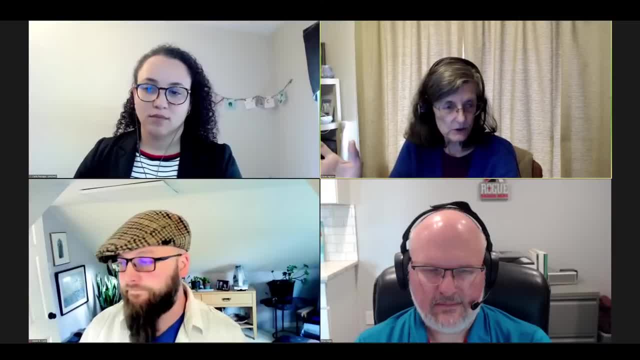 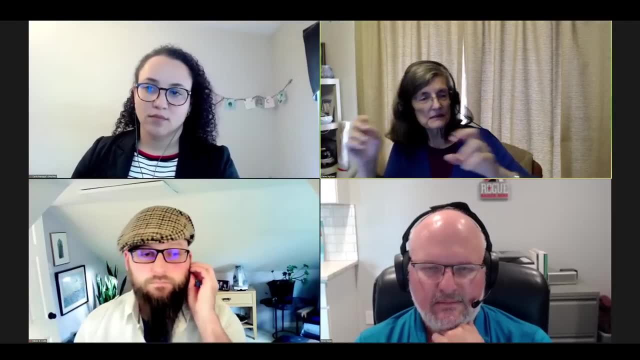 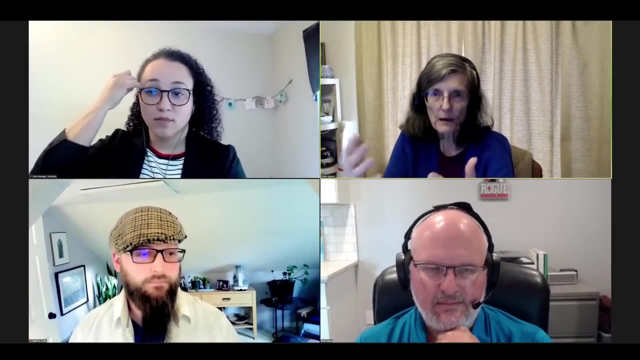 and adding more food or deciding to wait on another day. If that's your lifestyle, that you can spend five minutes, 10 minutes every day basically interacting with your worm pile, your worm compost, then go for it. But what if you don't have that kind of time? to every single day, be able to interact and work with your compost pile. So now thermal compost becomes the most probable way of you being able to get the amount of compost that you need for a small scale, for your yard, your garden, you know, a one to 10 acres. for a small farm. You'll be making a compost pile in the springtime, in the middle of the summer, late fall and maybe even again in winter, if your winters aren't too extreme. If you live in Minnesota, you're not gonna probably deal with. that full on wintertime compost piles, You'll just make larger compost piles the rest of the growing seasons. So with a thermal compost you're going to wanna search out the recipe for the starting materials. You've gotta be measuring that temperature. 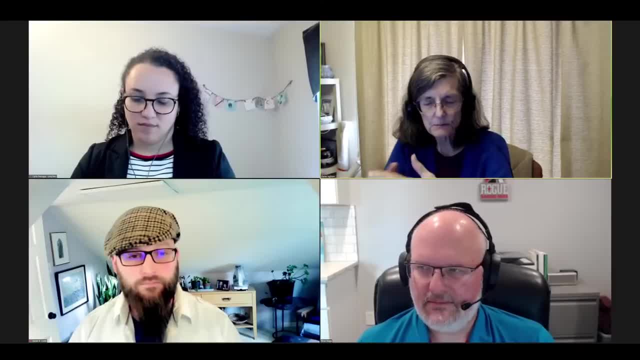 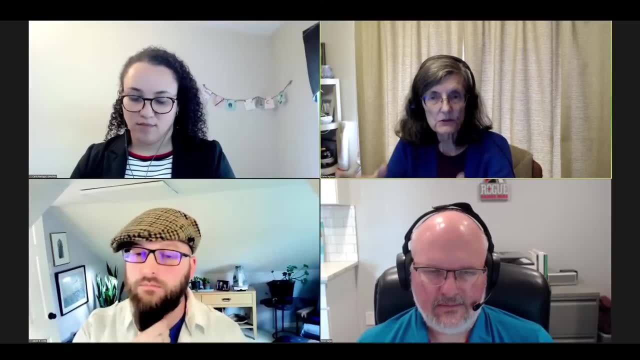 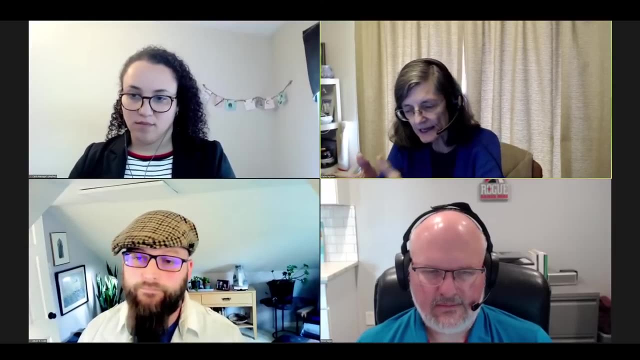 checking up on it every couple of days. typically You have to be able to turn that pile when the time and temperature says it's time to turn. But you only have to hold those temperatures. You only have to work that hard every day out there. working with your compost pile. You only need to work really hard for about 10 days. And then the process where things could go wrong if you're not paying a daily attention. that's over and done with by about day 10.. Another 10 days and you will have. typically, if you've done it right, you have compost that you could put out into into your potting mix. You could put it in the beds, You can use it to make extracts. You can use it to make tea. We wanna be able to put the liquid forms out on surfaces. 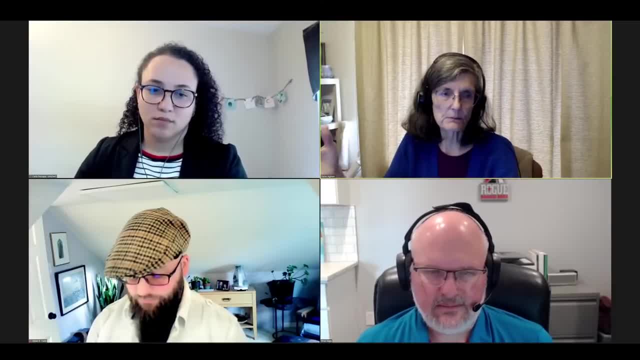 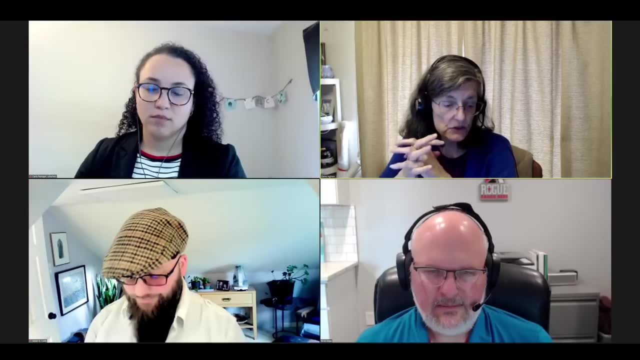 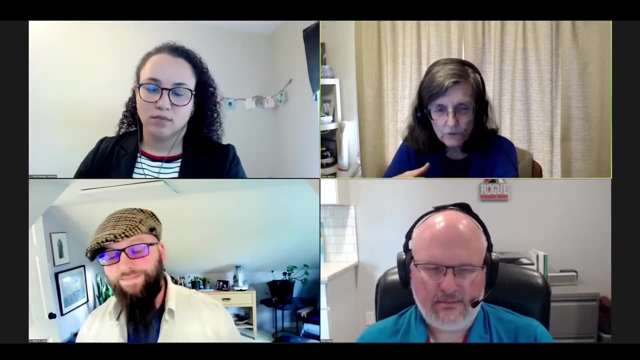 to protect the above ground part of your plant from the diseases and the pests and the problem organisms. We wanna put in drenches that get all of this biology into your soil. And there's we talk about several different ways of getting that biology. what works best for you? 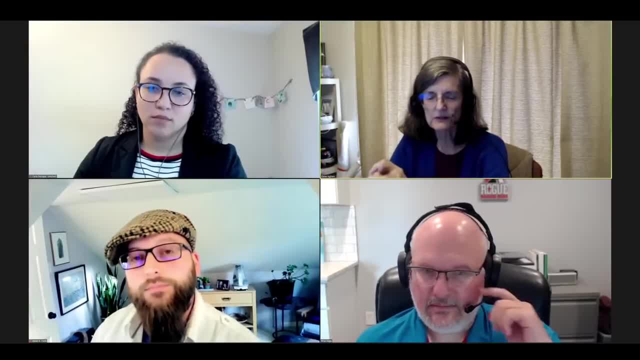 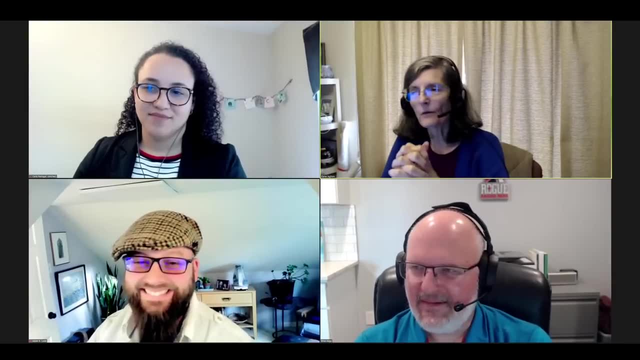 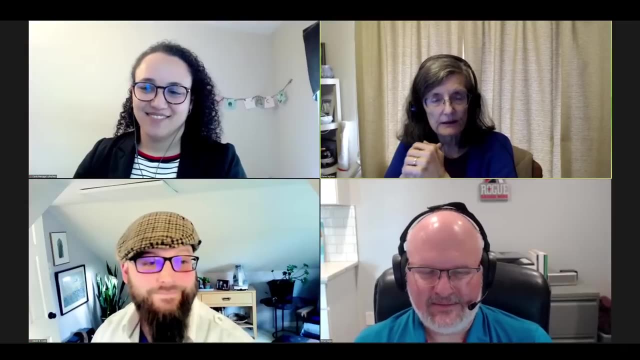 Well, what climate are you in? What plant are you trying to grow? What is your soil? So Ralph just said: where are we? Do we have any people in Nigeria? And yes, we do have people in Africa. So we're getting to be pretty around the world about this. 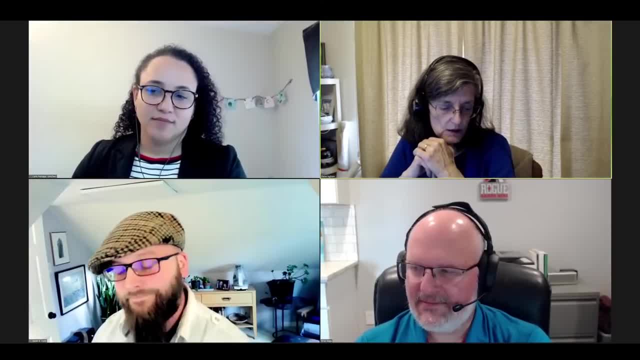 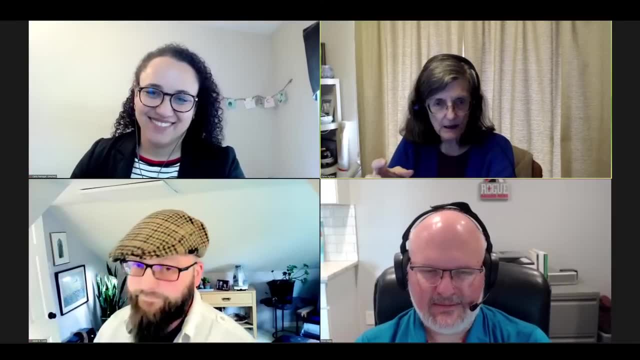 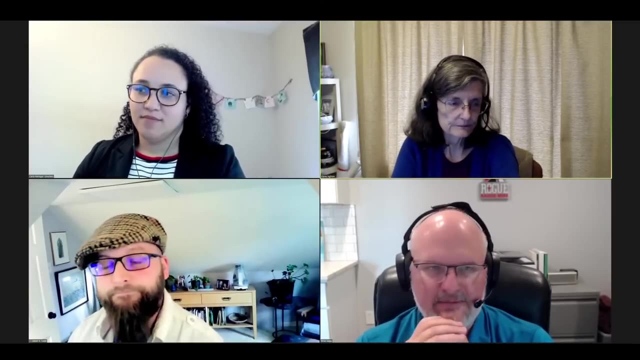 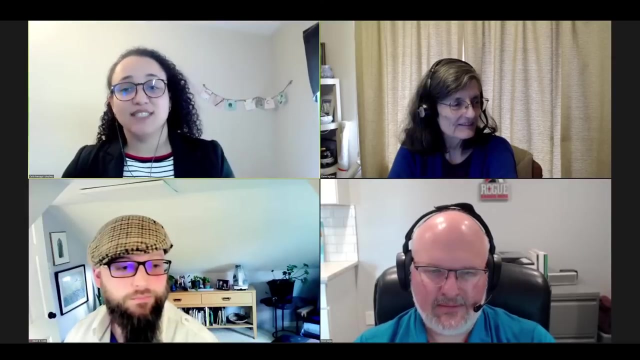 And we wanna help you to make it as painless as possible to convert from toxic chemical agriculture into non-toxic regenerative agriculture. And I just jump in little brief just to reinforce that until you decide that's your time to join our courses. 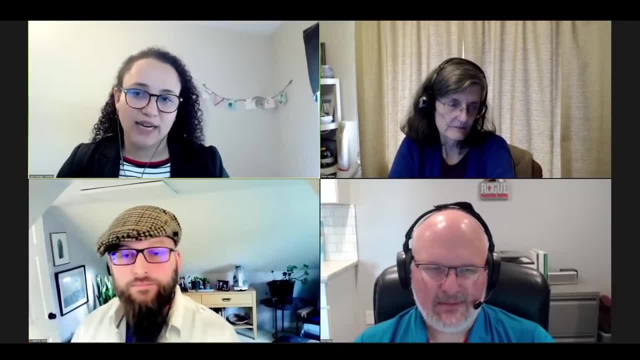 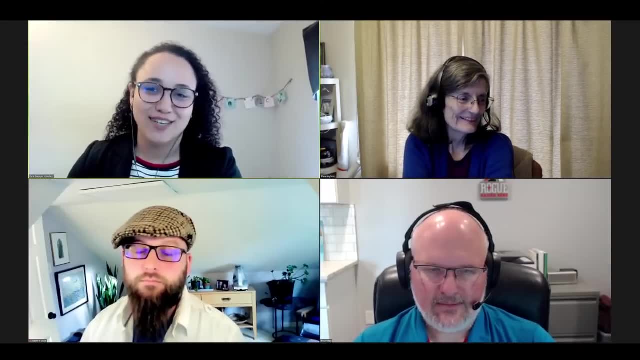 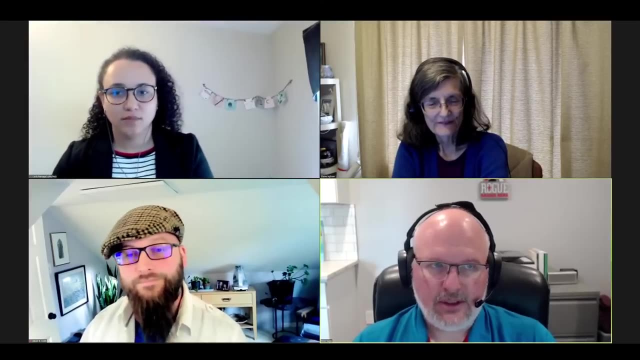 just go to our website and you can see a list of all certified labs and all consultants available that can help you understand the process until it's your time to join us in this journey. And so one thing: I was just thinking about tools that farmers can use to help analyze their soil. 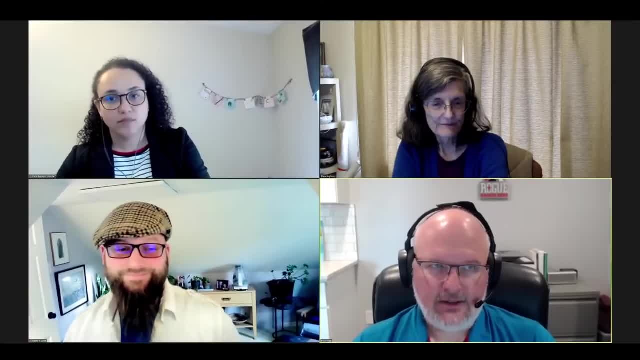 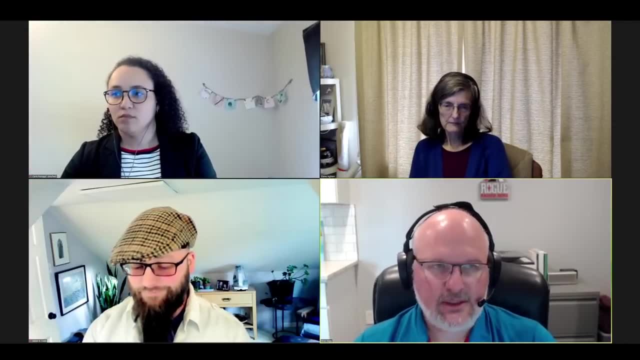 My experience working with a lot of people in agriculture is that they're very data driven. In most industries that's a very common thing, but farmers in particular. there's a lot of data inputs that they rely upon to be able to make certain decisions. 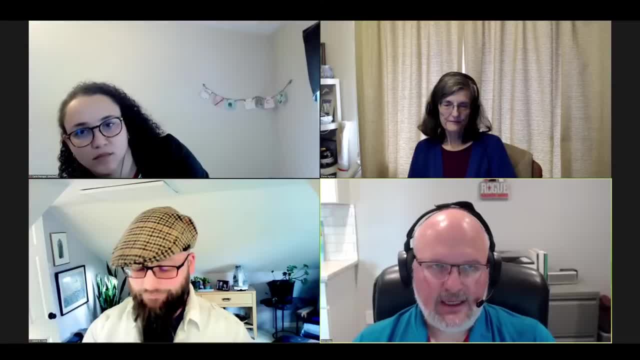 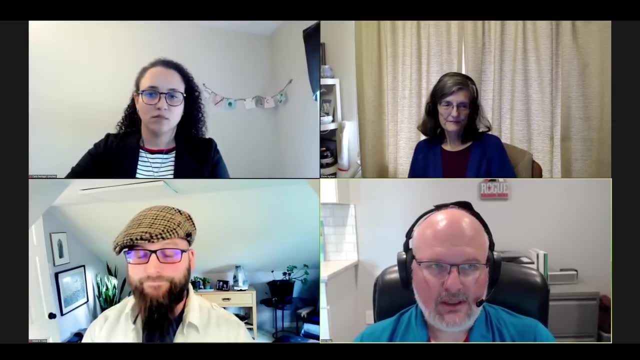 in their growing cycle, And so I actually I love the slide data that you put together around the keystone of the physical, the chemical and the microbiology, And what we really wanna do is make sure that, to fully analyze the soil, we wanna have a picture of all three. 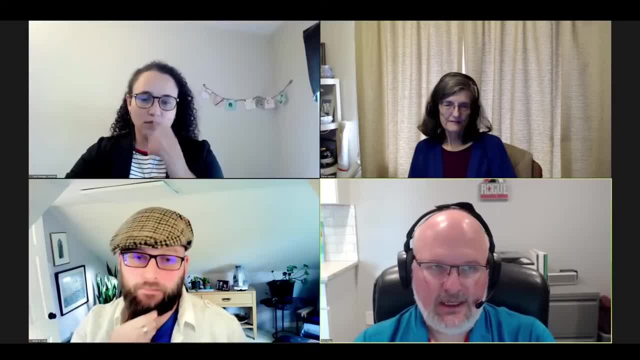 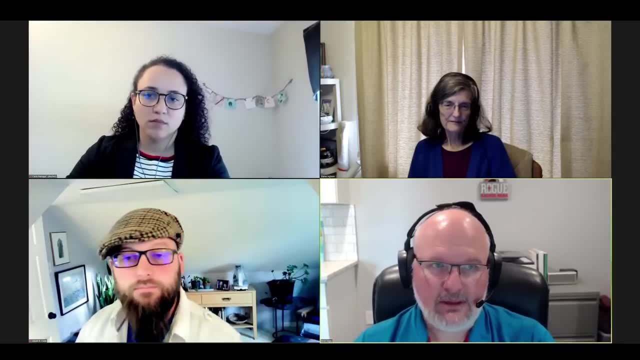 of those kind of premises. It really does start with understanding the microbiology. So either having your soil assessed so that you can get a good microbial assessment of where you're starting from is really, really important And, as Elaine mentioned, a lot of. 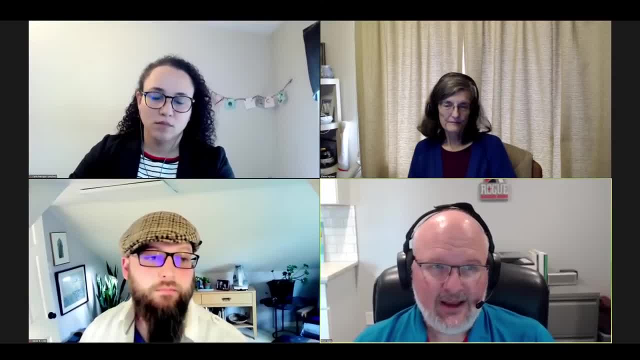 a lot of growers when they really start understanding that they're becoming microbe farmers as well as farming their other cash crops. a microscope is a very important tool. It's kind of- I use the analogy- if you were managing cattle. let's say: 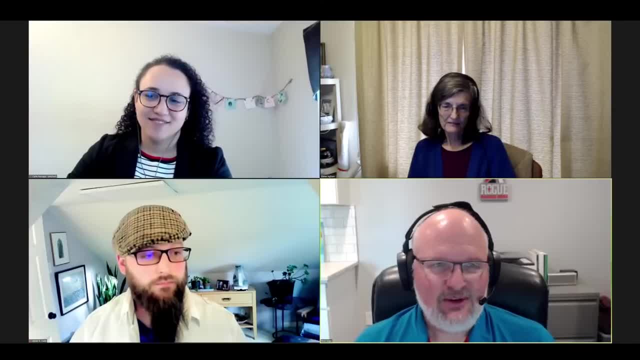 you had a thousand head of cattle, but you never saw them, you never had ability to interact with them. it'd be very, very hard to be a good rancher. in that sense, It's the same way as becoming a microbe farmer. 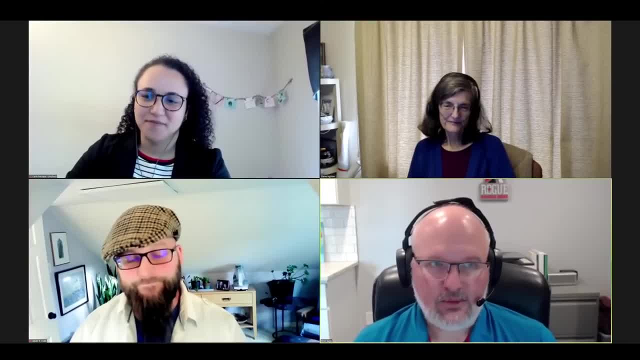 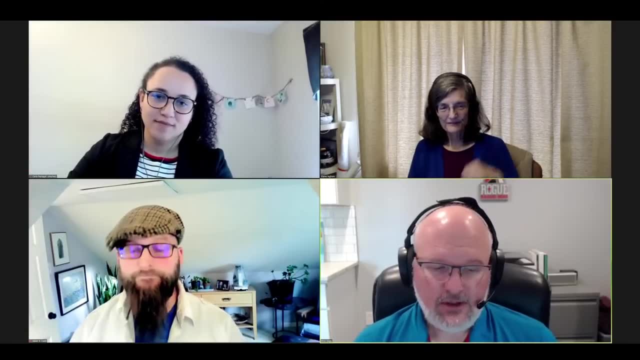 We have to have the tools to be able to observe that, And so that's one aspect of it: really getting that picture, understanding about the microbiome, but then also the physical part of it, doing like Elaine mentioned, going in and checking compaction. 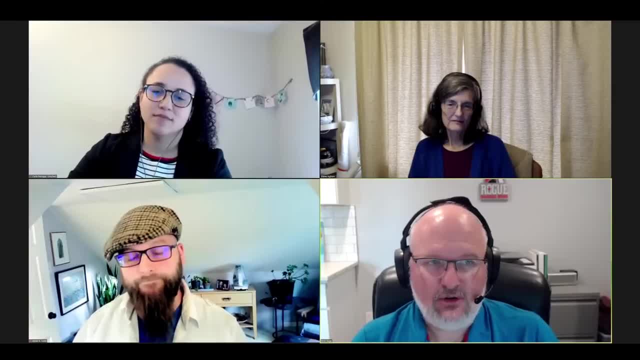 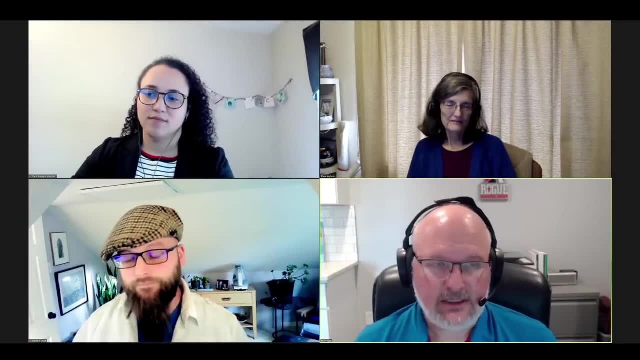 you know, using a tool like a penetrometer to go in there and map the compaction over time, Are you remediating that compaction away, Understanding the water infiltration talked about soil structure and the water holding capacity and usually deals with also aerobicness. 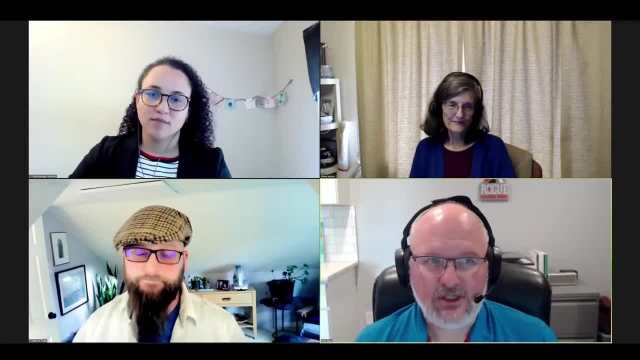 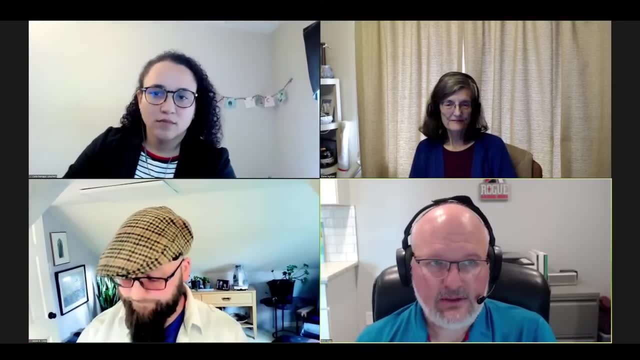 and anaerobicness of your soil. So measuring water infiltration is a very, very important tool, And a lot of farmers are ready today to do soil chemistry analysis And so understanding what the soil chemistry is as well. And then, once you have all those data points coming in, 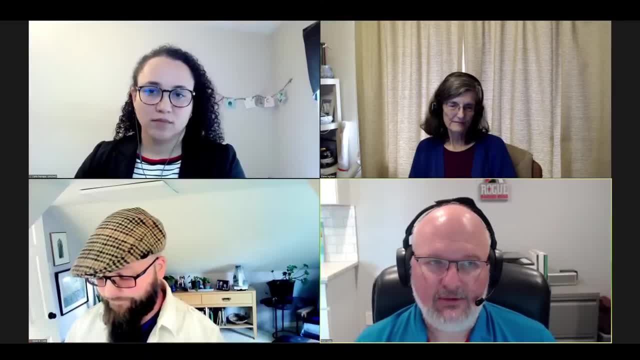 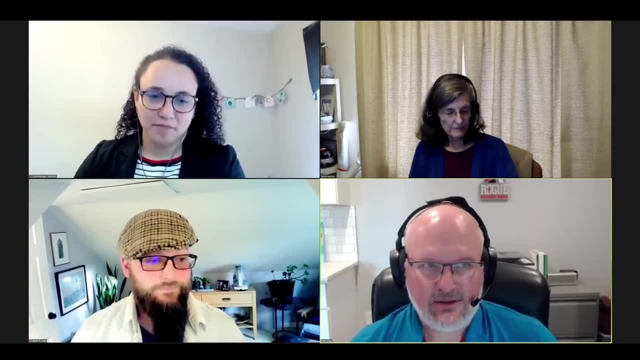 you can build a much better picture about the health of your soil. So I really encourage you, know farmers, put together a package of what you want to test, test those things over time So you can understand. yeah, the work I'm doing is really actually. 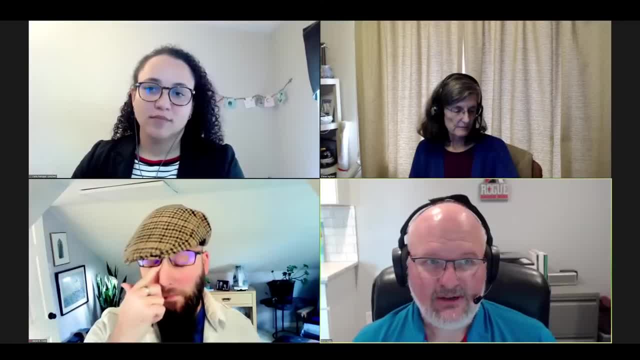 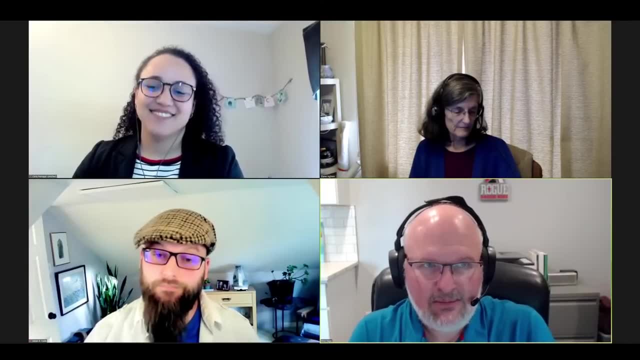 going in the direction I want it to go, And if it's not going the right direction, we have data to fall back upon. Then we have some investigatory tools We can go in and say: why was your microbial biome really growing? 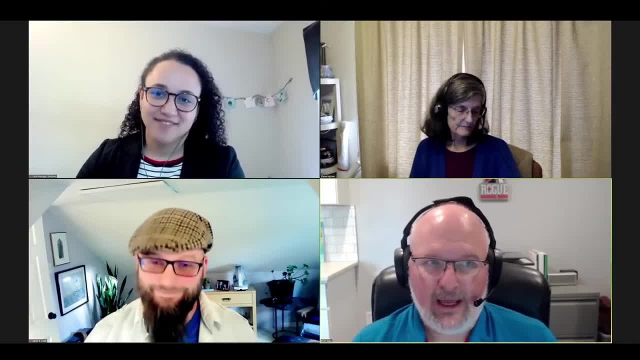 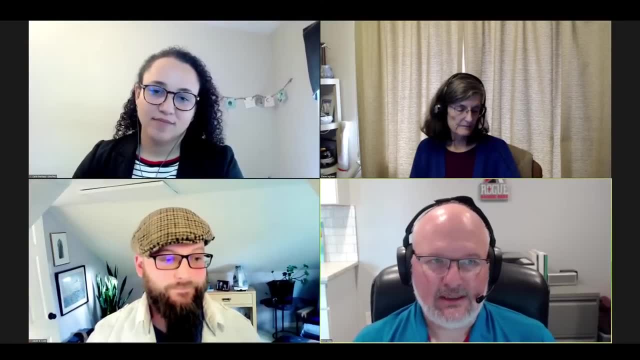 And then all of a sudden, wham, we have a major setback, What happened? And without those tools or that data, it becomes very, very hard to be able to understand those things. Yeah, it's alive and dynamic, So it changes every single second. 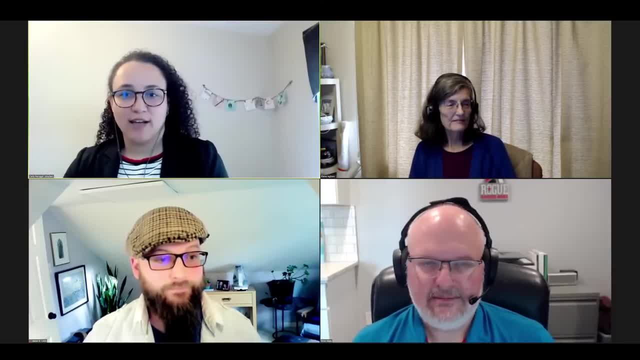 You need to see this as a big puzzle. More information you have, better decision you're gonna be able to take. So don't lose track of all these great things, right? So don't lose track of all these great things, right. 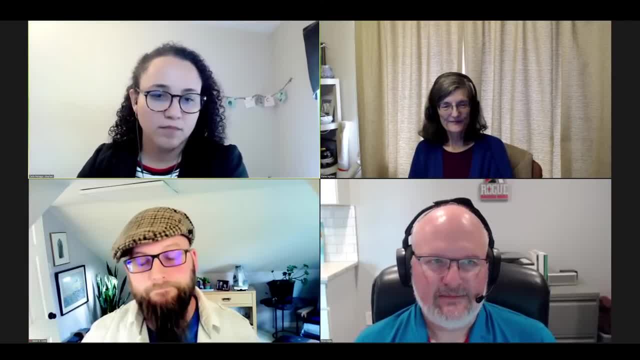 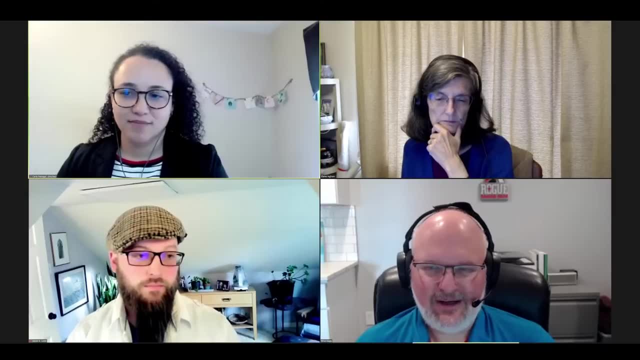 So don't lose track of all these great things. right, And that's the information that we have available For sure, Adam, anything else you wanna add before we move on to the next question? Elaine, good, I'm good, All right. next question. This one's from Phil, And Phil says: are there any disadvantages from mulching a vegetable garden, perennial beds and fruit trees with hot compost? I think we'll have to. probably was it compost that went through a thermophilic cycle, or is the compost hot right now? 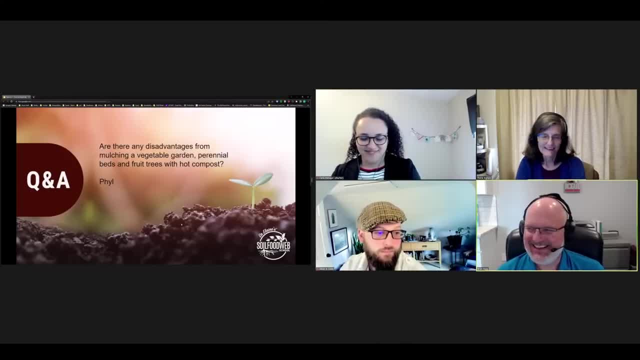 So we'll have to tackle both those parts of the question. So we'll have to tackle both those parts of the question. Exactly, if it's, your compost right now is 170 degrees. Exactly, if it's your compost right now is 170 degrees. 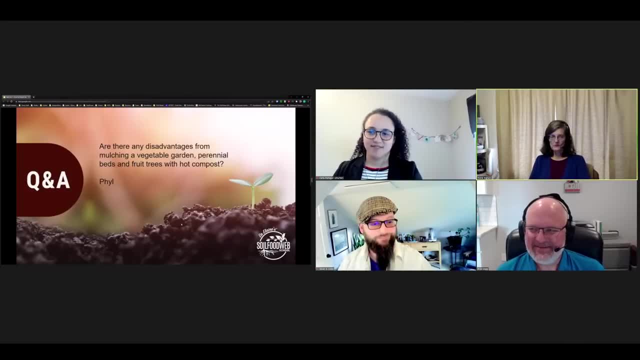 and you mix that, where it's 100% of your bed is that hot compost. you're just gonna kill a whole bunch of things. So let the composting process finish. let it get down below 131.. Then, when you mix that, 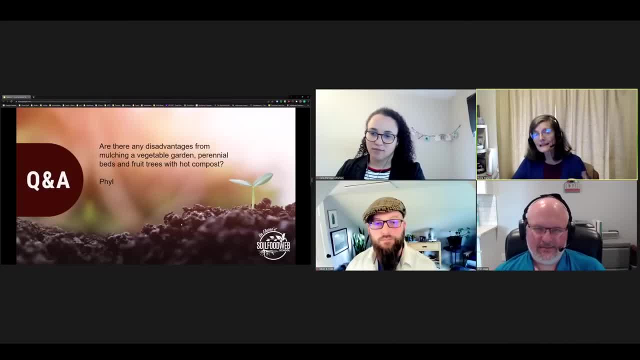 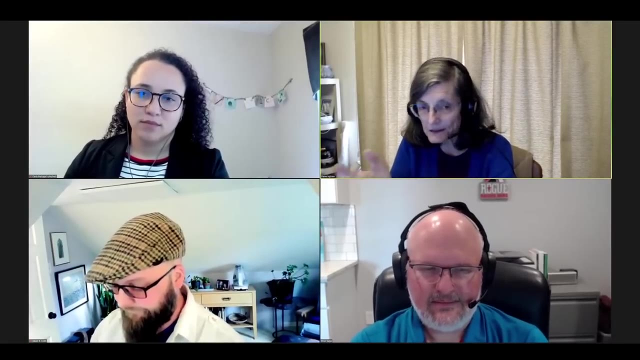 something that's at a temperature of 131, mix it into the soil that's present, So you've got a 20% of your hot compost up at a temperature of 100 degrees, or something mixed in with 90% of your site soil. I can guarantee that it's gonna be pretty much the temperature of the site soil, So you don't have to worry about burning the roots of your plants. You can just make a little small pot of hot compost made using the thermophilic process. 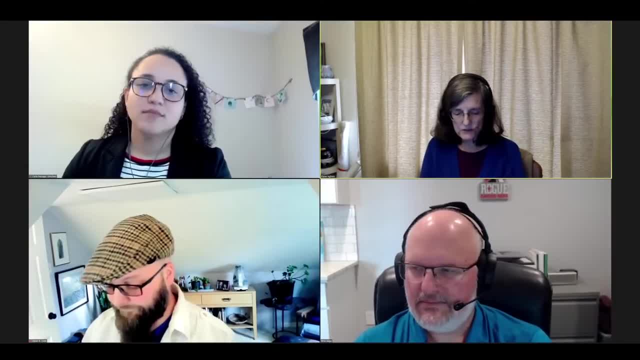 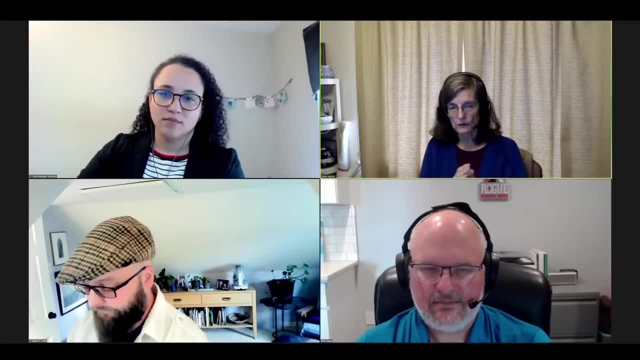 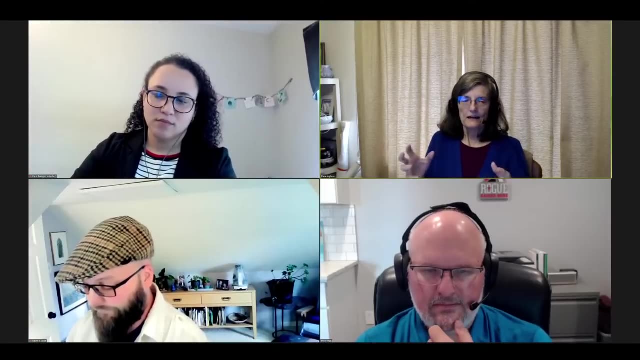 Again, go back to the. what equipment do you have? What is your lifestyle? Which kind of composting are you gonna choose? And most of the time in our world where you have limited time to do things and you've gotta kind of take a 10 day period of time, 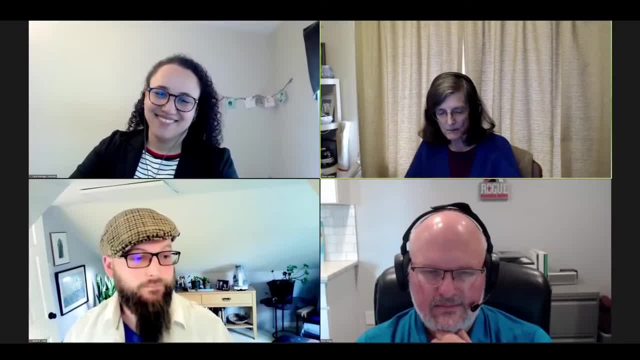 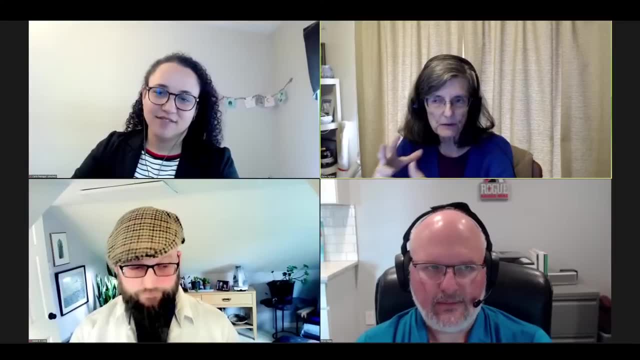 So you'll be home every day to do things. So you'll be home every day to do things. So you'll be home every day to do things, do that composting and check up on it. um, you're going to choose a thermal, um, thermal approach. 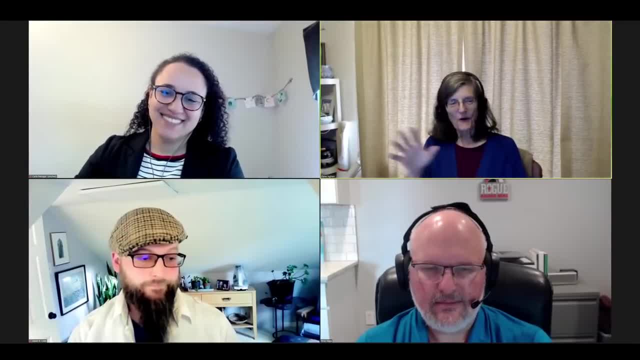 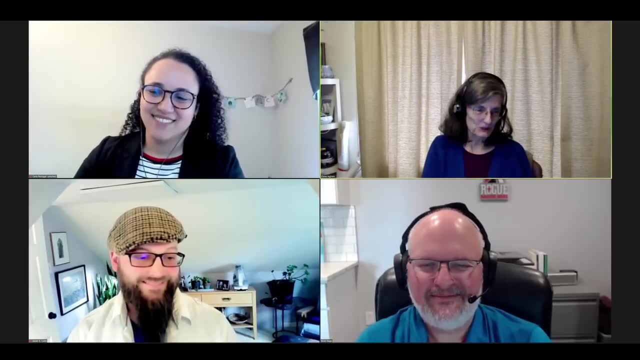 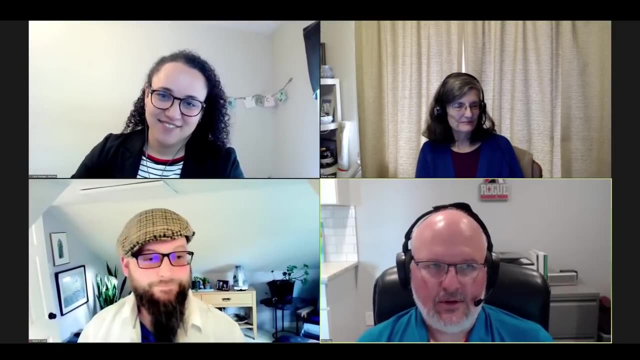 unless- okay, there are, you go off on all of. i can go off on all of these things that will enter into your decisions, so i will leave that up to you at this point. yeah, i just mentioned you know it's very common for us to use uh compost as a mulch or integrate. 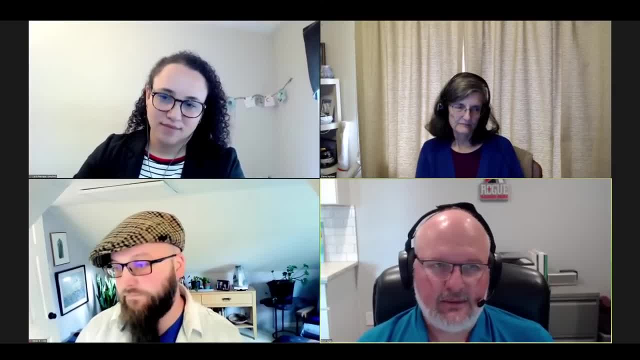 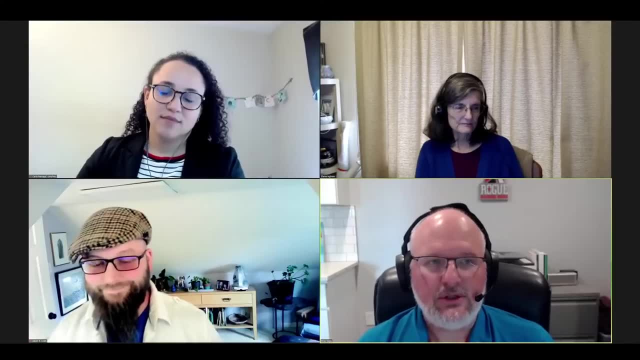 it into the soil. you know, when i'm making my potting mixes for my starts and so forth, i'll add a certain percentage of my good thermophilic compost and, um, you know whatever soil i'm going to use, uh for that potting mix. and there's times when i'm planting trees or vines, things like. 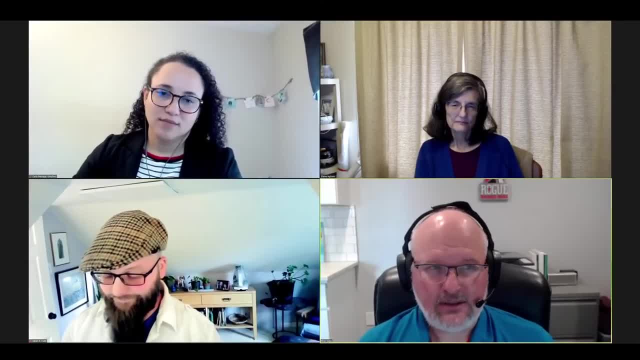 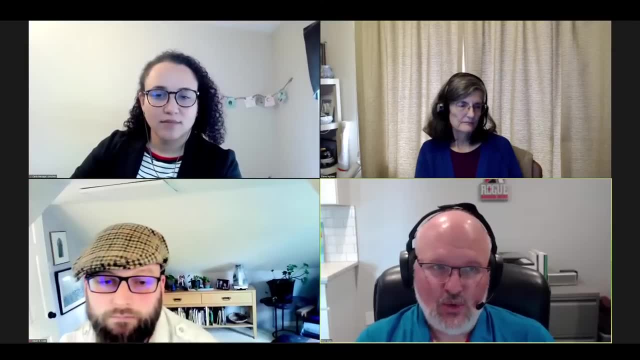 that i'll incorporate in the soil and then also do a top dress with that material as well. so it's very, very common for us. i mean really, compost is our tool to really inoculate the soil profile and also the soil profile, and then also the soil profile, and then also the soil profile, and 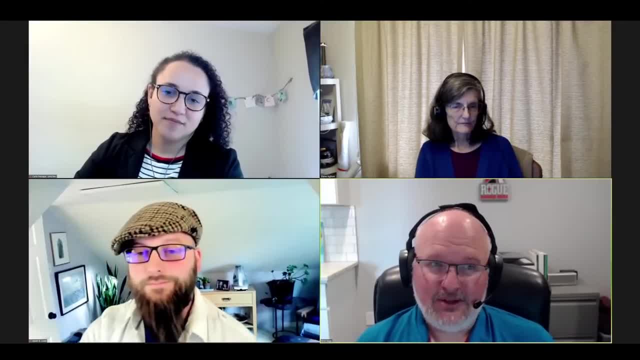 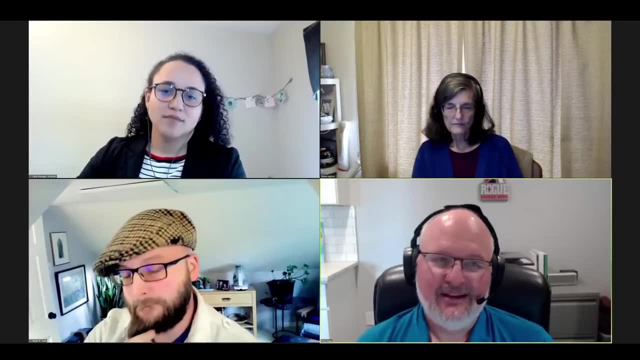 the surfaces of the plants. And, as Elaine was kind of talking about also, we got to make sure it's good, thermophilic or good compost. Does that be thermophilic? Is good? biologically complete compost is the key, key thing. Just thermophilic compost is one of the techniques that we tend to. 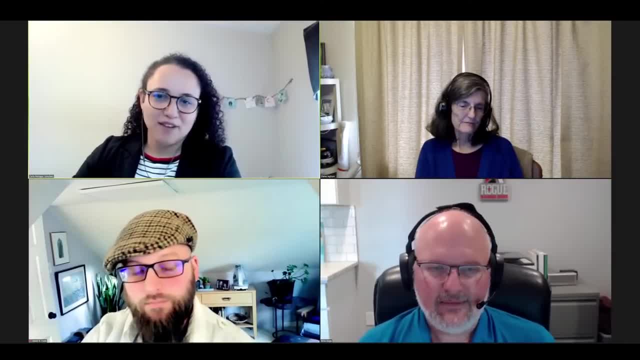 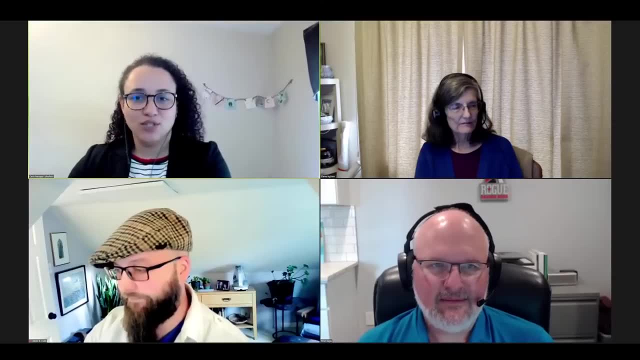 employ quite a bit And on this realm we need microscope work again. right, It's the only way to check if you have all the biology you need. We're going to help you to find the best time to use your compost, based on the crop that you're working with. And getting back to the mulch, 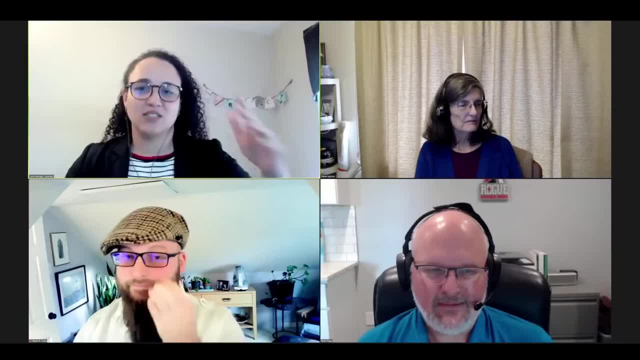 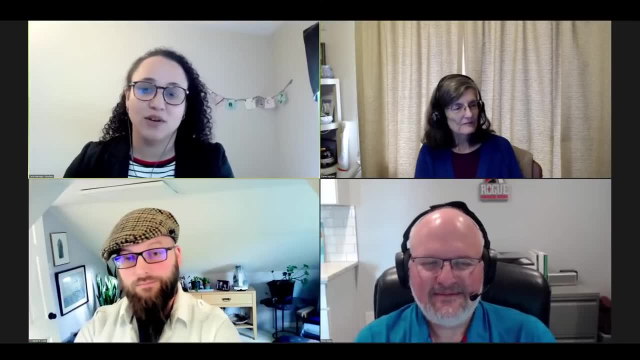 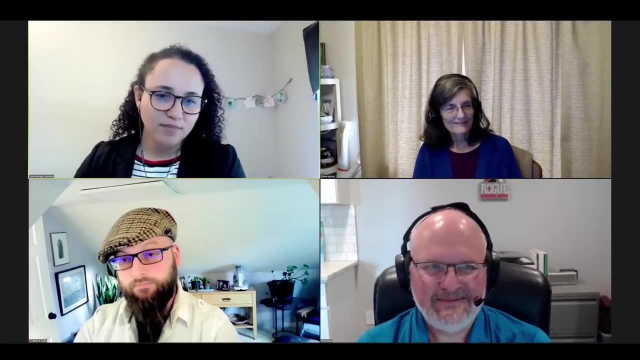 another good option as well is after you do your extracts and teas. that residue is a nice way to use as a mulch as well. So there is a variety of actions we can do to optimize our soil. Got it, Adam. anything else you want to add before we move on to the next question? 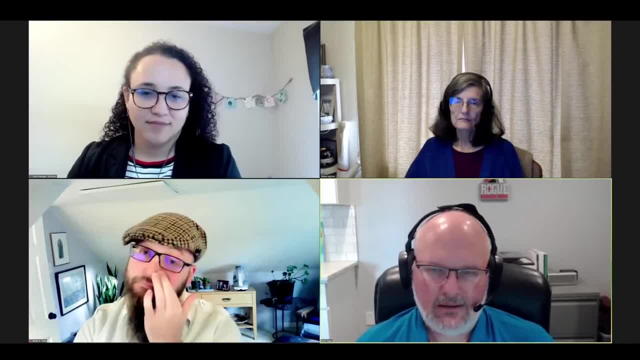 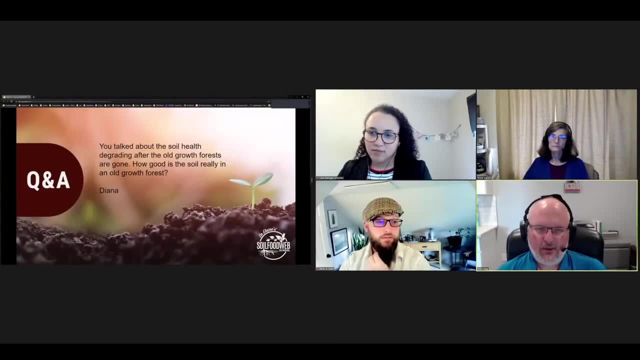 All right, Let me go ahead and share here. This question is from Diana And the question is: you talked about the soil health degrading after the old growth forests are gone. How good is the soil really in an old growth forest? I've lost the 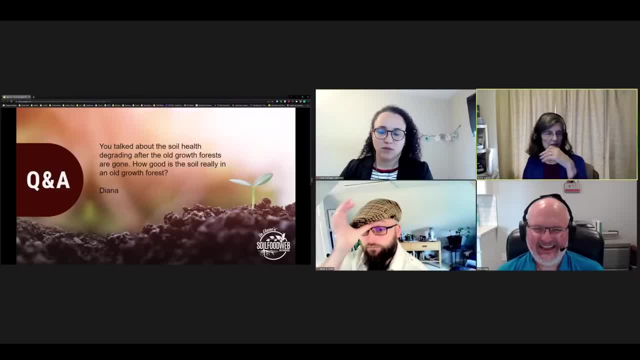 Can we read it again? Elaine, I lost the. My computer is doing something strange. I don't know why. Elaine, I can start this one because it's something that I said. Yeah, go ahead, Thank you. So it's again this thing where there's not a single measurement or answer about soil health. 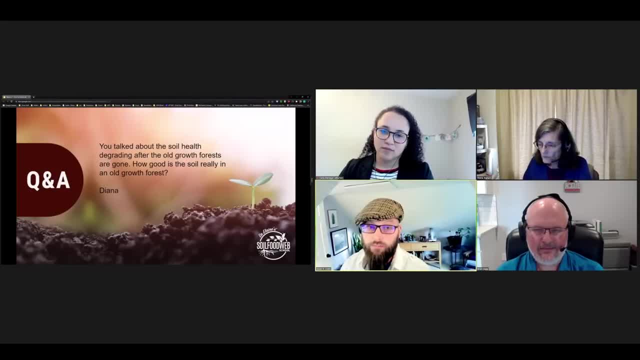 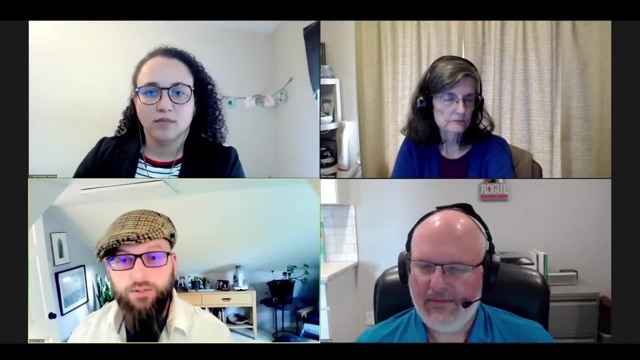 Old growth forests, especially in the northern parts of the world, tend to be very dominated by fungal biomass, which tends to make them very stable. Now we get into Some unhealth in forest ecosystems, sometimes because of how they're managed, And I wasn't. 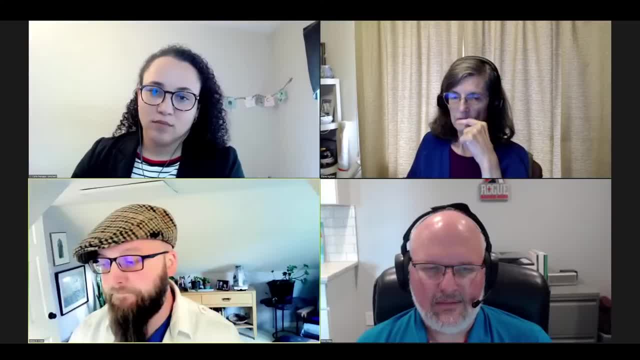 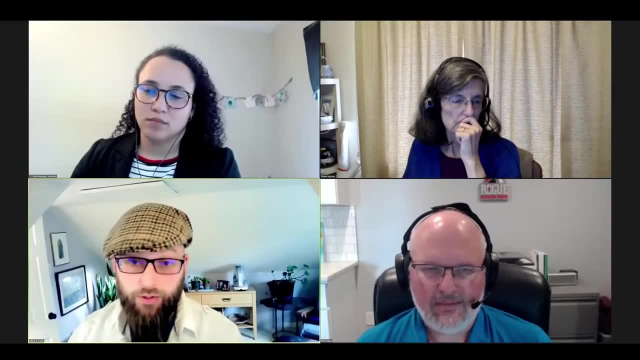 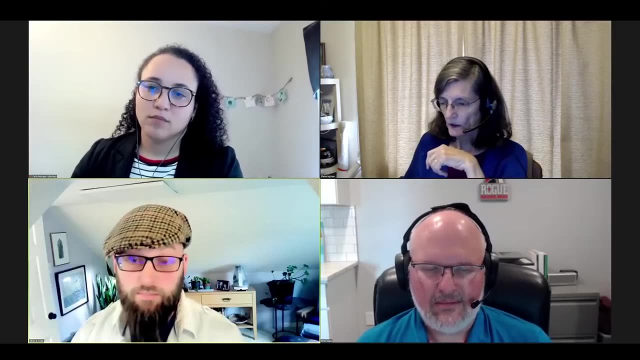 necessarily talking about like a monoculture, like forestry forests where they're all pines or something, because I think there's a lot of disruption of the soil in those systems. There's heavy equipment, There's often high fertilization, There's some use of herbicides in many of those. 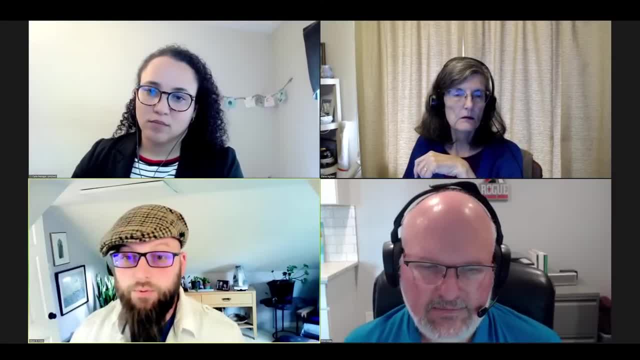 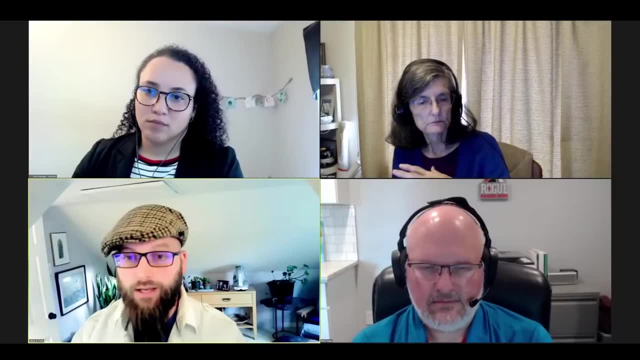 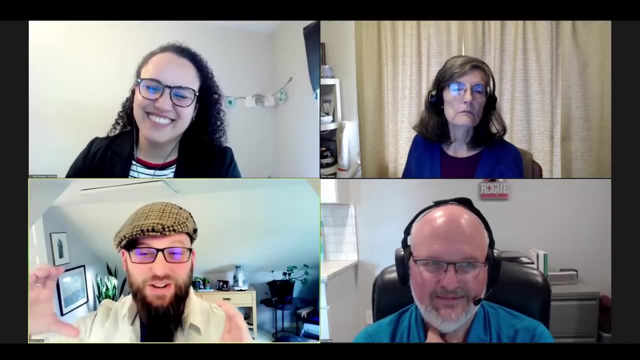 systems, But I'm thinking more of those really biodegradable systems, And I think there's a lot of that need to be changed, Because the soil is an extremely diverse forest, especially in tropical settings where you might say, like within a football field, you know, or soccer, football, soccer fields, a mountain space. 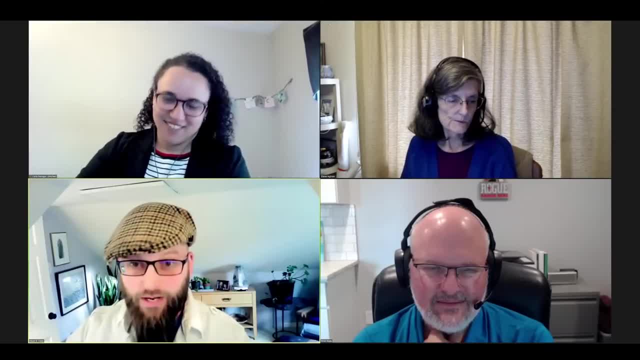 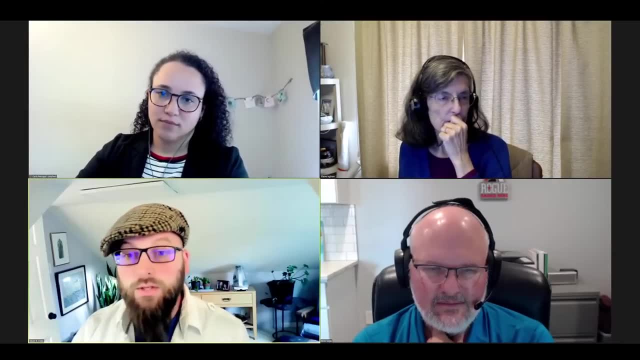 you have like hundreds of species in there, Right, And if you slash and burn that, of course it's going to be a huge disruption to the soil health, And what we see is that, in many of these cases too, there's significant slope in the environment, And so it's going to be a huge disruption. 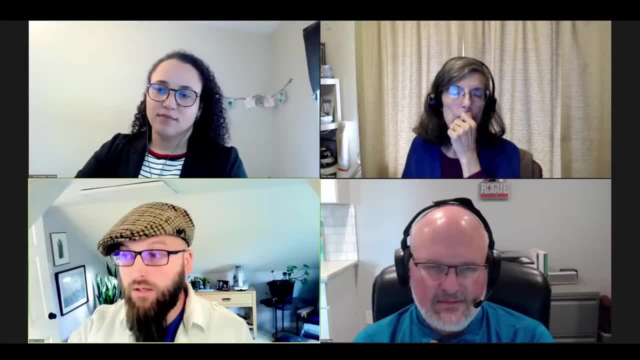 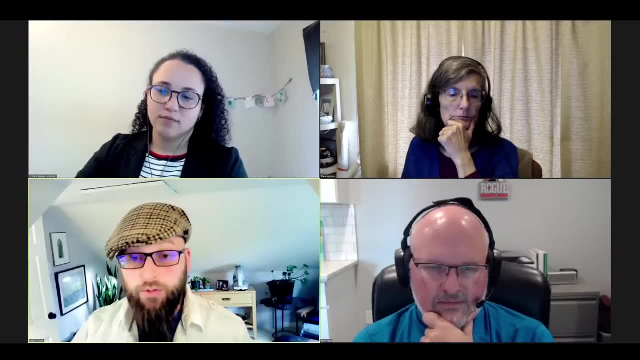 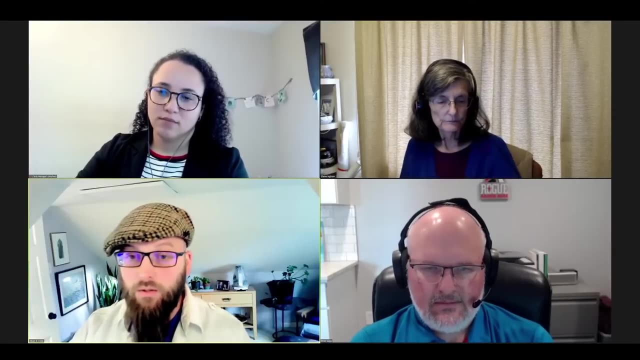 situations and so if you cut down the trees or whatever the plants and try to cultivate that, you get massive erosion pretty quickly, especially the forest systems that maybe have a large litter layer. that acts like a protection as well against wind or rain causing a lot of movement. 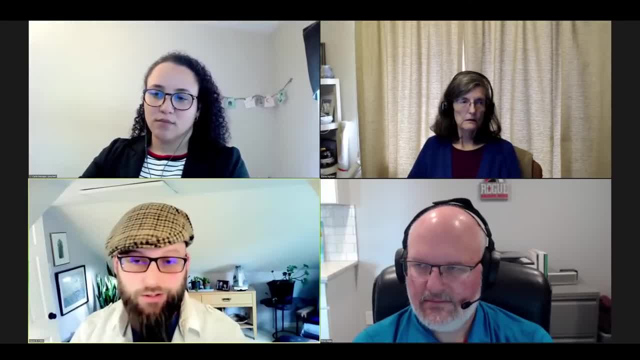 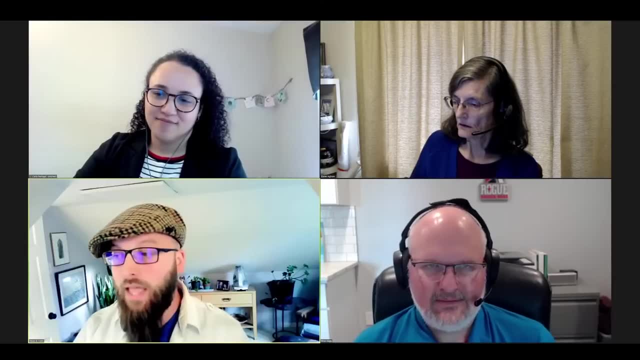 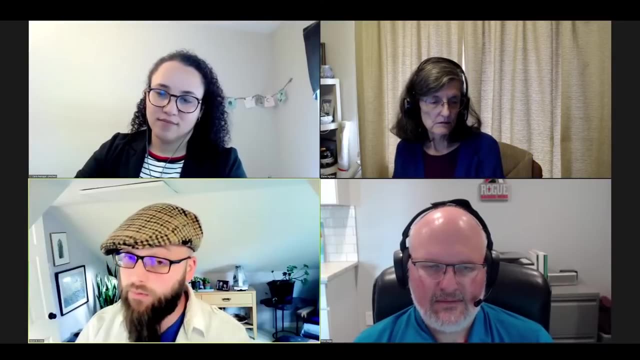 of soil. so i mean it's the classic ecology thing to say it depends, right. but in general i think of forest systems as having some of the strongest stability of soils around the planet and that doesn't mean i mean if you go to some places they might have very low like nutrition in their 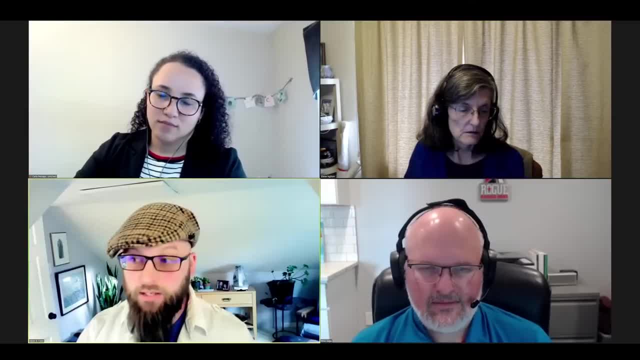 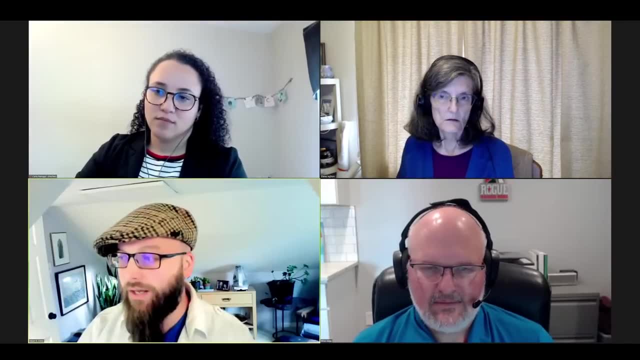 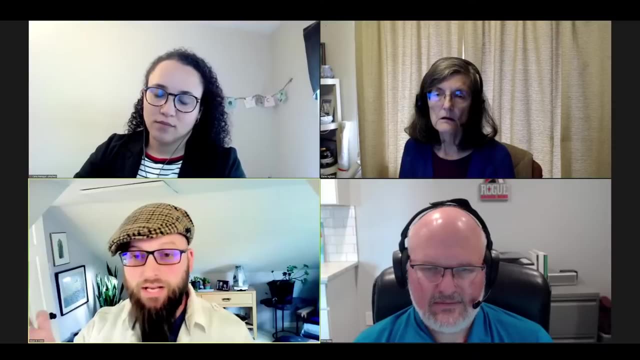 soils because of, like the parent material that's there and and or you know some other common disturbance that that happens naturally in that system. um, i, i'm trying to think of the actual name of it, but there's a. there's these two islands in indonesia and it's pretty amazing because you go to one and the soil is very low nutrient, like everything on. 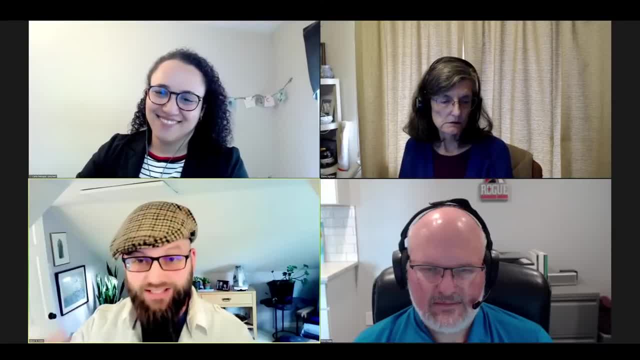 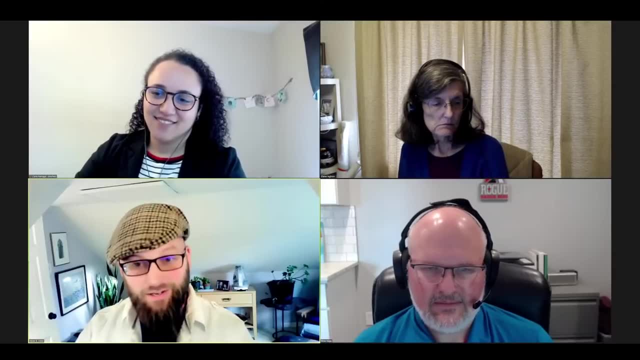 the island is very toxic and poisonous because it's trying to keep a hold of the nutrients, like all the plants are really aggressively like: don't eat me because i can't spare any nutrients. and then near that is a different island which gets constant resupply of nutrients and everything is. 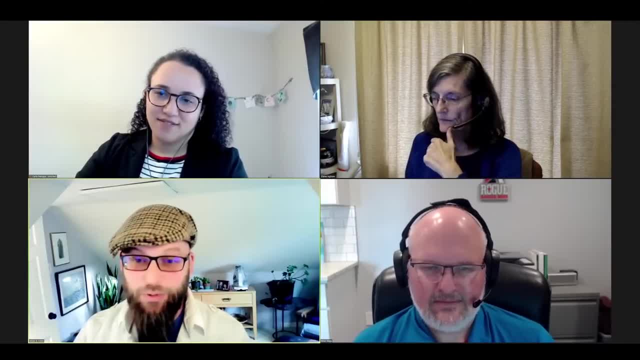 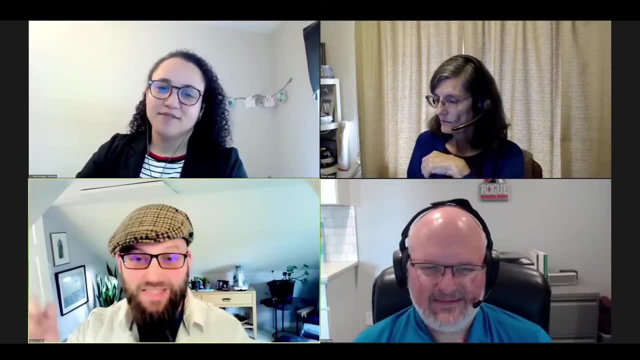 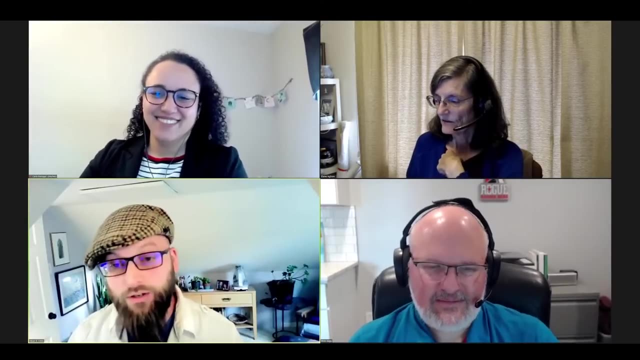 so abundant and and uh and relaxed. and even the monkey populations are different. they're like on the island with the low nutrients, and they just sit around and cuddle all day on the island with a lot of nutrients. so you know, you can see this variation in the world. it's part of nature. 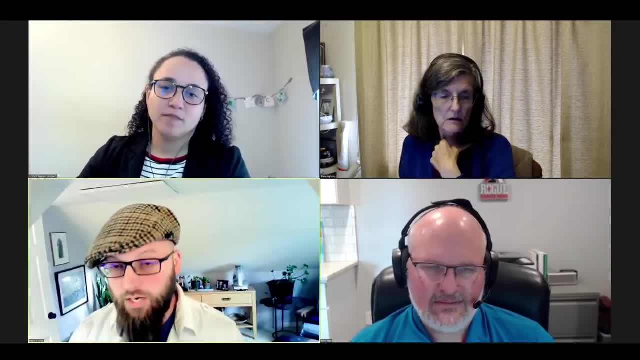 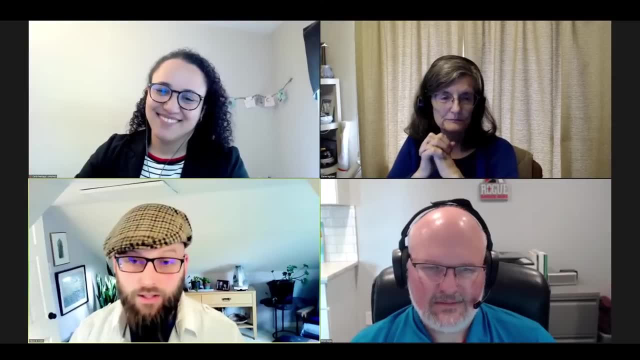 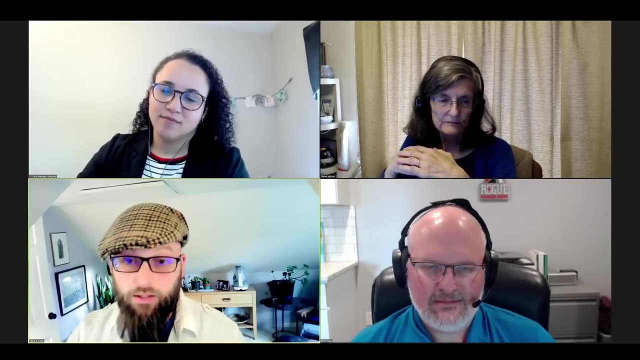 to just have these, these broad differences. but generally, deforestation- i don't quote me on this statistic, but i conceptualize of deforestation as maybe being about a third of the problem with soil loss in the world today and a lot of the problem is that the problem is that. the problem is that the 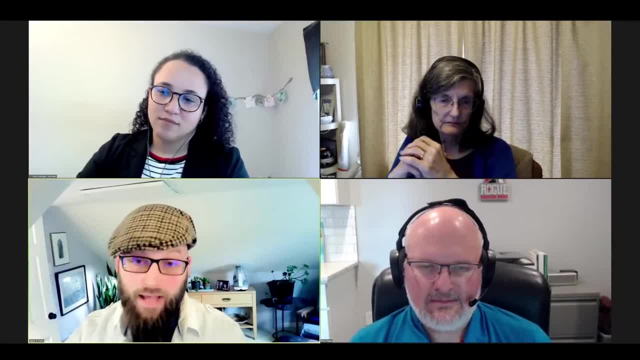 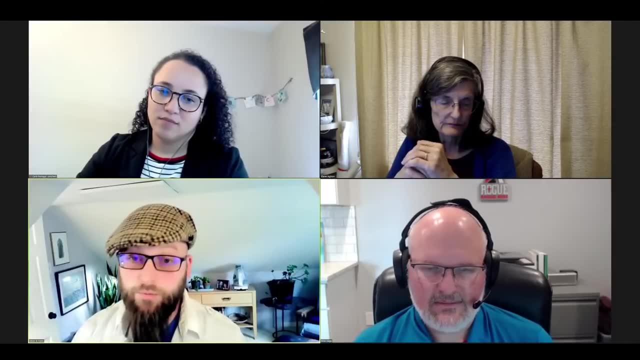 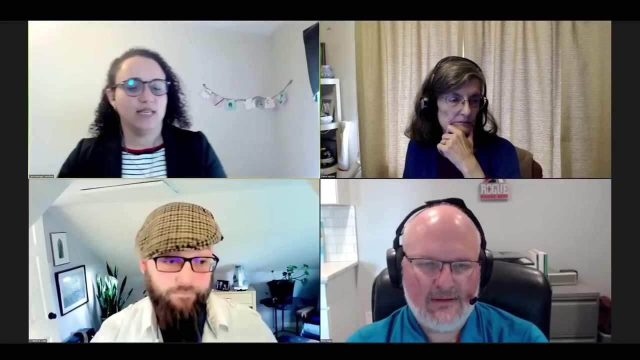 deforestation is to try to create land for row crop agriculture or cattle or something else, which can often be a very inappropriate plants or animals for that system to support. yeah, if i can jump in, it's something that i see happening a lot in tropical areas. the deforestation is advancing. 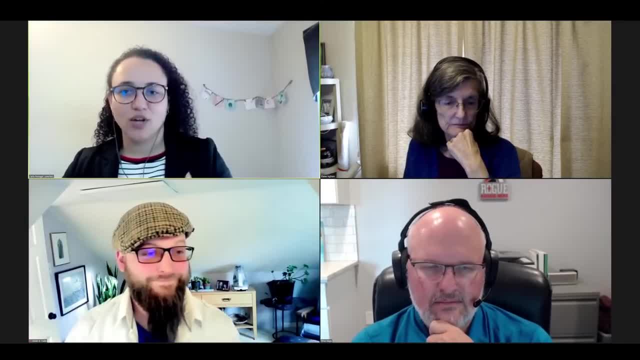 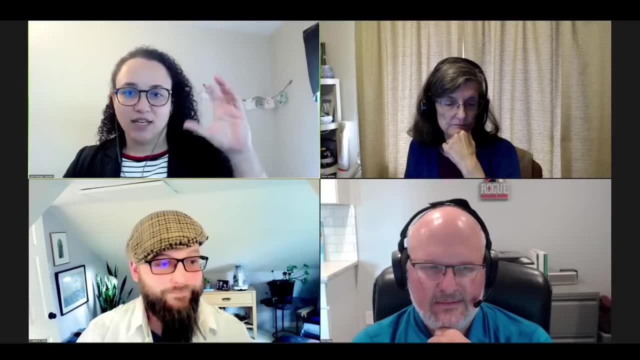 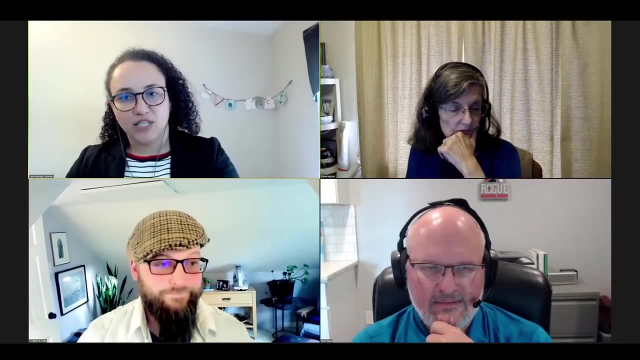 because they're using so intensively the soil to grow crops on the industrial agricultural land. so they're using so intensively the soil to grow crops on the industrial agricultural land. so there is no nutrient right. so it's time to move on. so this is where the regenerative agriculture 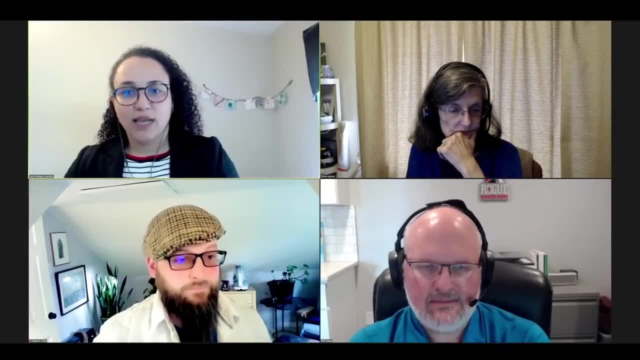 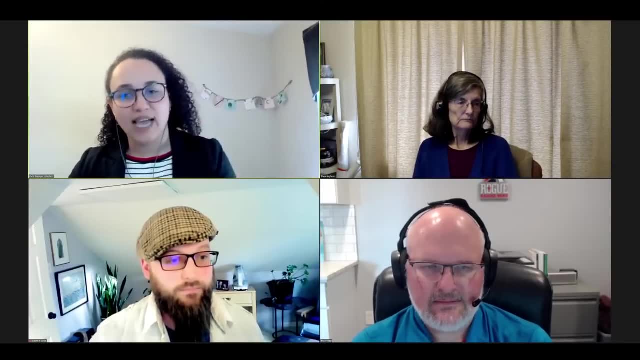 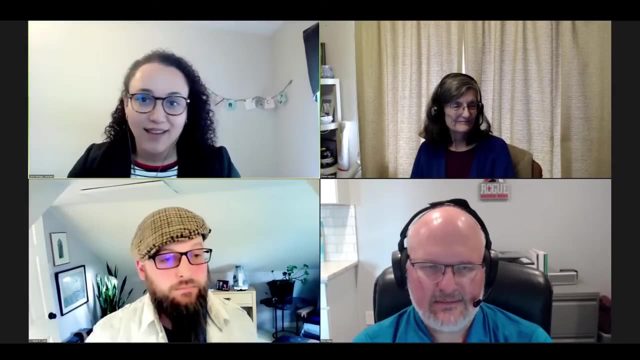 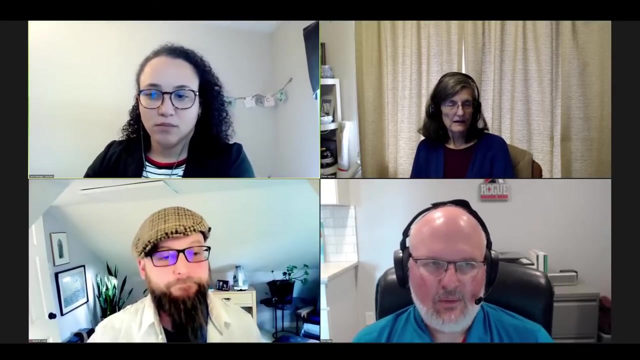 has a very, very important role because we can help stop this deforestation movement as well. right, if you can restore the soil, restore all the nutrients, cycling in the areas that are red, not in this original condition anymore, we can increase the yields without having to put down more in forested areas. you know one way. i also look at the question that came from. 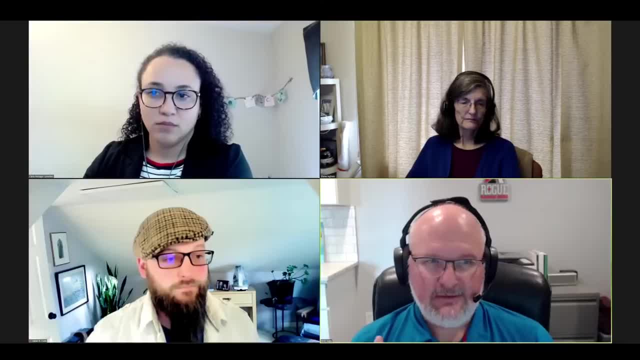 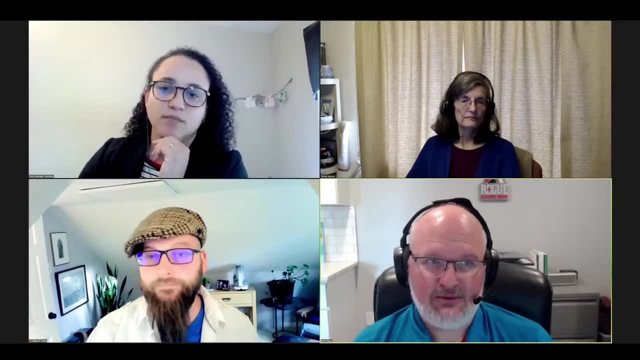 the attendee is that it's all about perspective too. so when you're talking about an old growth forest, the microbiome is going to be probably set very well for the plants that are thriving in an old growth forest, which can be tend to be, like adam saying, very fungally dominant. but if you're going to want to plant, you know row crops or you know brassicas early, more early in the year, and then you're going to want to plant those types of plants, then you're going to want to plant those types of plants, then you're going to want to plant those types of plants. 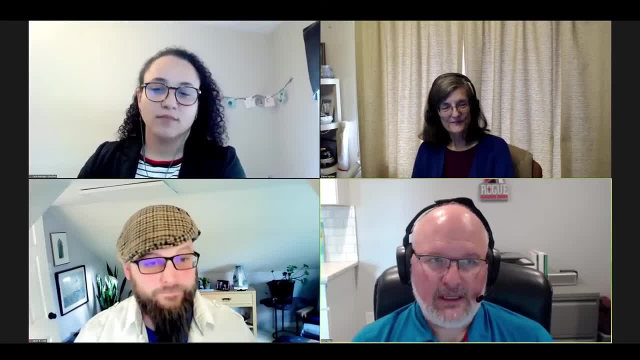 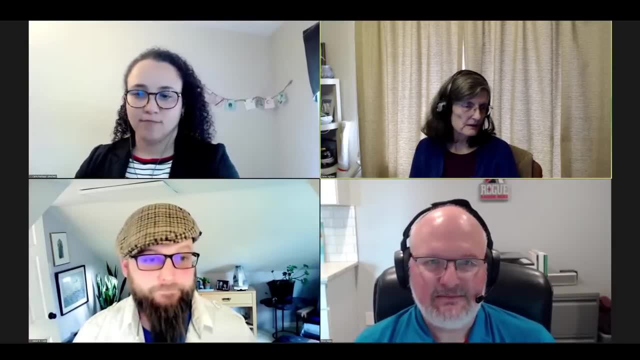 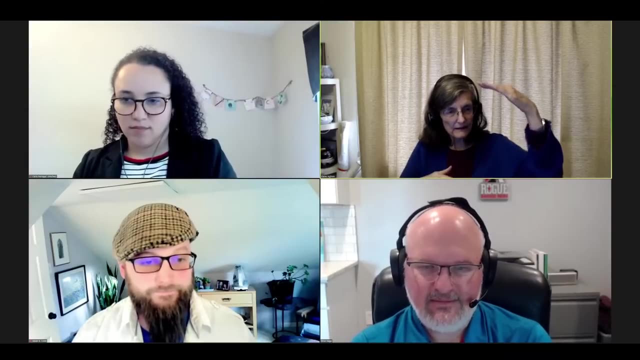 and so it's a matter of perspective, of understanding what are the plants you're trying to grow, and it doesn't have the appropriate microbiome for those types of plants. yeah, and that's really what you need to understand is, uh, that an old growth forest soil is not the proper balance of the bacteria and the fungi in that soil. it's balanced for trees, for. 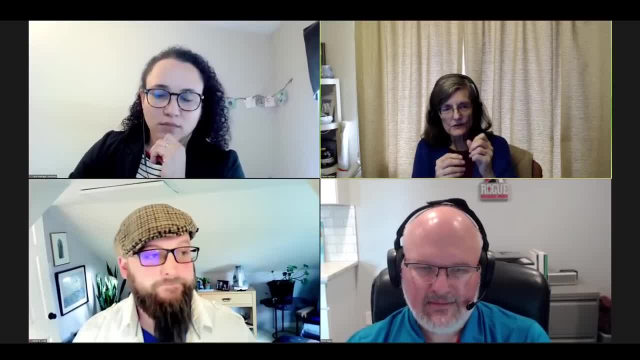 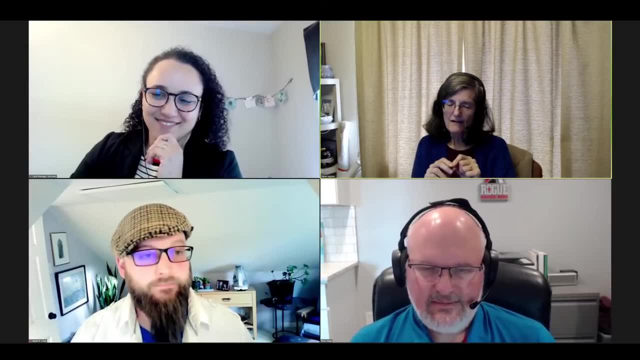 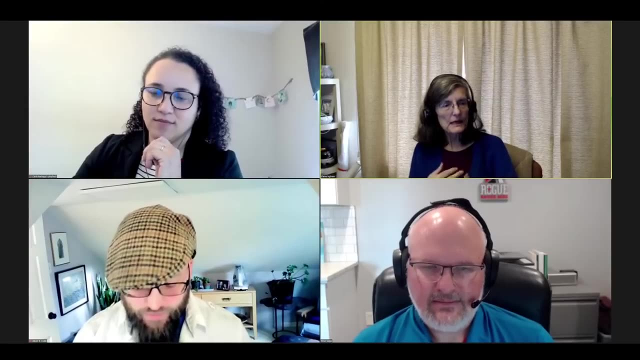 old growth forests, for example. so you could take a very small amount of that forest floor, a pinch, you know, like a a quarter of a gram or something, and you inoculate your compost pile with that material and you would potentially be able to grow some really good old growth fungi. you're 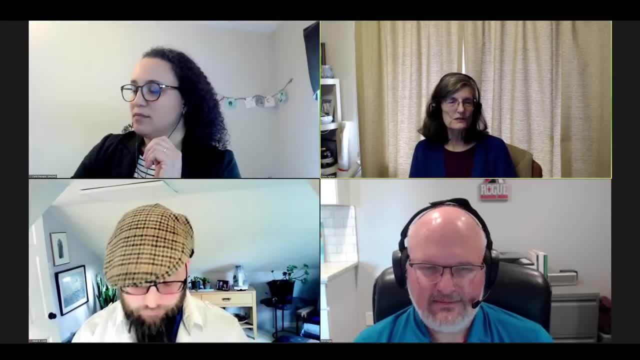 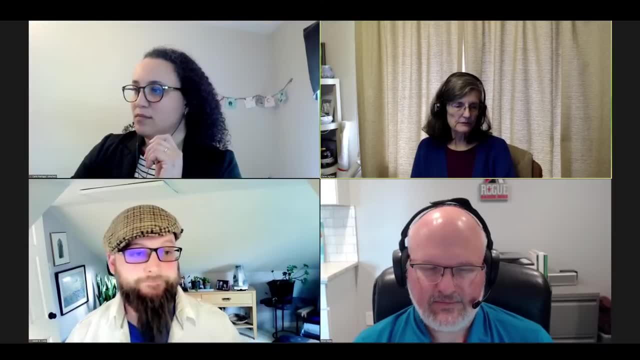 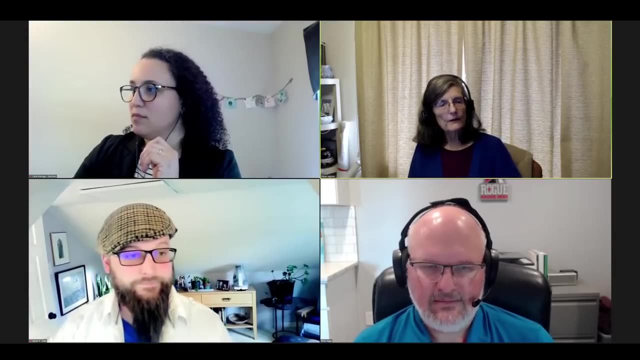 not going to be able to grow at all because the conditions are so different. so, um, building up your compost piles to have all of the diversity of microorganisms. that's what that composting process is all about: is getting the biome for your area, for the crops you want to grow. 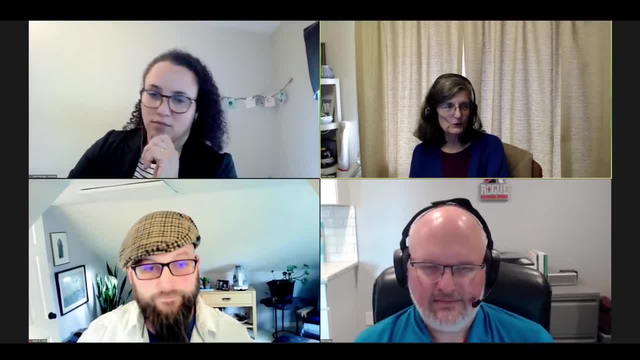 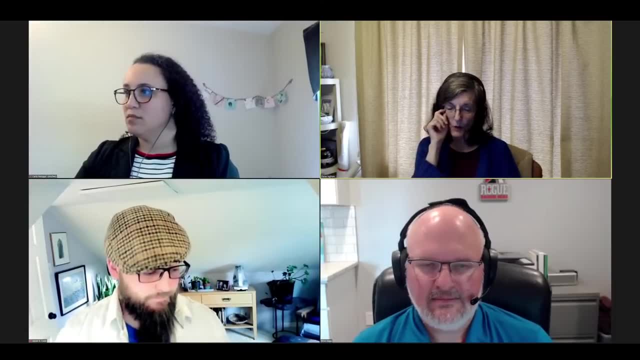 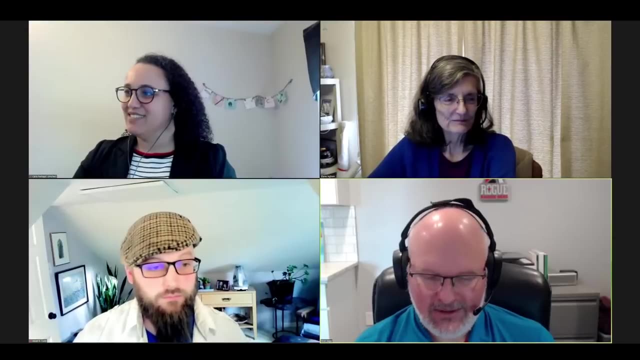 and that's why it's so important to get get that microscope so you can use that microscope to see if you have the organisms, what's missing in your soil. so i can go on and on. well, i just have one thing i just want to add to your point there. elaine was. 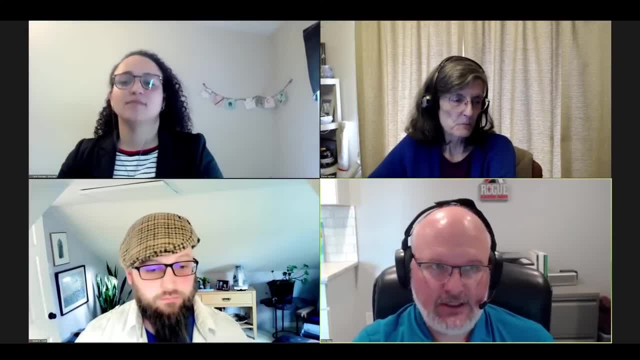 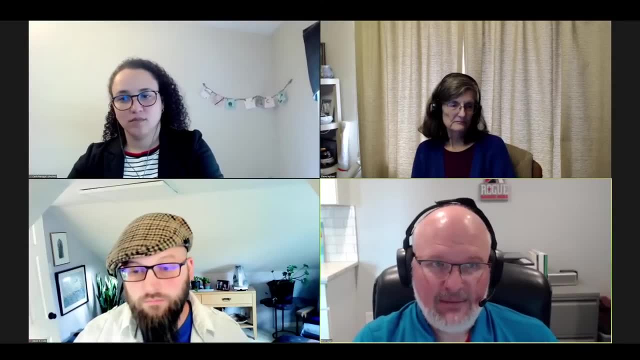 a lot of people get focused in on the biomass of bacteria and fungi, and which is great, that's. that's one major aspect to you know, uh, the compost and the quality of it, but the other is the diversity. i mean, if you, you have massive amounts of biomass, but what if it's pretty much just a? 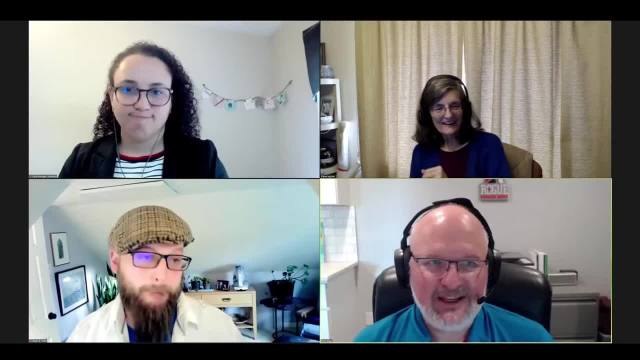 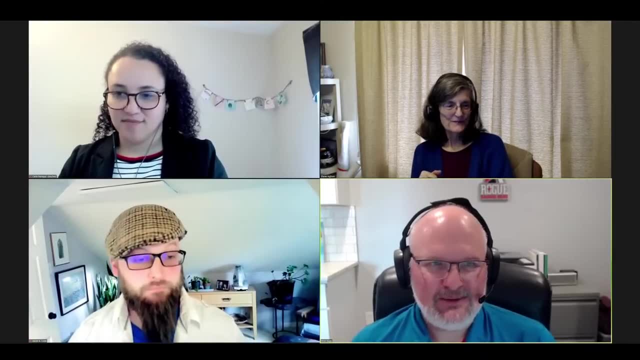 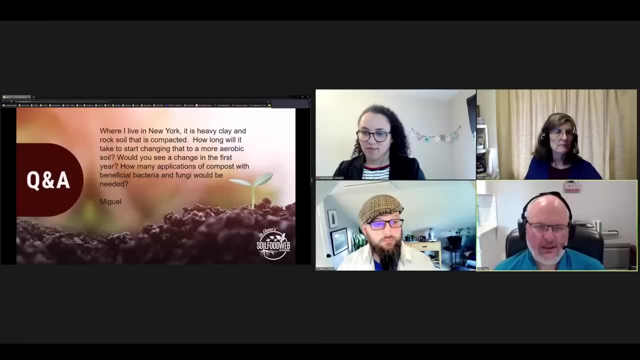 couple species of fungi. uh, am i gonna get the nutrients like i'm looking for? probably not. okay, anything else panelists you want to add before we move on to the next question? right, okay. next question is from miguel, and miguel asks where i live in new york. it is heavy clay. and rock soil that's compacted. how long will it take to start changing that to a more aerobic soil? would you see a change in the first year? how many applications of compost with beneficial bacteria and fungi would be needed typically when we're dealing with something like this? 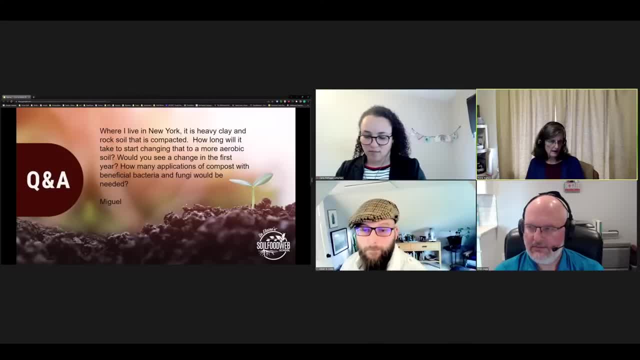 we've got to see how heavy that clay actually is and how compacted is it. so it's gonna determine how we're going to apply the organisms to your soil to be able to get those organisms down into the top, you know, three to four feet in that first growing season each year. you'll then see the microorganisms. 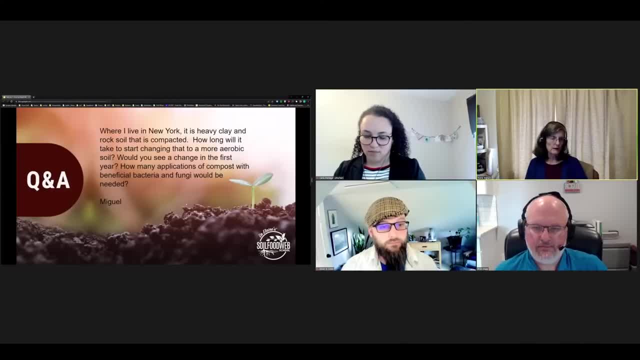 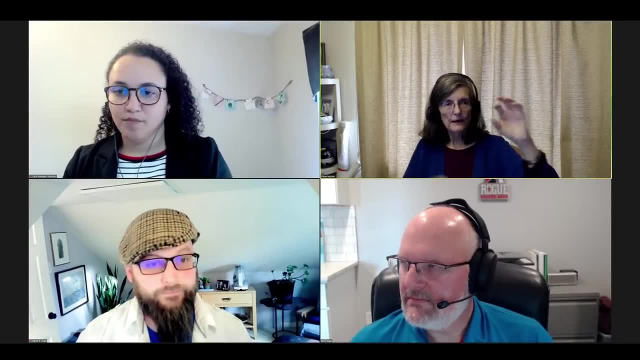 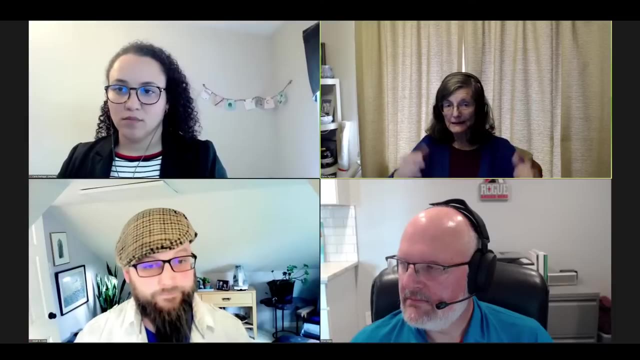 chewing away at building structure deeper and deeper and deeper, because all of our plants, they do not grow on the surface of the soil. they're supposed to be moving downward into the soil following water that has been collected and held, if you've got the right structure built by. the bacteria, fungi, protozoa, and i know it's micro arthropods, earthworms, on and on. so if you've got that ability, the roots are gonna to build the structure, go down every year. you have less and less problem with drought because your root systems are going to be able. to reach, though, that water stored in the soil, doing exactly what it, mother nature, said it to do: get this biology back into the soil. have the water be held so the root systems grow down this whole silliness about your. your roots hit the compaction layer and go sideways. that's not normal. whether or not that's normal, that is a six soil. so get that metal rod, find out how far down that compaction is and then start to do the work to break that open. and if you follow directions, we can typically get that depth of the soil, get your roots growing down, sometimes as deep as 10 to 15 feet. um people. 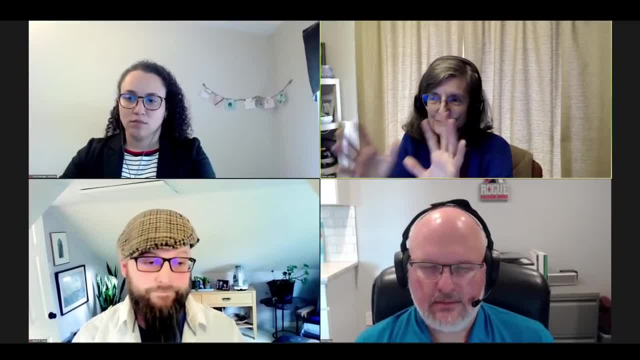 get your roots growing down, sometimes as deep as 10 to 15 feet. um, people just don't understand that. um people just don't understand that roots isn't they're supposed to be growing low. they shouldn't have roots growing bad movements. um, roots isn't they're supposed to be growing low. they shouldn't have roots growing bad movements. gets estimated by the habits in the soil. the soil's growing more as the earth is growing. another soil that definLY abseiling and also �ämänote2. so it will be ok. that's why I said um, thinking it's a key device. that's because it. supposed to go down that far? how far down can your trees put their root systems? well, if you're growing some old growth- cedar or hemlock, or- you can have the root systems going down 350 feet. if you're growing cherry trees, you can have a root system that goes down 100, 150 feet, and so 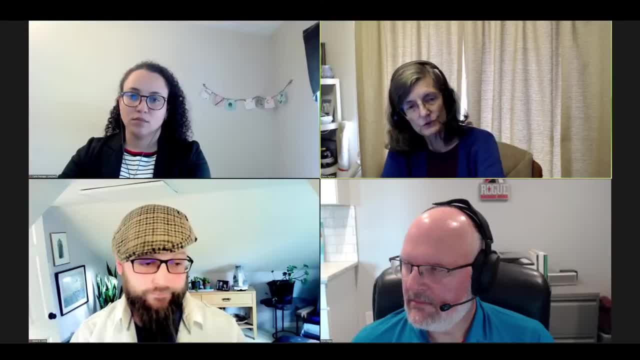 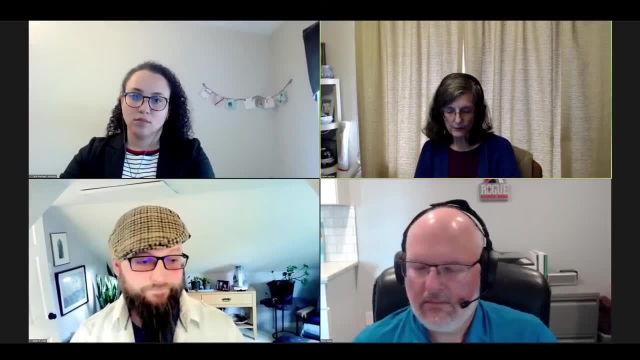 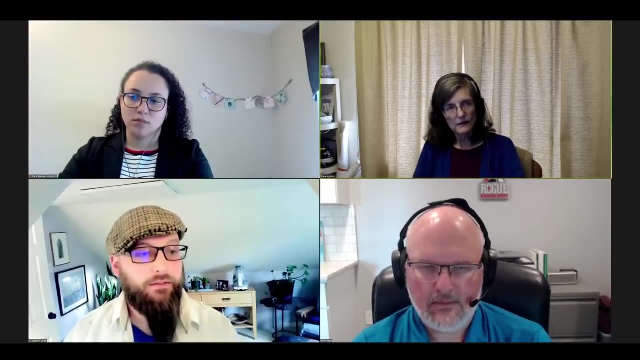 you don't have drought bothering you, but you do have to build that structure. you've got to start getting that biology into the soil. so typically we're going out with a pre-application before you put down anything else. we're going to get the compost in there. are you going to apply it? for the last time ever you're going to till that soil and break up the compaction that's in the top four feet or three feet, whatever the equipment is that you've got to do that job. we then want to make certain we put in drenches whenever we detect that. you're going to have a root system that goes down 300 feet and so you can have a root system. the biology and the soil around the root systems of your plant is not in the proper balance for your plant. so is it an early successional grass that you're growing? is it different kinds of? 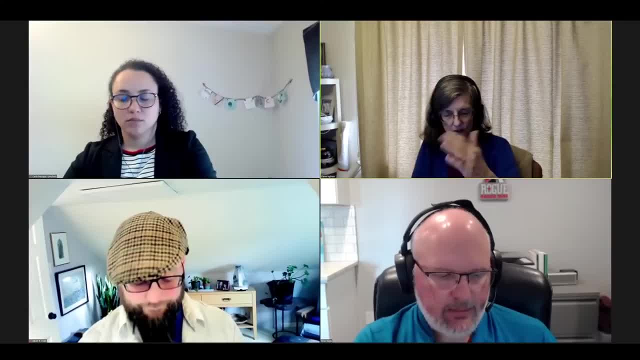 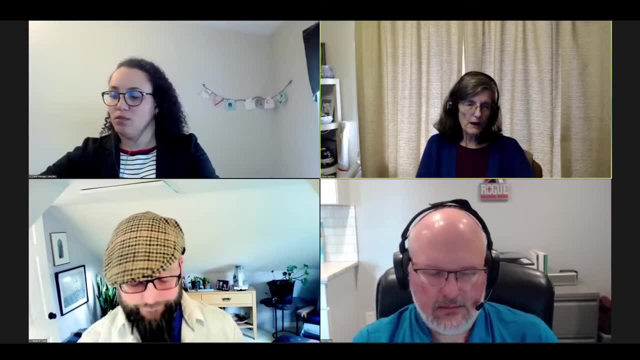 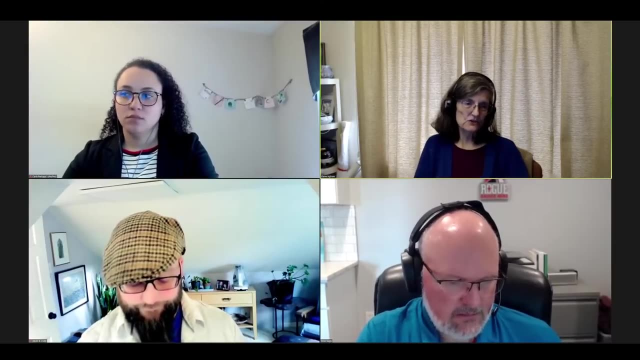 brassica coal kale crops, you'll have a different ratio of fungi bacteria. as you grow in perennial grasses, you need a different food web it. when we go through succession and explain how that works, you'll see that it's really easy to understand how these things, how different plants, require different 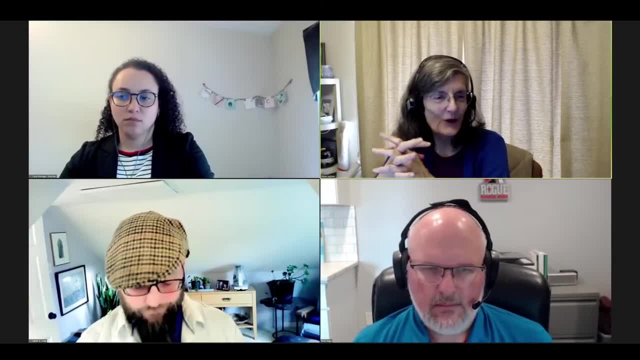 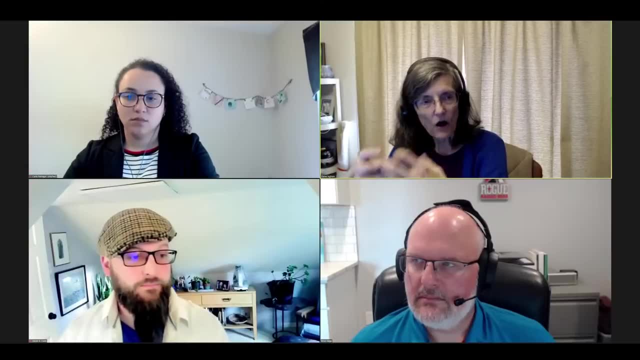 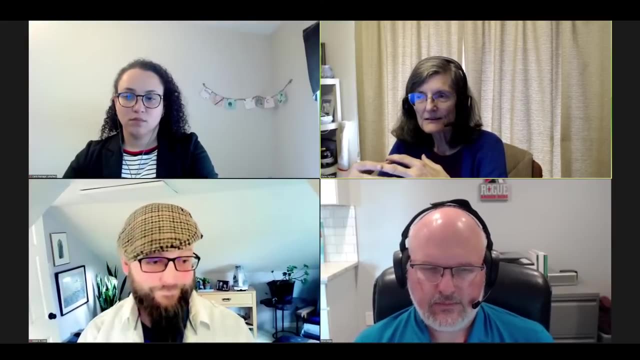 kinds of organisms in their root system to be able to grow and give you maximum productivity. make certain that that plant is got all its defenses ready. your immune response by your plant requires that that plant has all the nutrients that it needs. if the plant doesn't have the nutrients, 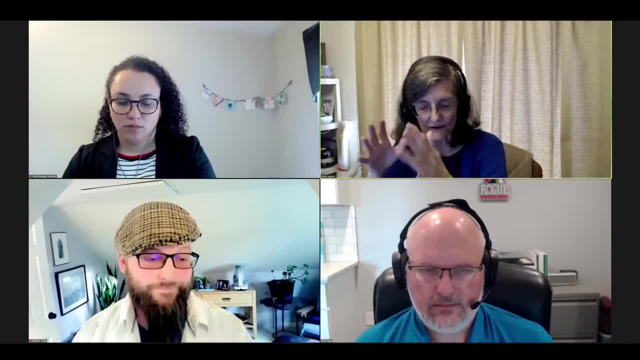 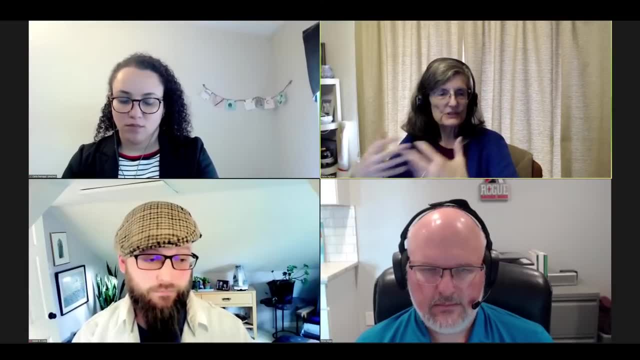 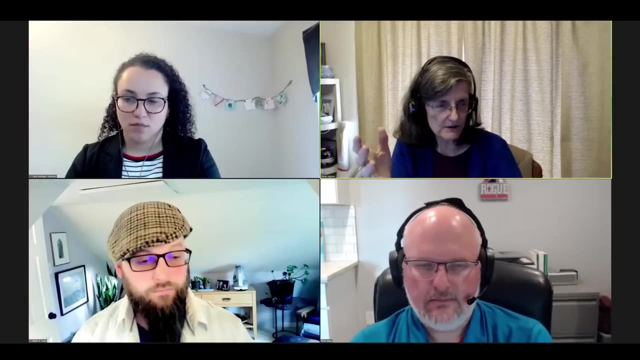 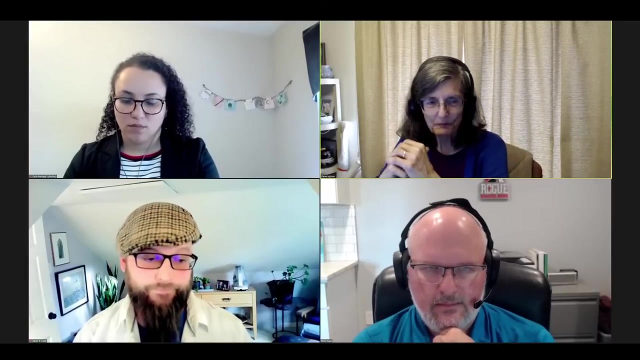 they're not balanced well inside the inside of the tree or the crop, you can't have the resistance develop to any of the diseases or pests, because the plant's still too stressed to be able to deal with any more stress. it's just like you, after you know, passing all your midterms and 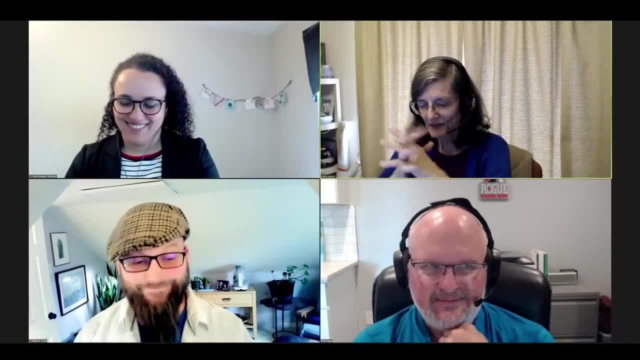 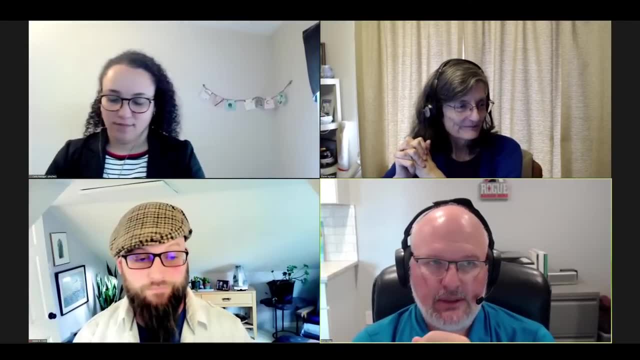 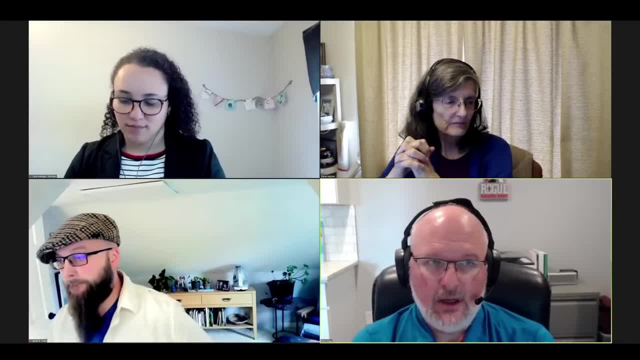 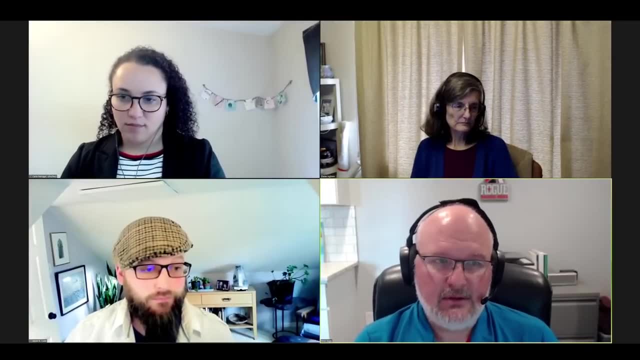 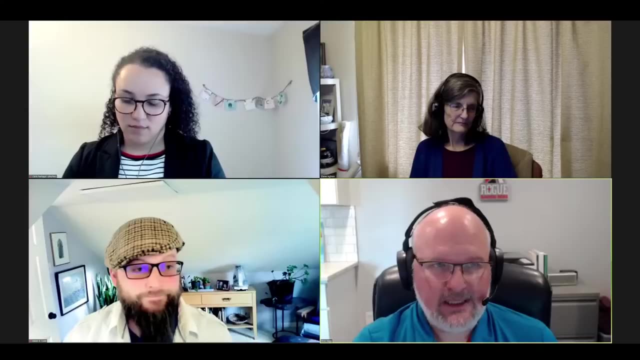 There are going to be Cases- I run across the time- where you deal with the heavy contamination issue or problems that you're just having to undercover As you going along and it can be kind of a slow transition. other cases you know you do all the right thing is you're decompacting. the soil. you're adding biology or putting plants in the system. You know, keeping the soil covered, including the wood crops, You know what you would be able to garden all at once in a year Would bephusian in years to do a great job. that you get the soil to grow it back together and support soil. 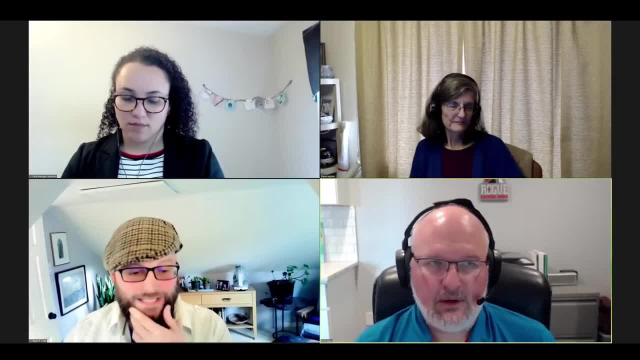 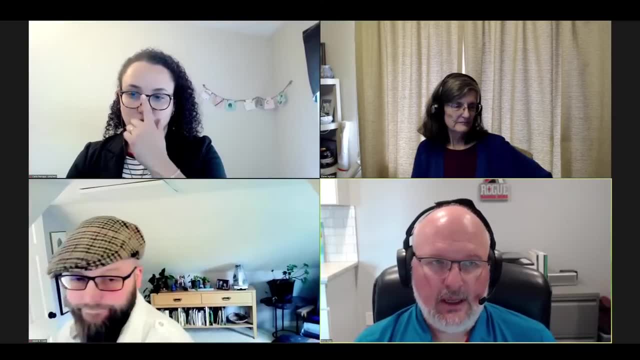 And you can see significant benefits. I'll use an example with one of my farmers. They were putting on 200 units of nitrogen per year in their orchards And after one year of us doing remediation work we were able to step that down from 200 to 80 units. And that farm still has significant challenges with compaction and some of the ways they have to manage the farm. So you know, we could probably see much bigger gains if we didn't have some of those other headwinds in front of us. And so from my farmer standpoint, hey, that was over, like a 60% reduction in input costs. That's big. That's a big, big change that you can see within a year's period of time for sure. We have a lot of examples on the website of how much money was saved or what. What was the improvement in nutrients? What was the reduction in the costs? You don't need any more pesticides, You don't need the herbicides, You don't need the inorganic fertilizers. It's all going to save you money. 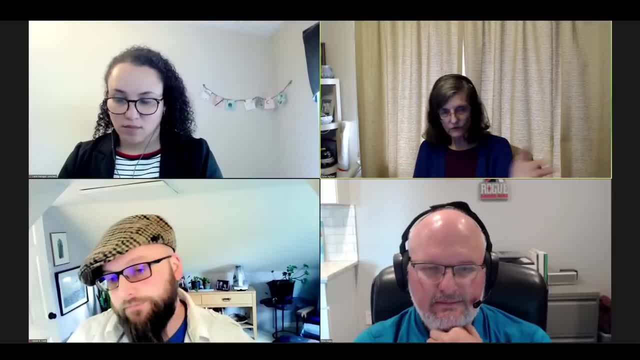 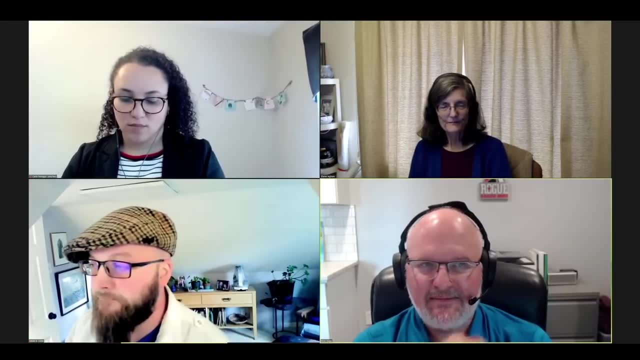 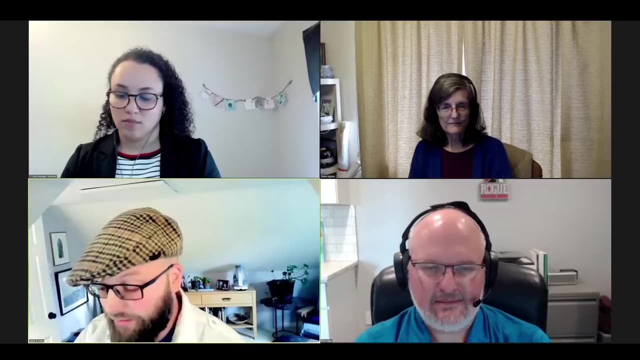 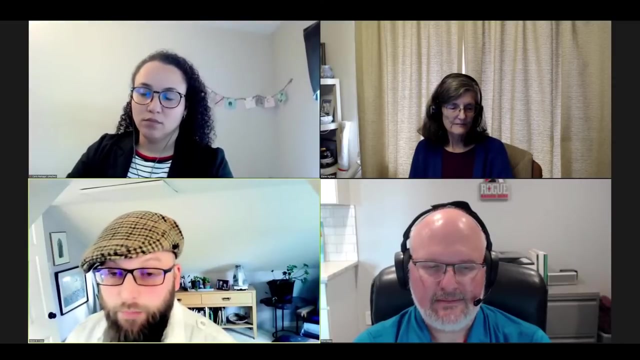 Never mind the fact that you're not running your tractor back and forth over your field umpteen times. Right, You know this is not a scientific peer-reviewed source, but I'll talk about my observation of something. I took the foundation courses and Elaine taught about the flocculation of clays where they don't have the right mineral balance between calcium and magnesium. 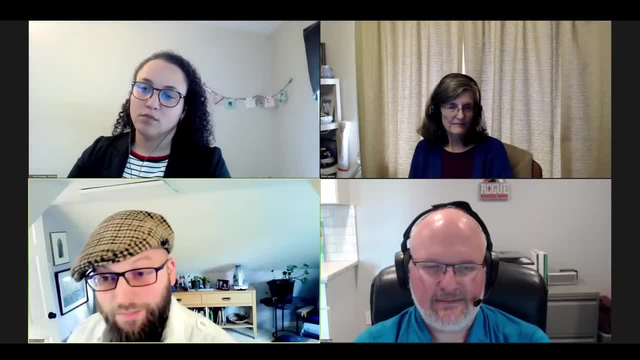 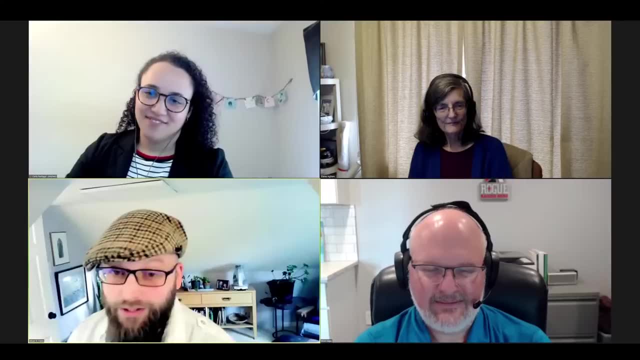 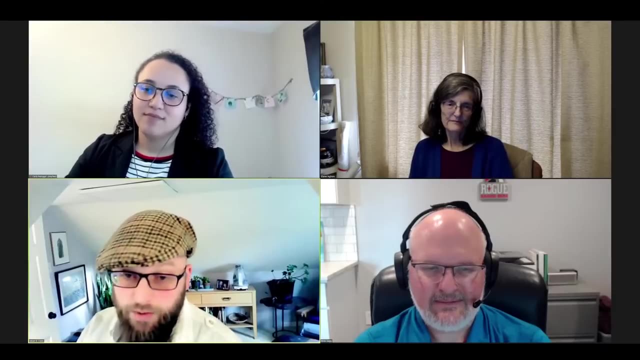 And she mentioned oyster shell, which I happened to have some of, And so I went and I shook it out on my garden. I didn't even do a lot of incorporation into the soil, maybe a little bit with pitchfork that I kind of aerated the garden area with, but I just took this bag which I had. bought to give to chickens and I used it there, And it wasn't the only thing I did to change the soil system. So again, not a peer-reviewed study, but within the later two months of that season I dug down and said, wow, there's all this pore space. that wasn't there before. There were all these worms. 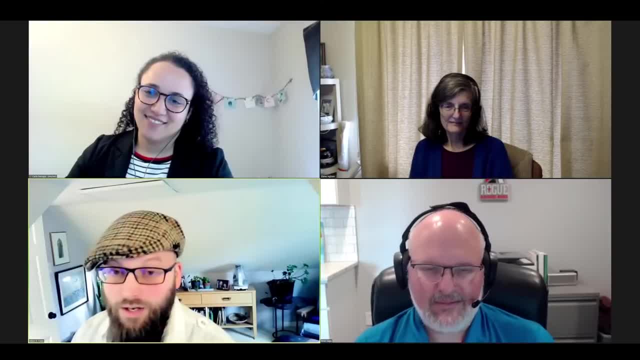 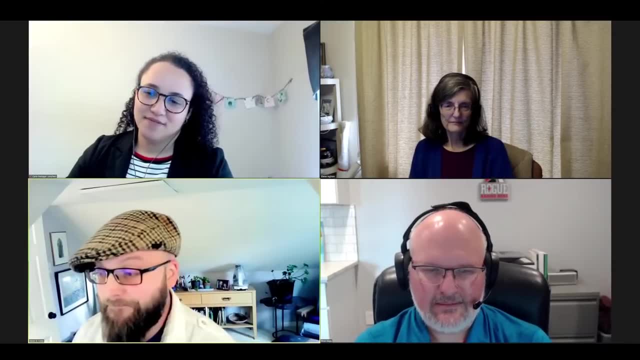 It was like it had previously been such a competitive Pacted clay soil where blackberries had covered the area for a long time. And and I said, well, it could be that the flocculation thing, which is just a complicated word having to do with you know, the soil particles are either attracted to each other or they're a little bit repelled by each other. 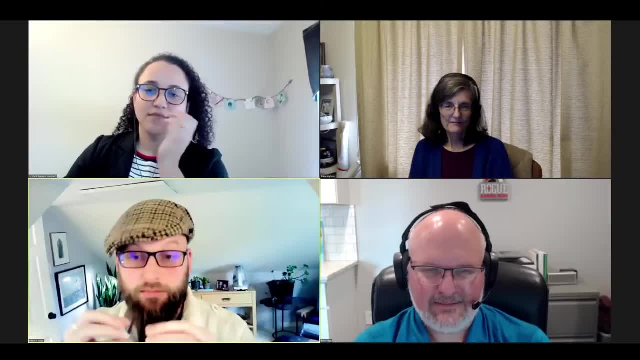 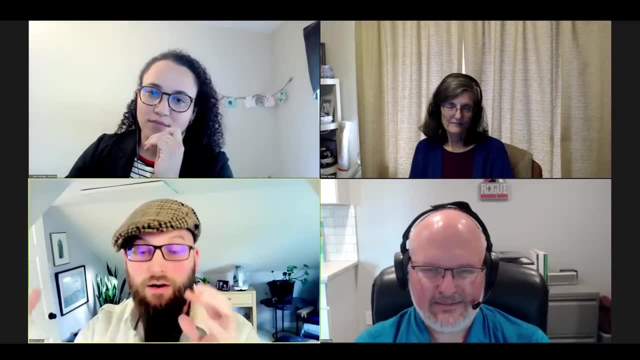 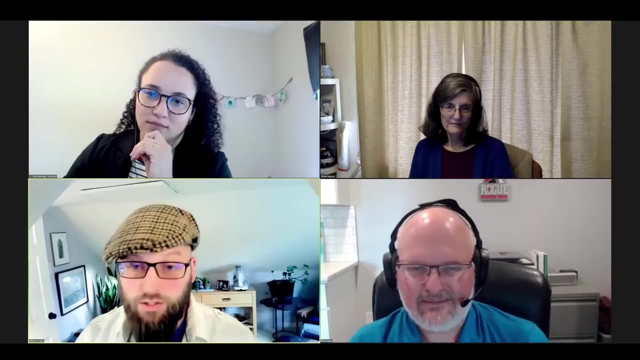 And if you bump up that calcium load it seems like it helps a lot of those clay soils push apart from each other a little bit more, so that biology and air And water can get in there and keep changing that system. So there's an example of a physical or chemical intervention that can work in tandem with the biological to really improve the situation. That's what we love about fungi, because fungi end up trying to regulate to that kind of perfect balance, which is great news for us. Let the fungi do the work instead of me. Exactly A lot of nice Exercises, as if you have like some leftovers of compost, just put in one location in your garden or backyard. Give it like a couple months and go back and scavenge below the compost pile and then outside the compost pile. The difference is beautiful to see. Yeah, for sure. Okay, let's move on to our next question. This question is from Rue. 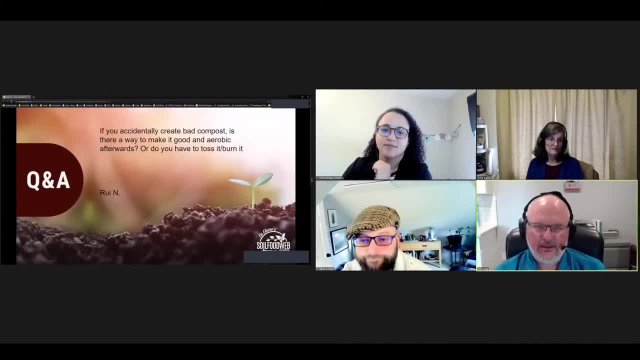 If you accidentally create bad compost, Is there a way to make it good and aerobic afterwards, or do you have to toss it, slash, burn it? No, do not burn it. It's still good organic material. You just have to take it through a good thermophilic pile system. You know, the bad compost is typically because you allowed that compost pile to go anaerobic. You didn't turn it enough, You didn't turn it when it was appropriate to turn it. You didn't get the oxygen back into the pile. And you know we keep discovering more ways to get oxygen easily back into that pile. So you don't ever make a bad compost, unless you utterly ignore absolutely everything Mother Nature is trying to send to you, like smacking you upside the head over and over. 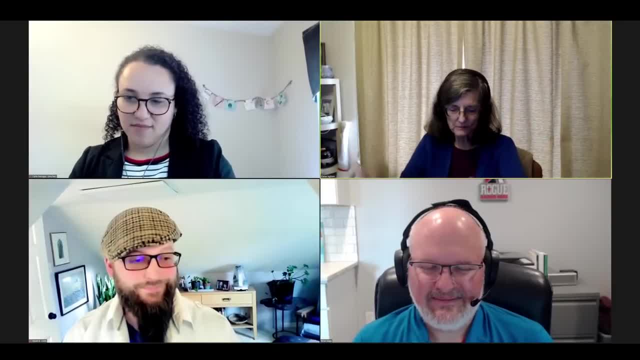 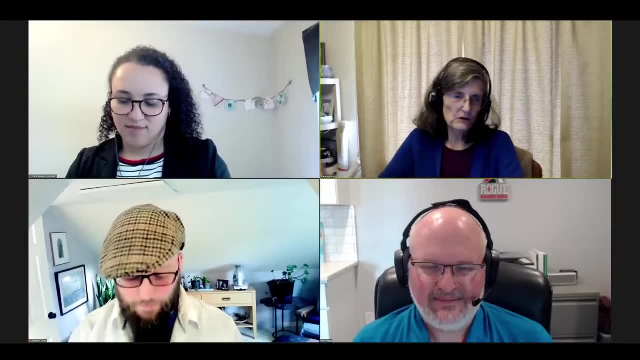 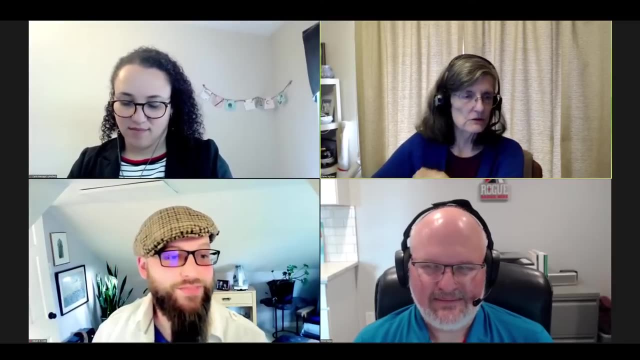 How long, How many times is it going to take till you wake up and and do what's right so that you keep the Oxygen in that pile? And, of course, if you take our FC courses, we'll go through all those little secrets with you so that you can always be assured that you make good aerobic compost. 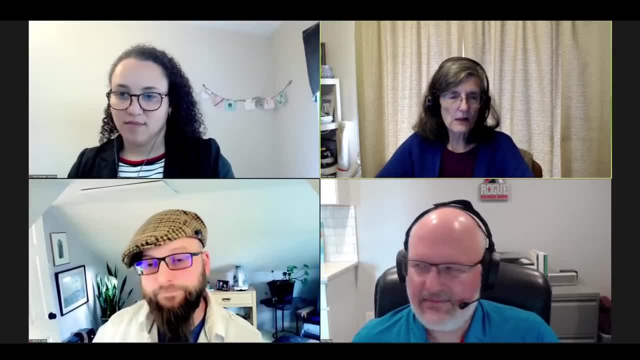 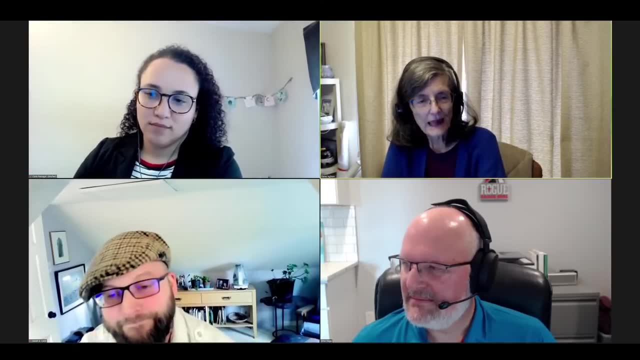 You don't have to worry about is E Coli or Salmonella or Pasturella or any one of those human pathogens. They are strict anaerobes. You know, even E Coli is a facultative anaerobe. 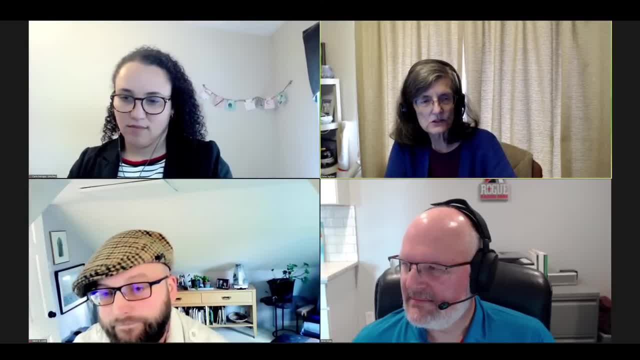 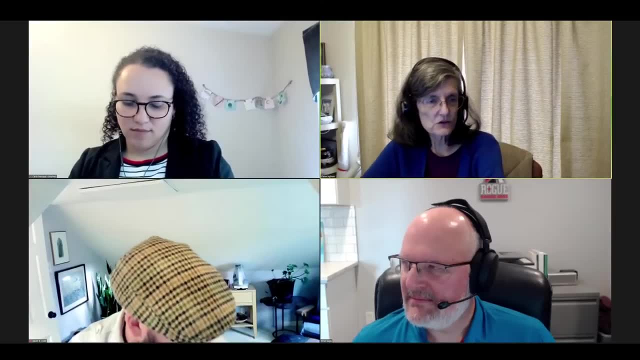 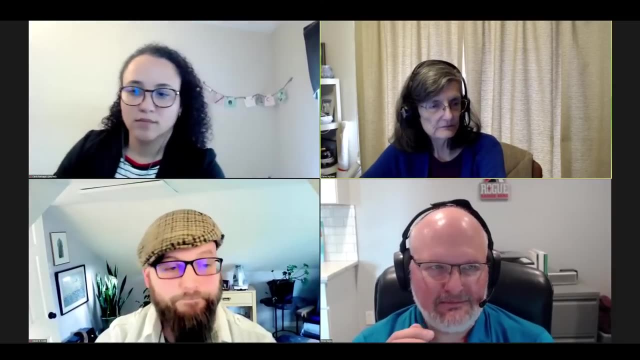 It does better When there is reduced oxygen, So get the oxygen up. All that is really going to select for the beneficial organisms that will prevent the diseases and pests, et cetera. Great Panelists, anything else you guys want to add? 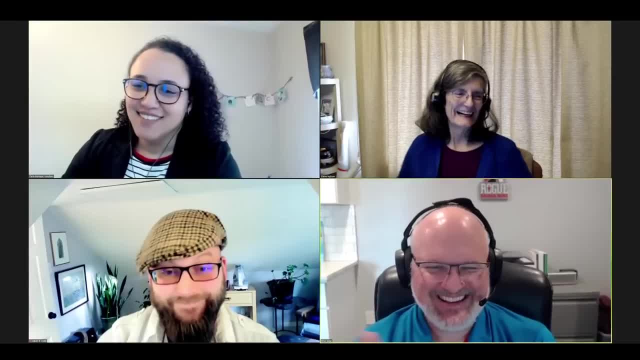 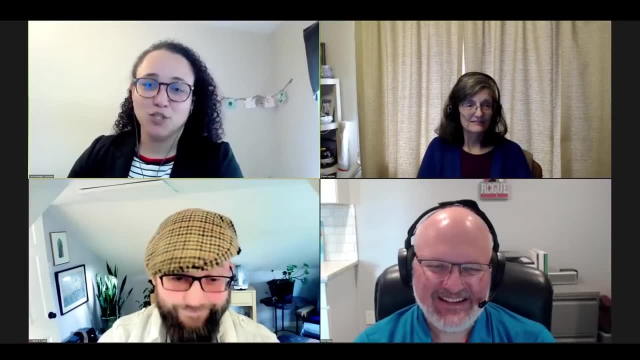 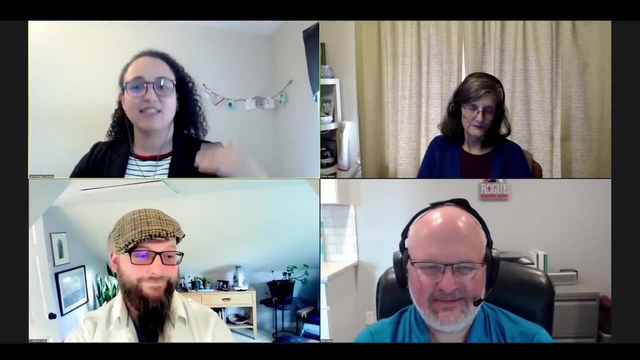 Yeah, just a pretty easy answer: Yes, you can. Someone just said that the only thing that you can lose is time, And I dare to say that not even time, Because we learn much more When something goes sour. there's a good chance to revisit our steps and crosscheck, revalidate our mindsets. 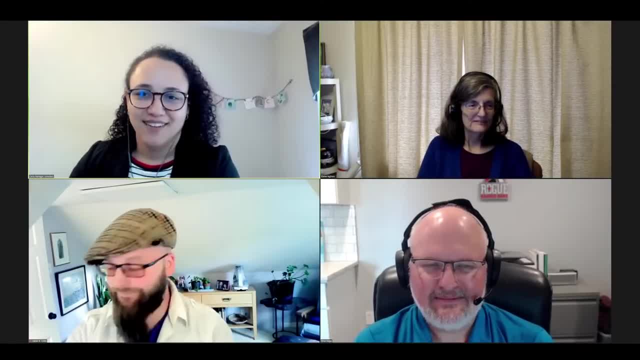 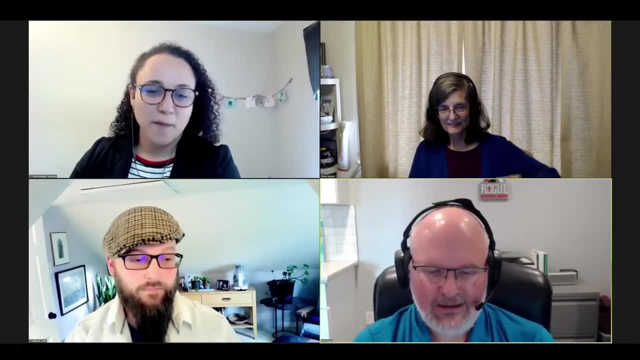 Someone said as well as about mindset. So yeah, it's all a learning curve. Exactly Yeah, And you know- a lot of people I'll talk to you, know my clients or students and so forth- that when you're making compost, there's an intuition that gets built over time. 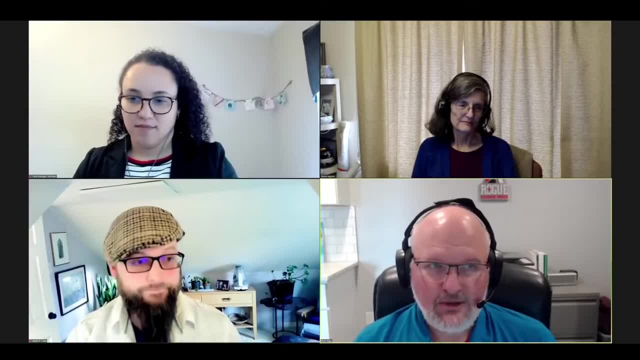 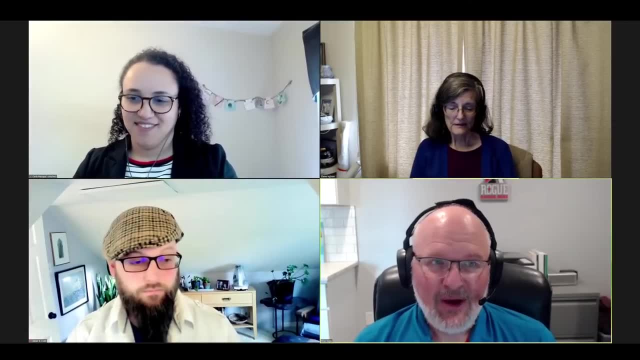 And that's because of your successes and your failures. Um, and pretty soon when you start making a lot of compost, Yeah, And pretty soon when you start making a lot of compost Piles, you'll know pretty early on, like I did, assess my starting materials very well. you know, or wow, overwatered. 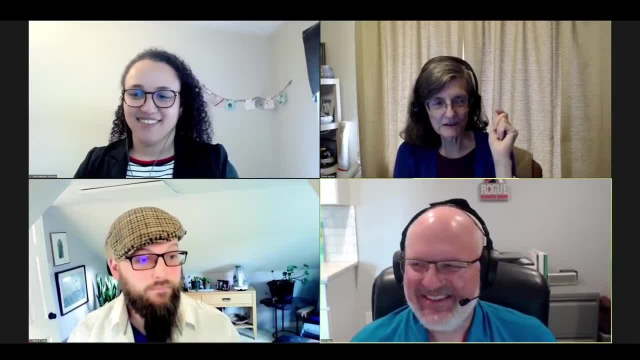 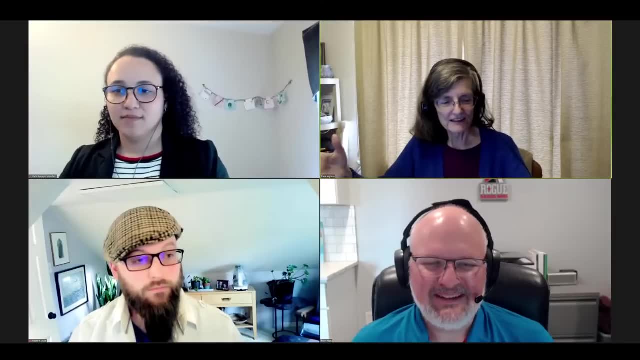 Yeah, I should have done that. You lift the tarp off and you go: oh um, that doesn't smell good, Exactly, And it's not past the point of recovery. It's really easy to get it back if you pay attention. 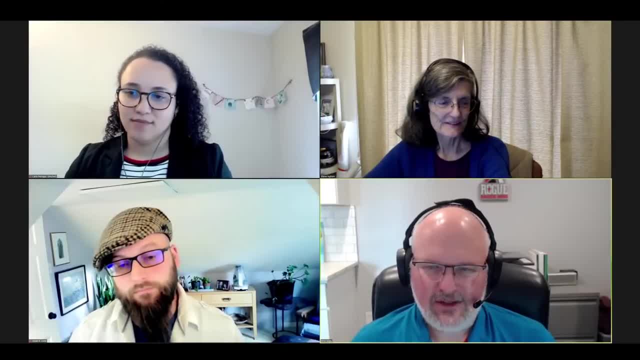 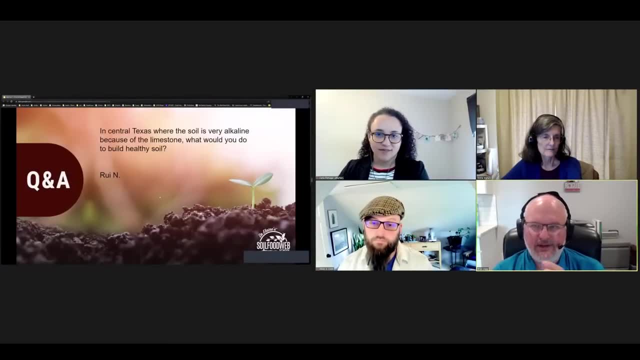 Yep, Okay, Next question. This question is from Rue as well, And the question is in Central Texas, where the soil is very alkaline because of the limestone. what would you do to build a healthy soil? Grow lots of fungi. The fungi require slightly acidic conditions and the fungi will fairly quickly move the pH. the right kinds of components come out for growing the fungi. So you really want to shift the bacteria Bacterial to fungal ratio bacteria in aerobic conditions. the bacteria generally are going to be those species that will make alkaline waste products, holding and keeping the pH in that soil on the alkaline side, which is what those bacteria want. So make certain you get a lot of fungi back into your compost pile and use that inoculum to drop the pH And get that pH back to around six, five, six, eight, where most of our- you know it's certainly our better- crops need that, that, that pH level, instead of the really high alkaline pHs. 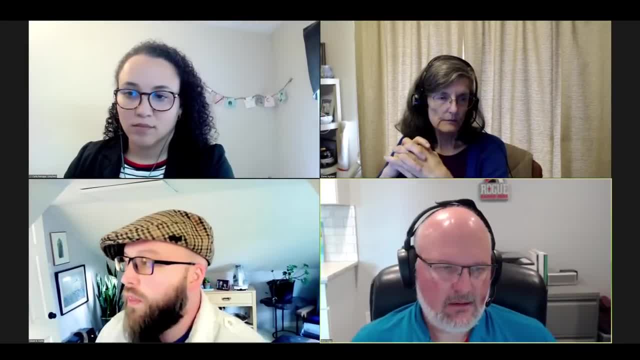 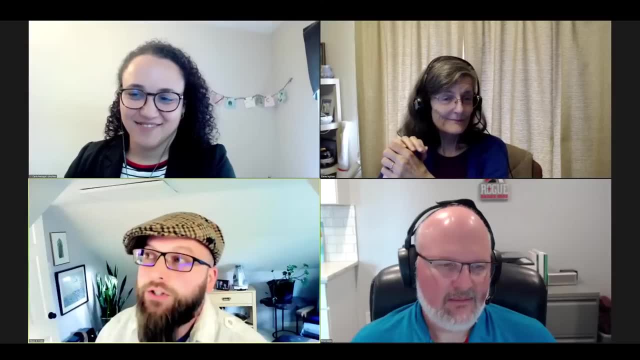 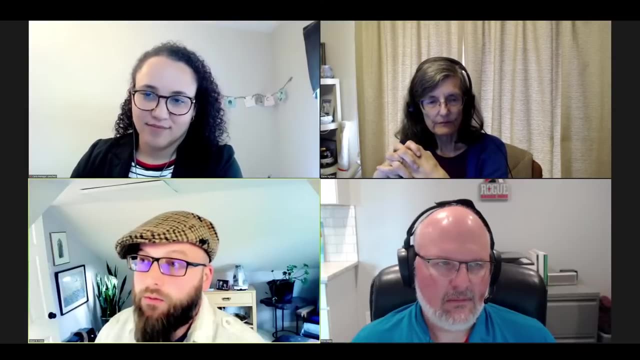 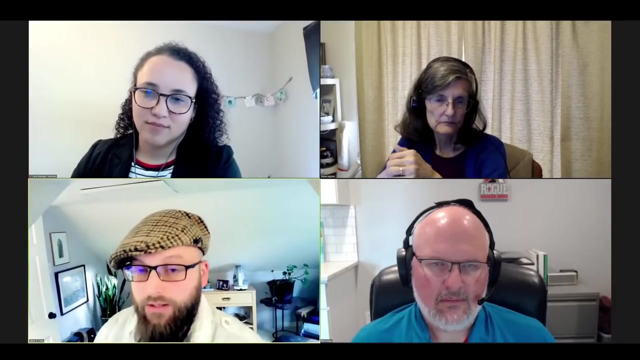 Panelists. what say you, Any other, any other comments you guys want to make to that? Hmm, it's a really good question. I I've seen a lot of potential in really good organic matter to buffer any pH imbalance, whether it's acidic or alkaline. Whereas you know certain things like biochar as an amendment, might be associated more with like taking the soil from acidic to alkaline or to neutral towards neutral- There's probably not very many neutral soils in the world, But yeah. so I think of that as like I think of getting your organic matter up and adding organic materials and seeing the accumulation of organic matter as one of the best investments you can make on any future disturbance to that system or overcoming any natural tendency because of the mineralogy in the system to to be. 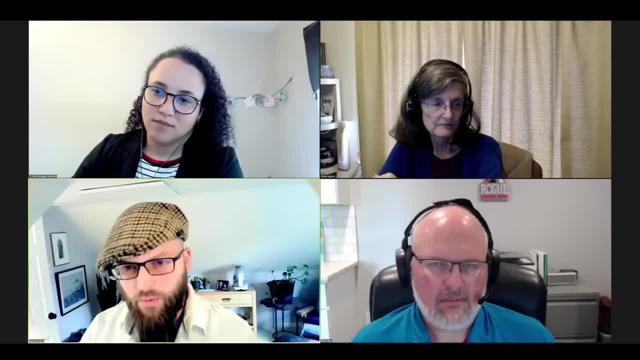 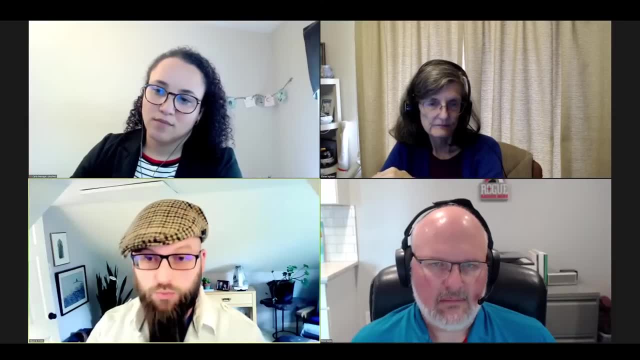 Yeah, Far from the target. And the reason why we all focus so much on getting the pH right is that we know that that some of the minerals are really a lot harder for the plants to absorb and and for the microbes to access and for things to be alive and thriving. If we go very high pH, very low pH, And it depends on the plant. Some plants like lower pH than others, Right, But yeah, I just think organic matter is one of those few. It's almost always the right thing in the world to to get your organic matter up. 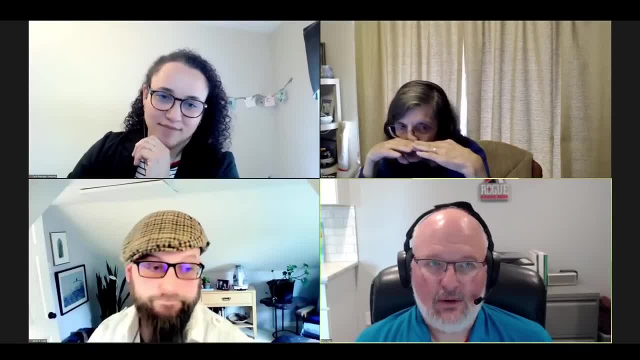 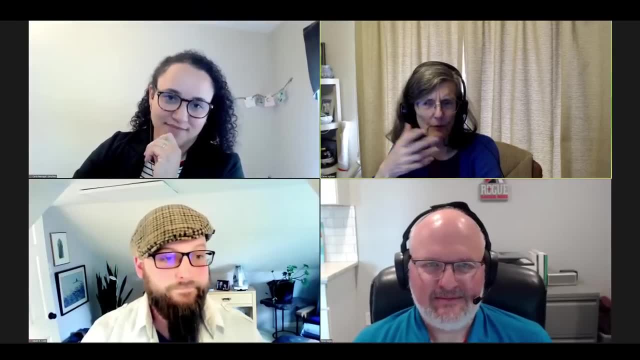 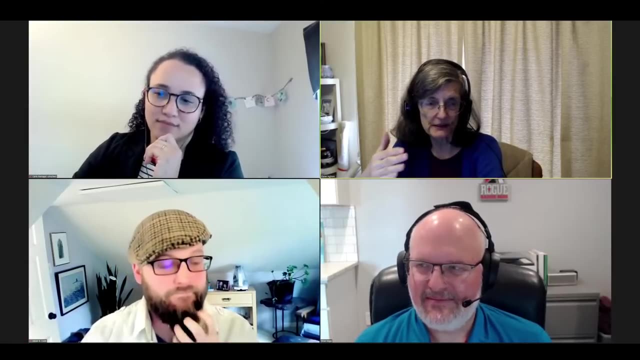 It's going to buffer that system And we know in most agriculture systems that organic matter is way, way too low. Minimum organic percent organic matter, from my point of view, is 3%. You have to have it over 3% or your organisms aren't going to go to work because there's nothing feeding them. The root systems are in trouble. They just don't have the nutrients that are needed by this, the bacteria and fungi surrounding those root systems, to really move things along. So, above 3%, how high can you go? My attitude is: I would like to have my soil be 100% organic matter. Because I want all those good organisms moving their way through that organic Matter- having lots to eat, lots of air passageways, lots of flow- get the biology to what the plant requires. So yeah, somewhere in between 3% and 100%. 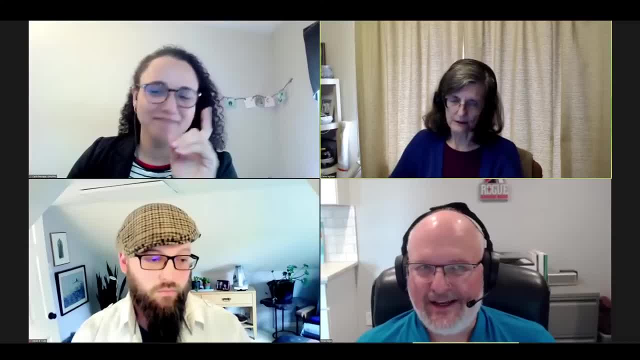 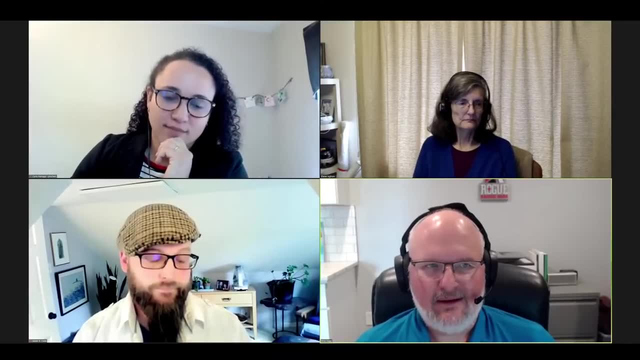 But just not below 3%. And we see it all the time. You'll go into fields and there'll be 0.2%, 0.3% organic matter And the structure's not there. It's usually compacted, very anaerobic. 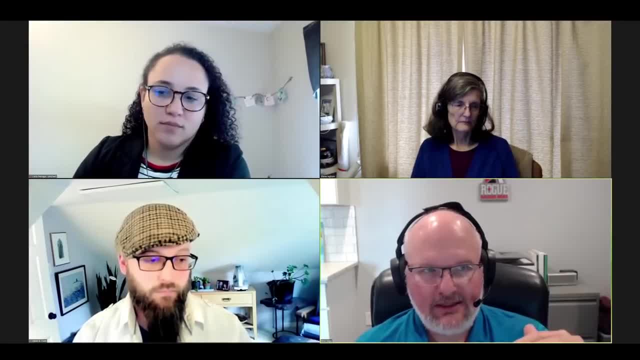 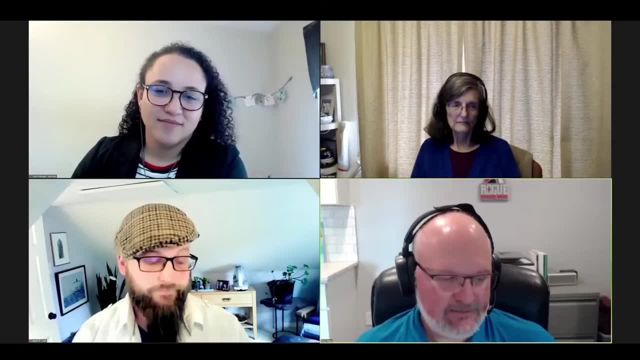 And we struggle, They establish. You know, it's kind of like a curve If we're getting all of a sudden we're getting above 3% organic matter and things really tend to start to happen fast. Okay, It's just a quick joke that I make with my students. 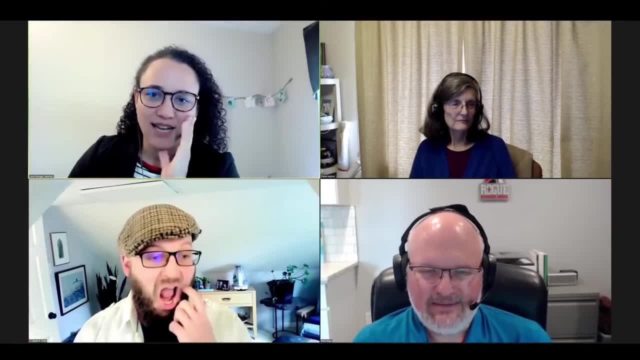 It's just like when you're moving to a new house. The first days is just like you don't even know where to start to unbox things, to put it in place, until you reach that curve. Okay, now I'm feeling at home. 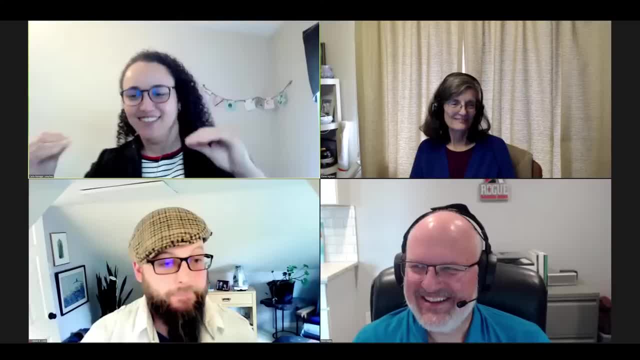 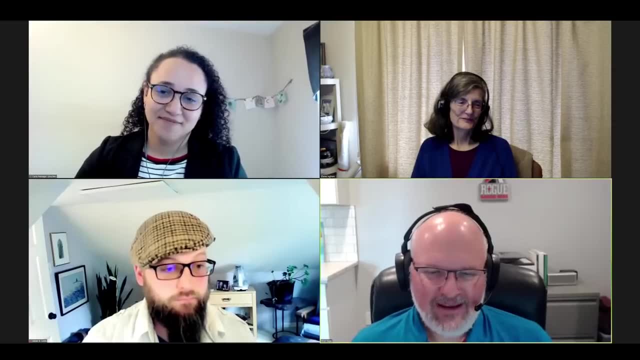 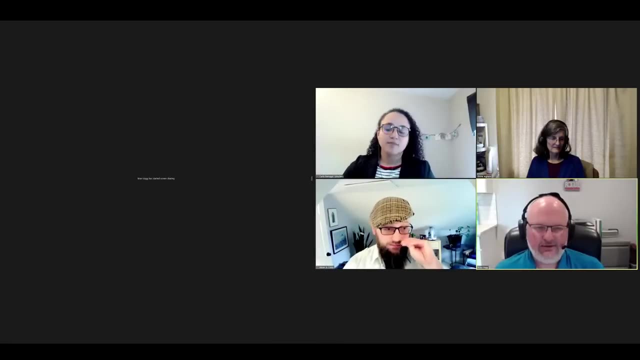 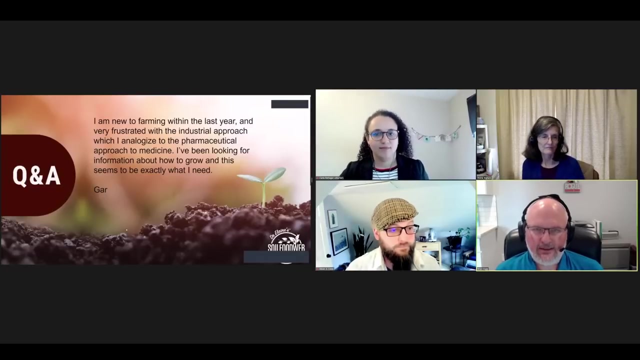 I can catch up. So it's that same logic, right? We have to put ourselves in the place of this little Guys. what they need to try, Sure. Okay, let's move on to the next question, and this one really is just more of a comment, and then we'll move on to the question itself. but this is from Gar, and Gar says: I'm new to farming with within the last year and very frustrated with the industrial approach, which I analyze. 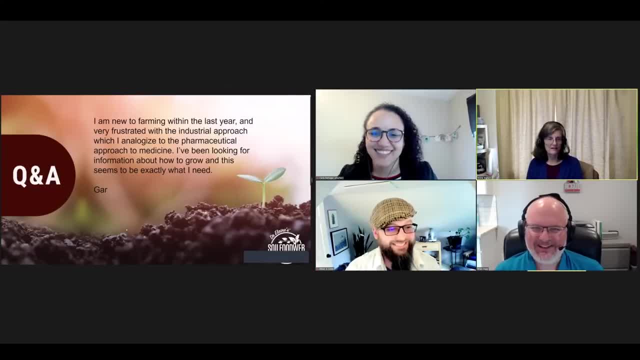 I apologize, He apologizes. He apologizes to the pharmaceutical approach to medicine. I've been looking for information about how to grow this. It seems to be exactly what I needed. I hear, Gar, that was kind of my my way as well. 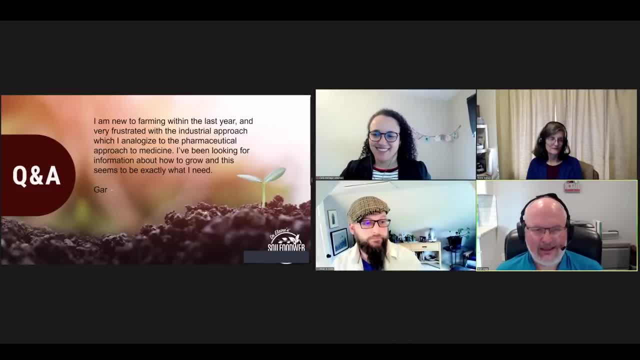 I started, very conventional my homestead and said this does not make sense. And then when I really started understanding about the soil food web, it was like okay, dots have been connected. Hoo hoo, Now I'm getting it. 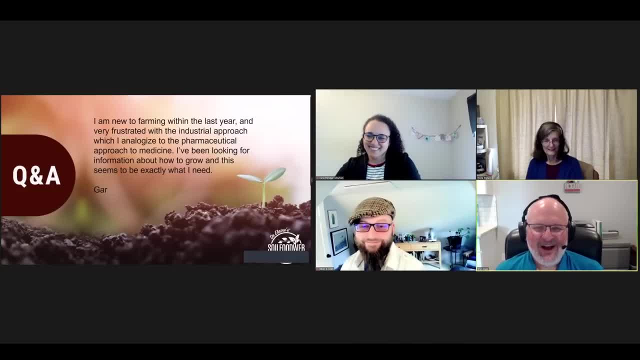 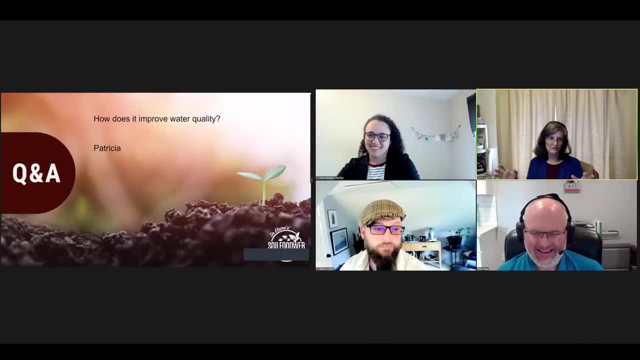 So thanks for the comment, Gar. Okay, Um, you go ahead, Elaine I. I started out working in natural ecosystems and putting together the model with uh all of the guys at Colorado state university, uh University of Georgia, all over uh working on that food web. 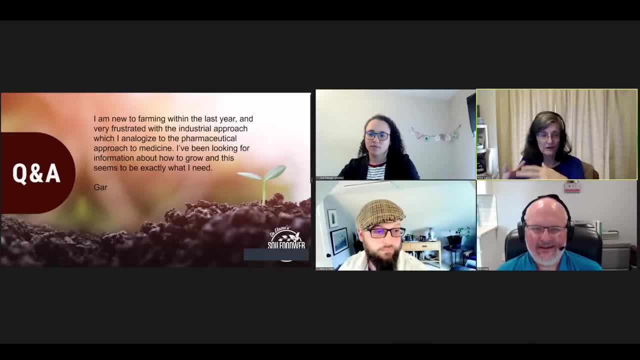 And then I came into doing um agriculture and I was blown away. How could you even begin to think about growing a healthy plant in something that has none of the health factors that soil has to have in order to grow a healthy plant? So there's, you know, slightly different. 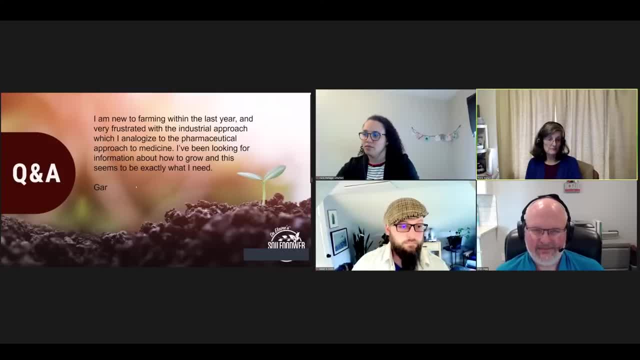 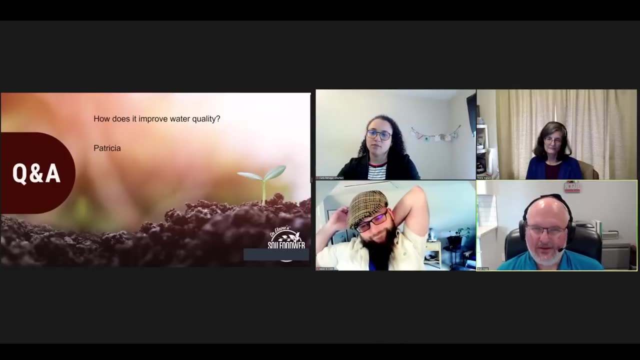 Um, initial approach, but we both came to the same kinds of conclusions. Okay, Uh, let's move to a question from Patricia, And I think the question is: how does what we do improve water quality? Um, and I, I really think there's kind of two parts of this. one is, um, you know, really, the water quality of the water sheds that that come off of the lands, that that we treat. 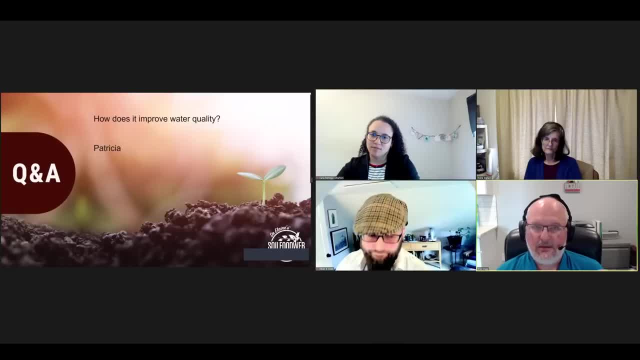 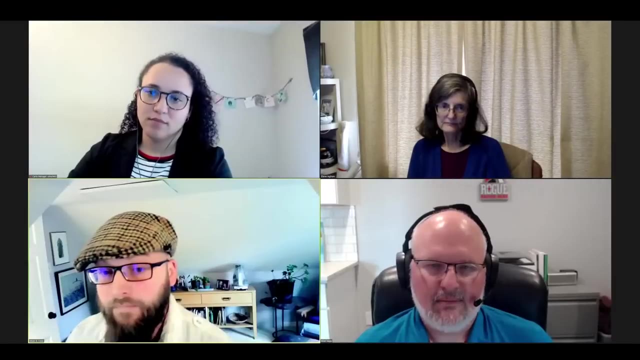 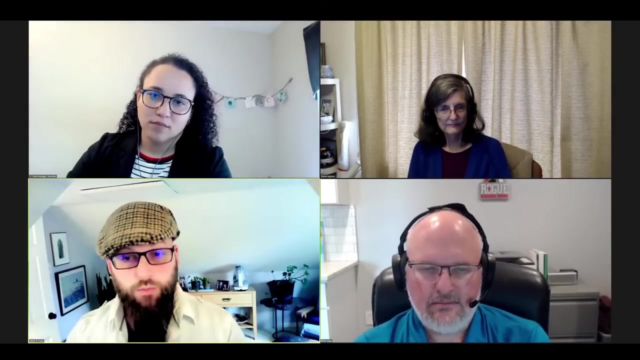 Um, and then also, how do we improve water quality that we're using in, Okay, Our, on our plants as well? Anybody want to tackle this one. Well, I mentioned that industrial agriculture, because there's so much, so many excess nutrients and um herbicide and pesticide and other residue that can get into water streams. that represents, um like a clear disruption. 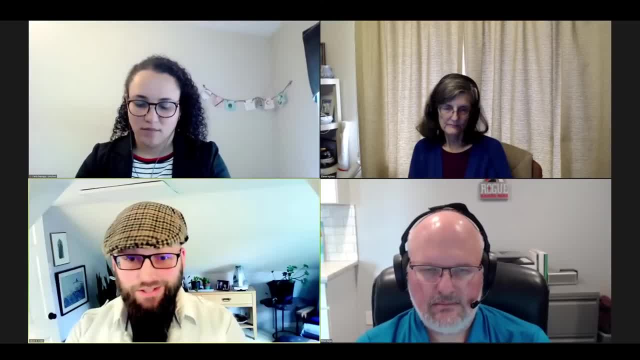 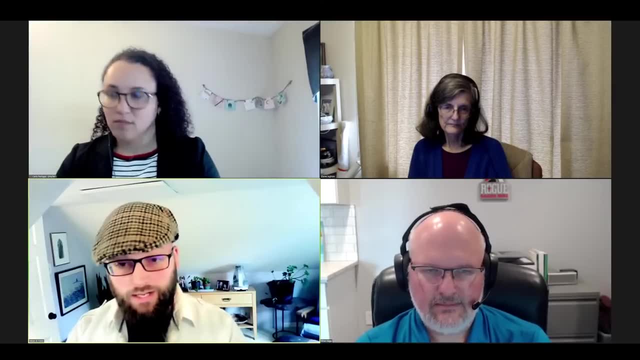 So it's a, it's a this, as opposed to that statement. if you, if you aren't putting all those chemicals that get into the watershed, that's an instant improvement. But then over time, with the accumulation of um, you know, organic matter, we use this as an umbrella term. 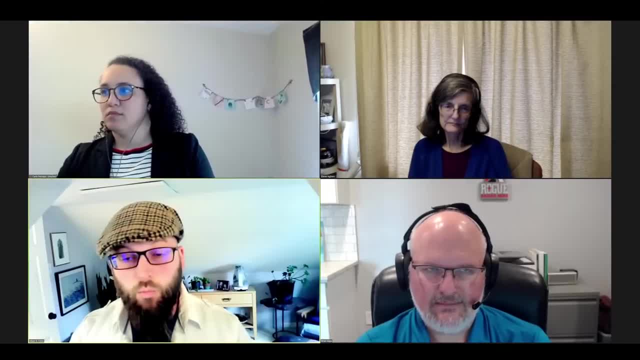 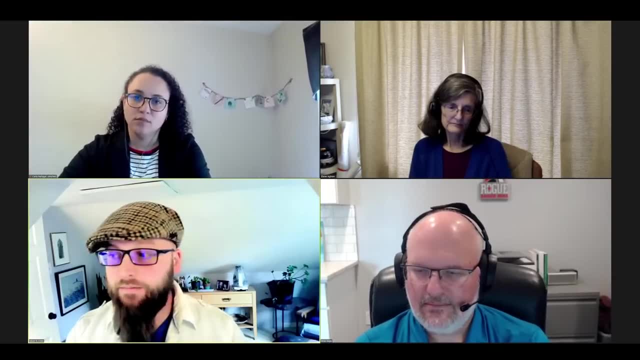 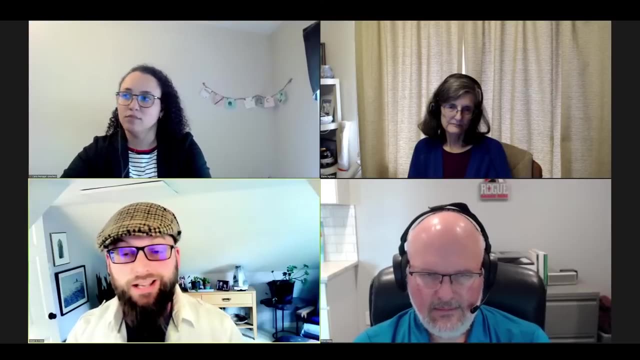 There's different kinds of organic matter And when we get the fungi, especially, really doing their work of entangling soil particles and all they have this we we talk about it being recalcitrant or resistance- They have this kind of organic material, these kinds of carbon structures that can last a long time. 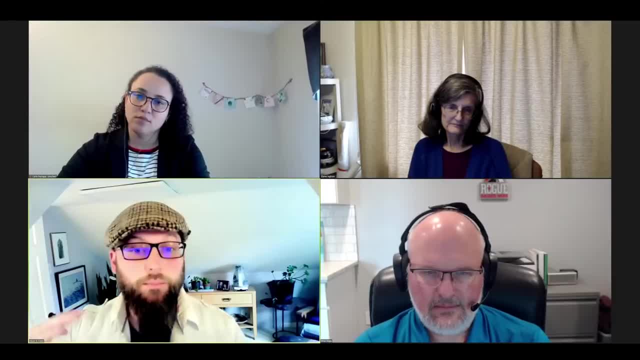 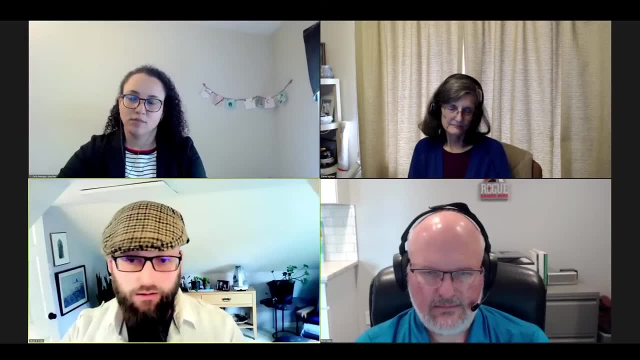 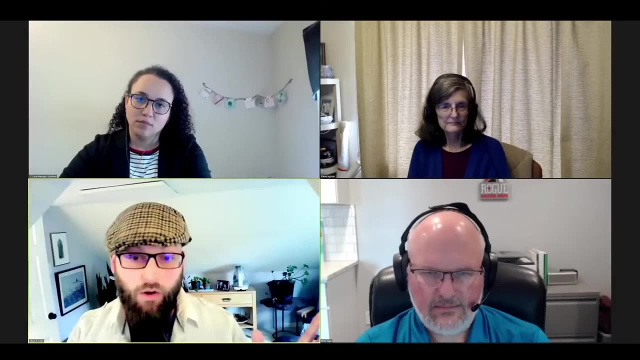 And so when people say like, oh, my organic matter Is only 1% or whatever, I think that's not just about having organic, putting more organic materials in. it's about creating the forms of organic materials that won't just be gobbled up and blown off as CO2 all the time. 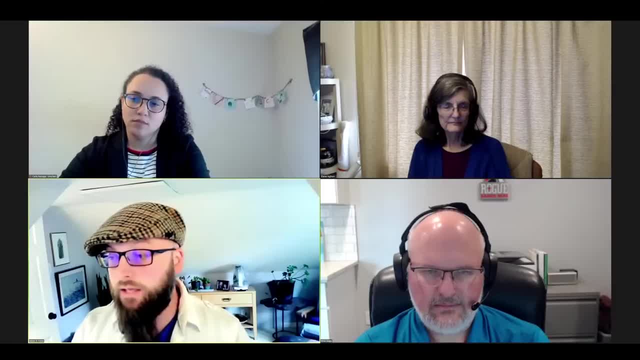 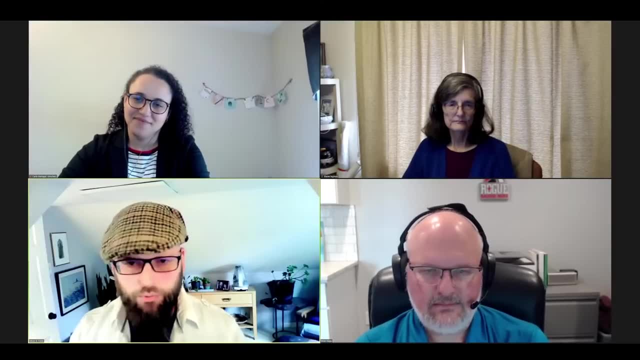 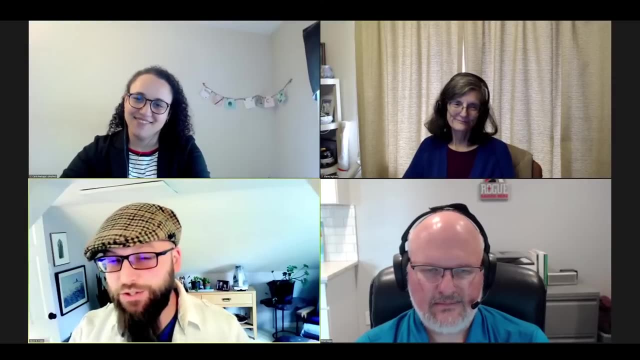 Right. So those resistant forms, and if you really get your fungi and your plants working in tandem, that's a huge way that you can um improve that. So it just so happens. And, and Elaine, Yeah, You know, um, I can't remember the case really clearly from the FCS. 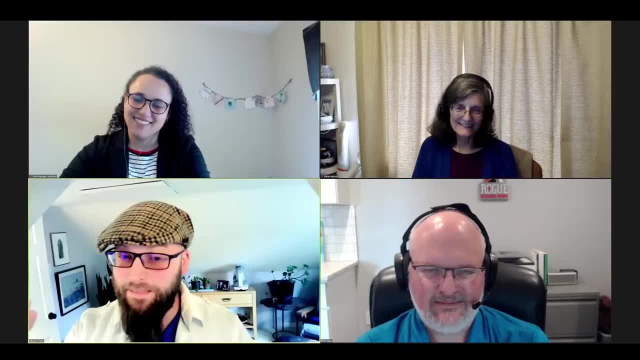 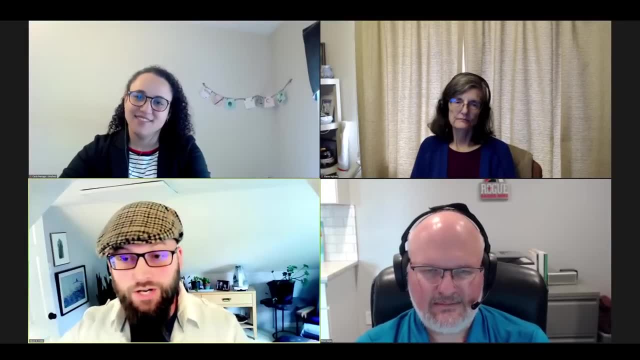 So I'm hoping you can where, like there's research that's been done where they've taken water and filtered it through soils and increasing the amount of fungi in that soil, It means that the water coming out at the bottom is cleaner and cleaner right. 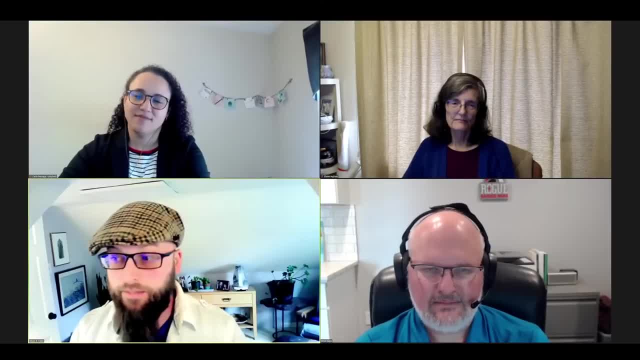 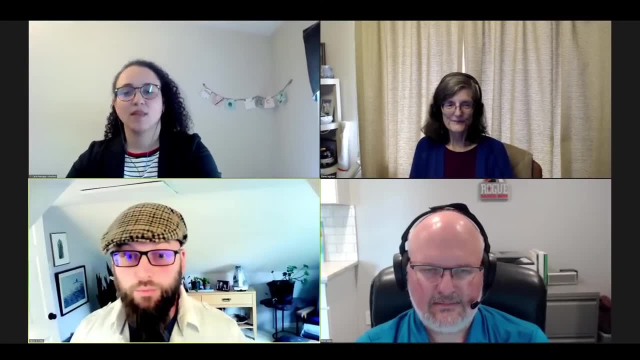 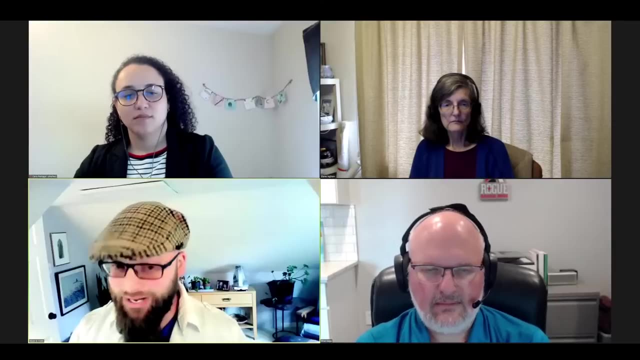 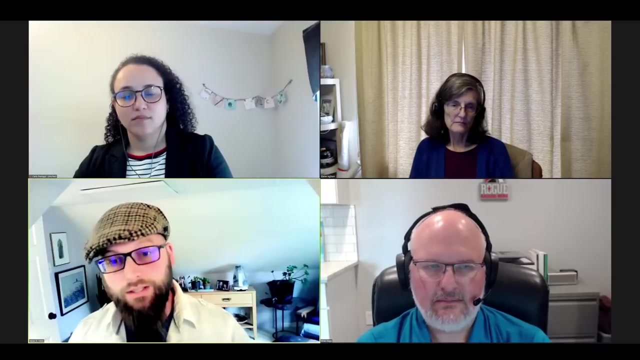 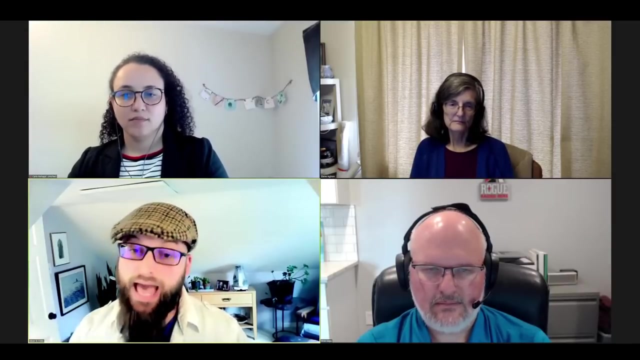 It's like filtering actively the, the contaminants or the nutrients or whatever you want to say, the sediments And all So really it's like creating a water purification that's, that's biological, right there in your soil system. So those are the two main ways I would think about it. improving, like downstream watersheds, is we're taking the chemicals that are harmful out and we're putting in the biology, which is this very active filtration system. 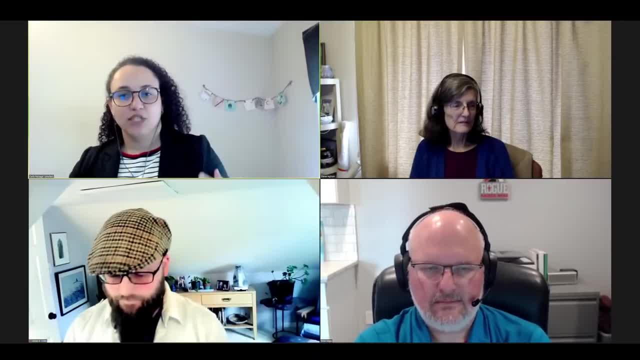 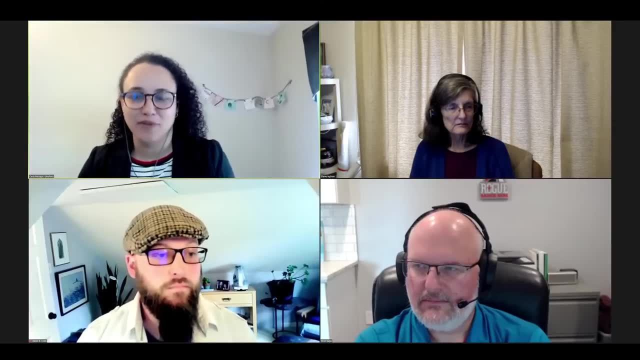 Yeah, And thickening landscape in general. We have to remember, We have to remember always that the riparian forest, riparian woodlands, are exactly the filter that we need, So we need to respect this limit. Some countries have this under the law. So it's protected by law. Other countries doesn't. But we cannot expect just this coming from law or government to do this job. So if you have any water flow in your property, work on restore that riparian zone in your property- already doing amazing job. To recover the water quality through the whole entire watershed system. I like to. when we're doing hydroponic kind of work is always right after you've run your water by all of your plants sitting in the whatever kind of holding pattern you have, that water should go through a large filter. 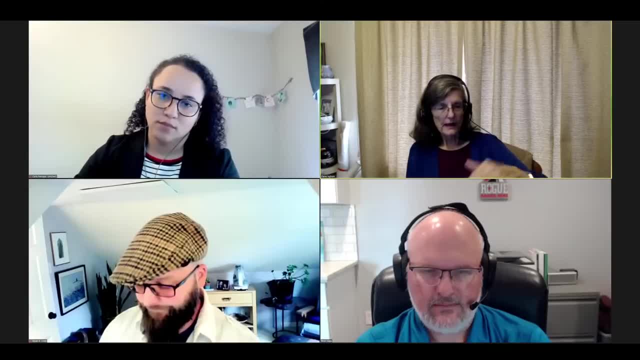 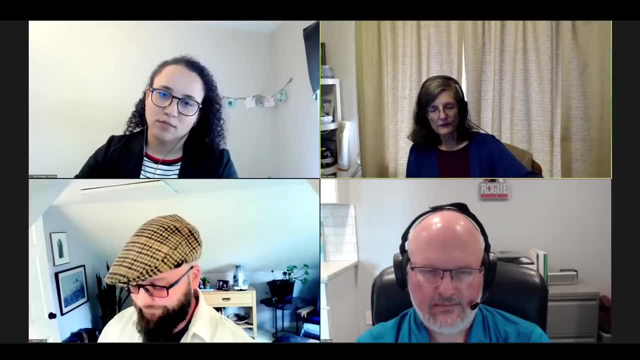 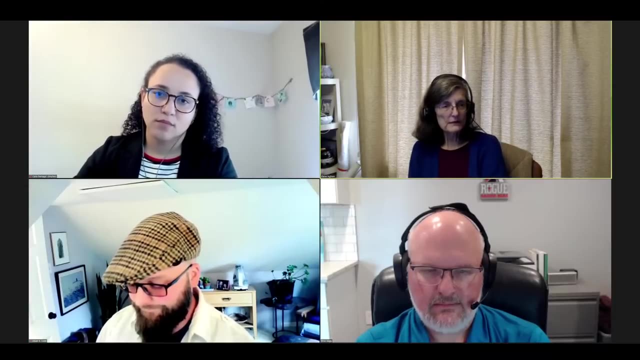 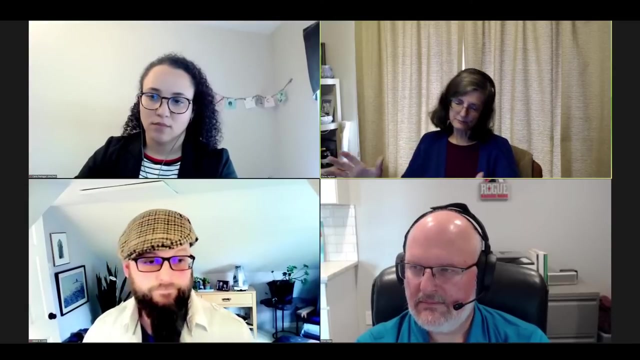 That's basically just your compost, And have all of those out of balance nutrients get held in that organic matter. So now, what comes out of that? Don't run through your compost. Well, put it right into the tank where you've got your fish growing, for example, because now those fish are going to be pooping and peeing, as the case may be, into that water. And that water then goes up And your plants take out that high level of nutrient that's present and it goes back into the compost and it works really well. You don't have to be worried about. you know what do you do at the end of the growing season. 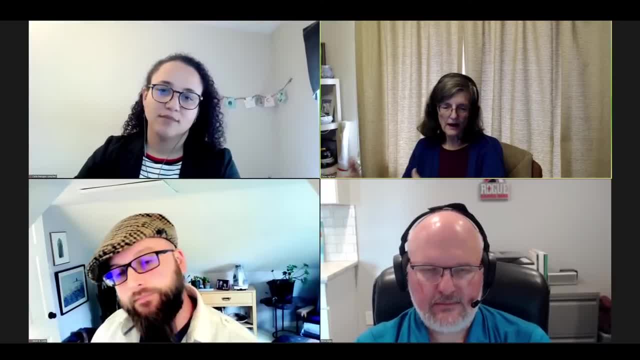 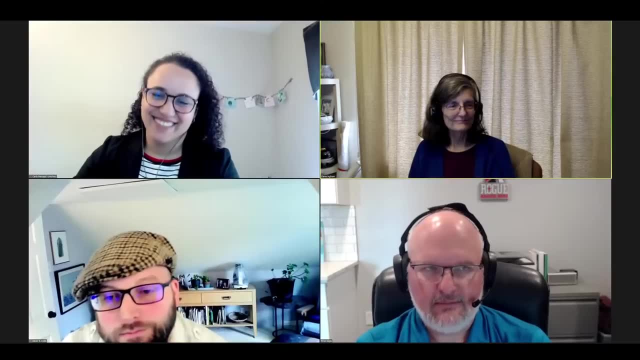 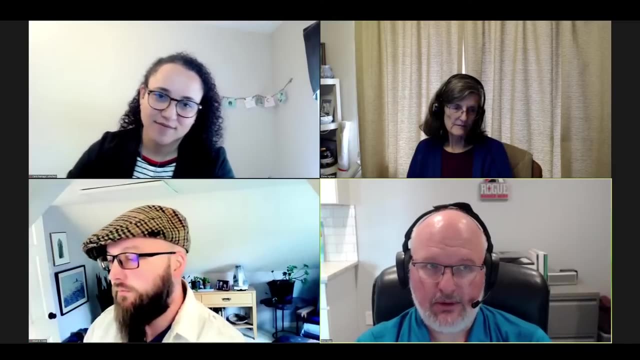 And now you've got this water that's just chock full of all kinds of imbalances. So let nature do that work for you. Yeah, And I think you know watershed issues are definitely becoming much more prevalent. I mean, you look at, like the Gulf of Mexico, right? 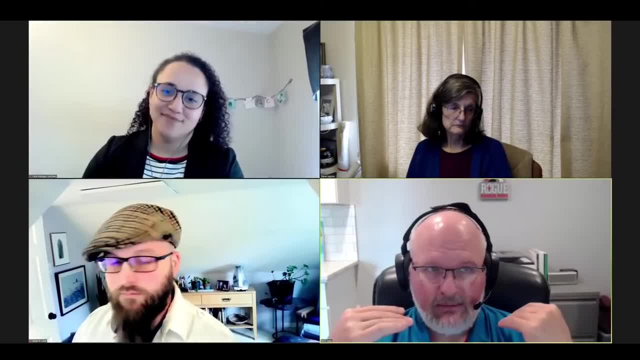 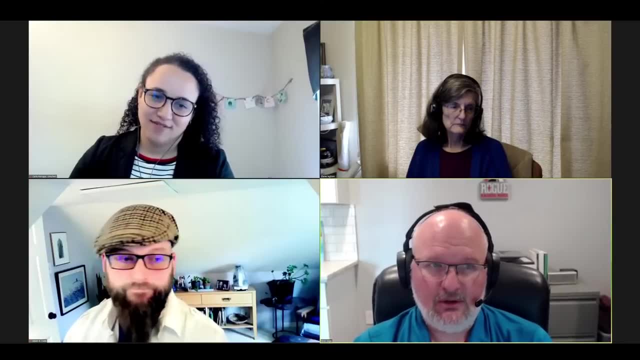 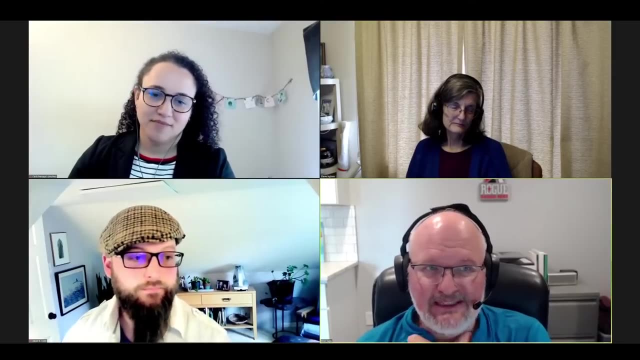 It is Wow. All that stuff coming down through the Mississippi watershed out into there is creating these massive dead zones. That's simply because it's just so much nutrient load that's just being pushed right into those big areas. And could you imagine being in the fishing industry- the impact to your business, right? 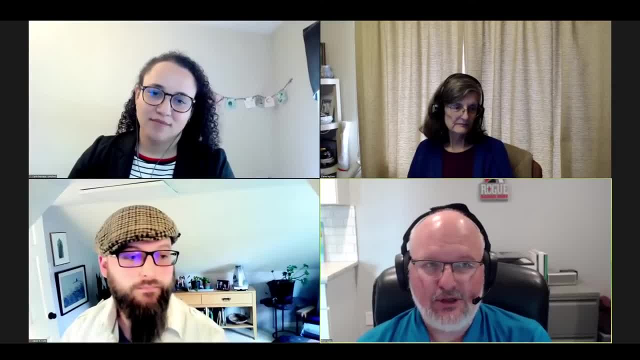 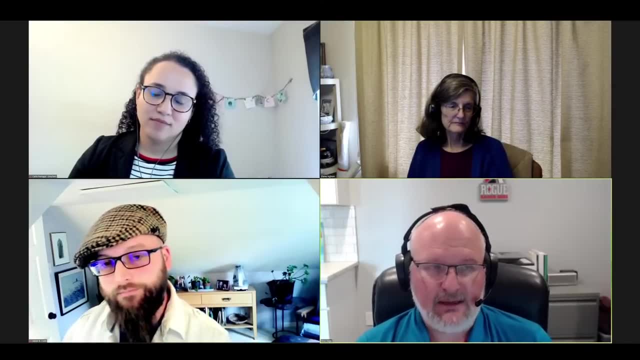 And unfortunately those costs are, Those costs aren't being necessarily appreciated on the land that's being grown, that's applying all those chemical fertilizers and so forth. And we have to look at, as Adam was talking about ecosystem management, Look at the entire ecosystem. 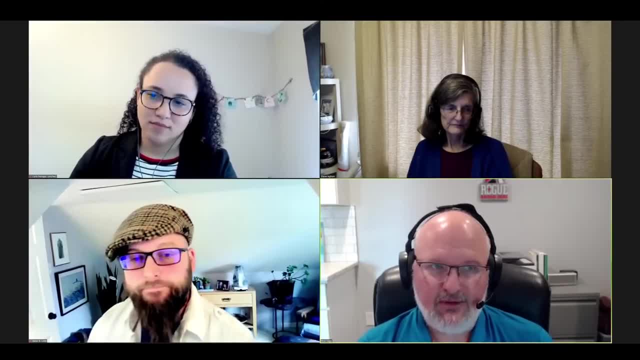 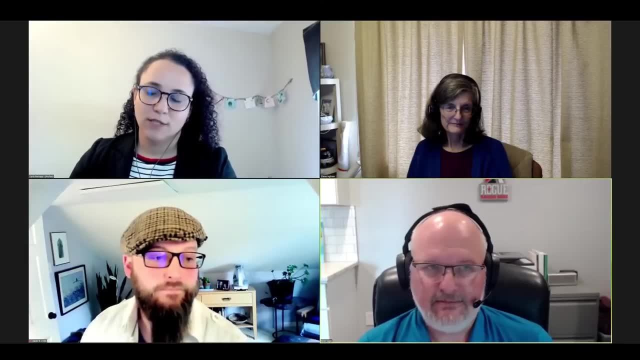 And this is something that is not just for the own individual farm, but for all the watersheds that come off of farms. We really, really need to have this kind of work be done. So, Okay, Anything else you guys want to add? 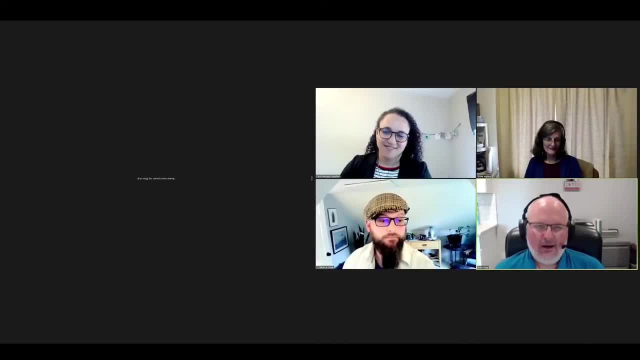 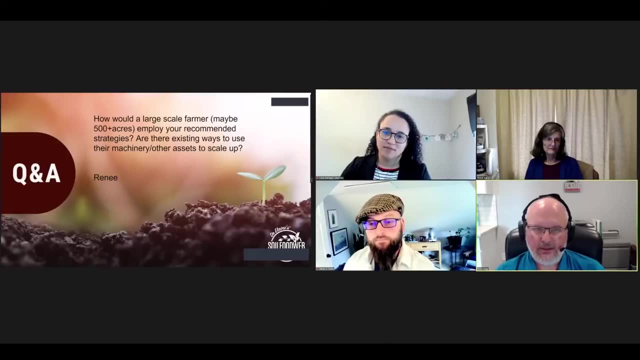 Let's move to the next question. Okay, This question is from Renee, And Renee says: how would a large scale farmer, maybe 500 plus acres, employ your recommended strategies? Are there existing ways to use their machinery, other assets to scale up? 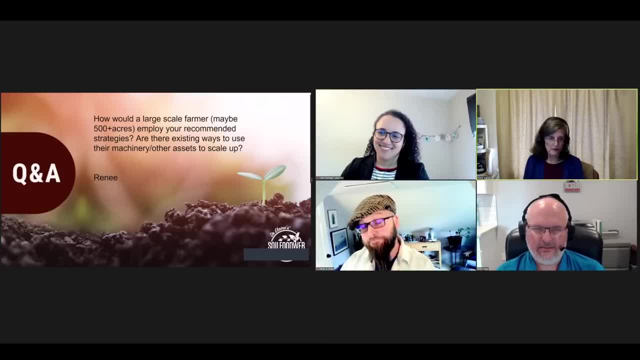 Let's say, you panelists- Yep, The answer is yep. We work with large and small scale farmers around the world. We have some people that we're working with that have you know 50,000 hectares of land Or 50,000 hectares? you know 40,000 hectares, 40 hectares? 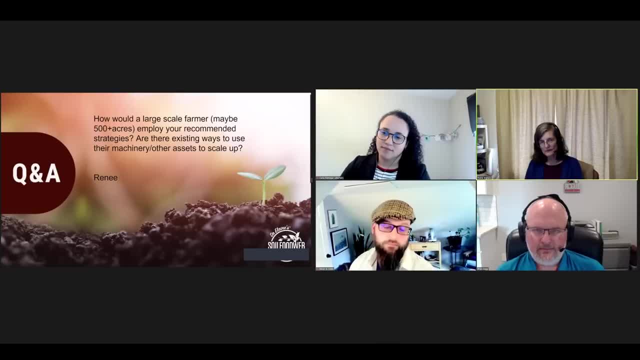 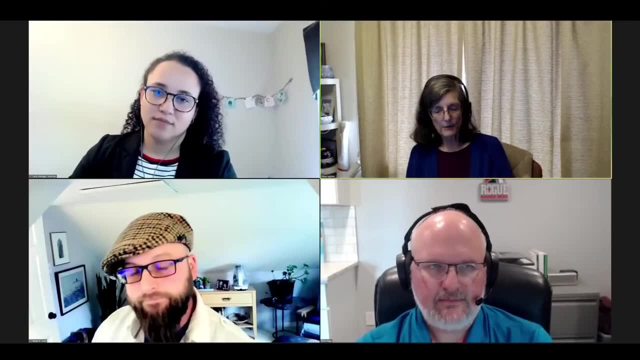 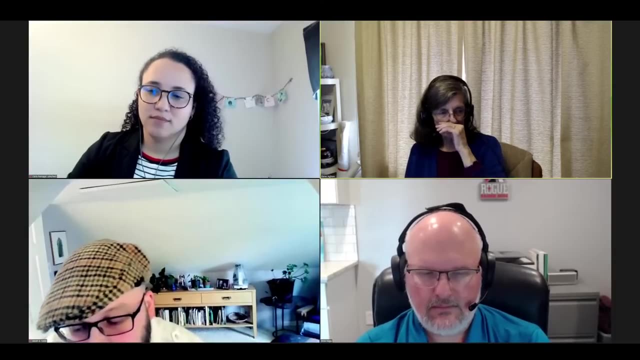 So the whole gamut, And so it's the same mindset. We have to test the soil, find out what's missing, Make the compost So we've got the organisms in that compost material, And then add that into the soil. You've got to be testing that soil and making certain that you have the right materials. 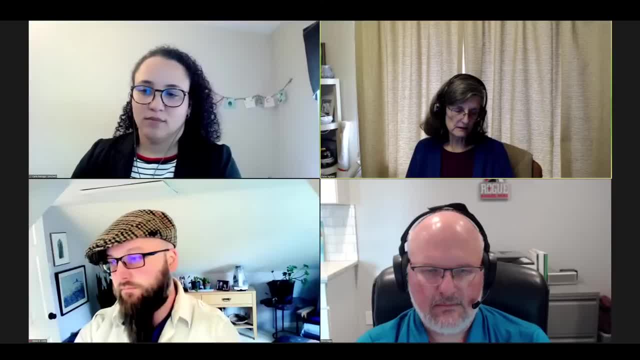 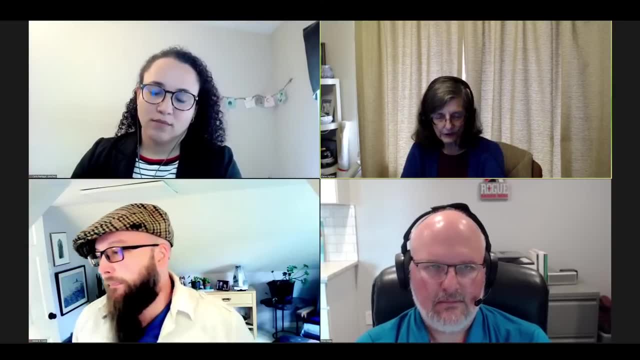 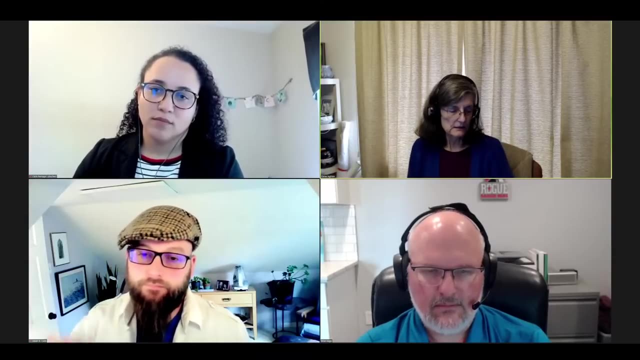 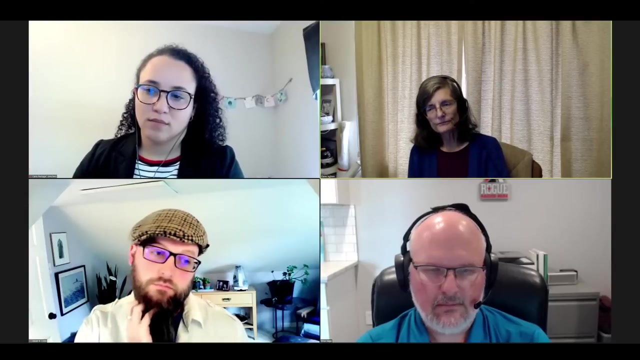 you have, you're putting back in the organisms. you know which organisms are still missing. so you keep working on that until you get the balances correct for the plant that you're trying to grow, based on successional understanding, successional processes, you know. so we're always discovering new ways of doing things, new ways of getting these. 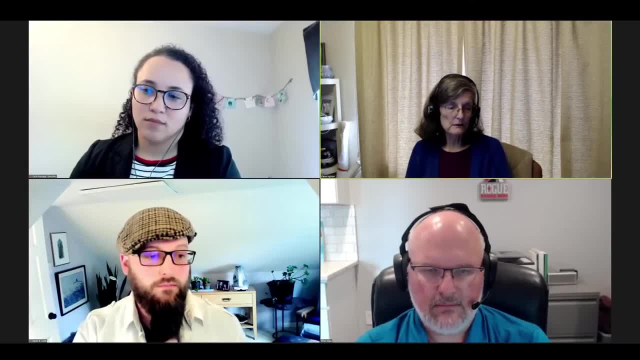 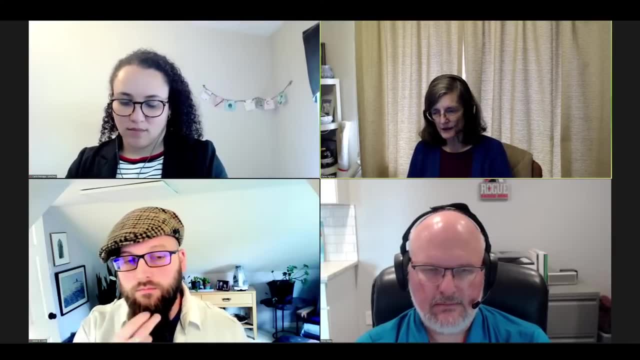 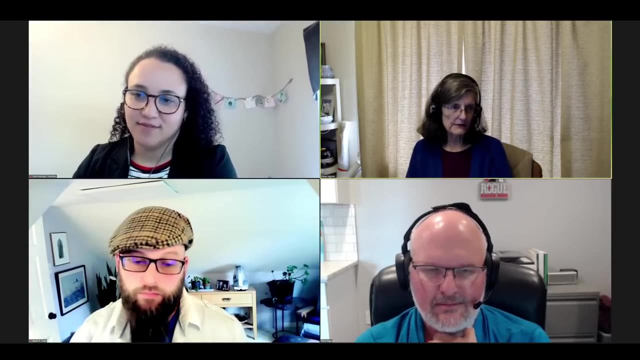 large-scale systems up and going, but we have quite a few places where in the first year that they shifted to working with us in the methodologies out there and just make sure that when you come to take the classes that you let it be known or that you are large-scale growers and 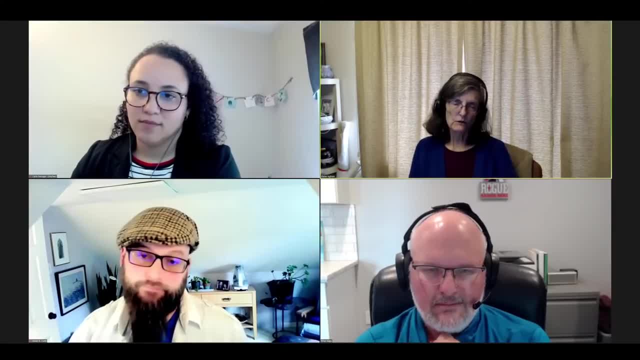 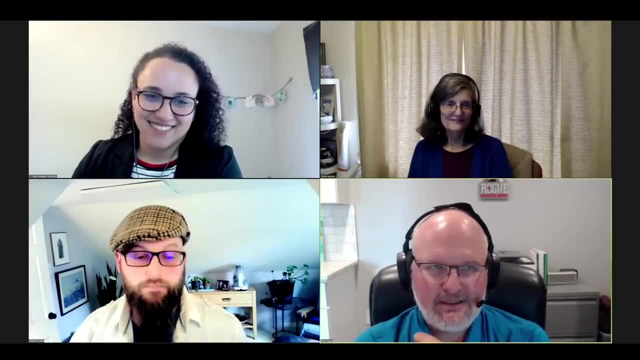 that's what you want to pursue and hopefully we'll have the advanced class ready for you by the time you get there. you know this is a common misconception that i i come across all the time, which is: you know it sounds like what you're talking about. it's really good. 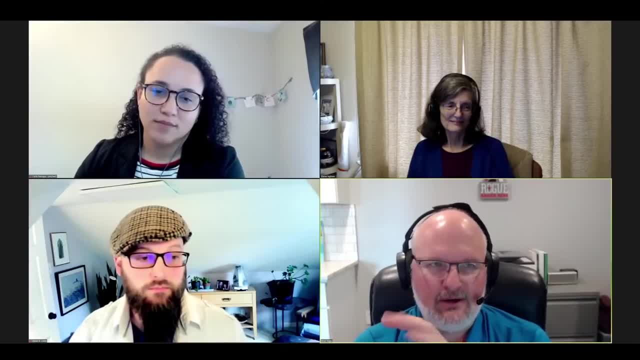 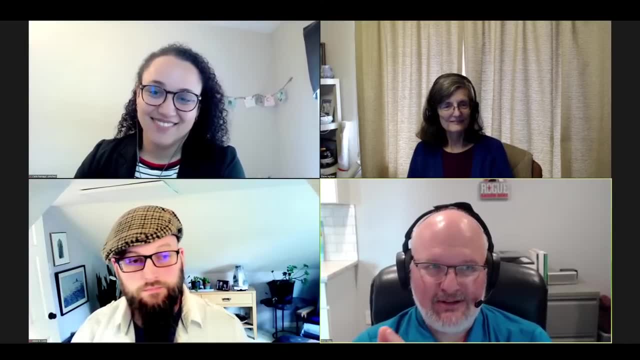 for the backyard farmer, for the homesteader, for the market gardener. but you know, at my scale operation this doesn't apply and it's like: no, no, you really don't understand. it really truly scales to a very large, it's the largest scale farming that you could possibly imagine. uh, this scales. 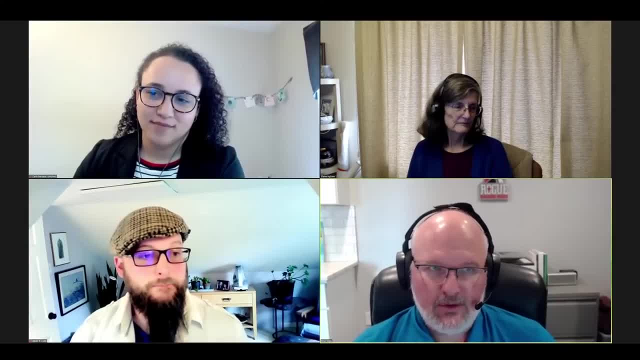 beautifully well and in fact, a lot of times when we go through, i'll go with the client and say: you know i'm going to do this and i'm going to do this and i'm going to do this and i'm going to do this. let's go assess all of your equipment that you have, and we'll find that for the vast majority of 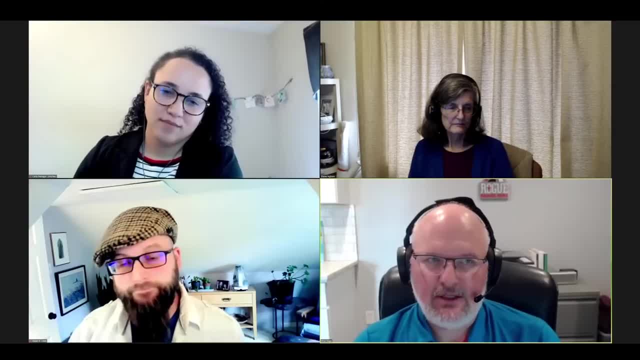 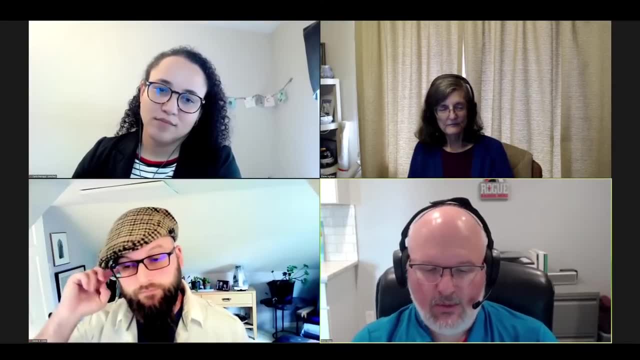 it. we can either use it the way it is or there's just some minor modifications. maybe we have to swap out a pump- you know something similar to that- or swap out some of the the tubing or piping and things like that, and so, in reality, a lot of the existing machinery we can use or reuse. 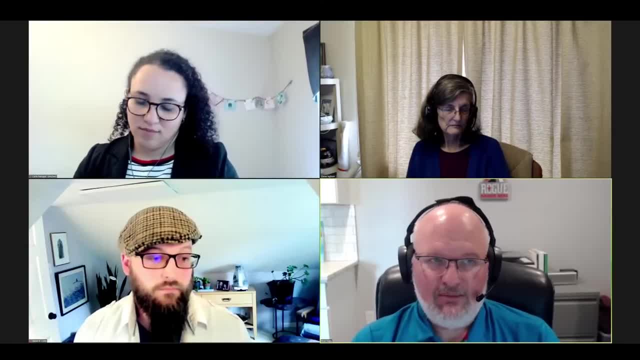 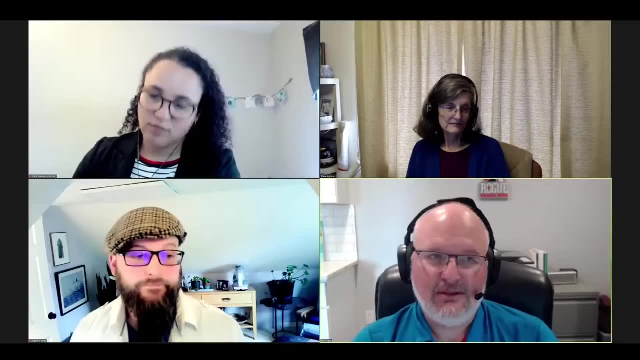 now there's just carry it to take. you know they're going to put, you know, glyphosate out in one part of their field and you're going to use those same spray rigs, all right. well, you have to be very meticulous about how you're sanitizing and cleaning and doing those. 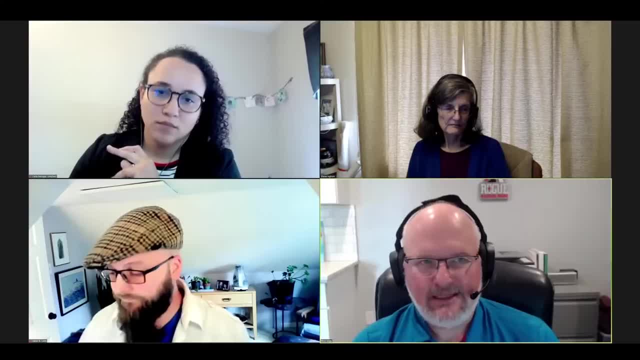 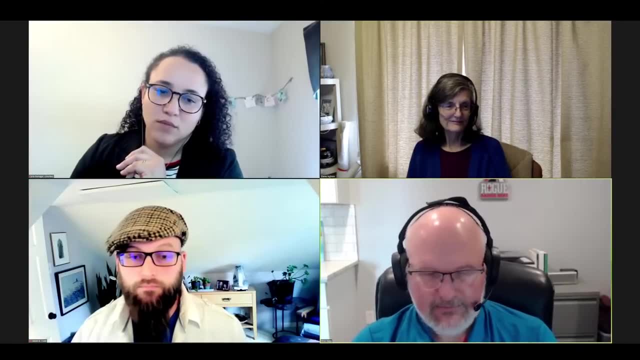 kind of things. so there's some additional processing work you need to do, but that's minor, but that's usually well within the realm of any kind of farming operation to put those things into place. so, yeah, so it's about a good plan. right, investigate what you have to define the adaptations. 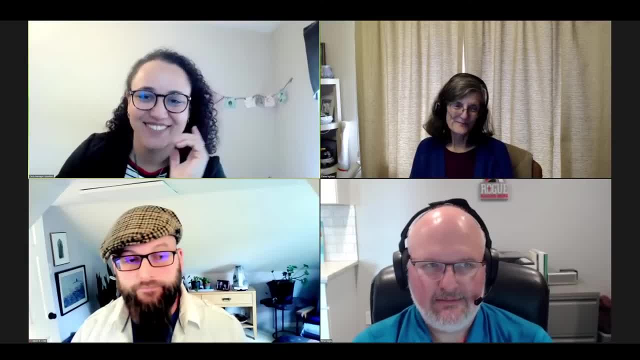 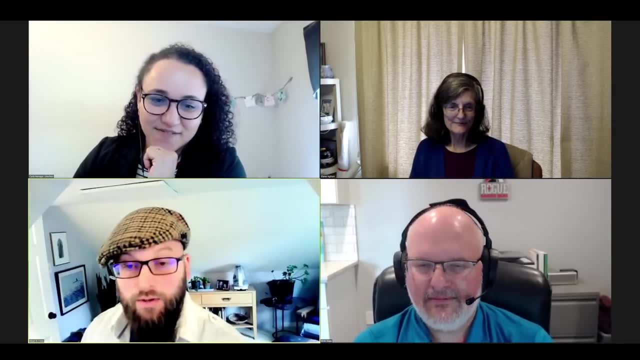 and work. it's a lot of work, no matter what, right, yeah, and i would, um, i would point back to- i mentioned it in my talk a little bit earlier, but i would point back to, i mentioned it in my talk- the january webinar series on our youtube channel. i believe the third or fourth webinar in that. 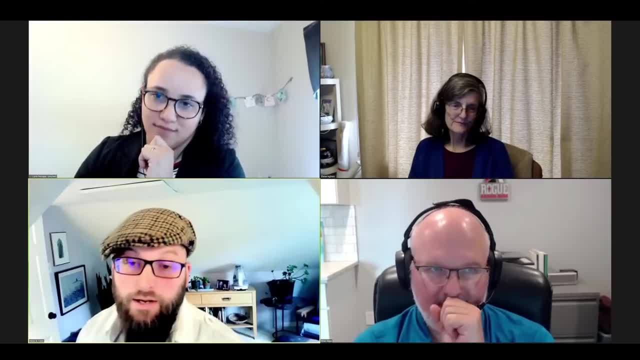 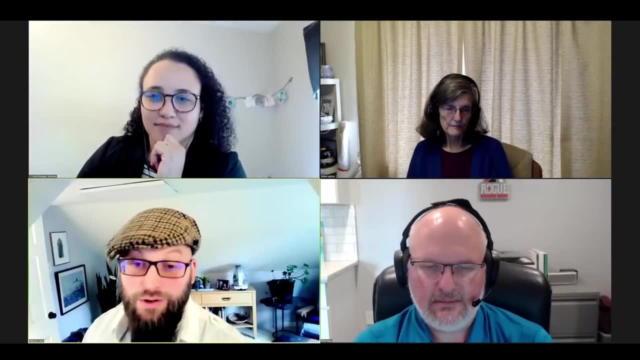 series we had adam york on and he talked about utilizing principles related to what he learned through us and worked through, one with one of our consultants and eventually not only his 10 000 acres but another like 90 000 acres of land around him where he's helping other farmers transition. 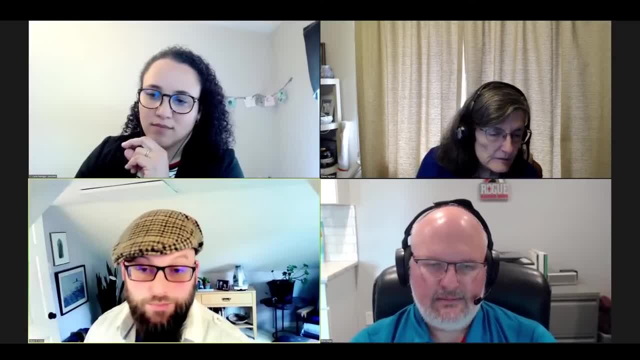 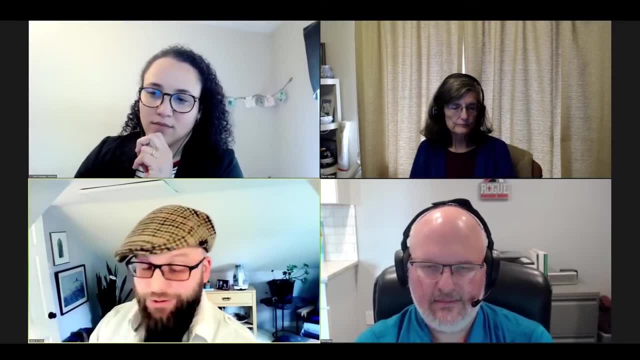 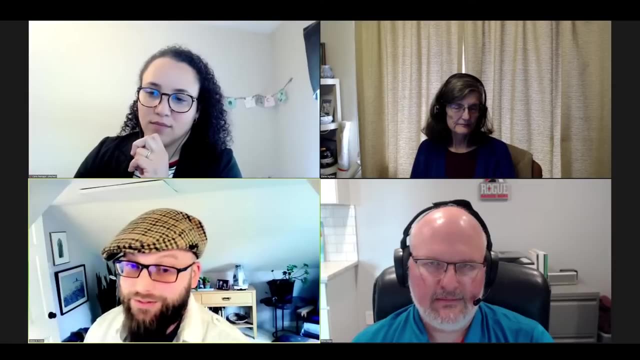 and so you know i think he's helping other farmers transition and so you know i think people sometimes i mean it makes sense that people want to see that it works. so there are pioneers out there that we can go see that it's working and we can. a lot of times when people get on this um track they're really excited about 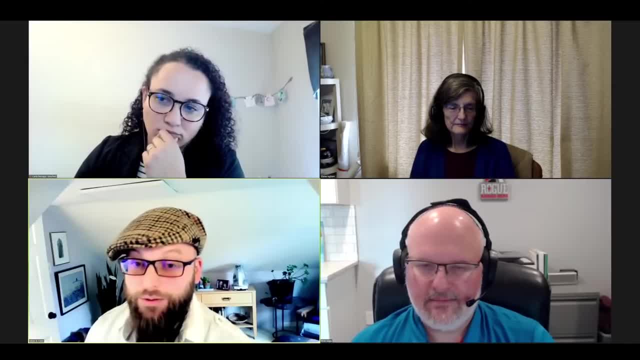 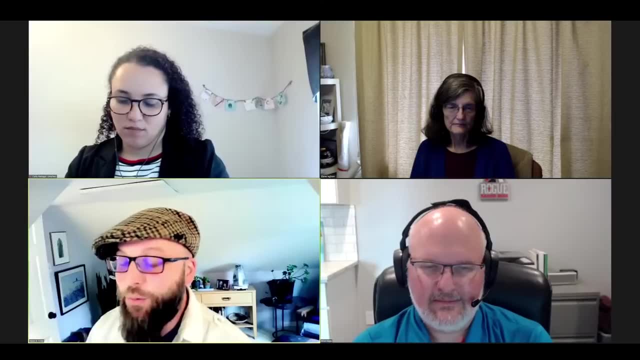 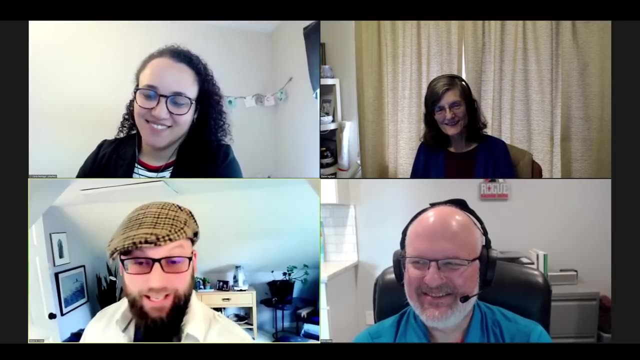 it and they're happy to share. they're happy to have visitors out um to see them. i can't speak for any of them, but i'm saying the regenerative agriculture, um what we call them, the early successional plants in the ecosystem are out there and we can go and and see what they're. 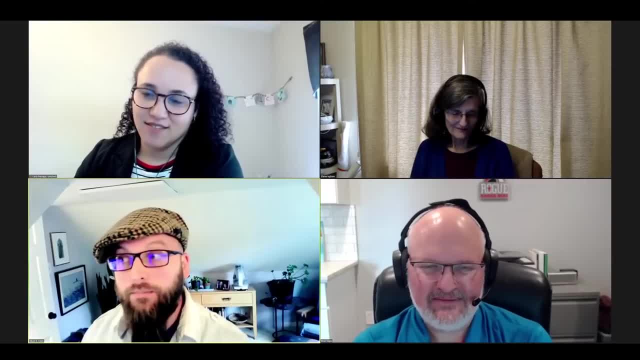 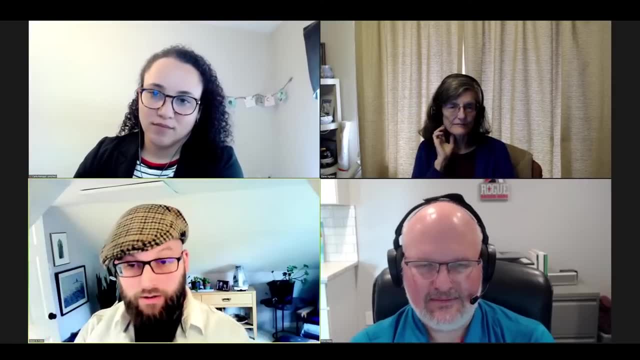 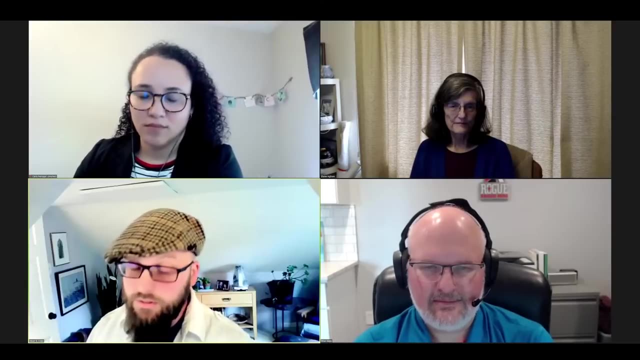 doing and see that it works, and and see which tools. um, each person needs to think through which tools they could integrate today, or which things they need to trial in a small area of land to prove to themselves. this could change things here. this could reduce my costs, because you know all of. 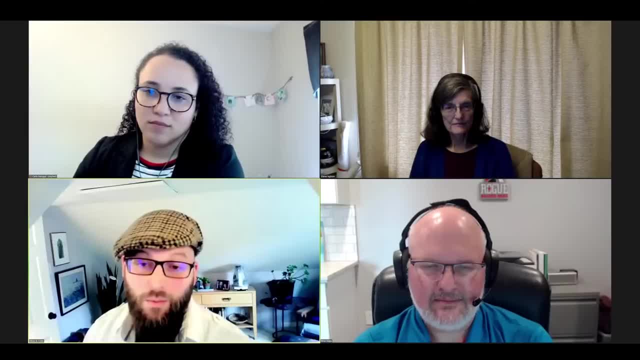 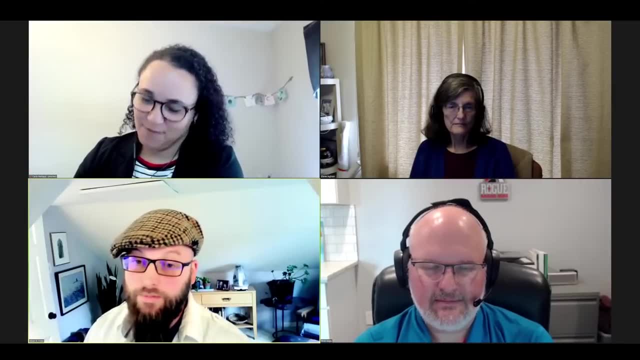 my friends who are farmers and rangers. the first thing they're going to ask me about when i talk to them is: you know, what's that going to do with profitability? and that's an important thing for us to understand. there's there's a reason to be um cautious, but there's a reason to reach for the. 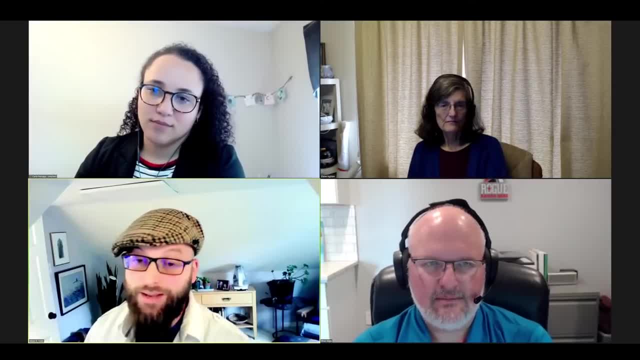 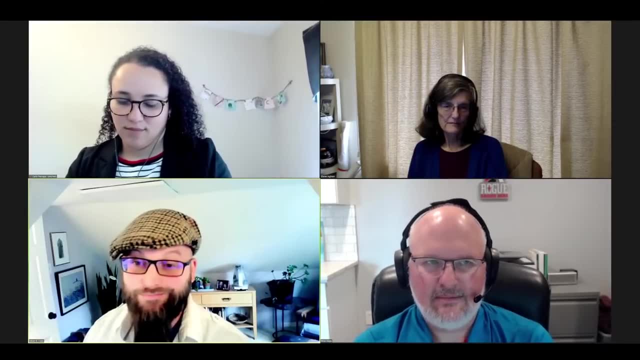 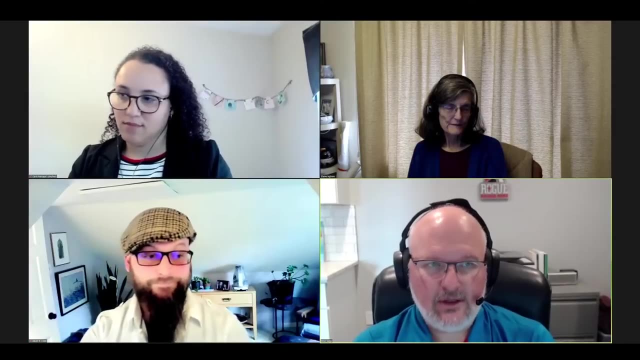 regenerative options as well, because the same old way of doing chemical agriculture is going to increasingly not work in the next few decades. and you mentioned a really important point to the discussion i have with all my clients around. trials is a good example. you know, trials accomplish two things in my mind: um and one. the first one that really, i think most people 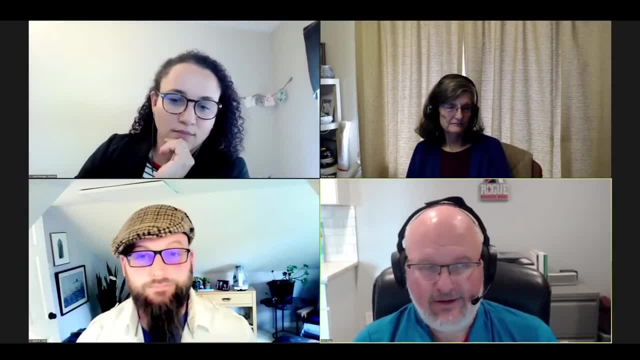 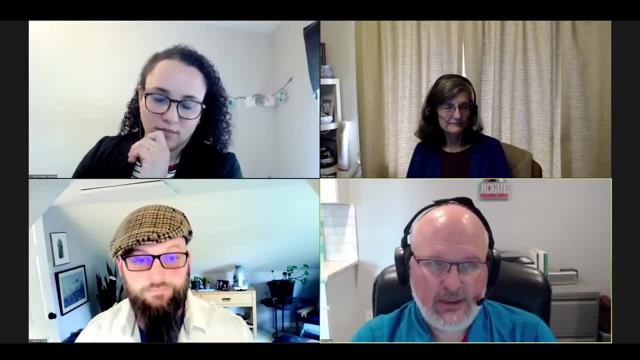 think about trials. prove to me that it works, or prove to myself. you know that where, where you're, you're telling me i need to do to. my farm is going to work and that's an important aspect for for some people. other people are like: i don't need that. i i think i get it. let's go full, full bore. the. 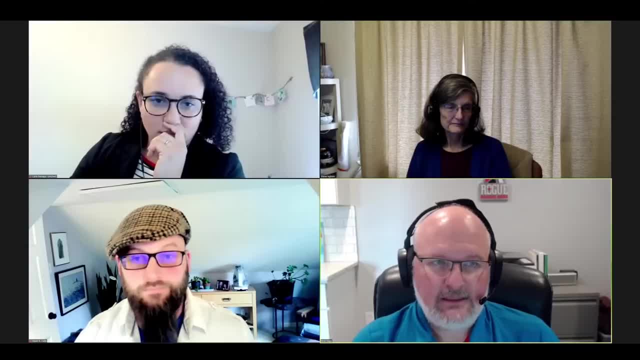 second part of a trial to me is that a farmer will learn at a small scale what are the changes to their operations that they need to do, and then they can think through: how can i apply this now into a large scale? and so trials are always an important thing, even when 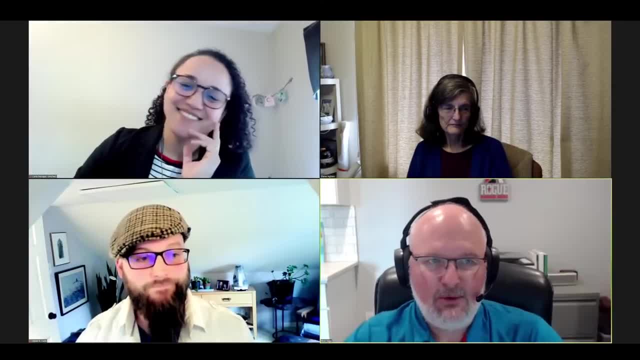 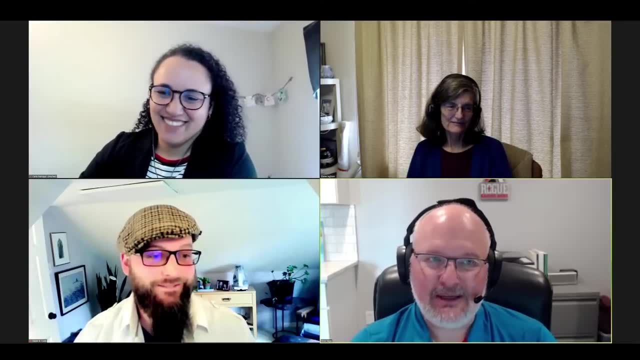 i have clients, i'm saying, nope, don't need trials, let's just go full bore on this. i want to go all the way and i'm like, put the brakes on hold on a second. there's a good aspect to doing a trial, because i want you to learn at a small scale what needs to be done so that when we go to large scale, 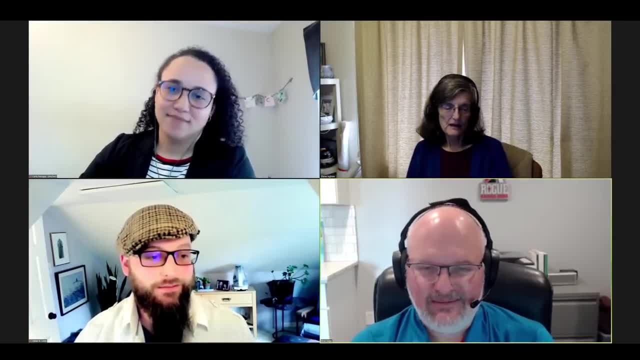 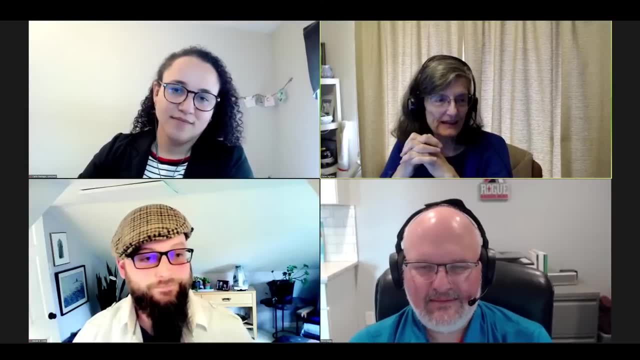 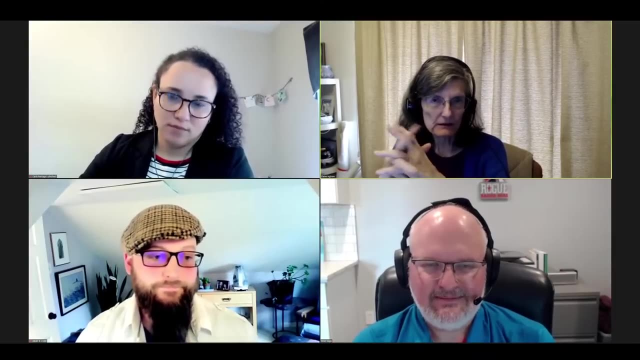 you know all those nuances are already internalized and that all the underlings, the, the in the field can understand what's being done and if, if the field is changing, you know, think about it just in the same context. you know, learning about what's happening in the field, or getting 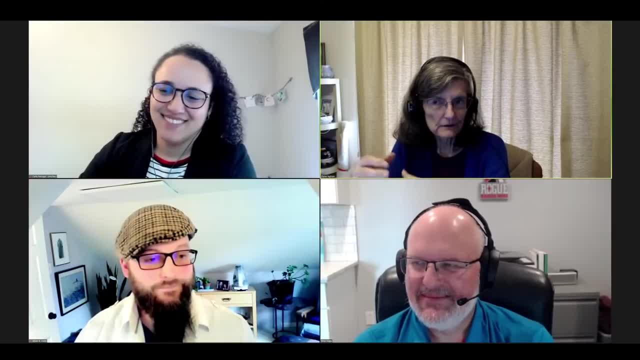 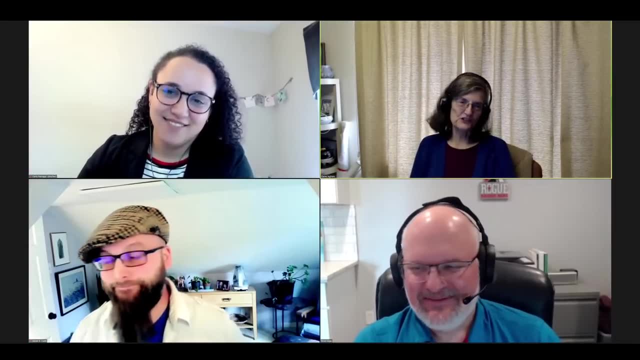 a trial done, and so on, and so forth, and so forth. so the data that we want to get is very important and it's- and i'm very grateful that we have a lot of experts that are doing the trials right now and do the trials on our own, and so forth. so if you can't get them now, i just want you to know. that you can. if you have a farm like this, there's a lot of possibilities. there's is a lot of things to do. it's a lot to do in your own farm, or your farm is very important. if you're, you know if the field is changing. you don't you know if you're looking and also if you're trying to do the trials. 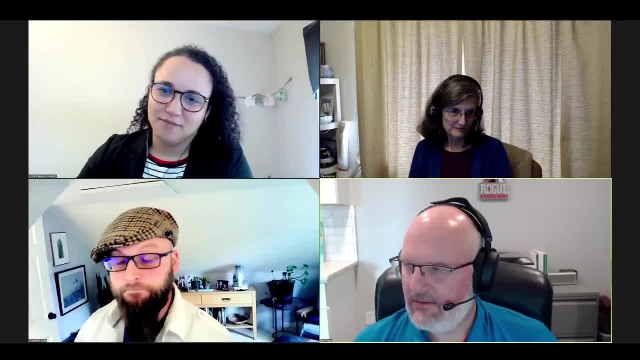 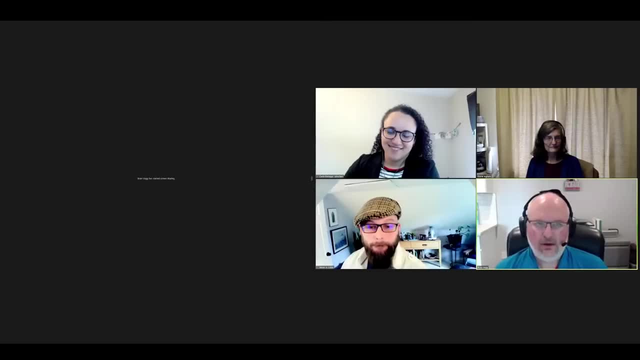 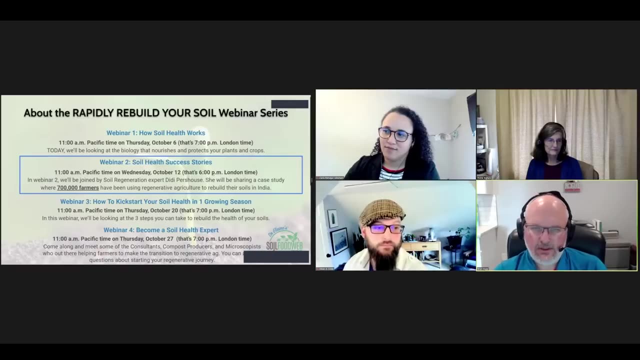 we go ahead and conclude today. okay, so let's go ahead and move on to the last part of our webinar, and really, what this is is just to remind everybody that we have two more- or sorry, three more- webinars in the series for october again, webinar two is soil health: successes stories. 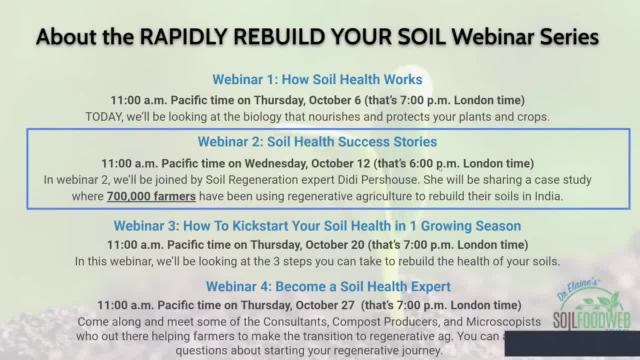 and this is going to be with dd per house as one of our panelists, so that should be a great, great webinar, and that's on wednesday, october 12th. then webinar three, which is how to kickstart your soil health and one growing season, and that's going to be on thursday, october 20th, and then webinar four. 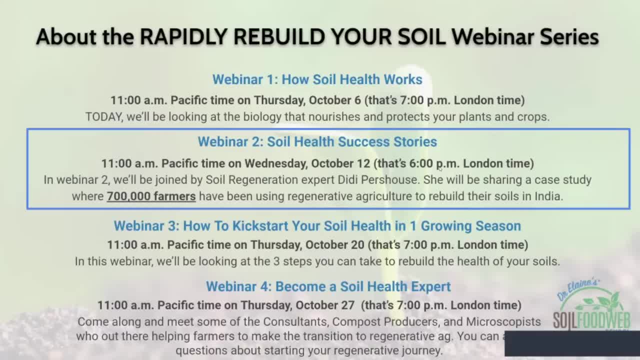 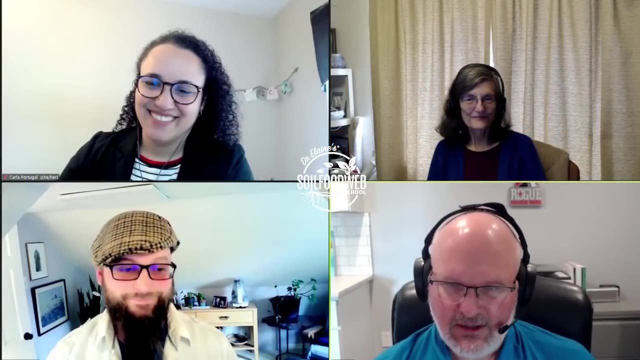 become a soil health expert, and this is going to be getting to hear from people like myself- consultants, compost producers and people are doing lab tech work, and that's on thursday, october 27th, so we hope to see you. everybody here that attended today's webinars and our other. 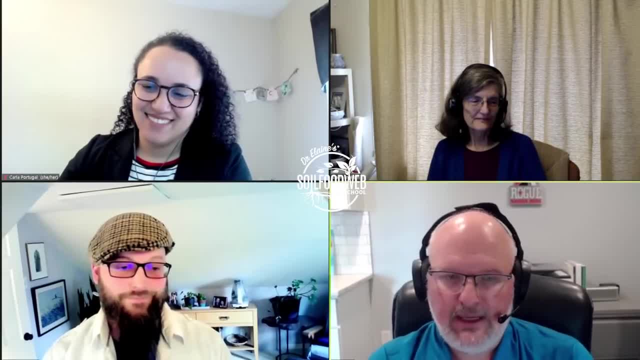 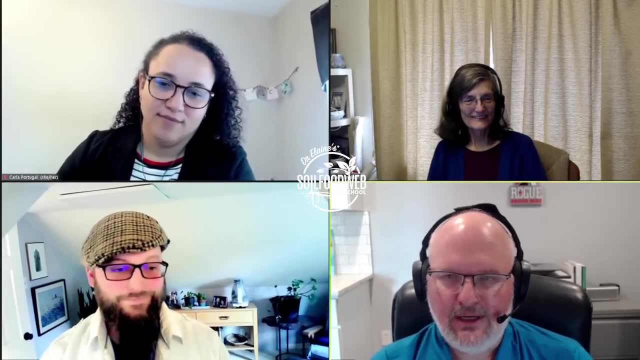 three of the webinar series and, uh, i want to throw out some thanks. so, again, thank you to the audience for attending today's webinar. i hope you enjoyed it and i will see you next time. bye, bye. it's great for us to be able to share our knowledge with you and that you guys.